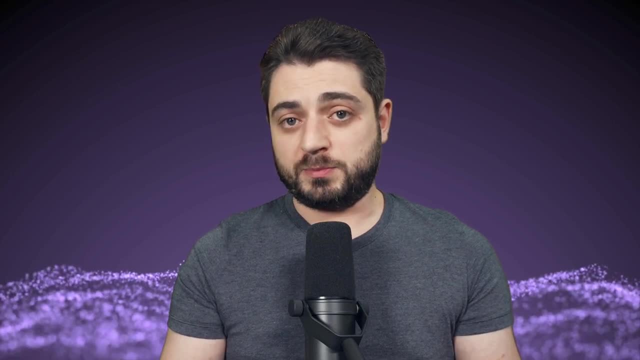 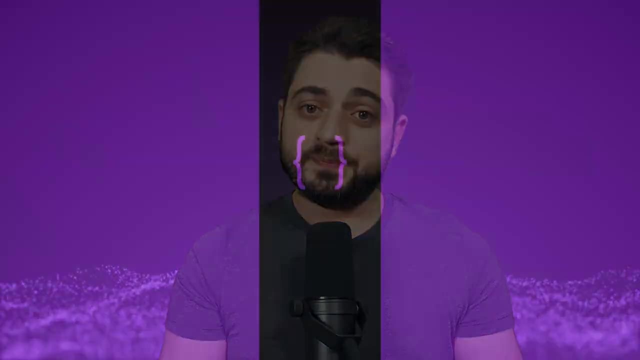 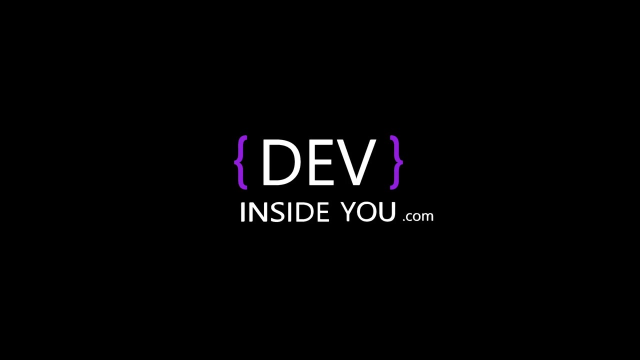 crash course. In fact, we'll cover pretty much everything you need to know about functional programming. Now that I'm thinking about it, I might as well call this video like this: Yeah, I think it sounds good. Anyway, let's roll the intro. Hey, Vlad, here from devinsideucom, Welcome to another video. Now, this is mostly a Scala. 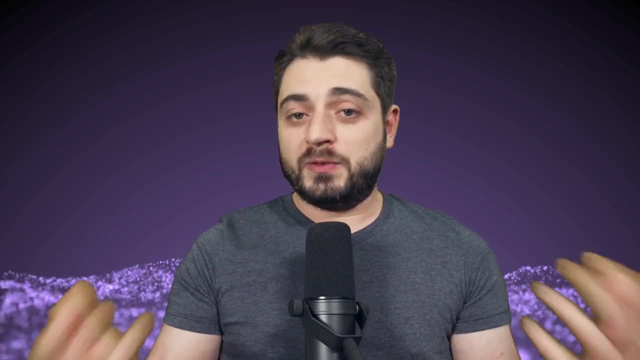 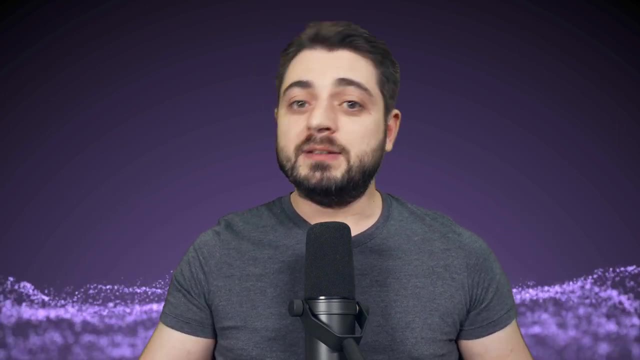 channel. however, if you stumble on this video for any other reason, don't worry. most things are applicable to any other language and since you're new to Scala, allow me to welcome you to the Scala community. Welcome. Scala was one of the first, and it might actually be the only. 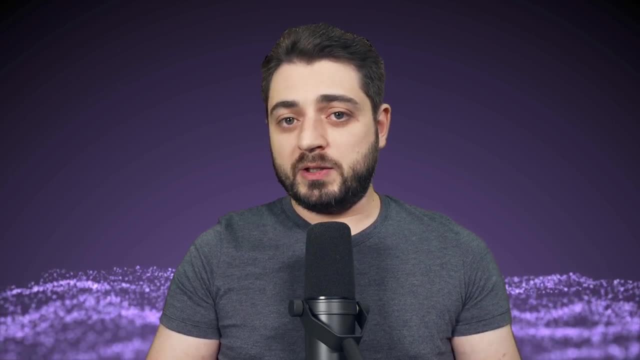 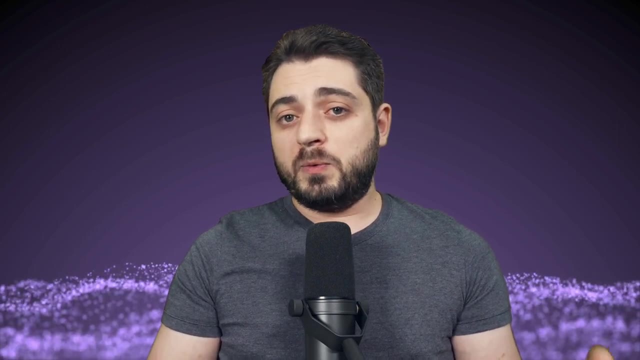 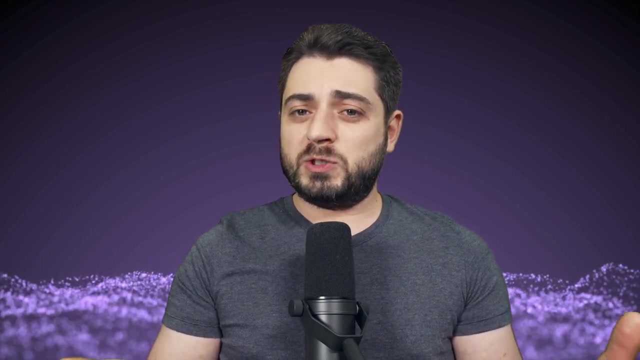 programming language out there that successfully managed to combine the object-oriented and functional programming worlds in a seamless way. Now, nothing is perfect in this life. everything has trade-offs. One of the challenges that this, even though successful- mix poses is the fact that now you, as a programmer, are left with too many choices for building software. 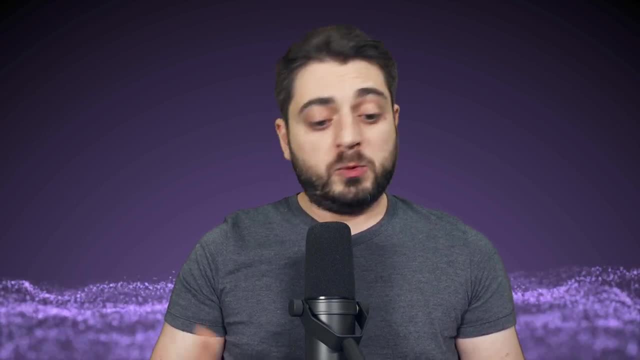 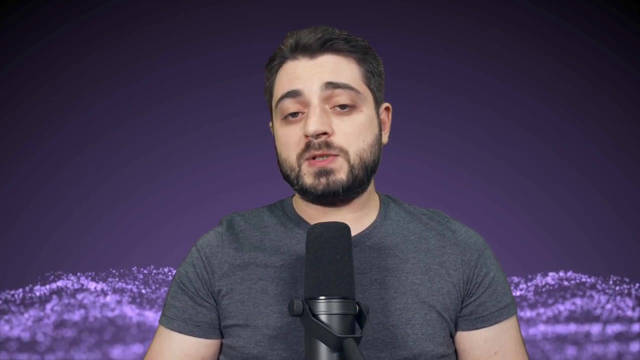 and so, since the beginning, the always evolving Scala community was searching for the best way to do it. Now, since you're new to Scala, there will be a lot of by the ways in this video, and here's the first one. Even though Scala is a general purpose programming language, 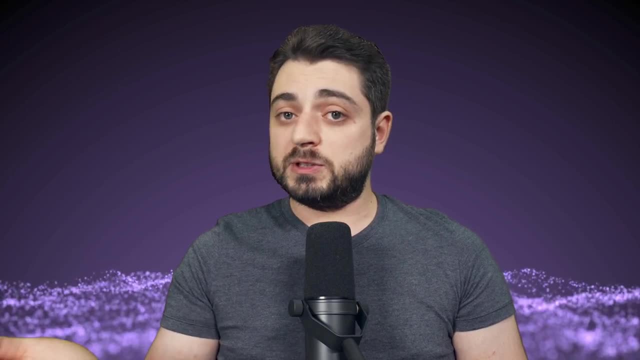 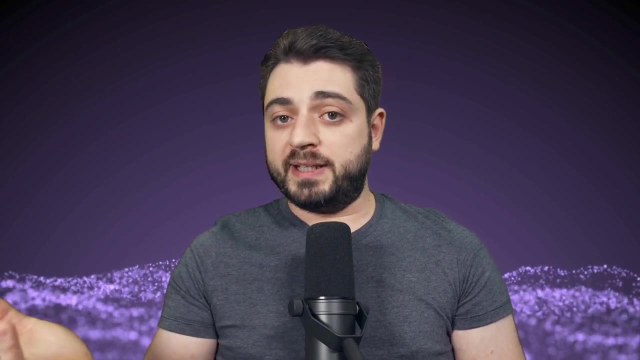 it found its niche in a, wherever java found this niche, which is in the back end of web applications, which is also what this video is concerned about, and b, in the world of big data, which is not what this video is concerned about, since I'm not a data engineer. If you're serious about diving, 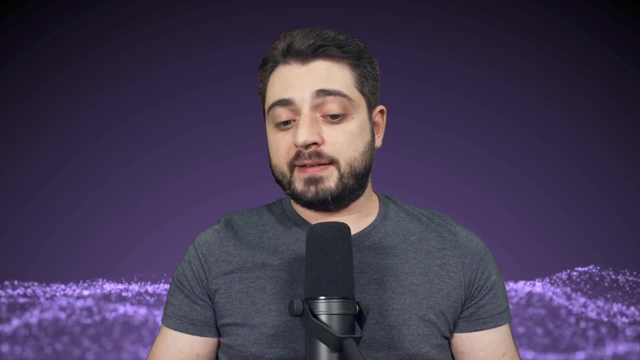 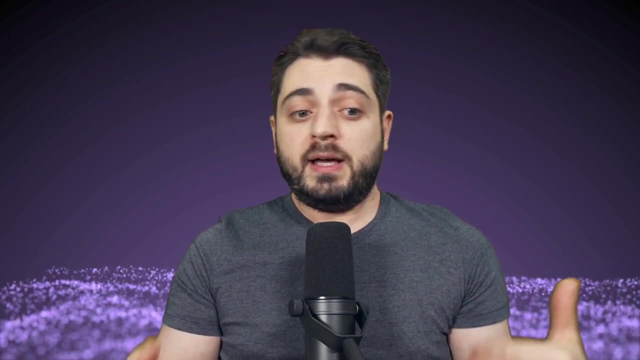 in the world of Scala. rather sooner than later, you will discover the fact that we have a lot of tax tags to choose from. some of them lean towards object-oriented programming, some of them lean towards functional programming and some of them are somewhere in the middle. Now back-end applications. 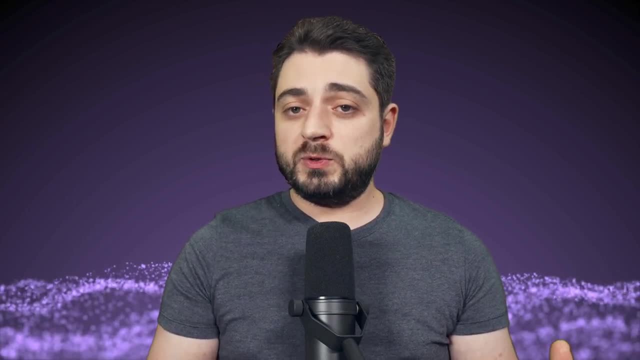 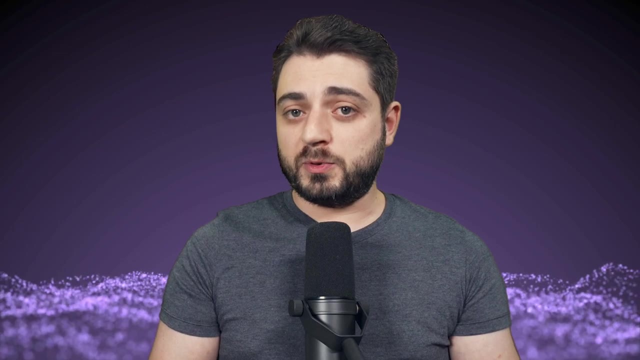 tend to grow over time, and functional programming offers solutions for maintaining large pieces of software, and so over time the scale of the software will be much larger and so the scale of the software will be much larger. Scala community lean towards pure functional programming. We will talk about purity later in. 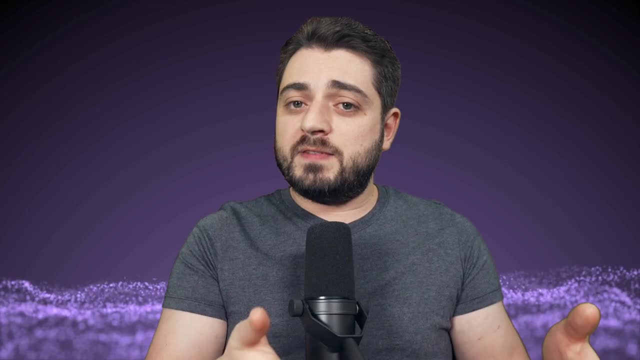 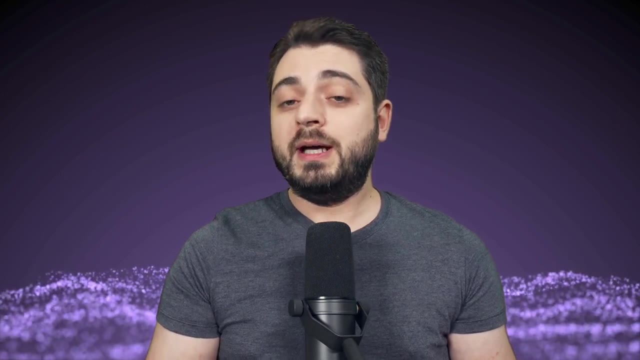 the video, but the point I'm trying to make is that even within this functional niche, you still have choices. So one of the goals for this video is to help you choose, and the way we're going to go about this is by explaining the appeal of functional programming in a non-hand, wavy way. 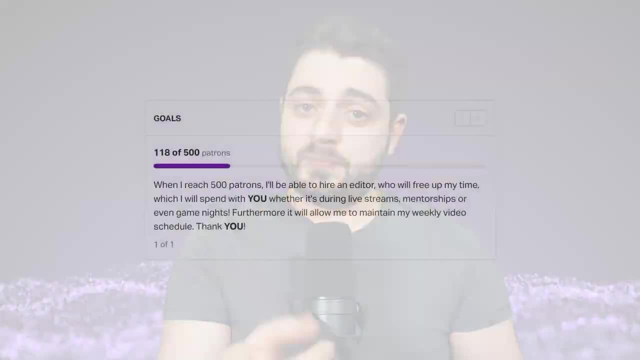 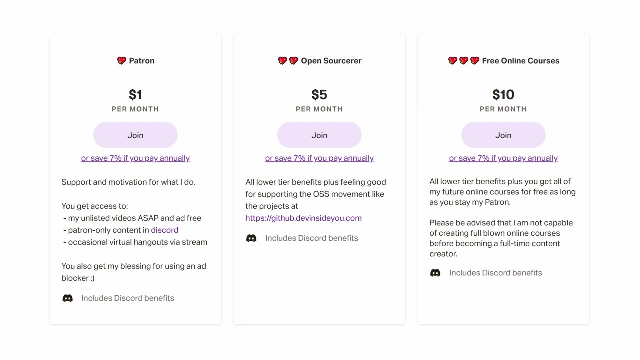 Let's begin right after the message from our sponsors, which is you, the people who support me on Patreon. Without you, I wouldn't be able to pay for my video editor, who allows me to spend more of my time to hang out with you doing live streams or answer your questions on Discord. There's many. 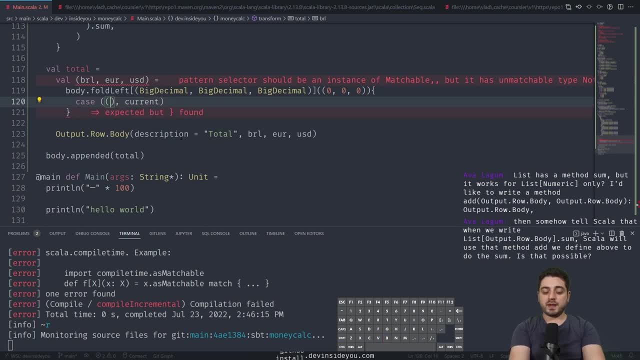 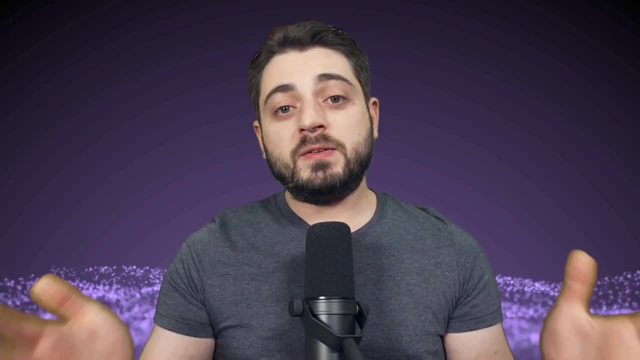 of you and only one of me. so every dollar counts because eventually it adds up. Special thanks to Fred, Albu and Johan for being my highest tier patrons. Thank you. Now let's talk about functional programming. First and foremost, I already made a video about programming paradigms, so you might. 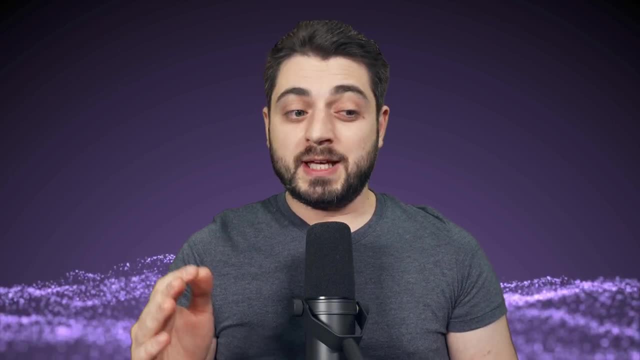 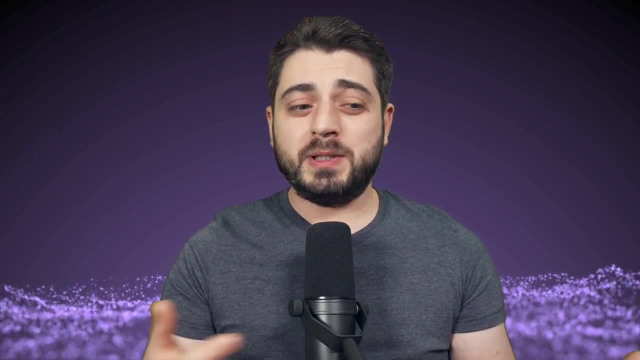 want to check it out. Also, I made a Scala crash course which is three and a half hours long, so you might want to check it out as well. By the way, guys, the theme for this video is to be sort of going to move pretty fast. okay, This video, even though it is for beginners, it's not for absolute. 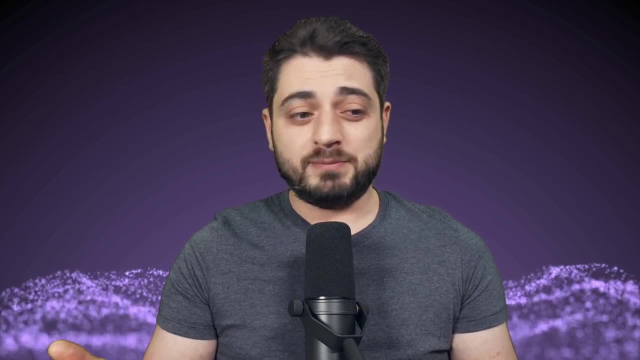 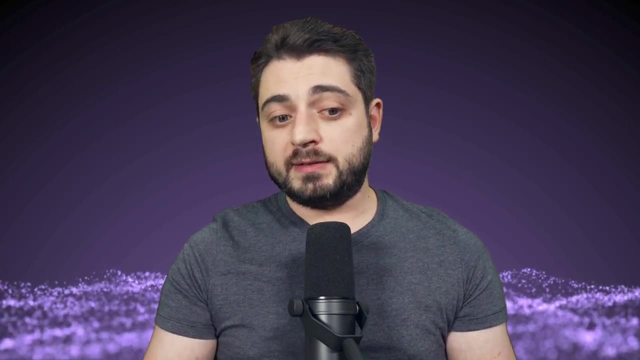 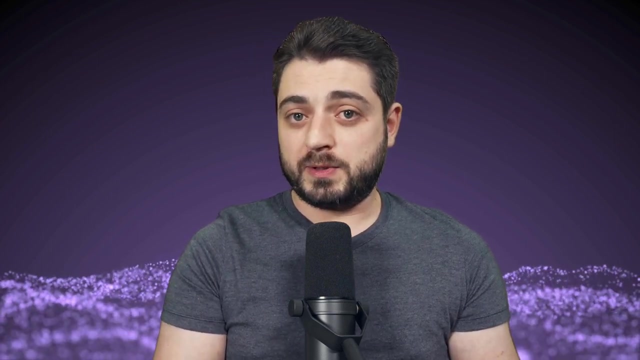 beginners like I hope that you have, like maybe a year of experience in some other language. Now, what is functional programming? Well, functional programming, same as any other paradigm, is a set of constraints, aka a discipline that we, the programmers, follow to maintain potentially large pieces of software. Now, one important thing to keep in mind is that this discipline 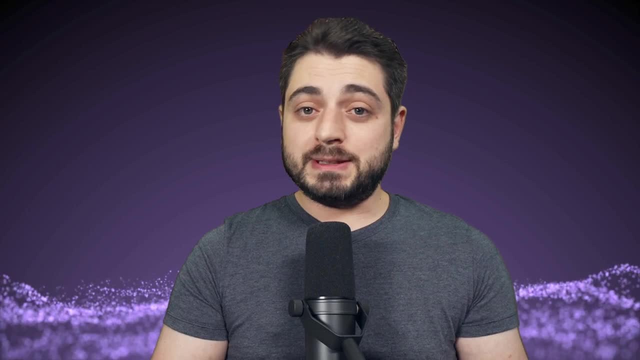 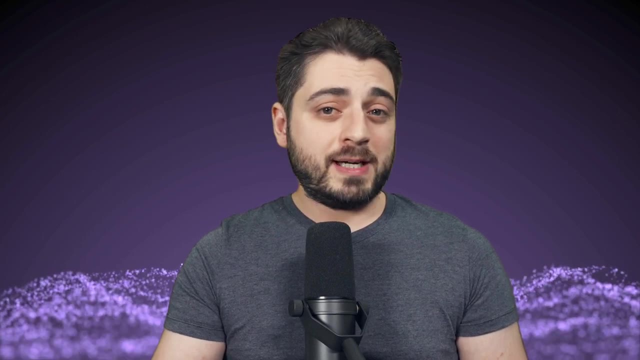 is imposed on you, the programmer. Now, programming languages, type systems, tests and other tools are useful, but at the end of the day they're not bulletproof and if they were, would have Skynet and you wouldn't have a job. Now, every discipline has a cost and functional. 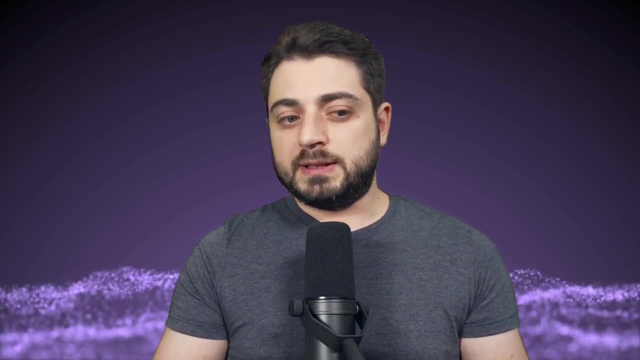 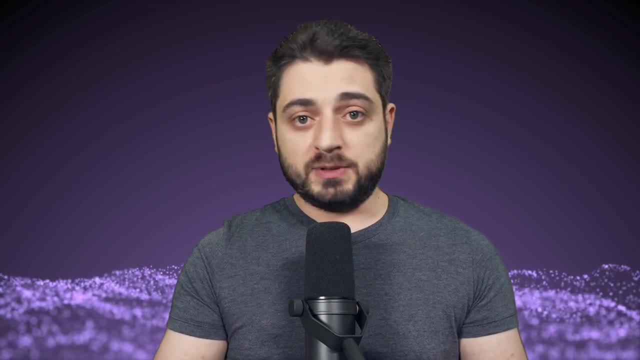 programming is not excluded from the statement. It's only worth the price and thus valuable in large, always changing applications. In fact, this is what software is all about. right, It's about change. Software is easier to change than hardware. Now, what is the value of functional programming or in other words, why would we constrain ourselves to follow this discipline? Simply put, as a programmer, we have many things to worry about, and functional programming removes some of those worries. It reduces bugs and prevents regressions, thus giving us more confidence when we want to change our applications, which is something that happens all the time. but remember, it's not. 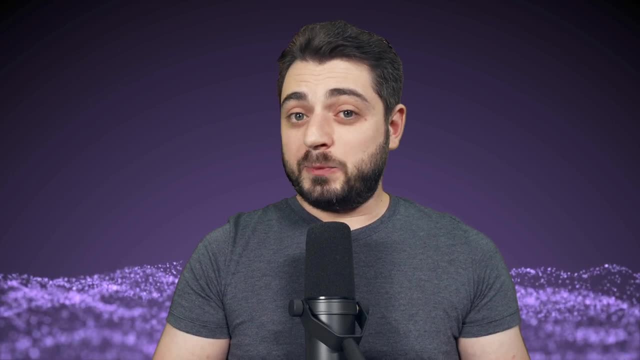 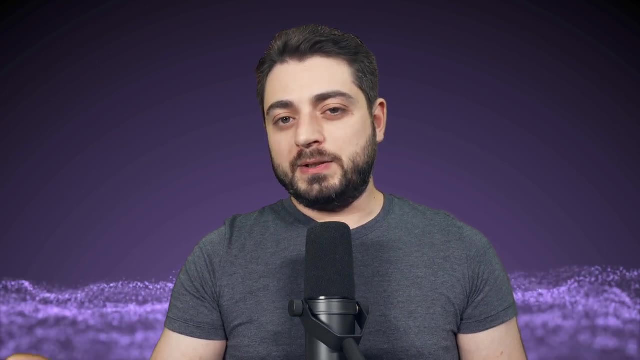 bulletproof. Now, what is this constraint, though? What is it exactly that we need to give up Now? the answer to this question is assignment, but it doesn't really help you, does it? This is also the reason why, usually, when FP is presented, you're just bombarded with buzzwords like immutability. 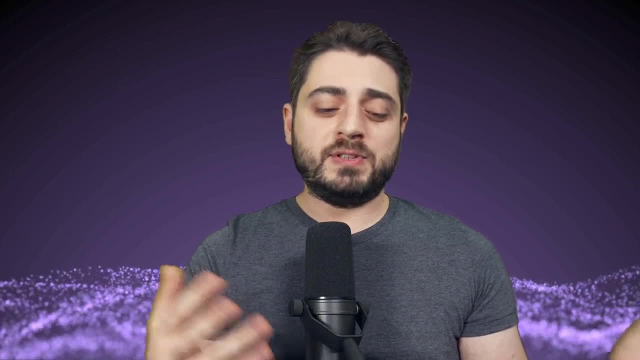 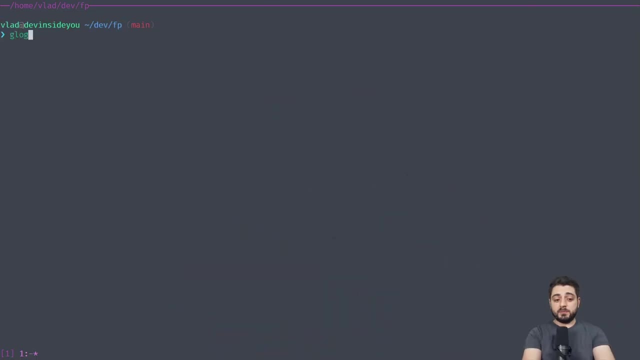 helps with concurrency, and there's talk about recursion and lambdas and referential transparency. as I said, many buzzwords. instead of giving it to you straight, What I have for you today is a repository with 32 commits and we're going to go through all of them. I used to do all of this stuff. 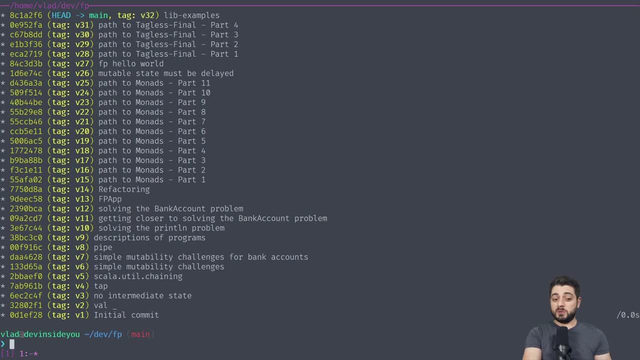 live, but it turns out that typing takes a lot of time and this video would be like three hours long. so we're going to simply run through 32 commits over here, and this repository is also going to be on github, and if this video turns out to be too long, I'm going to cut it into two. The goal is to 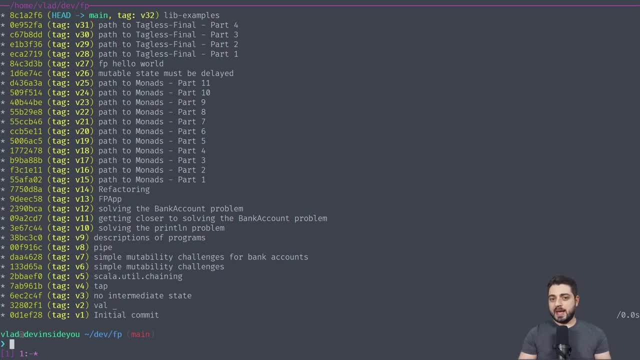 focus on the question that most FP beginners have, which is how to do an immutable print line, and somewhere along the way, we're going to define functional programming very precisely. without any hand waving. Let's start going through this repo. So git allows you to only go backwards. 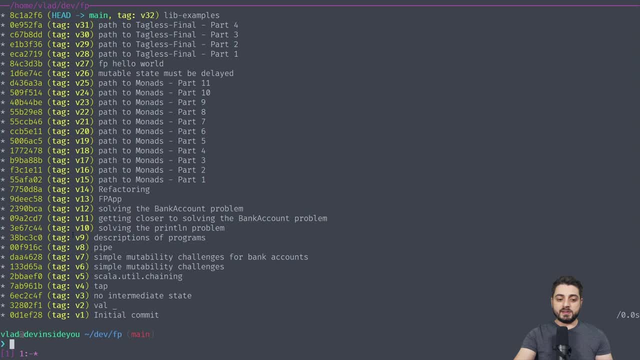 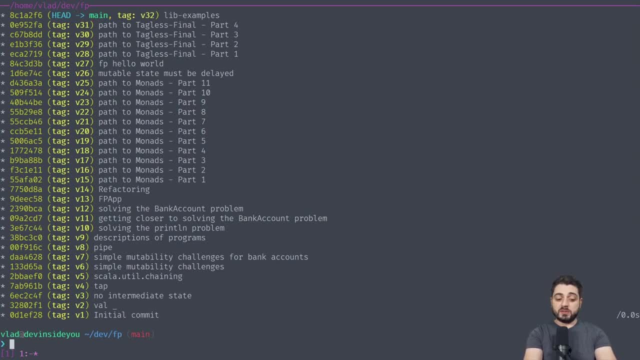 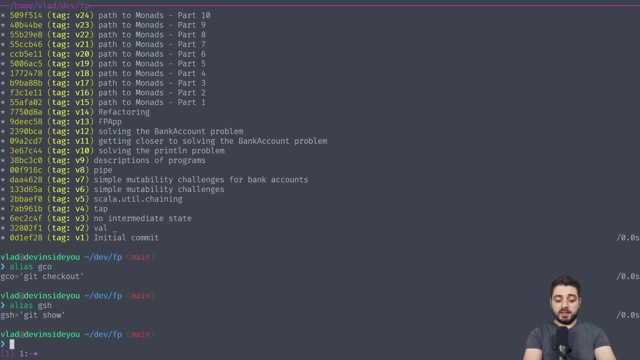 plugin which comes with a bunch of aliases. so today we're going to use a bunch of uh git aliases, okay, so I'm going to show you a couple. so gco is git checkout, uh, gsh is git show and git show. hyphen s is like git show. you know short, and yeah, this is pretty much all we're going to need. so 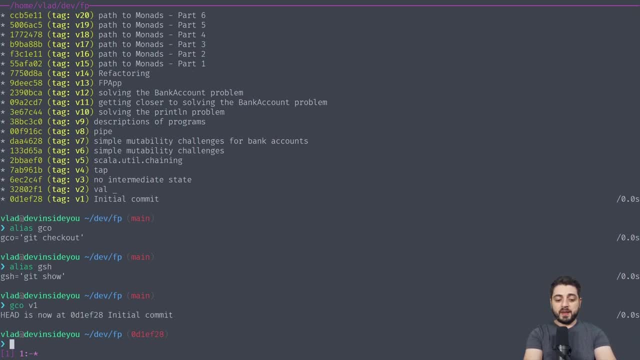 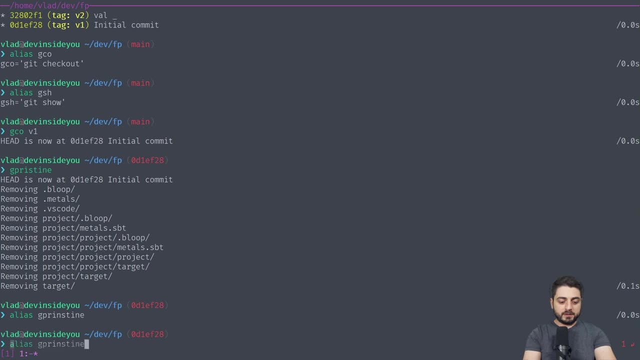 what I'm going to do is I'm going to check out the v1 right, and I'm also going to do gpristine. uh, gpristine is pretty much going to remove a bunch of stuff that is like uh, laying around. hold on gpristine. 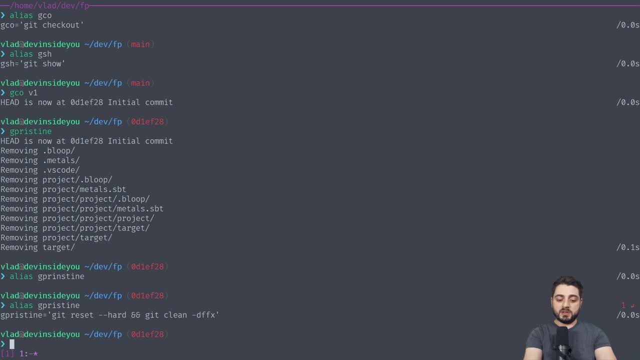 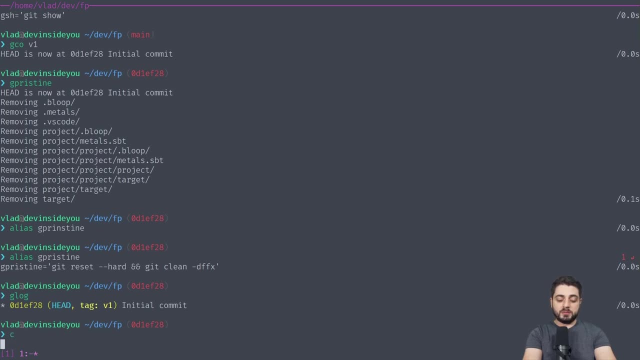 like this: okay, so it's basically git reset hard and also git clean with a bunch of flags, okay, so, as you can see where now I you know if I do log it, you know the hat is over here. so this is the initial commit. so I'm going to open it with visual studio code and I'm going to show you what we have. 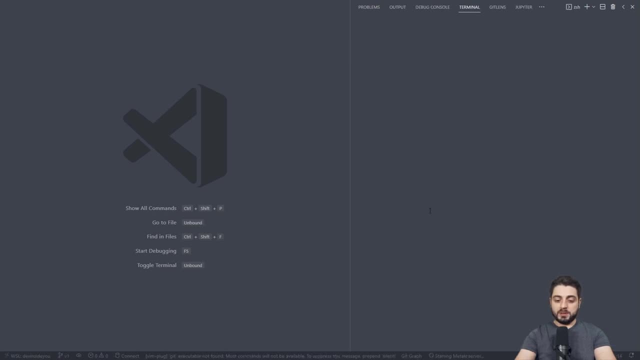 while it's loading, we're also going to uh import the- uh, the build project. I'm going to give you like a couple of pointers about Scala, but ultimately this video is not necessarily about Scala. uh, it's not about, like, the build tools and anything like this. but you know you're a beginner, so I'll try. 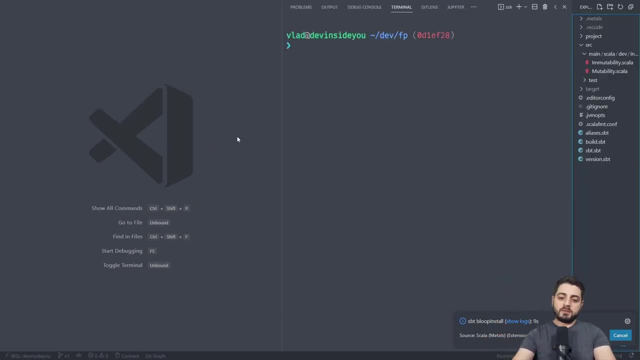 to give you like a little bit of something so that you're not completely lost. what we have over here is like is the terminal, and over here is my uh file tree and, as you can see, I prepared two files. one is called mutability and the other one is called immutability. so what we're going to do? 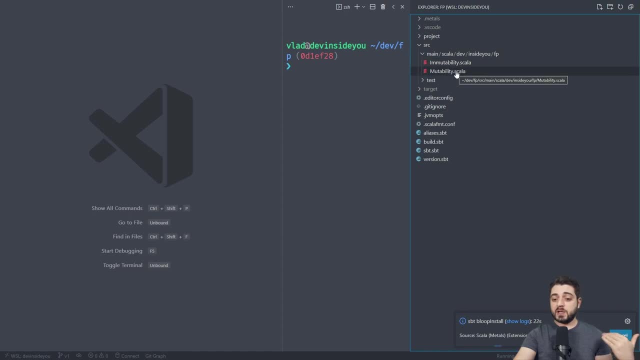 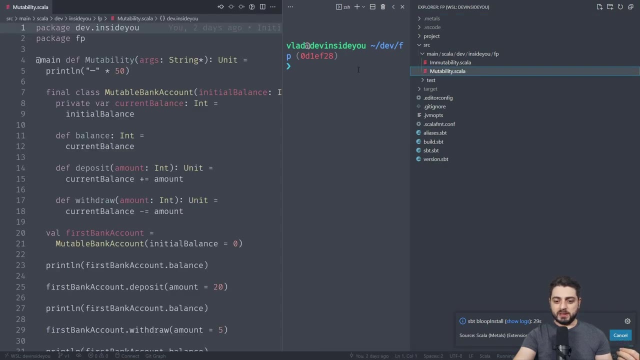 is we're going to run with a typical uh banking account example. I have two versions: one is immutable version, another one is immutable one and I'm pretty much going to use them just to just sort of explain to you. you know the, the Scala syntax and stuff. okay, in fact. 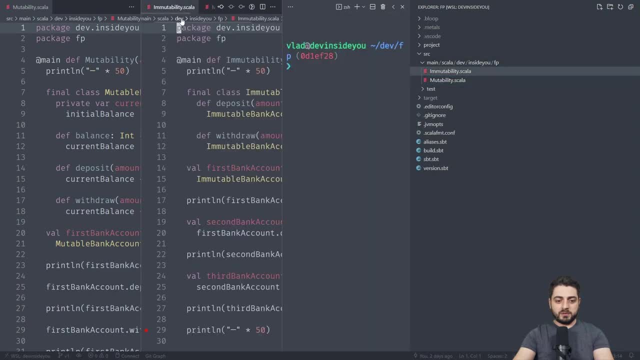 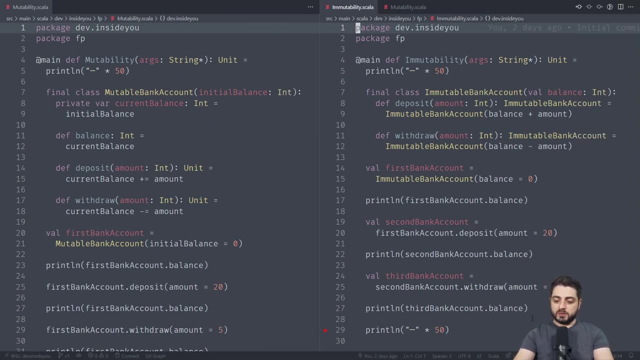 maybe I should do this and I'm going to throw like the immutable over here and go like this, and for now we're going to disable the the console like this: so once the built uh tool finishes compiling uh, we're also going to have a buttons over here for running. 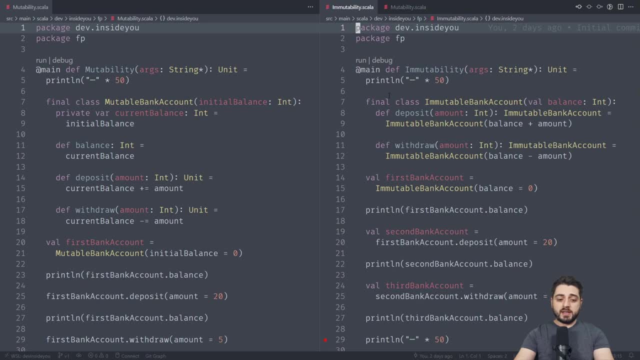 and debugging, but we're not interested in that at all. we're using Scala 3, which has, uh Python based indentation syntax. so, for example, this is a class and, uh, this here is a body of the class. it's indented, uh, by two spaces and there's a colon over here. uh, the syntax came in in Scala 3, okay. 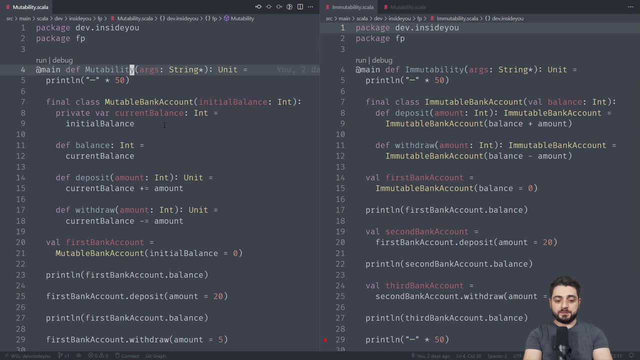 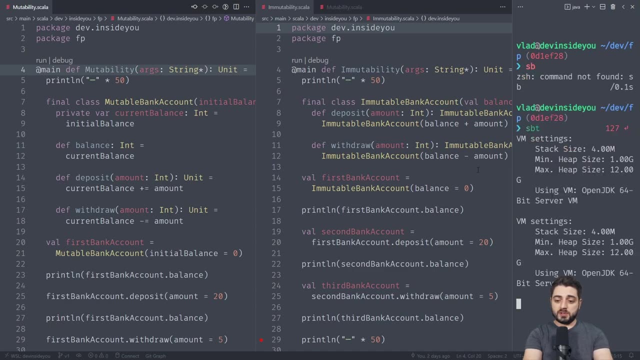 so, uh, this is pretty much a main method and, um, this program pretty much creates a bank account, mutates it a little bit. uh, in fact, we should probably run it. so I'm going to launch SVT, which is, uh, Scala's build tool, so we're going to 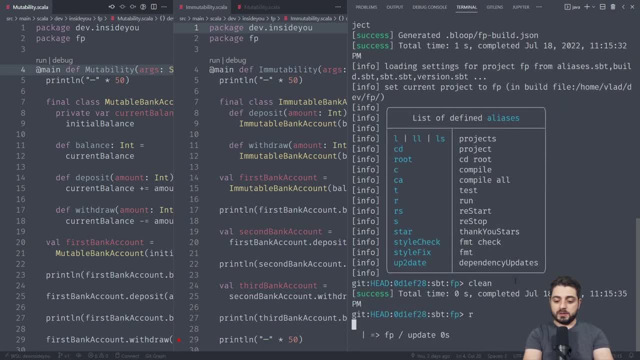 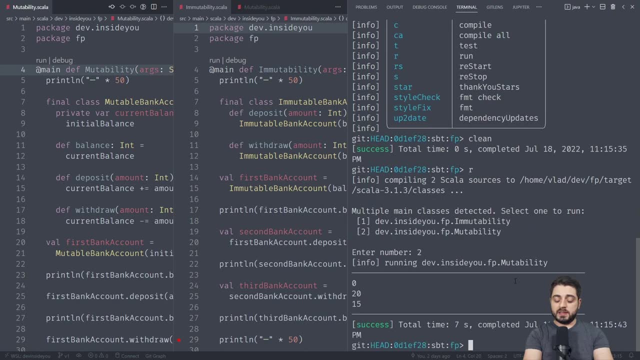 come on there, you go clean the project and we're going to run it. it's going to compile. it's just only two files, so the compilation is going to take just a couple of seconds. so we're going to run the mutable version and it presents 0.2015. so now we're going to run the immutable version. does the same. 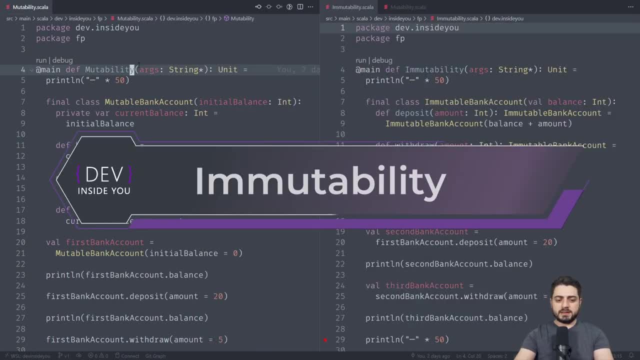 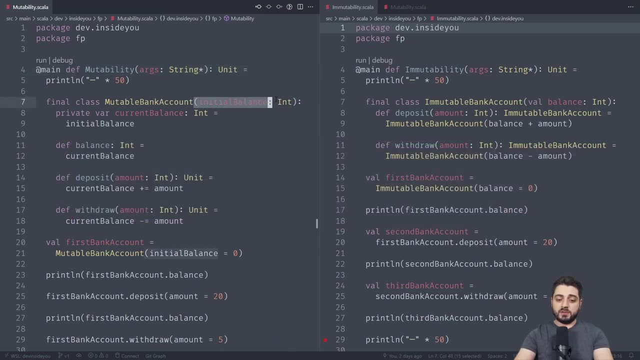 thing. okay, so let's go through, uh, through the scope. so this is like the main method: uh, we're printing hyphens. then we have a class, uh called mutable bank account. uh, this is how constructors are done in Scala. so this field, initial balance, is of type integer. it is not going to be accessible from the. 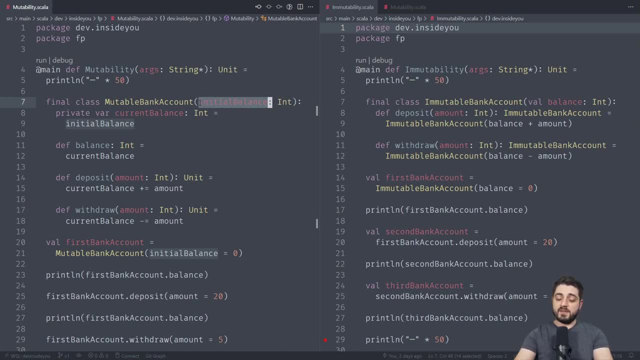 outside, so in Scala, this is technically a private val. valves are constants, okay. so, uh, everything that is here is two things. one is, this is the constructor body and also this is all the members of the class, which is: you know functions, you know methods. uh, right, and other fields okay. 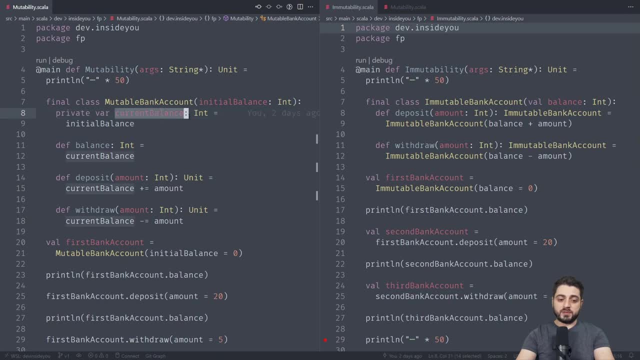 we have a private variable right, which means a mutable reference to an integer and in the beginning, in the constructor is going to be um instantia initialized with the initial balance. okay, uh, this is pretty much a getter for the balance right. so this is just a definition, this 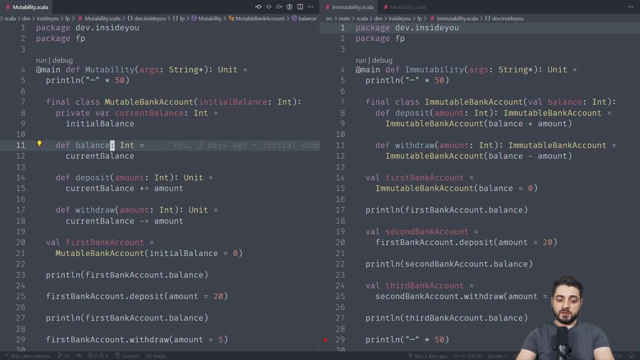 is a method without any parameter list and its default value is going to be a current balance. but this is a method, right, and because this variable is immutable, whenever this change- you know, changes the- the getter will give another value. we have deposit and we have withdraw. uh, the. 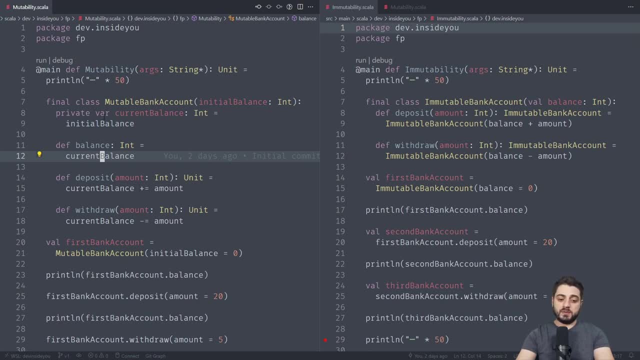 much. you know. we give it in the amount. we're either adding it- the amount to the existing current balance, or we're withdrawing, we we're removing it. we're not worried about, uh, arrow handling or type safety or anything like this here. okay, over here we're creating our first. 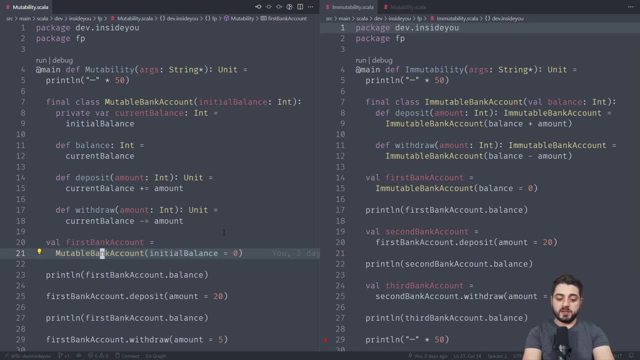 mutable bank account by giving it the initial balance of zero and we are printing it out, which is why we saw the zero. then we're depositing 20, let's say, dollars, and then we're printing it out again, printing out the balance right by using this getter right because it has access to the 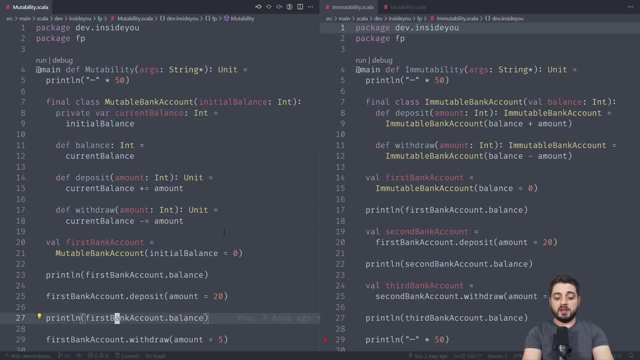 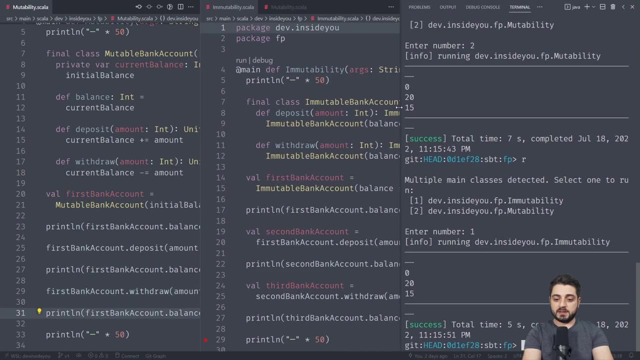 immutable variable. every time the printout is going to be different. so printing it out and then we're withdrawing five dollars, and so we're left with 15, right, so over here we had 0, 20, 15.. let's have a little bit more space, like this. okay, the immutable version works pretty much the same way. 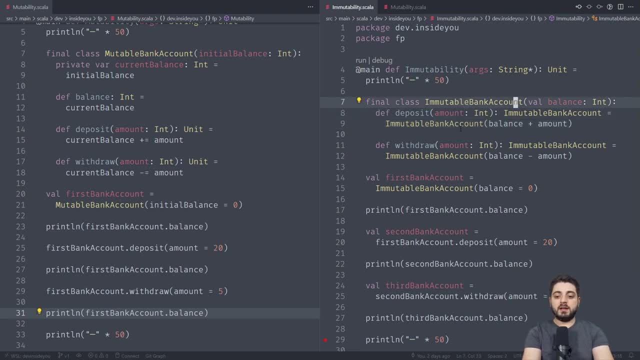 like most things look exactly the same. it's a final class. now. this is not a private val. this is a val which means it is accessible from the outside, so we can do immutable account dot balance over here. and let's say we want to do this because we only wanted the getter to be visible, but not the 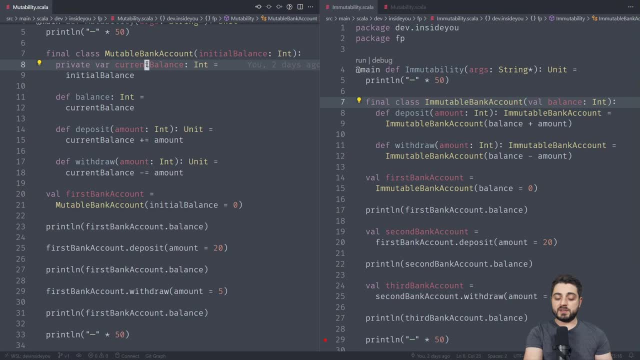 setter right. only the methods inside of this class will be able to modify this current balance. but on the other side, you're still going to be able to see it. immutability doesn't have any issues with it, right? so we can have this balance because it will never change, right? so over here we're. 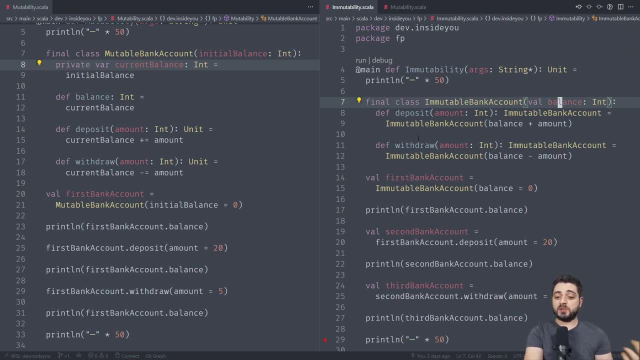 instantiating the immutable bank account with a zero, and it will be forever zero. so how do we deposit or withdraw things? well, instead of returning a unit, which is something like void and We are going to every time we're going to change something, we're actually going to. 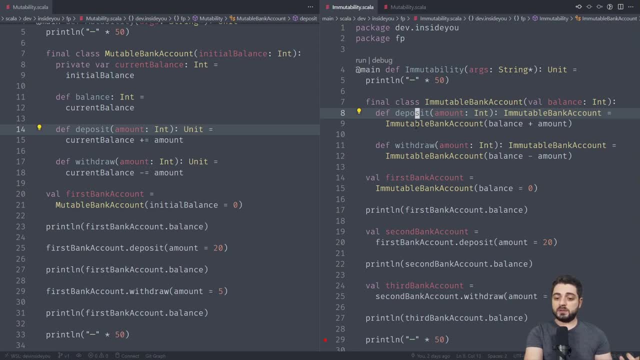 create a new bank account. So over here, as you can see, deposit creates a new bank account, takes the balance of this account, adds the amount that we're passing in. withdraw, has a minus over here, right, And so anytime we deposit, we're actually creating a completely different bank account. 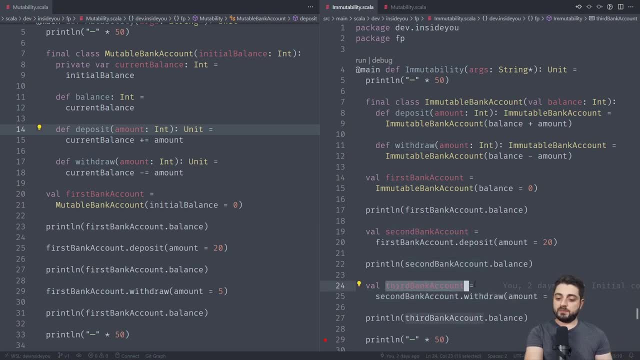 okay, Over here, withdraw completely different bank account. So we kind of have like versions of the bank accounts if we stick around using those vowels. Okay, I think a debug point sneaked in somehow. Now this point is already very important because immutability already seems more sensible. 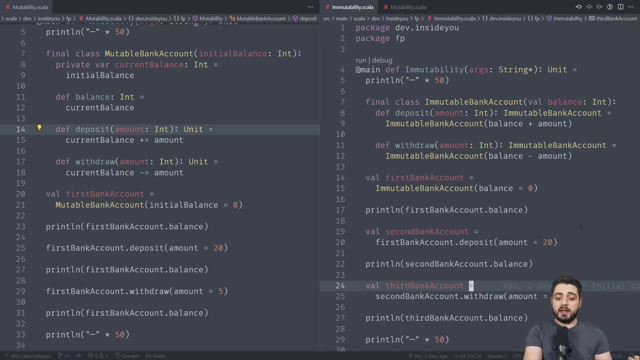 right. You kind of have this intuition that immutability is somehow better. You know, there's no mutable state, so it's probably good. If there's no mutable state, then there also cannot be any shared mutable state. So this is how concurrency is solved. 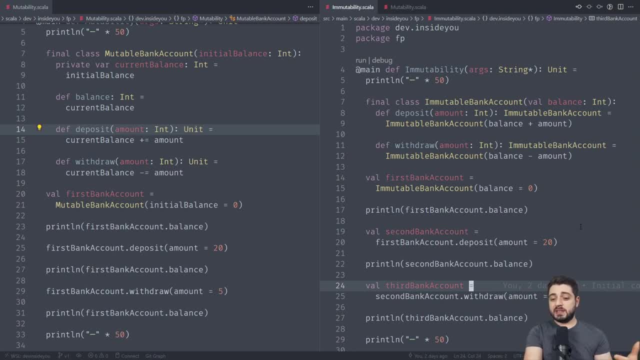 You know, usually around this stage people also talk about referential transparency, but this sounds like a very fancy word. So Don't worry about any of that. We're going to discover all of these things step by step, and there will be no stone left unturned. 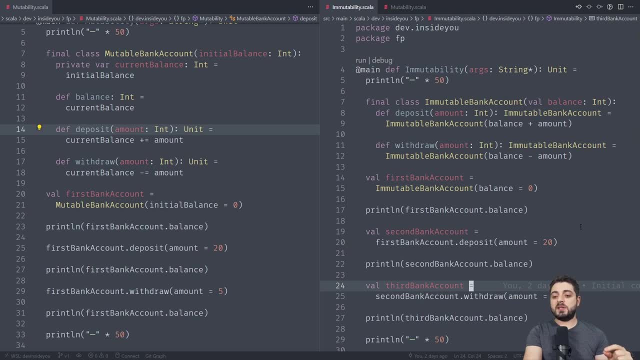 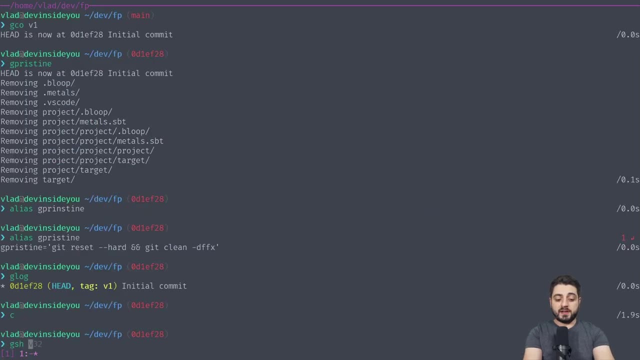 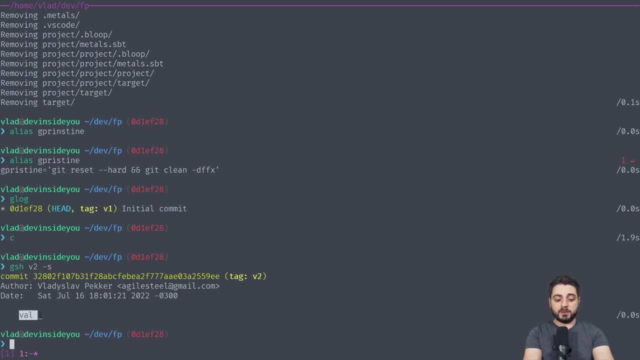 right. So you will know exactly what referential transparency is and you will know exactly why immutability makes more sense. Not every commit is going to be very big, okay, So let me first see. so when I do this short thing, I'm only seeing the description, okay. 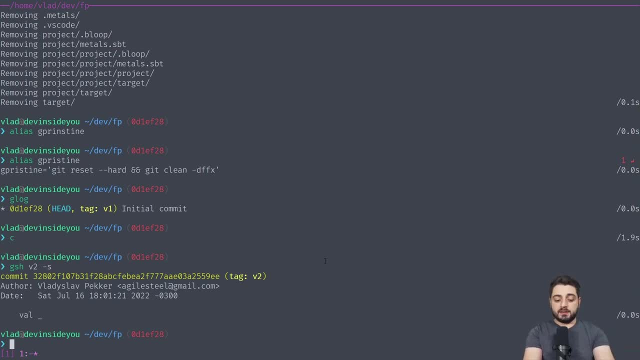 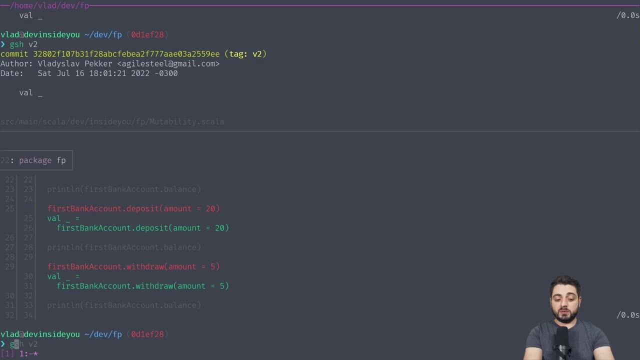 It's just to remind myself of what it is going to be about, And Now we're actually going to see what happened there, okay? So, as you can see, this is the only thing that happened there, and I'm actually going to check it out, okay. 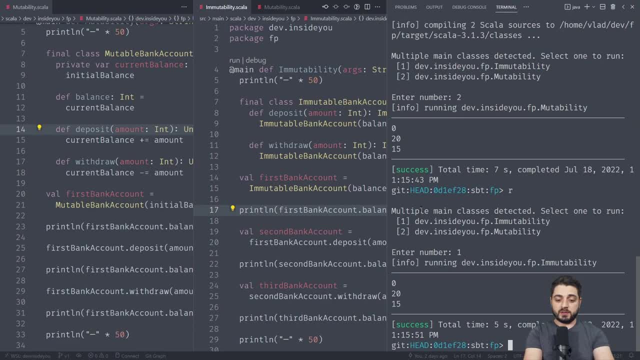 In fact, I think what I should do is I should do this over here, okay, So I'm going to open the console and I believe I can do something like over here split terminal. I'm going to use the SH, okay. 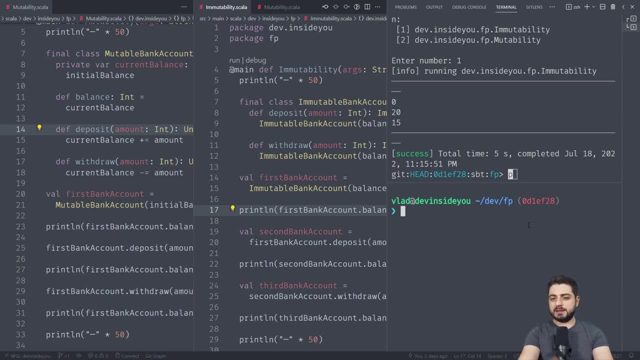 And I know that I'm covering like some parts of this, but it's not that much of an importance of what is written Like in the bottom right corner. So what I'm going to do is I'm going to check out V2.. 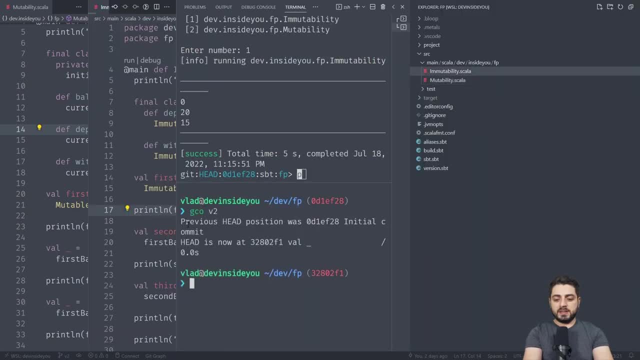 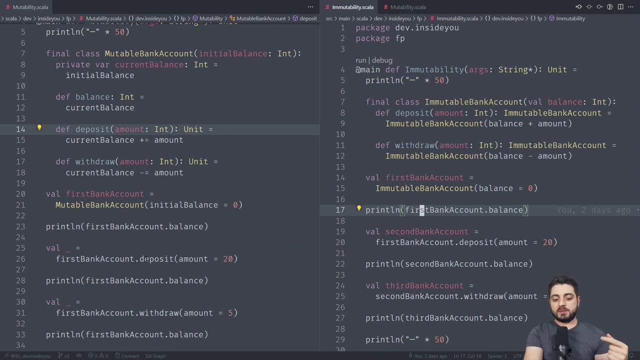 So, as you can see, this is the only thing that changed, and I simply made this change because I'm kind of like walking you through the whole thing Just to point out that there's always something returned, because we're in Scala and Scala is an expression-oriented language. 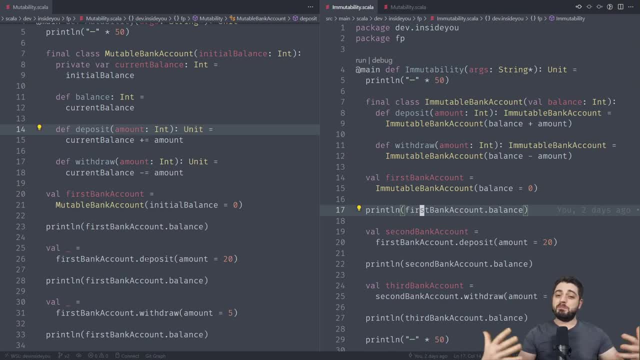 So everything is an expression, which means everything has a value, and because it's a mix of functional programming and object-oriented worlds, every value is also an object. There are some optimizations when it comes to primitive types, but None of them matter today. 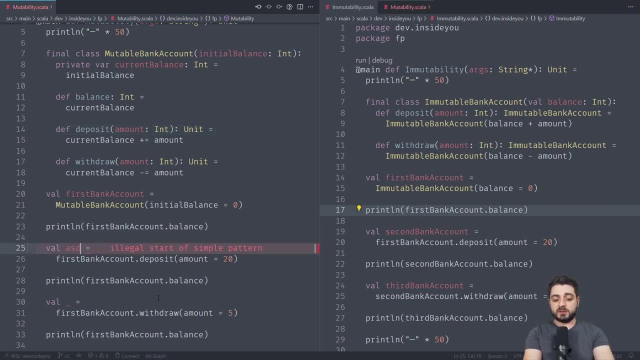 This is just a fancy syntax for when we are not interested in specifying the name for our variable because we're not going to reference it at all. right, But it will become important much, much later in the video. why I'm pointing it out like this. 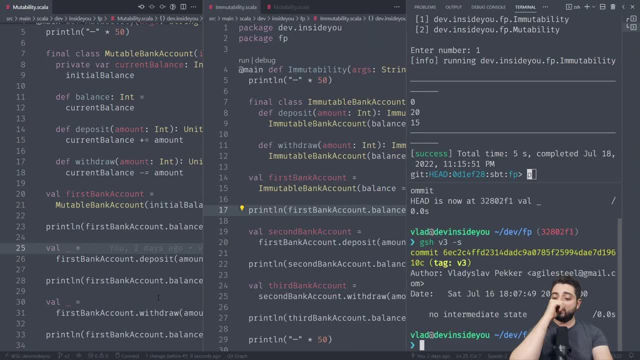 Let's not dwell on this, Let's just move on. So version 3 is no intermediate state. okay, So over here we have an immutable bank account, but we kind of go through like intermediate states. First, we create, like the second bank account. 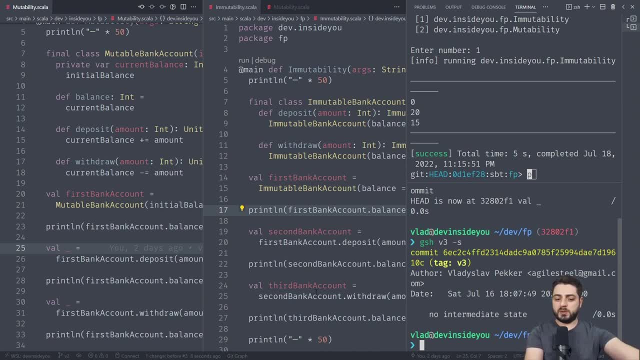 Then we create the third bank account. But at the end of the day, we just wanted to create the third bank account And we kind of do like the same thing over here. We're not creating intermediate states, but we're going through intermediate steps. okay. 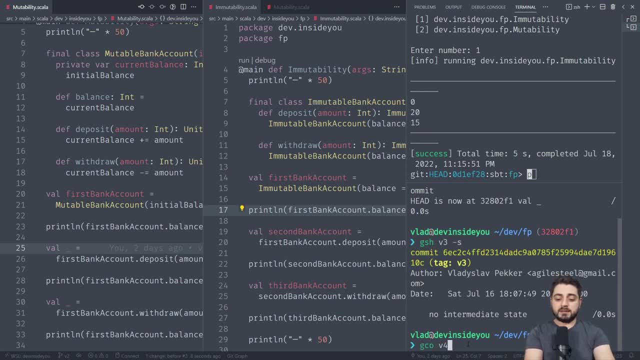 And so all that this thing is showing is that you could, you know, because one of the things about functional programming is that usually people say, oh, you know, it's like less code, it's like you know, everything is shorter, it's nicer. this is not what this is about. 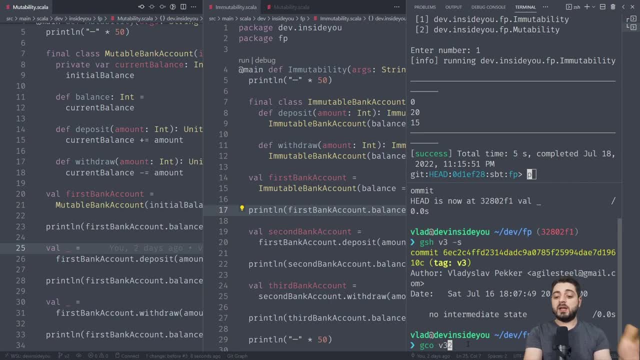 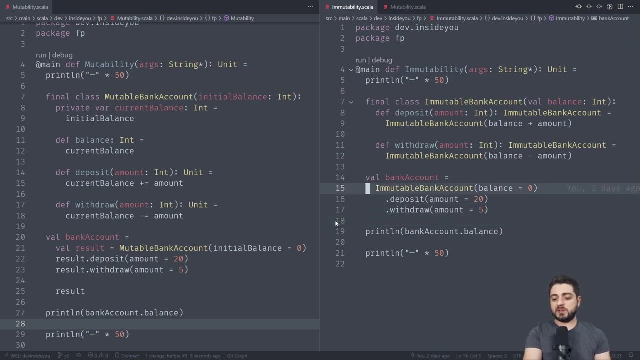 I want to show you that you can do this both with the immutable version and the immutable version as well. okay, Basically, over here, we're not using this, We're not using any intermediate states, So the immutable version kind of makes sense, because this is also called fluent interfaces, right? 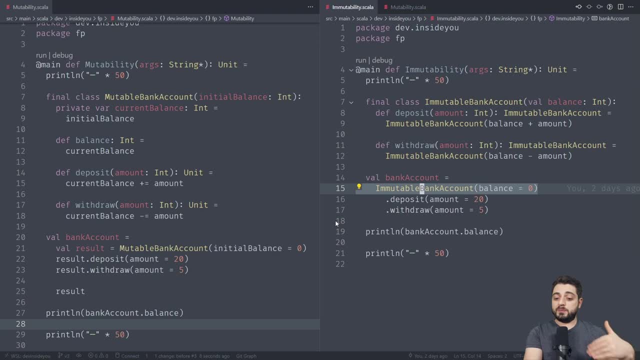 Because this line gives an immutable bank account. On that immutable bank account you can call deposit right. But what does deposit return? Well, it returns an immutable bank account. So on that immutable bank account, you can call another method called withdraw. 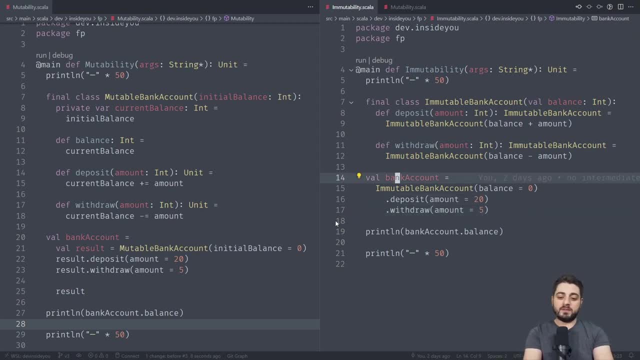 And at the end of the day you're getting your third bank account but kind of have only one val and therefore we- only you know. it kind of feels like we only had only one bank account, okay. Also, usually it's one of the beginners concerned about functional programming that there is like some copying taking place. 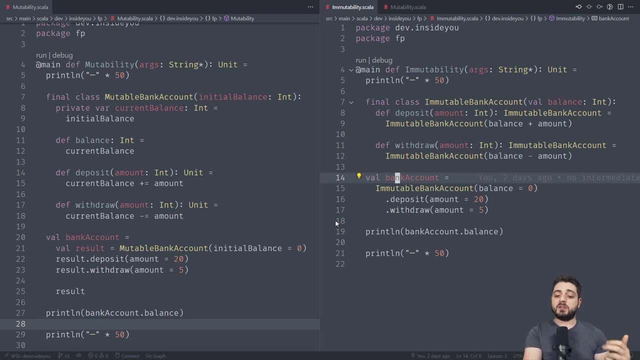 But you know, most of these problems in functional programming are actually solved by a thing called persistent data structures, But I'm going to talk about them today. We're also going to talk about recursion, which is a common thing that functional programming tutorials talk about. 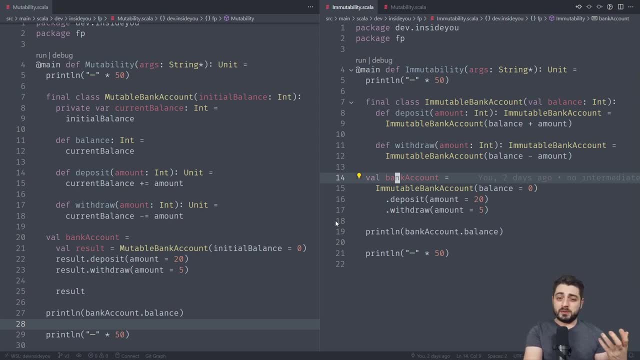 Because, ultimately, functional programming is not all about recursion. And also, especially like in real-world application, even if your entire application is written in purely functional, you might not have even a single recursive method, because all of these things are like abstracted away. 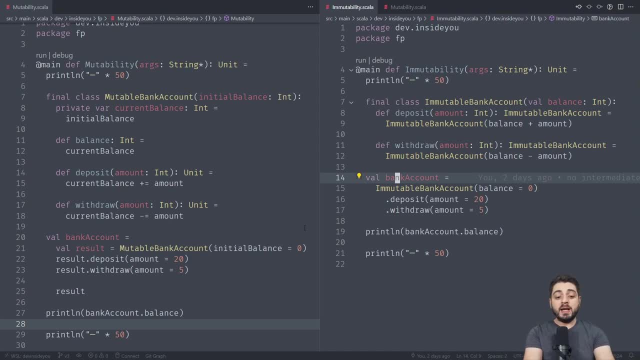 They're hidden behind. you know utility methods. So the immutable one kind of works the same way right. So in Scala we can have, you know, vals inside of vals. We can have even classes inside of vals. Scala is a very regular language. 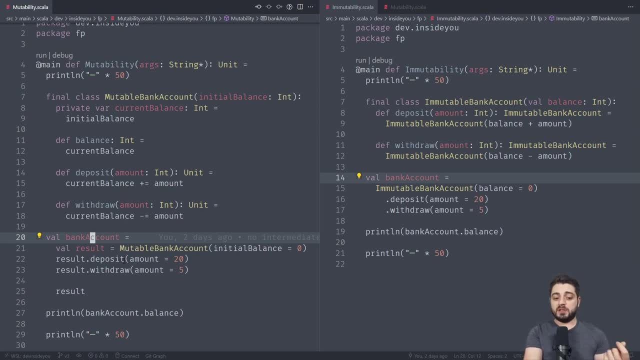 There aren't that many exceptions in terms of like syntax. okay, So we're creating a val bank account, but there's a teeny tiny val inside of it called recursion. Usually it's called result or some sort of like accumulation. 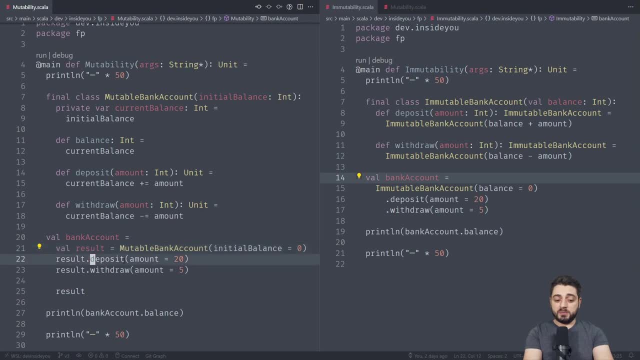 So this is essentially a bank account. Then we deposit, We withdraw And then at the end of the day we return it, okay. So this is also one of those things that usually, when you start out with Scala, people tell you. you know, don't use var. 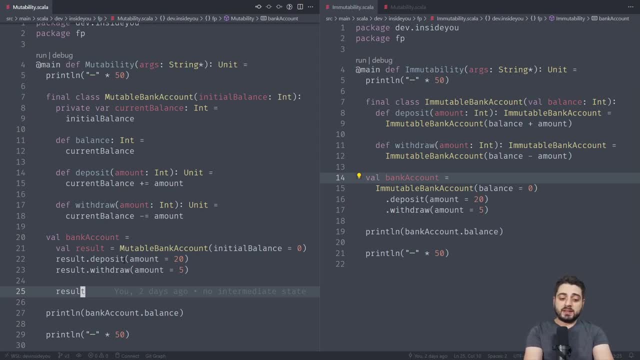 Var is like mutable stuff, But it turns out that mutable stuff has actually nothing to do with the vars because, even though this is a val right, the mutable state is inside of this thing, Like typical example would be an array. 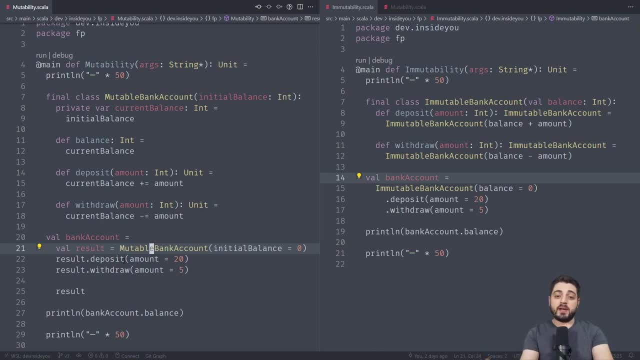 You can have. you know, val x equals 0.. You know array of 1,, 2, 3.. The array is mutable, even though the reference will always point to this array. It's just that the question is: what is this array? 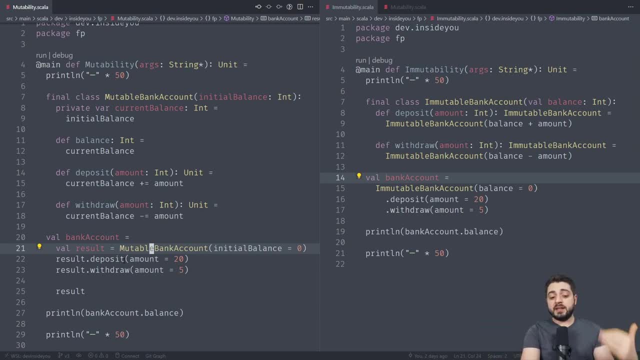 The array can mutate, It can change in place. Again, the point of this whole exercise so far was to show you that it's not all about, like you know, the fact that the mutable code is, like, shorter and more pleasant to read. 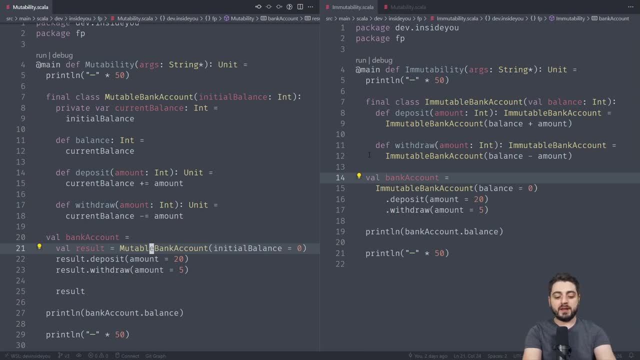 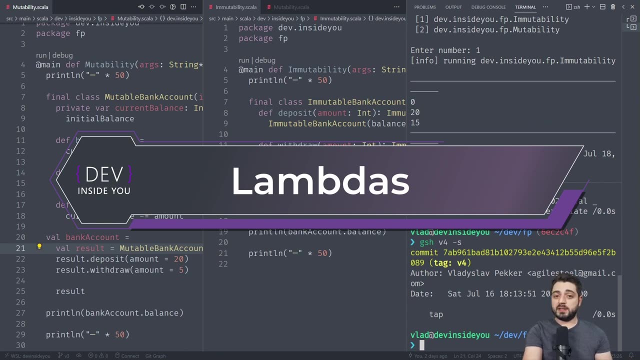 You know it is a point, but it's not like it's not what this is about. okay, Let's go and see what's up with the next one. So version 4 is tapped. So one of the things that you learn about is lambdas. 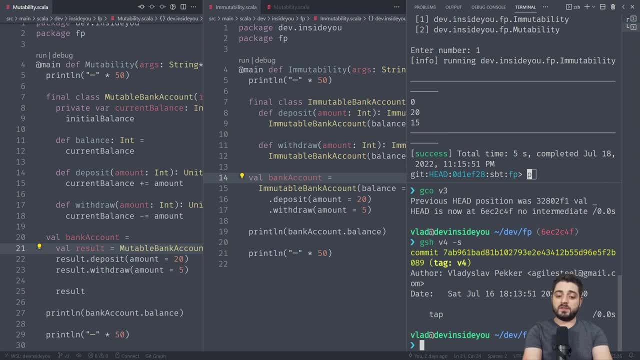 Lambdas are just a syntax for function literals, okay. So the same way as you can have a literal for a number like 1,, 2,, 3, you can have a literal for a function. Now in Scala, this literal is just a syntactic sugar for an anonymous class that is going to be instantiated, right? 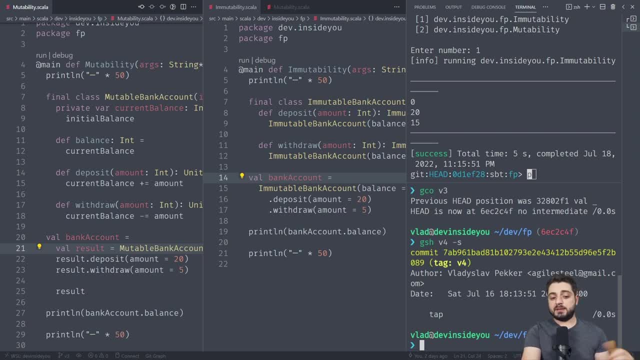 So it's going to turn into an object at runtime And there's a lot of like syntactic sugar around it. So what I want to show you is that you can even get rid of this val result, so that syntactically, these two things- even though one is mutable and the other one is immutable- can get even closer okay. 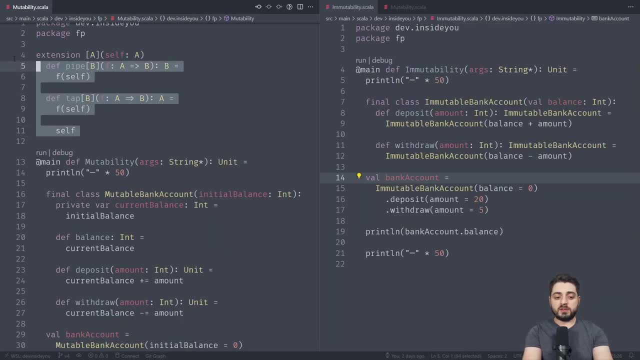 So I'm going to check it out. So this is v4.. These two functions are present in the Scala standard library. In fact, the next commit throws them out and uses an import. okay, But let me explain to you the syntax first. 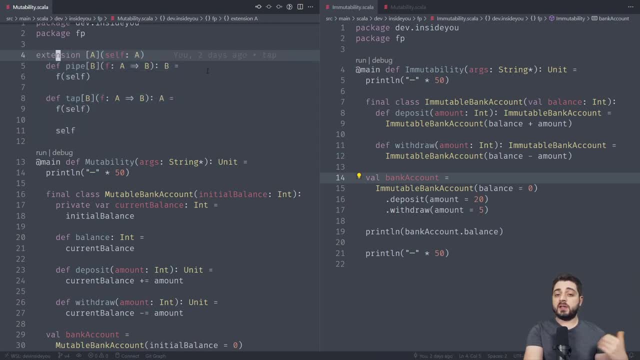 First of all, like this is a feature in Scala 3.. It is also possible to do this in Scala 2. It's just that the syntax would be slightly different, And this is an extension method. It's also present in other languages, like C Sharp, for example. 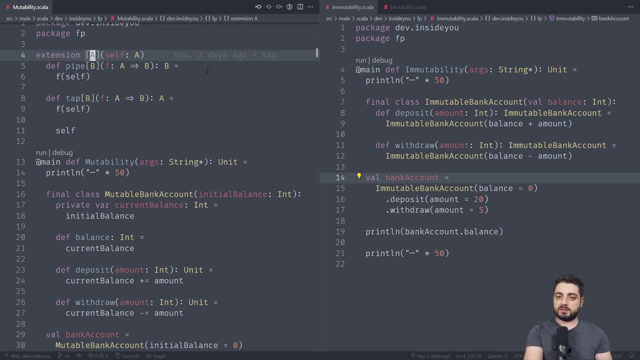 And this extension method extends all kinds of types. We're giving this type a name, a, which means you can stick any type into it, But in this scope it is going to be known as a right, And so you're going to be able to call a function called pipe or a function called tap right- this one on that thing that you're calling right. 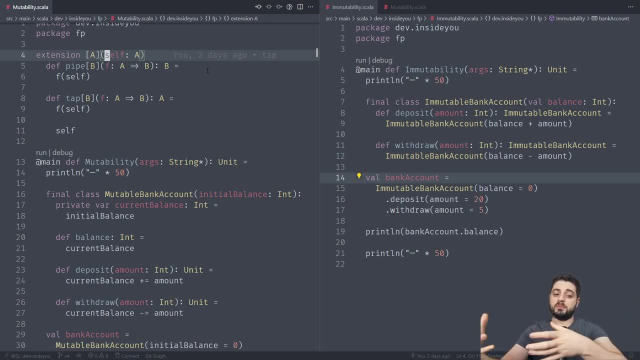 So you're going to be. you know, imagine you have something You can do: a dot pipe or dot tap. okay, This is what the syntax allows you to do. Pipe is a funny thing, Essentially. maybe I should give you an example. 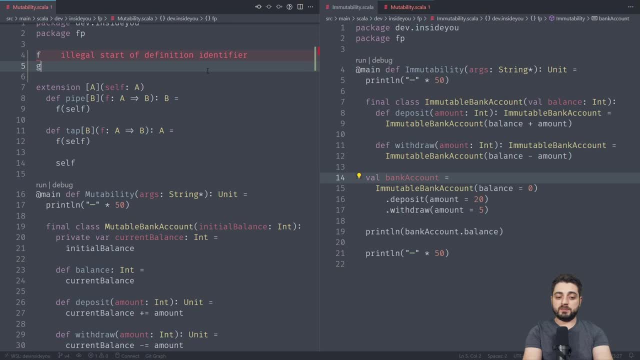 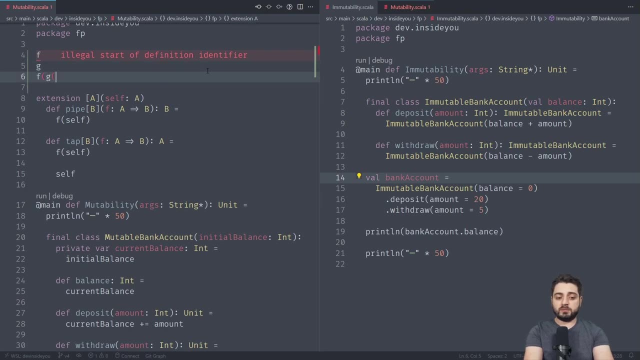 So imagine that you have like two functions, f and g. okay, And then you know, g takes an a and f takes whatever, you know, whatever comes out of g, And so this is how you would. you know how you would write this code, right. 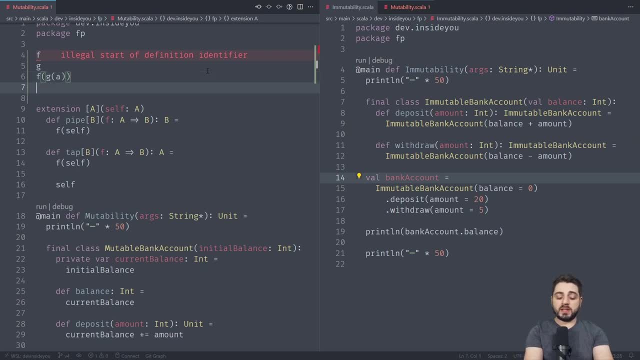 So you give a to g and then, whatever comes out, you give it to f. This code will allow you to do something like g of a right: Take the result, pipe the result into f, okay. Or you can even go, take the a, pipe it into g and then pipe it into f, okay. 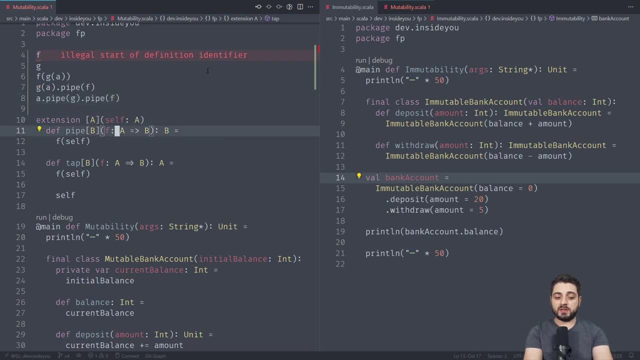 So this is what this thing would allow you to do, okay. So, as you can see, it is a high-order function. High-order functions either take other functions as parameters, or they produce functions as the result, or both, And at the end it returns a, b. okay. 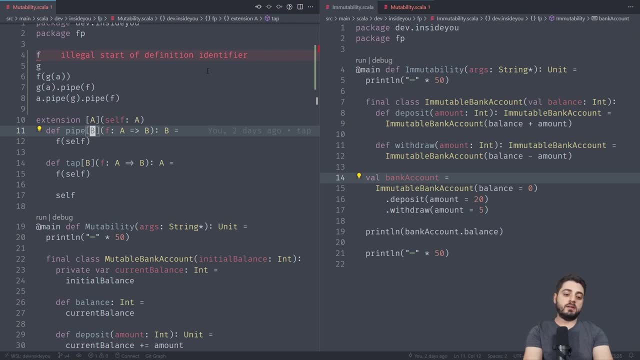 So b is over here. right, A little bit of generics, okay. So somehow we go from a to b just by calling the function. okay, The implementation is trivial. Now, tap is actually what we're interested in. so far, right. 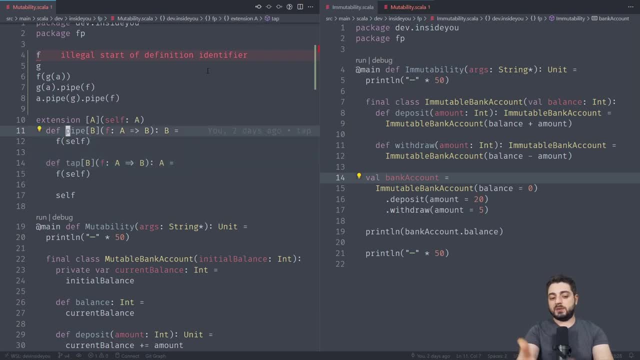 Because I brought in pipe? because, simply because it's you know, usually they are presented together, But we're going to use pipe only a little bit later in the video. okay, Tap is actually very interesting because, even though it looks exactly the same, at the end of the day it throws out the result of b right. 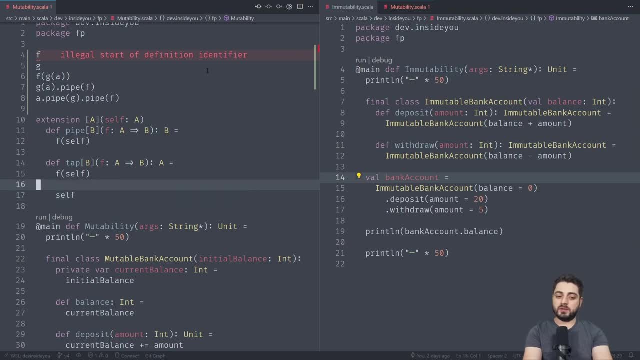 And it just gives you that thing that you called it on right. So, for example, over here, you know, if this was like a tap g, Right, Whatever g returns which is over here would be thrown out and then a would be returned right. 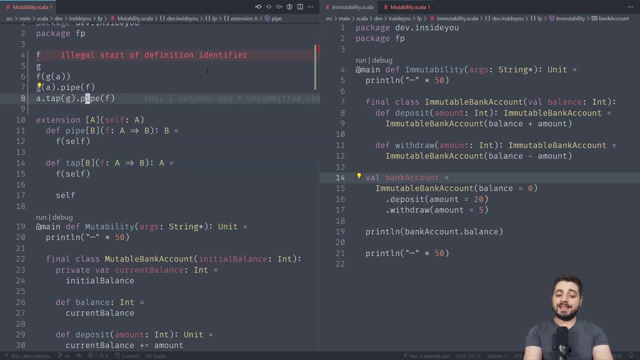 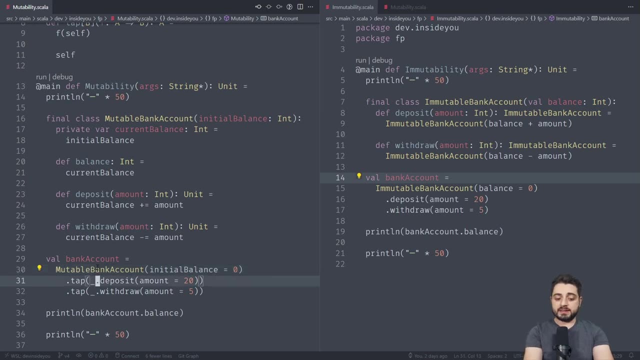 So this pipe will still be called on the a, And this is done exactly for mutable code. So if you look at the bottom, we're creating the multiple bank account and we tap into it. This is a fancy syntax for okay bank account comes in right. 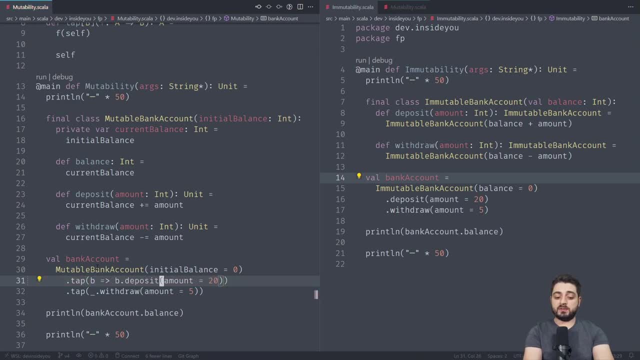 And now we're taking the bank account and we call deposit on it right Now. the result of deposit is unit: right, But look at this code. We're throwing out this unit. We don't care about this unit. We return that thing that we call it on right. 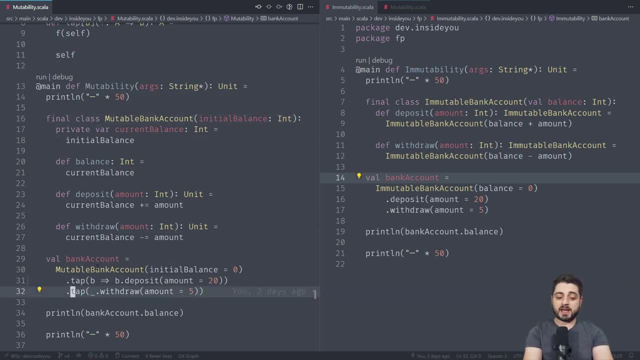 Which is this mutable bank account. Okay, So over here, this tap is still called on the bank account. Okay, So this whole thing, at the end of the day, does exactly exactly what it was doing before, but there is no need for this now. 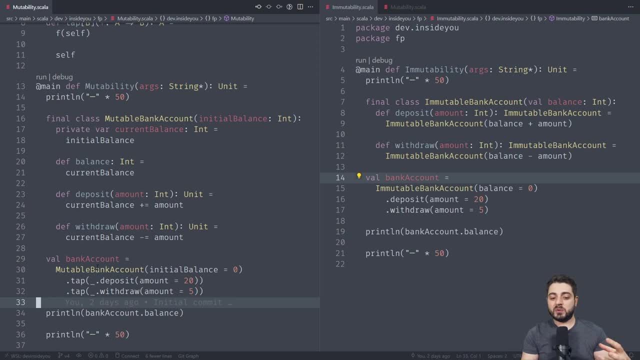 So this argument about immutable code, like you know, it's less code, It's not. it's not that valid. Like most of the times, yeah, you can. you can write very concise code. However, again, this is not what this is really about. 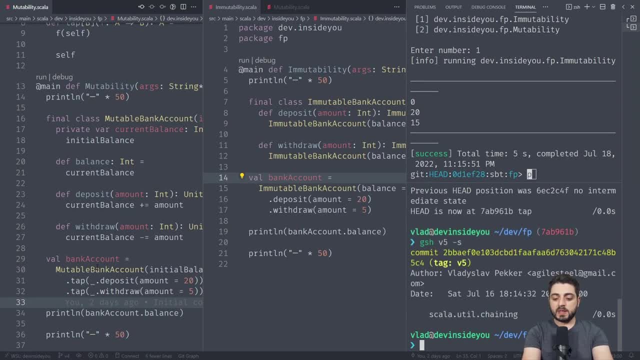 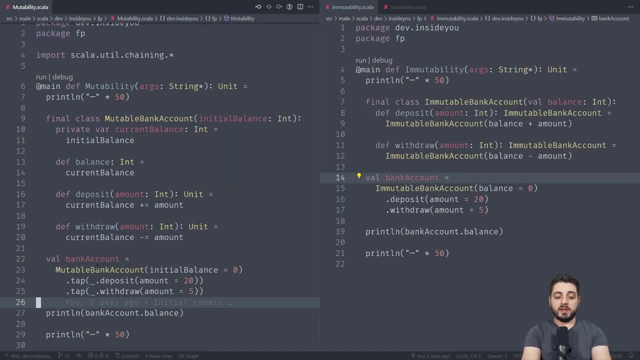 Okay, So let's say that the next commit, which is V5, is going to throw it out and just do an import to ScholarUtilChaining, because these two methods are so popular, so common that they are, you know, part of the standard library. 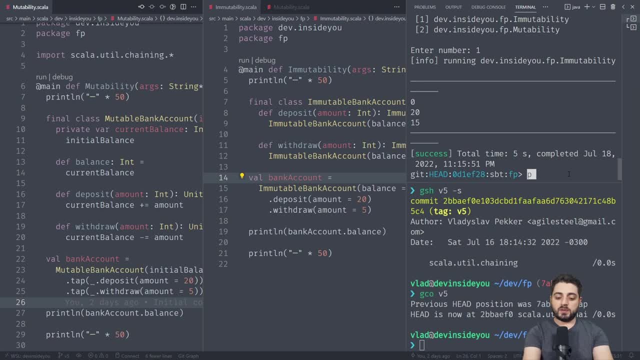 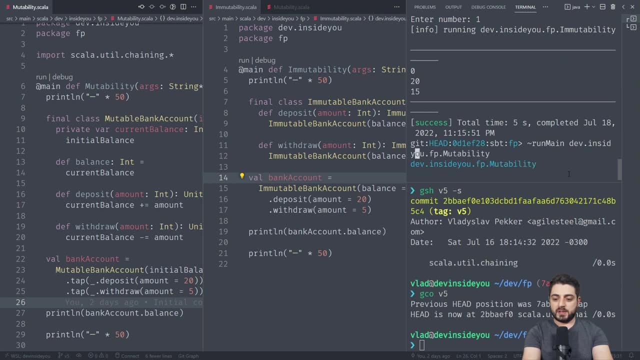 Okay, And, by the way, from time to time I should actually run the code. So what we can do over here is we can do, you know, run main and then dev inside you and let's run the mutable version. As you can see, the result is now only only 15.. 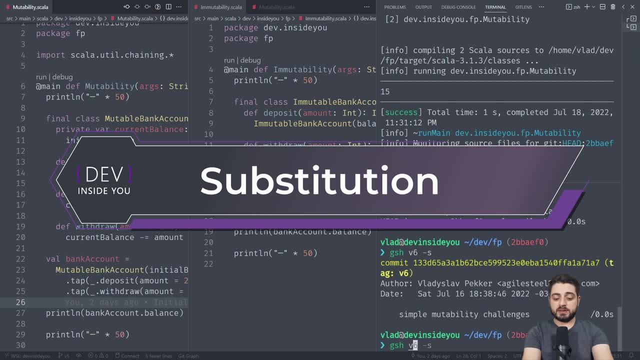 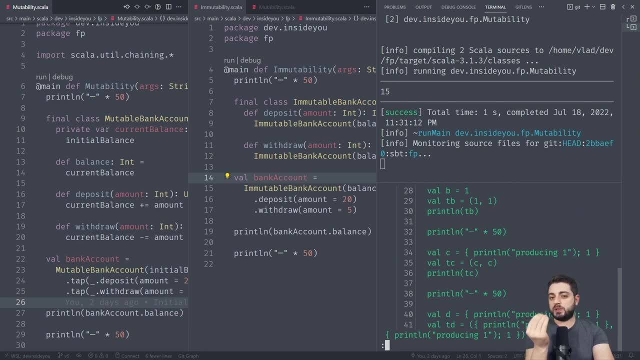 This is the next one. Simple mutability challenges, Interesting. I actually want to see what I, what I did there before I present it to you, So there will be two commits. in this entire thing There are, like the very crucial key points. 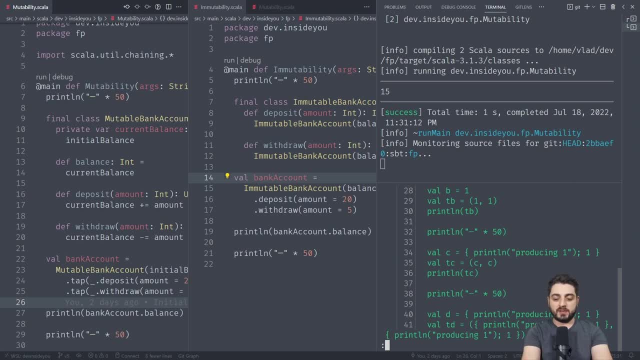 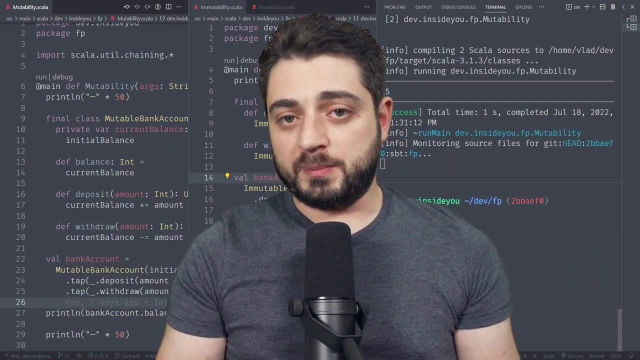 You really need to make sure that you understand them, because otherwise everything else is going to be very hard to understand. Let me talk a little bit before I present this to you. So the next commit defines functional programming. It presents a model for understanding how procedures, which are methods or functions, are applied. 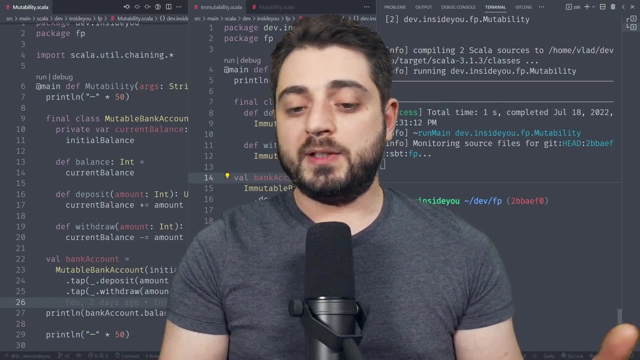 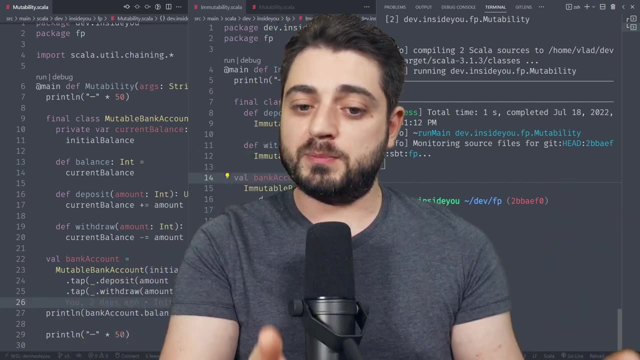 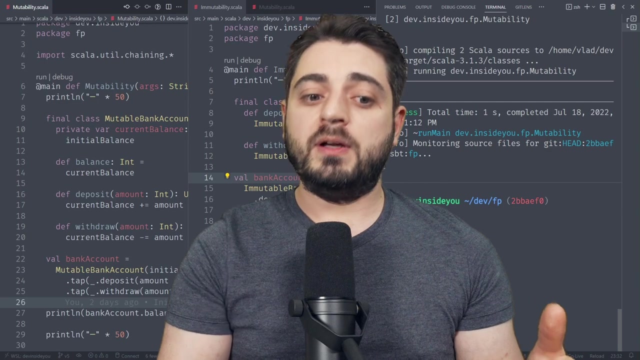 Okay How these functions are applied to arguments. This model is called the substitution model for applying procedures right For procedure application. So the substitution model for procedure application. Now, this model is not how the compiler or the interpreter interprets or compiles your programs. 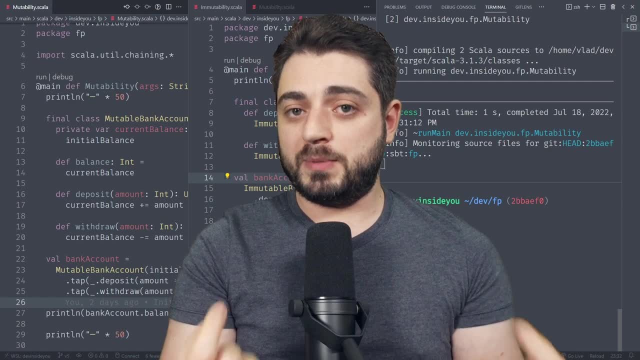 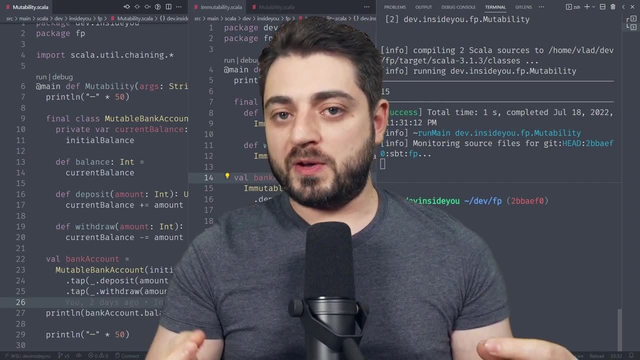 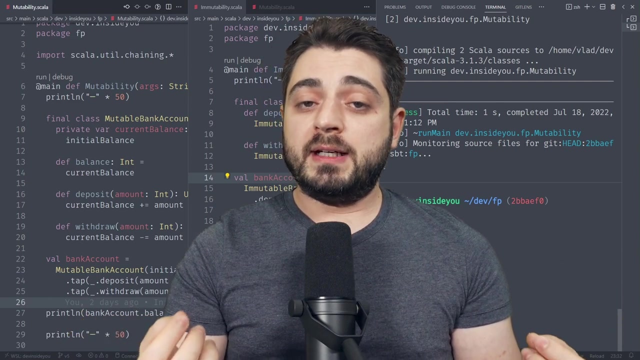 This is a model for you to think about your programs and to have certain guarantees. This model should be very attractive to you because this is the simplest model of how you can- how to think about programs or pretty much any other scientific or mathematical things. In fact, this model is being, you know, was presented to you in high school right. 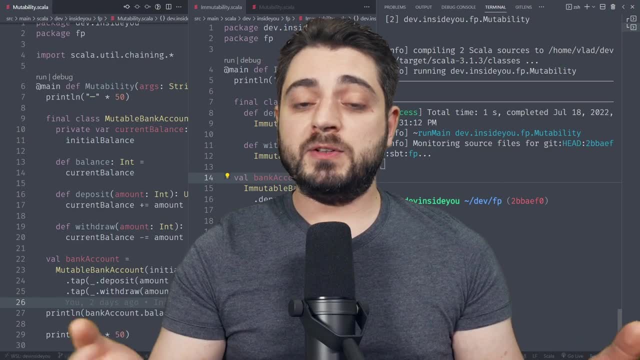 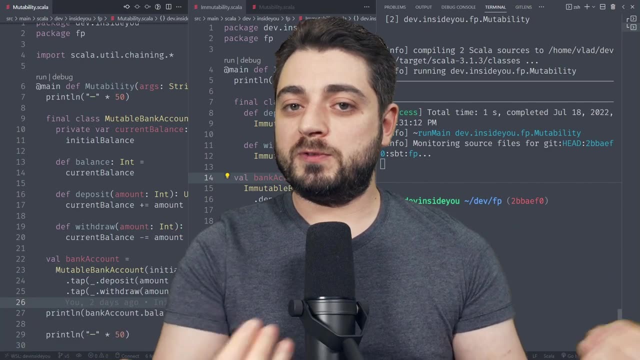 So whenever you know your teacher, I always use this example. Whenever your teacher writes on the whiteboard, you know X equals five. then, no matter what happens, no matter at what time you refer to X, everything else on the board will still see X as five. 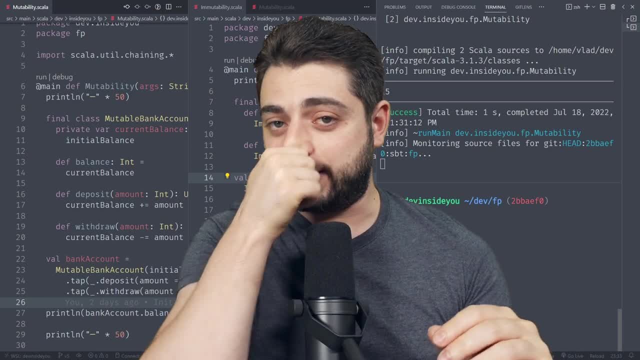 X will never change, right. So again, like immutability kind of like, kind of like sneaks in Right, But we're going to define it more precisely than just saying, oh okay, it's never going to change. 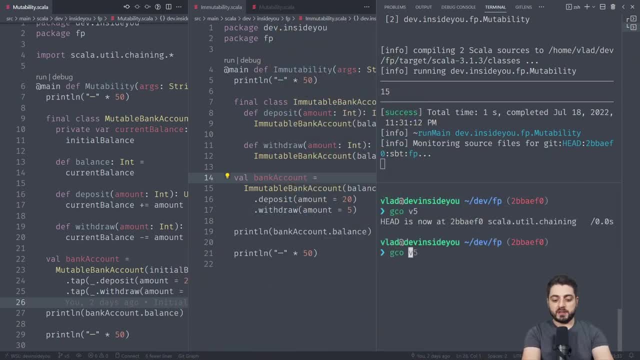 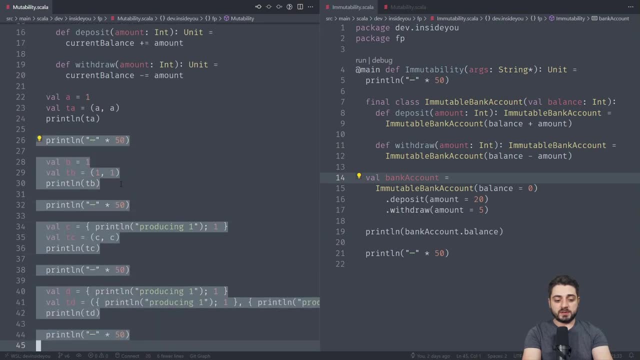 Let me check it out. Was it five or six? Okay, We're already at five, Okay, Six Okay. So this is how functional programming is defined. Imagine you have this code and I'm going to comment out. I'm going to comment out all of this. 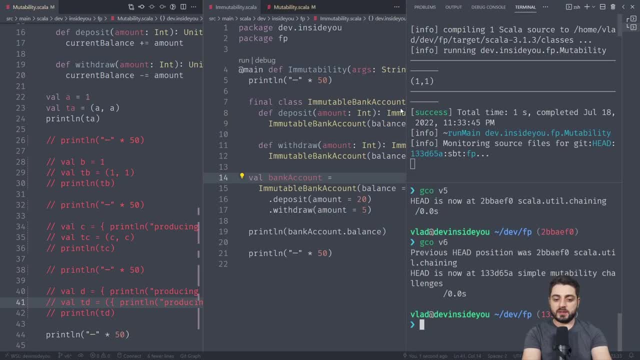 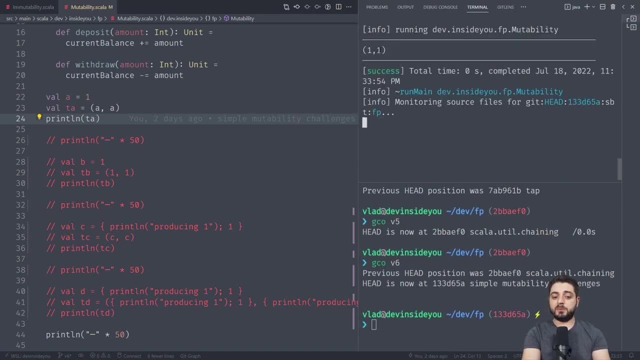 Okay, So this is how this program is running. In fact, we don't need the other version for now. This is all that this program is doing, right? It prints out one and one, which is a tuple. Okay, So now imagine for a second that you have a valve and you don't know what is on the right hand side of this valve. 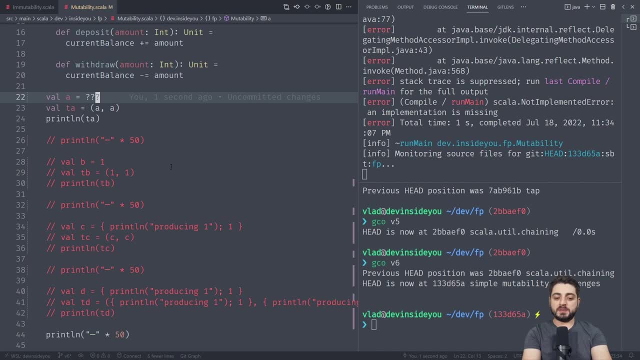 Okay, Like this. Okay, By the way, this code compiles because Scala allows not only alphanumeric variable names. So there is actually a definition called question mark, question mark, question mark, And all it does is it throws a non-implemented error. 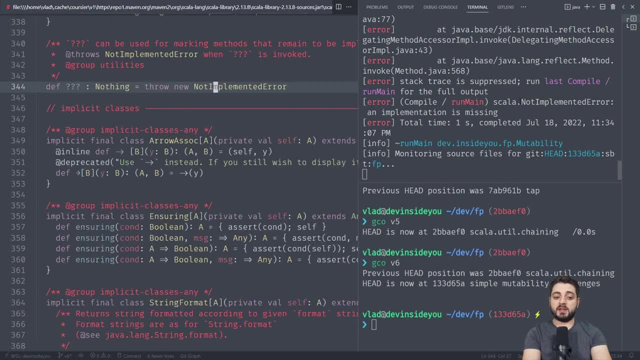 So we can jump in there and you're going to see that it just throws an unimplemented error. Okay, Like prototyping code. Imagine that you don't know what this is, which means that you don't know the type of this thing. 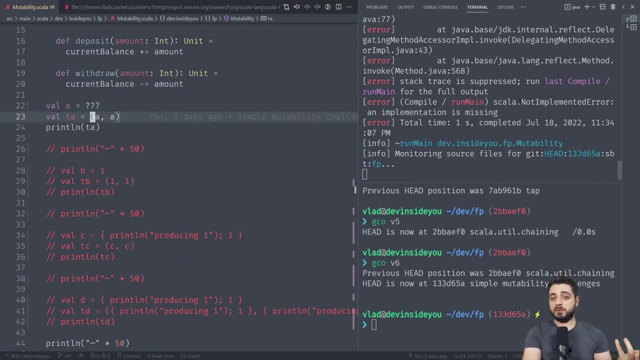 Okay, Now imagine that you wanted to create a tuple, which is a data structure without any special name. Right, You can retrieve these values by calling, you know, underscore one and underscore two. Okay Later, if you wanted to. Okay. 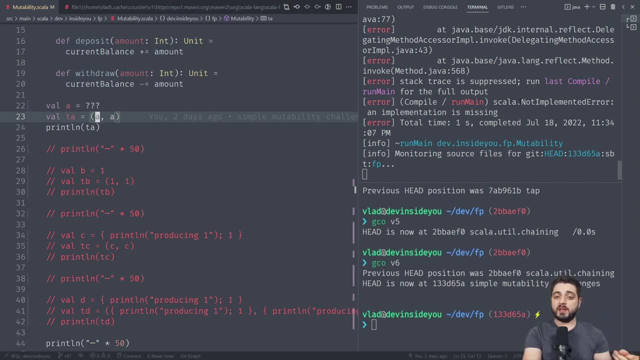 This is a tuple two, which is a heterogeneous collection. It can hold two things of potentially different types. In this case, it's the same type. Okay, You can see sticking it in there twice. Okay, So now you have a tuple of ACE, which is why I call it TA. 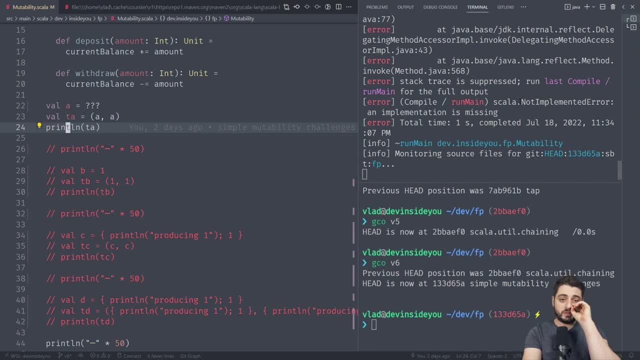 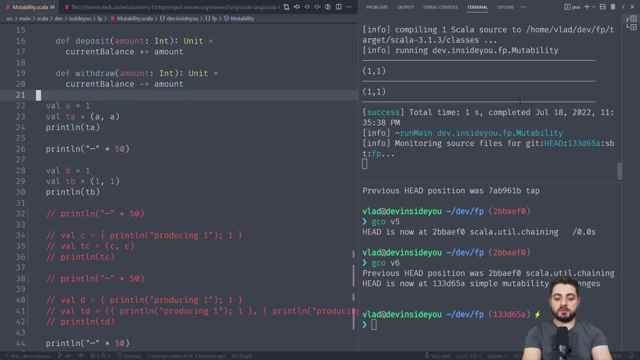 And so we are printing it out. And then you know, when there was one, you you actually saw the tuple. So here's the question: When do these two programs behave exactly the same? Now, what is the difference between these two programs? 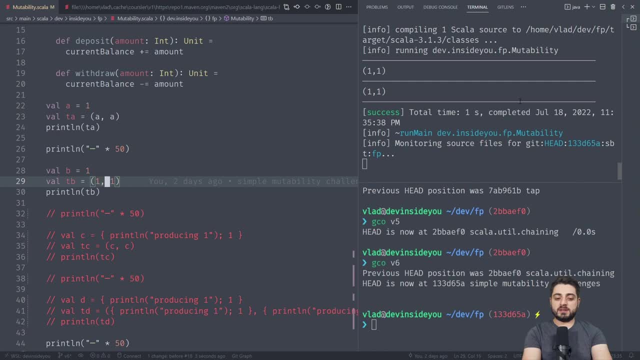 The only difference is that over here, when we're constructing the tuple, we are not referring to this expression, Okay, But instead we're referring to its value. Okay, Remember, the model is called the substitution model, So we're substituting the expression by its value. 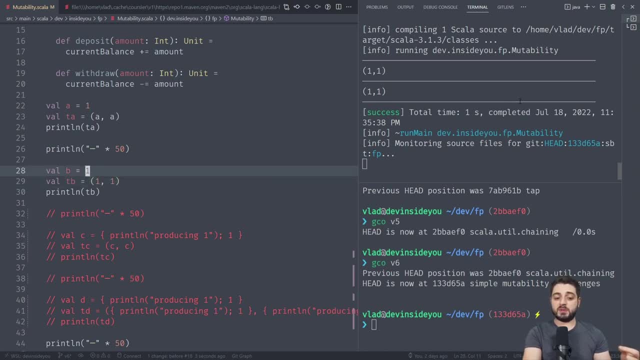 This is also called a referential transparency Right, So this expression is referentially transparent. if these programs behave the same, Okay, And for simple, simple values, like one Or an immutable bank account, These programs will always be the same. However, you need to know what you're dealing with. 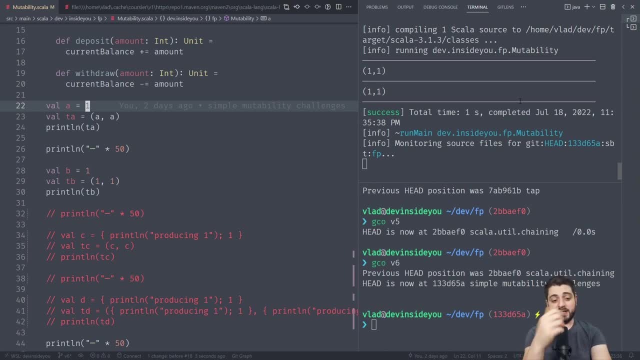 Right. In immutable program, you need to know what you're dealing with. Right, If this is an array, you don't know. If this is immutable bank account, you don't know. And here's an example, Right. So here we're introducing side effects. 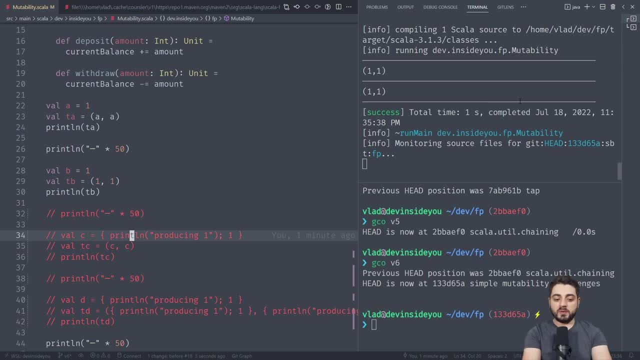 Effects that happen on the side. Okay, So all of these four programs are kind of the same, Right? So let's start with something: that a tuple is being created. In the first version of the program, the tuple is being created by referring to the expression. 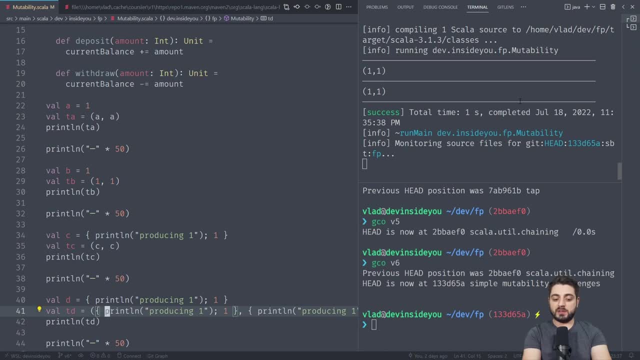 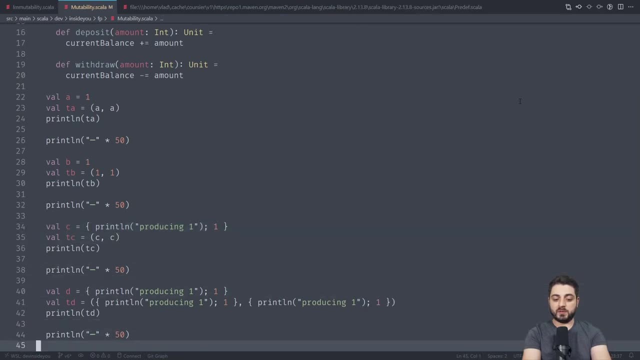 And in the second version is by literally substituting the expression with everything that is following the equal sign over here. Okay, I'm going to remove the console so that you see the whole thing. Okay, So, literally, like this, copied, Paste it once. 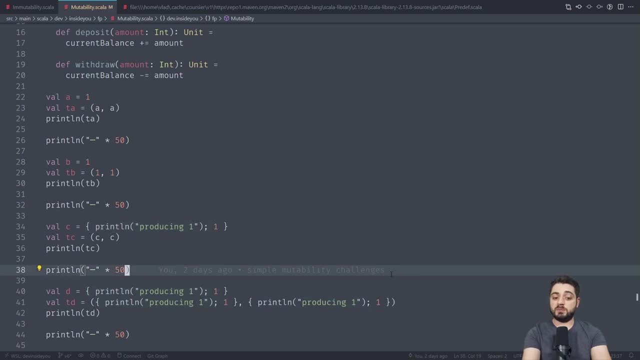 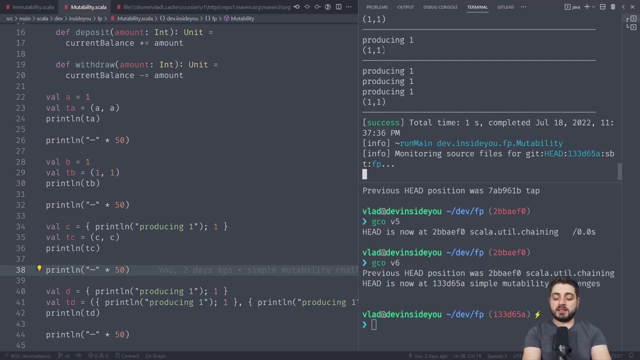 Paste it twice And a bit later we're going to have a version of this. was immutable bank account. Okay, But for now, for now, it's just print lines. So if we run this program now, you're going to see that it actually does not behave the same. 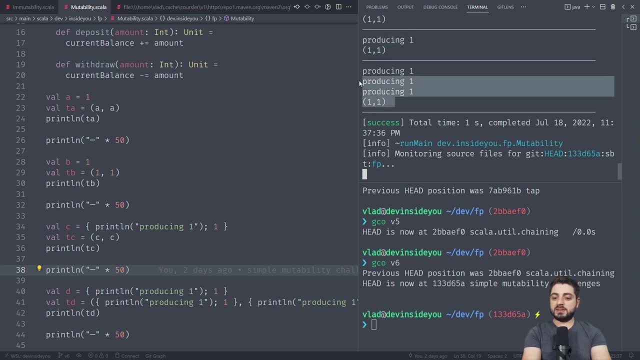 What does this mean? Right, So one program does this, The other program does this. This is different behavior. What does this mean? Well, it means two things. First of all, this expression, this one, well, technically, this one. 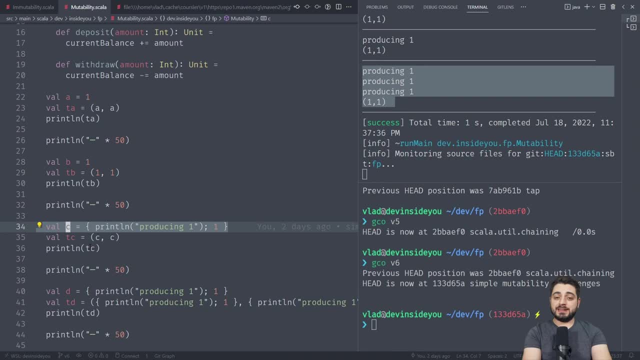 Right, But you know. you know what I mean, Right? This expression is not referentially transparent. So referential transparency is a property of an expression And it means that when an expression is referentially transparent, it means that the time when you refer to this expression doesn't matter. 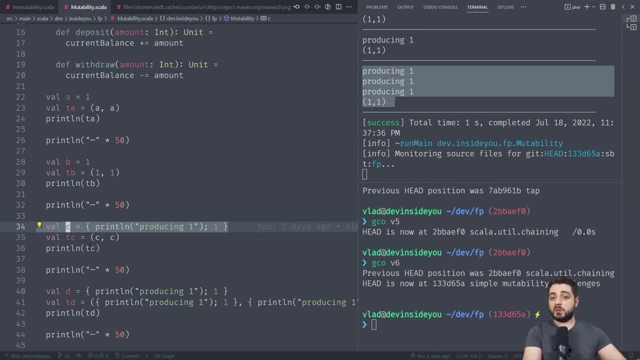 Right, Remember, like if X equals five, no matter if you call it, in 100 years, X is still going to be five. Remember, it's like this immutability thing. Right Now, the substitution model is a property of the entire application. 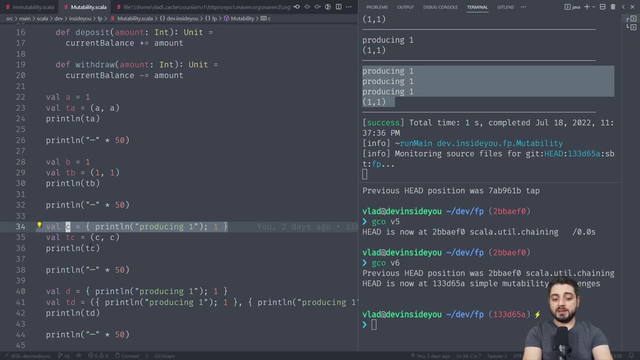 Right. So now, because we have, until we have this program, You know, Excluding these print lines. these print lines are just for you to, to help you understand, But these print lines were not around, Right, Like these two programs. 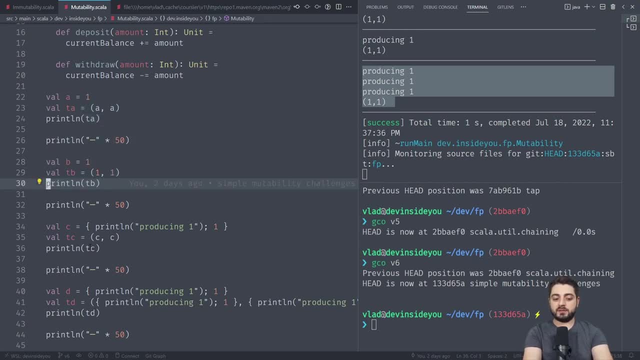 Right Again. like, forget about these print lines, like real quick. These two programs, this entire program was not breaking the substitution model for procedure application, Right. So it gave you certain guarantees. It allowed you to treat these expressions simply as aliases. 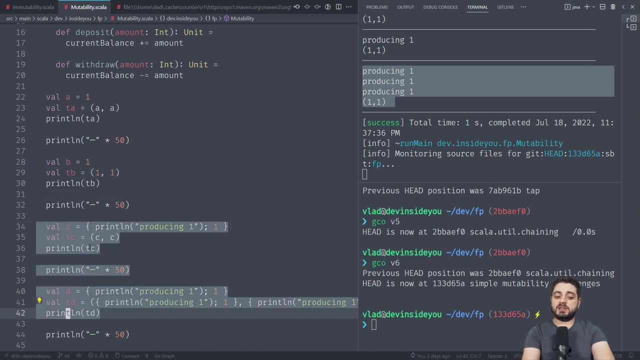 Right, But once we introduced this, we broke the substitution model for procedure application. And now, if this was a huge application, we would lose this ability to reason about our programs in terms of this very simple model, And this is a definition of functional programming. 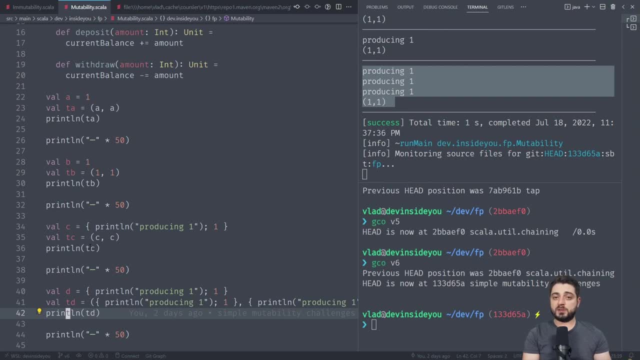 A programming is written in a functional style. It's a purely functional programming If you did not break the substitution model for procedure application, Okay, Which means every expression is referentially transparent, Which usually means every expression is immutable. There are some caveats. 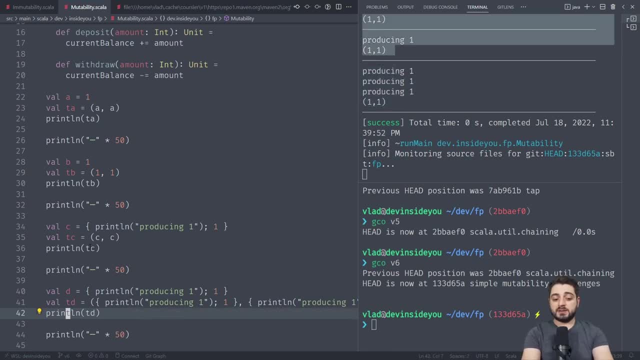 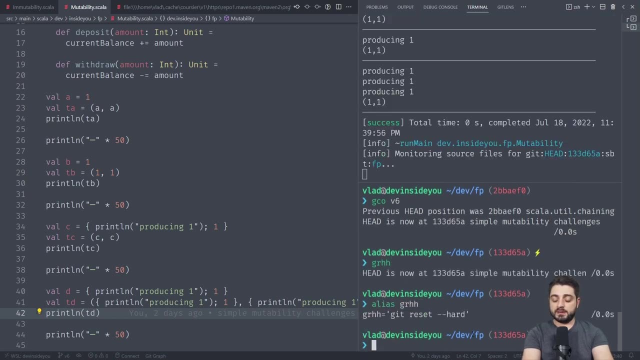 We'll get into that, Okay. So let's get into the next one, And the next one I'm sure is going to be, by the way, GRHH is git reset hard Right, Which means that you know, let's throw out all the changes. 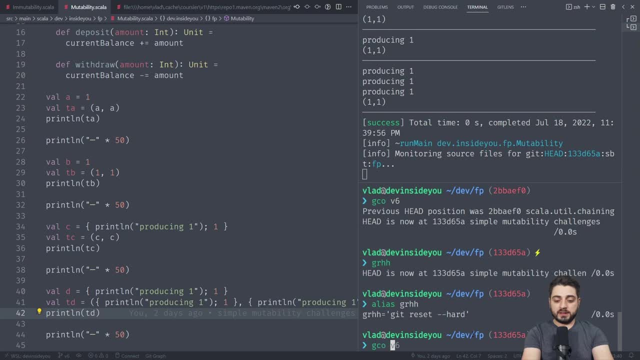 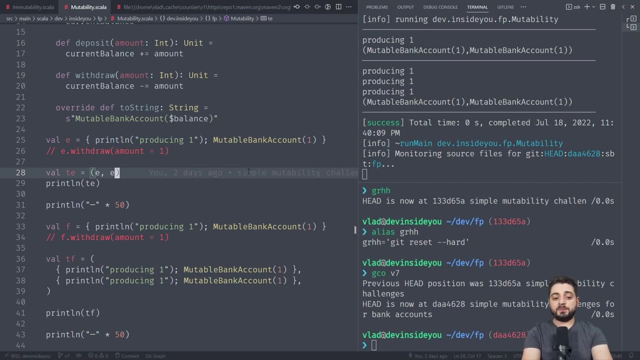 Okay, So let's do git checkout v7.. And I'm pretty sure that in v7, we're working with immutable bank account. Okay, Now It's exactly the same thing, Right? So we're creating something, Right? So there's something on the right hand side of the equal sign. 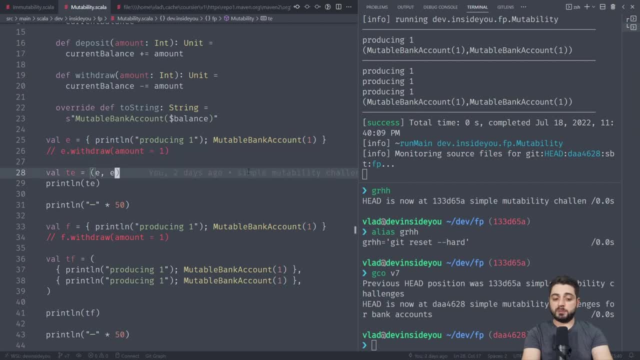 Right, We're not doing that yet. Okay, We're putting like two of these things into a tuple, Then we're doing a print line. Now, one important thing to notice is that, just because you have mutability, or just because you you know, you're breaking the substitution model for procedure application. 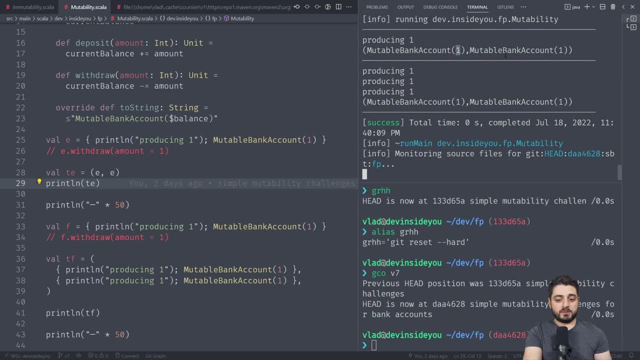 Sometimes your program will behave just fine, Right? So, as you can see, the bank accounts are not affected. Obviously, we've seen these print lines, but at least the bank accounts are not affected And you can say: well, who cares about the print lines? 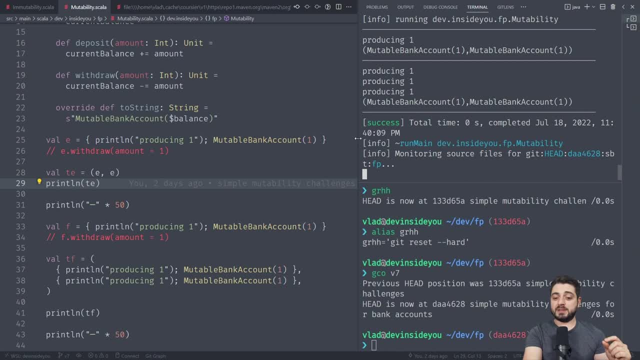 Right, But sometimes it is Right And this is the problem, Right. So because sometimes, with mutability, you will sometimes have bugs that are very hard to reproduce, because if you wanted to reproduce them, you will need to talk to your users and 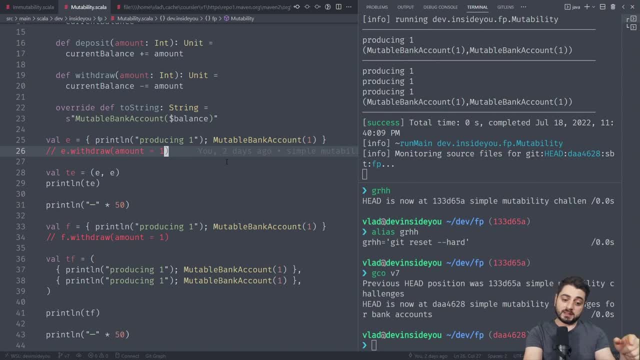 you would need to say, okay, well, what did you do? And then we'll say, okay, well, at first I did this and then I did that and then did that. And then you need to go to your program and you need to replicate exactly the same thing. 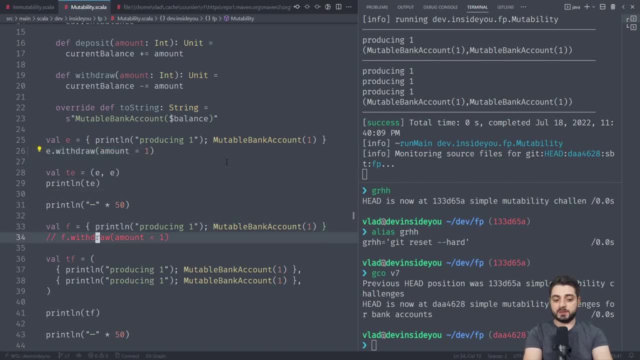 Okay, So here's an example. Right. So if we, if we do this right, then all of a sudden not only print lines change Right. The first- this bank account- and the second bank account was not affected. Okay. 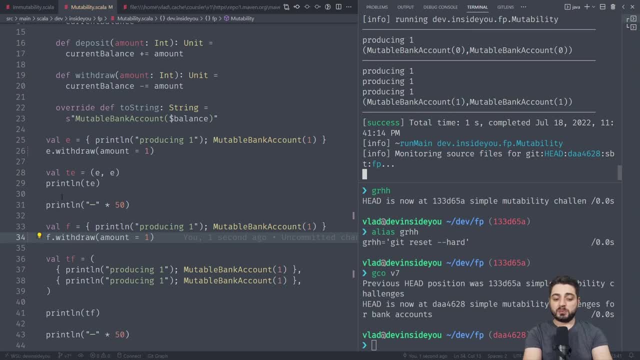 So second second bank account is still is still a one. Okay, So now these programs don't behave the same. The substitution model is broken, And why is that? Because this expression cannot simply be treated as an alias to some value. 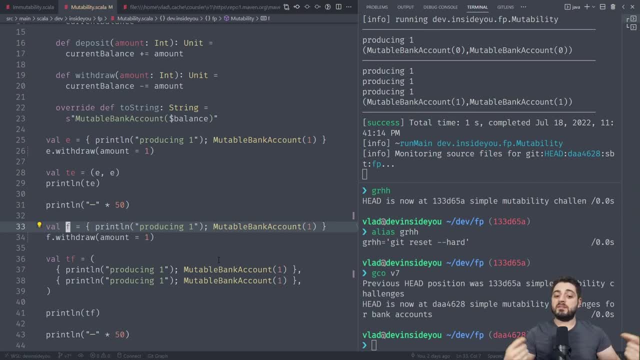 It is an alias only within some environment. In fact, the model that you need to apply here to think about your programs is called the environment model for procedure application. In fact, these are just like the official computer science term for object orientation, which is the environment model for procedure application and functional programming, which 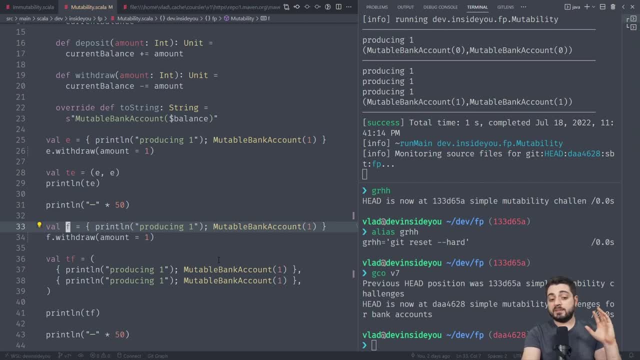 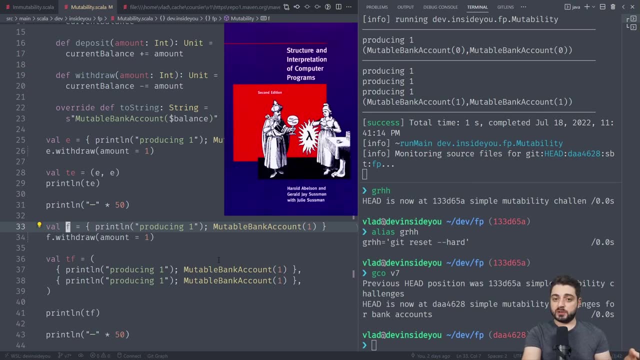 is the substitution model for procedure application, And I have very, very old videos about this And most of the stuff comes from a wonderful book called SICP, which stands for structure and interpretation of computer programs, And I have a review somewhere on my channel. 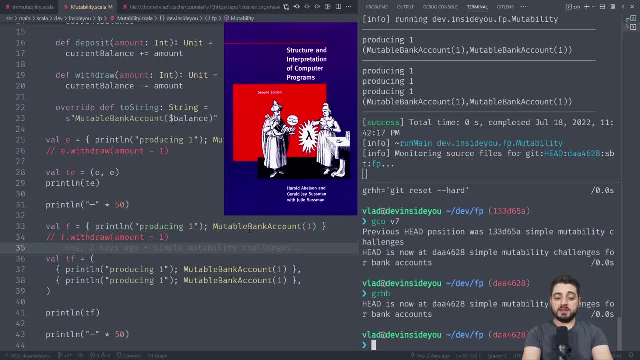 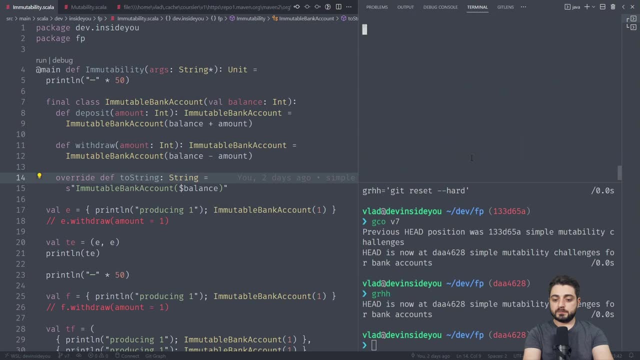 I'm sure you can find it. Let me throw this out and let me demonstrate the immutable version. Okay, So let's switch to running the immutable version. So, as you can see, it's the same thing, right? So ignore the print lines, right? 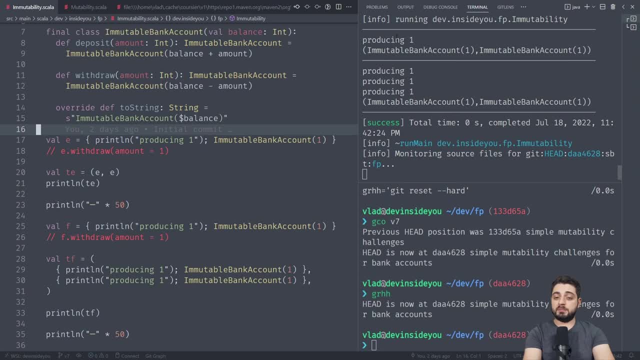 So the print lines are still messing up with the substitution model And you know the rest of the video is going to explain how to how to solve this problem. Okay, So look at this: If we enable these things, the bank accounts are still not going to be affected. 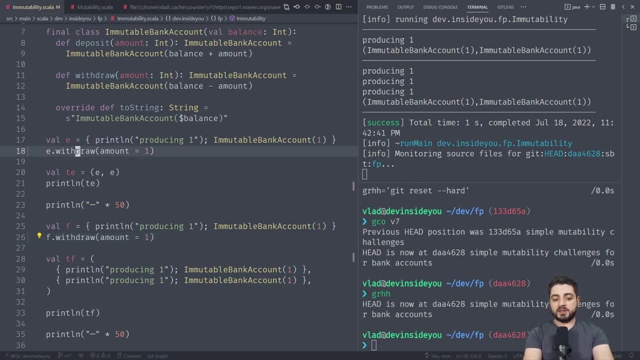 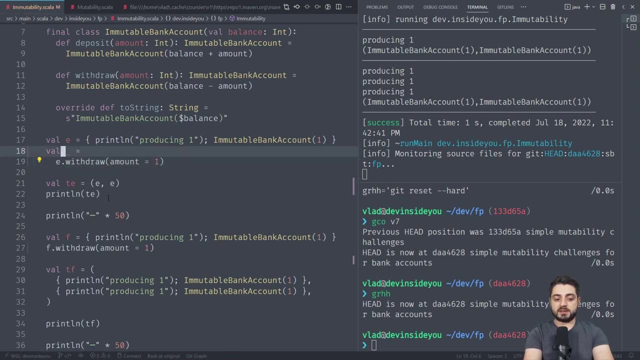 Right. Why? Because this simply creates another bank account And we're throwing it out. Remember this thing, right? So this equals sign- I'm sorry, this underscore here- And this equals sign, This underscore here- is another bank account. 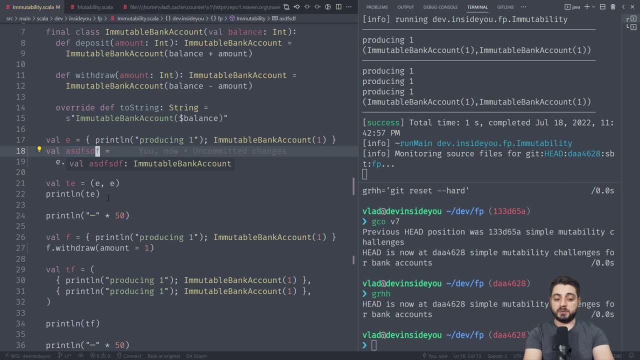 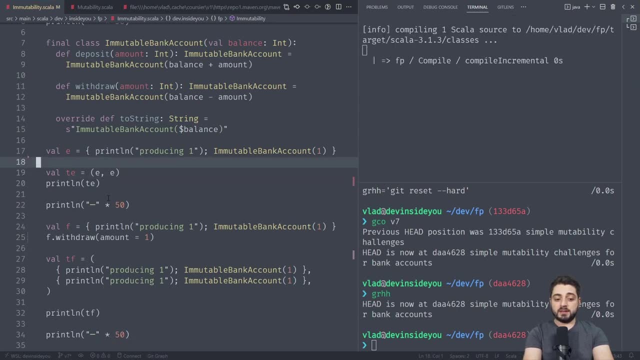 Right. So if I were to give it some name, you know my ID will actually tell me. well, this is actually an immutable bank account. We're not doing anything with it, Right? It doesn't participate in the rest of the program, which means that, you know, none of this stuff is affected. 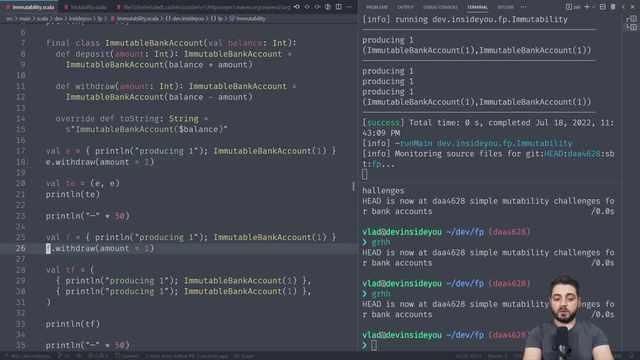 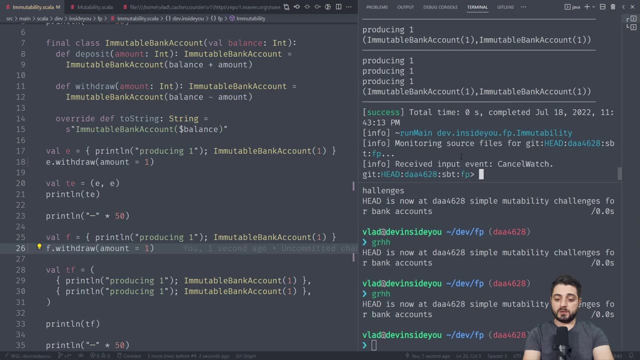 Right, Like this, Okay. So either like this or like that, everything is fine, Okay. And one important thing is that let me actually switch to the immutable version again. It is very hard to reason about this If we go to immutability. 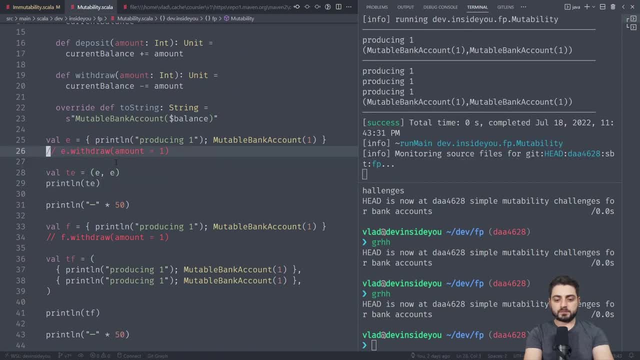 All right, And we do this withdrawal. Well, actually, look at this, So there's like one, one, one, one. Okay. So over here, this two string, which is something that I added, which you know, just prints out the bank account. 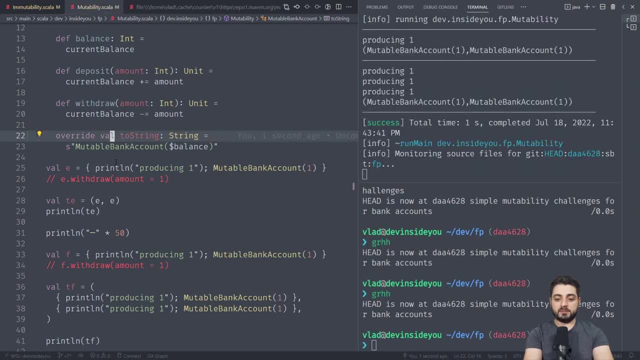 We change it to a val, It behaves the same. We change it to a var- Behaves the same. Well, it cannot be a var, Okay. We change it to a lazy val: It behaves the same, Okay. Now let me change it back to a def. 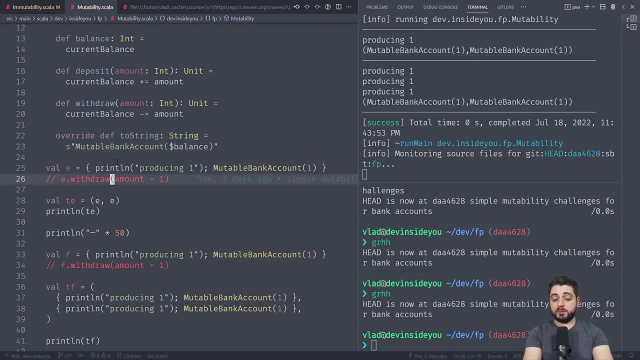 Okay, So this is a very interesting point, Right? Because, depending on what your program is doing, you might or might not create bugs, Right? So you have already broken the substitution model, but so far it doesn't bother you, But sometimes it does. 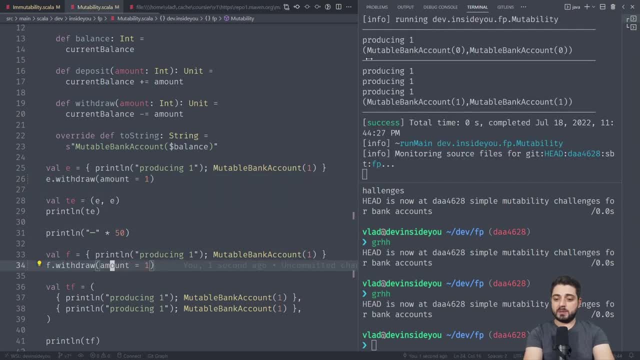 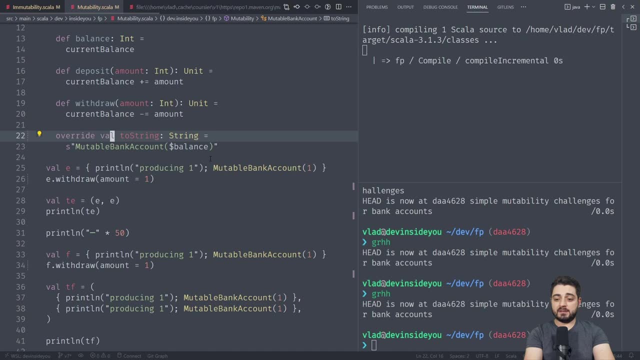 Right. So if we have this, Okay See, we have like zero, zero, one, one Right. So it's already not the same. But now also, if you go over here and do a val instead of def, then stuff change. 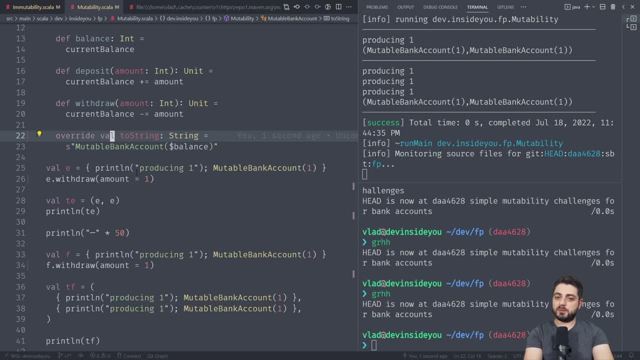 Okay. So it's very, very, very hard to reason about programs like this. Okay, Because the substitution model is broken, Right. But only because it's broken doesn't mean that you easily see it, Right, All right, So next one. 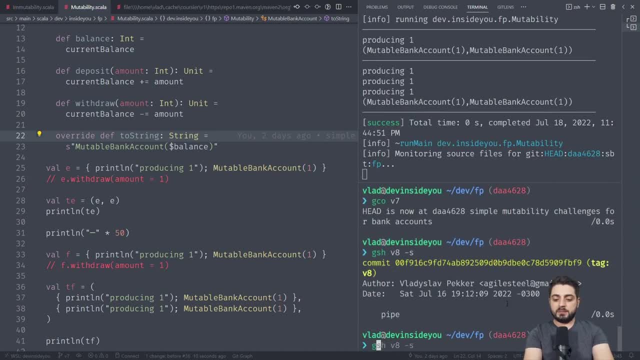 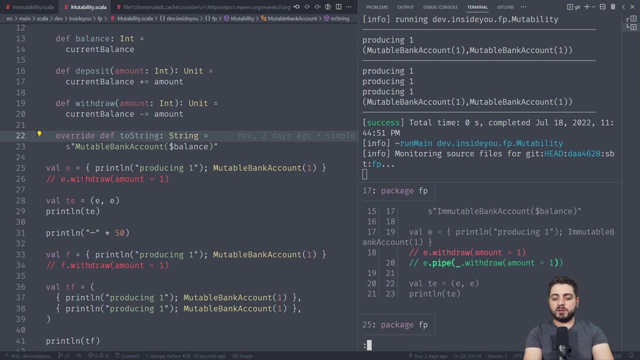 Let's show V8.. I believe, over here. I just wanted to show you the pipe because I introduced the pipe before, Okay, And it is over here, Okay, So this is going to be very no, it's actually. there is actually another reason why I'm introducing. 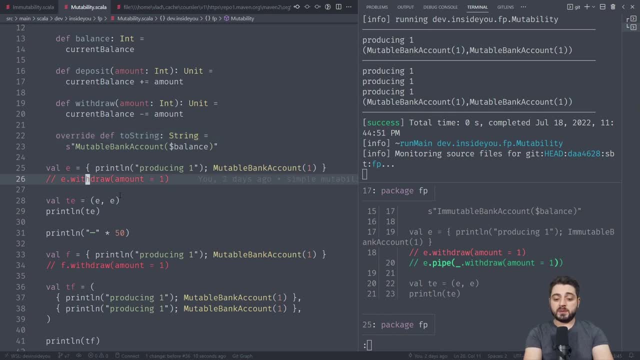 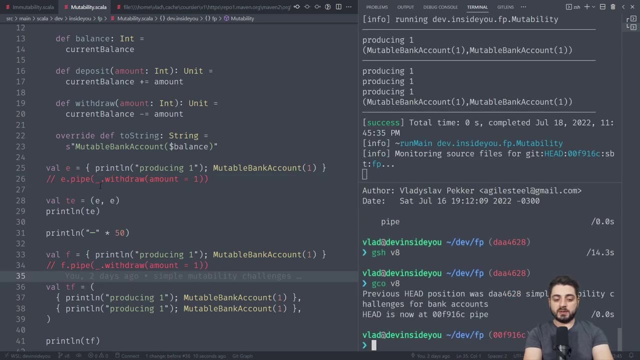 the pipe. It's going to be very, very similar. Okay, So another, another way like to write this would be like this: Right, So look over here, Right? So instead of just like doing like E dot withdraw, we can do E pipe. 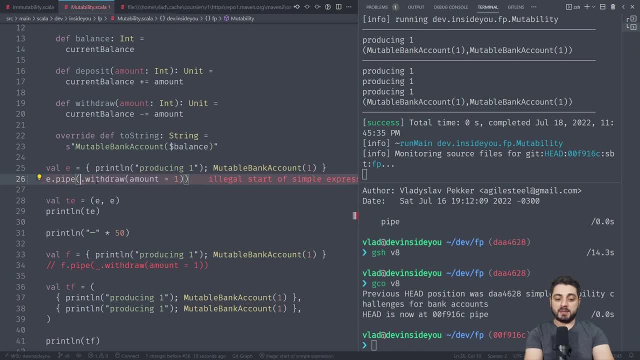 And then, like this is going to be, this is the same as, okay, Like it's, it's still. it's still the same, E Right? So this is like a little bit of a silly code, but but later it's going to, it's going to. 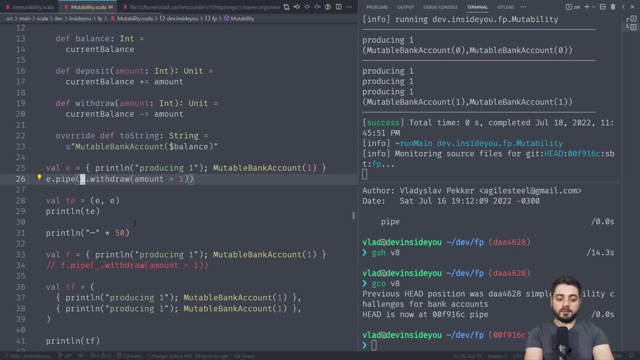 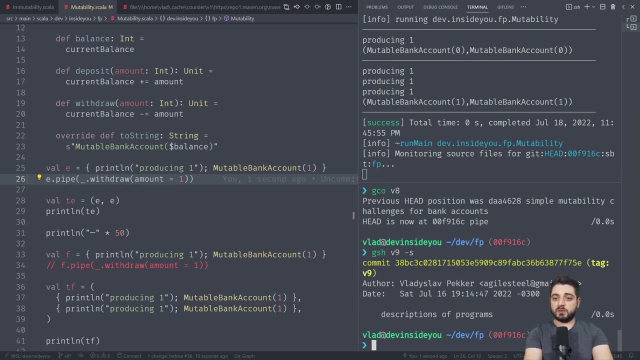 make sense. Okay, Like this: All right, Let's, let's have a look. Okay, So, let's have a look at the next one. This one is very, very important. Okay, So remember when you still need to solve the, the print line somehow. and, by the way, guys, 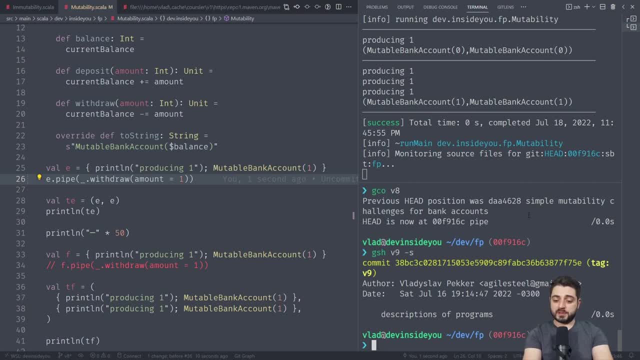 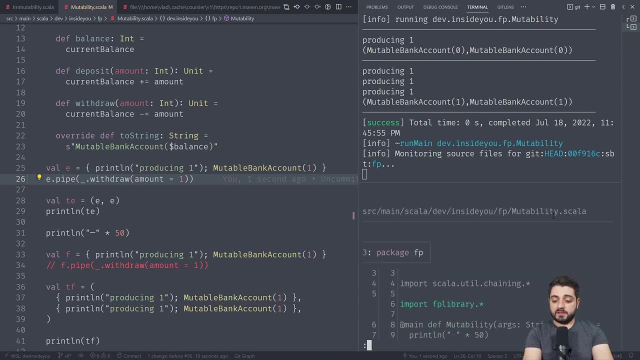 don't forget to hit the like button so that more people stumble on. this video really helps out the channel. All right, If I'm correct, then this is another one of those commits that is very, very important. Why are we having this problem with the print lines? 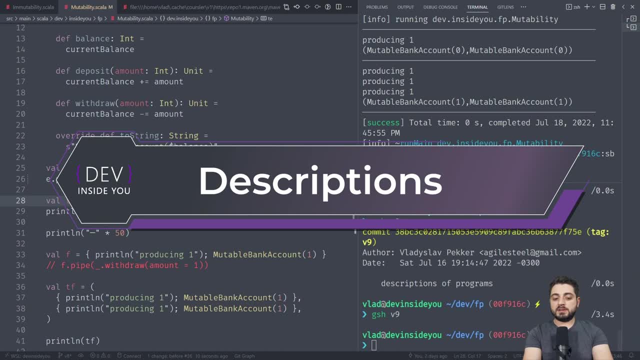 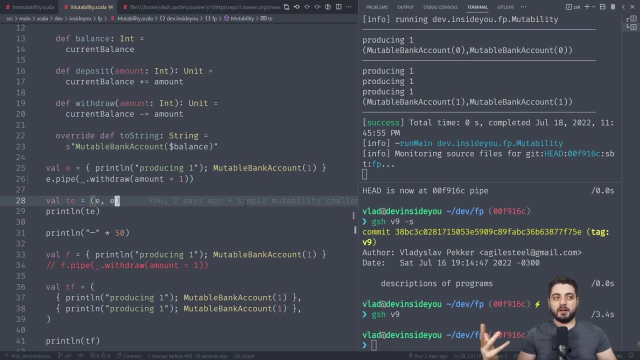 And usually the answer is because they happen too early. right, So they already happen. And therefore, you know, it's very hard to to apply the substitution model for things that already. they already ran, they already happened. you know, which is why most 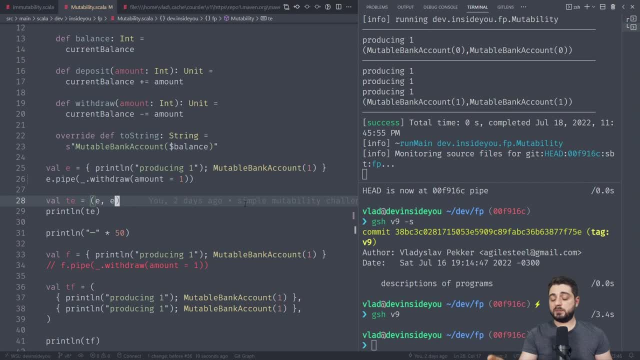 like very, very pure, functional programming languages, And we're going to talk about purity in just a second. Most of them tend to be lazy. They have. they have on-demand evaluation semantics, which means that this Val, you know, this code that is inside of these curly braces, is only going to be run when we're actually 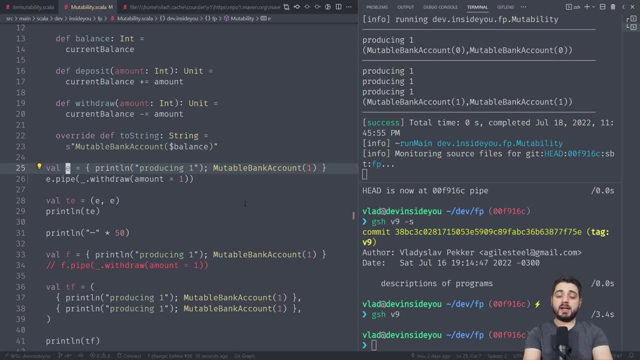 going to use the E. okay, It has different trade-offs, but like, this is what it is Like. most programming languages allow assignment, allow mutability. Therefore, most of them are so-called eagerly evaluated programming languages, or a strictly evaluate your programming, which means that if there is a Val, it's going to run immediately. 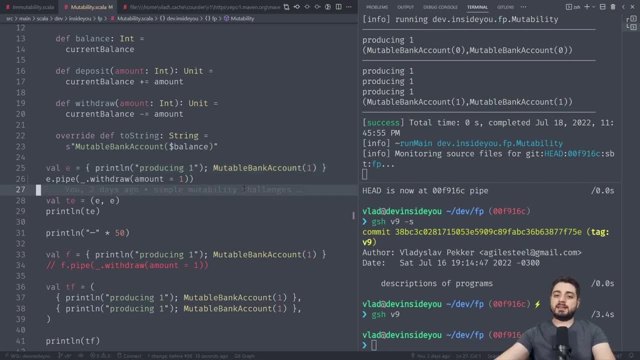 Even if you don't use it. Now the question is like: how do we solve this print line when we need to delay it somehow? right, Artificially delayed. And the way to delay it is basically to say: okay, well, we know that when this code runs, 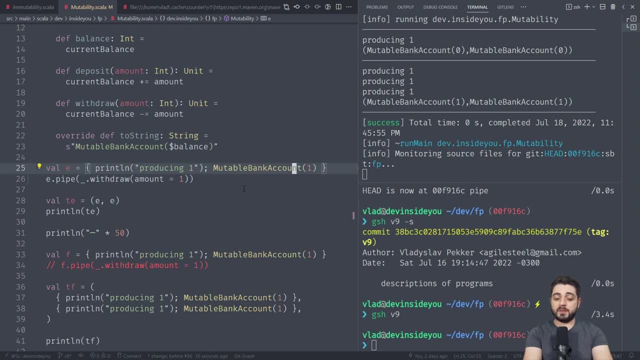 okay, Once we're going to, you know we're going to side effect, right, So let's not run this code, but let's remember how to run this code, Okay, Uh, usually, when functional programming is explained, the term description is used. 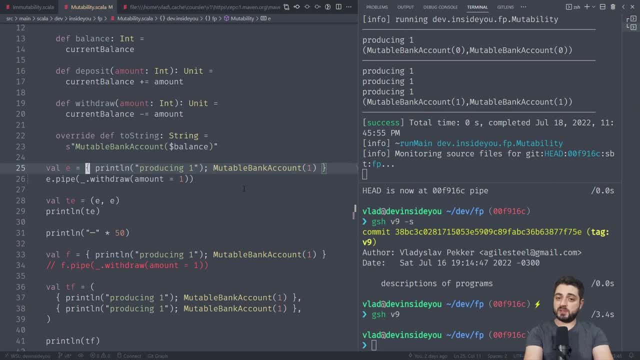 Okay, So let's convert this into a description of whatever happens inside of these curly braces. Okay, And the way you do this is by saying: okay, well, E is just going to be a function. you know that. you know it's not going to have any arguments, right? 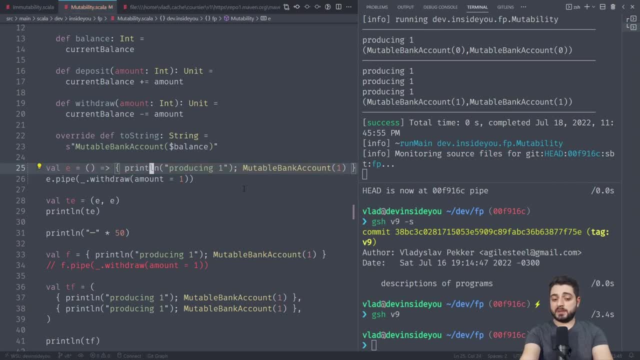 Uh, but when we're going to call it, then you know, then we're going to do the print line. So let's say we're never going to call it, Okay, Instead, what we're going to do is we're going to uh. so this basically delays this expression. 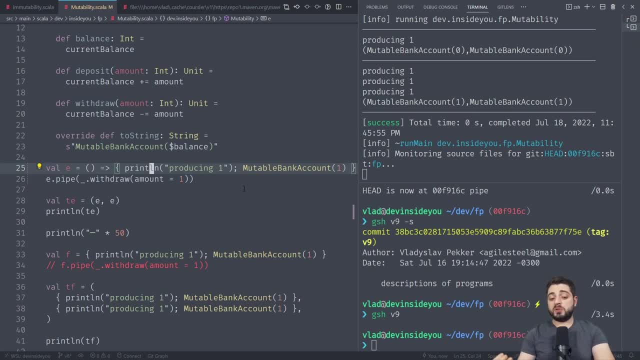 right. So we're going to delay all of the expressions. then we're going to figure out how to combine all of the expressions into one, And so your program, no matter how big- and I know it's very hard to imagine- imagine: 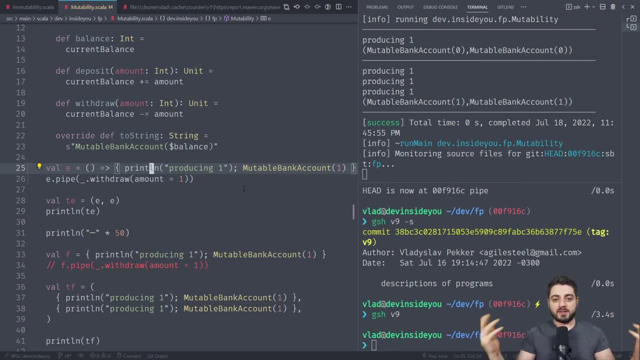 like a, like a backend application which, like, was like thousands and thousands of lines of code. All of them are combined in such a way that the entire program is like one function call, Okay, Okay. So let's say we're going to call this method, which we dramatically call, the end of the 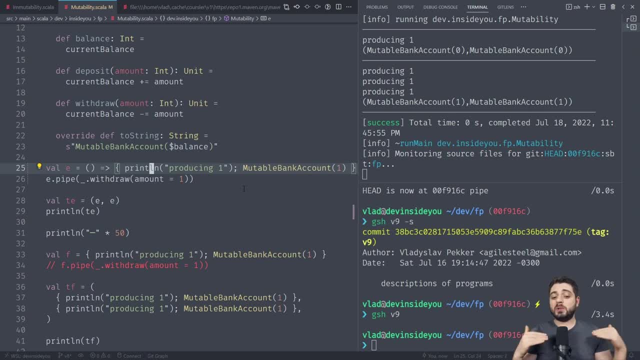 world. Only then we're going to call this function. And so until we call this function, we're in this perfect world where the substitution model for procedure application applies. So we can very safely reason about our code. We can very safely- uh uh, refactor our code. 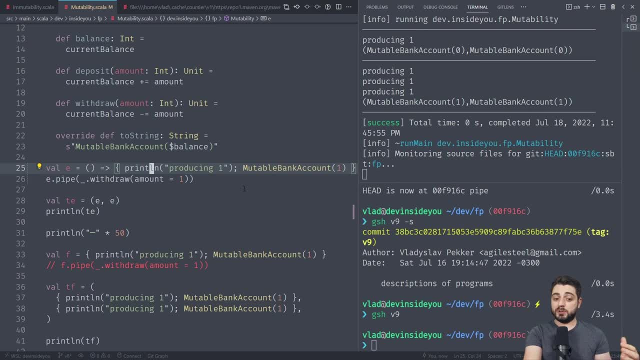 Uh, we don't have like weird bugs. We still have some bugs. right, It's not bulletproof, but at least we can reason about programs in the. it was the substitution model for procedure application. Okay, The next couple of commits and they're sort of like steps, uh to how it's done. 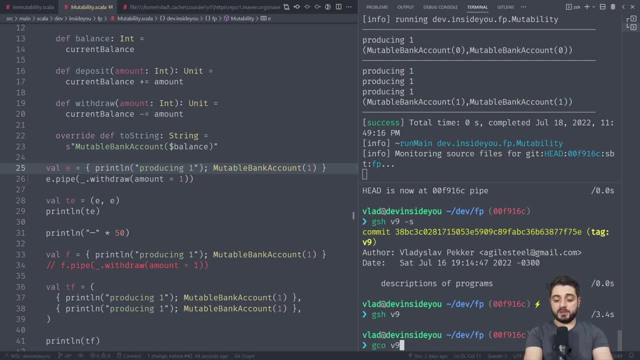 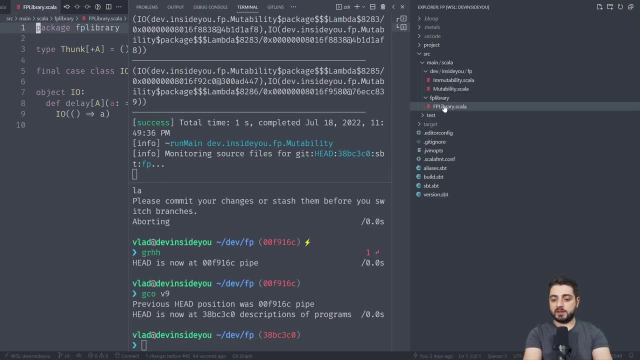 Okay, So most of this stuff is done in libraries. Okay, So what we're going to do over here is we're going to uh, write our own library. Okay, So it's just like over here, right? So it's just like another file over here. 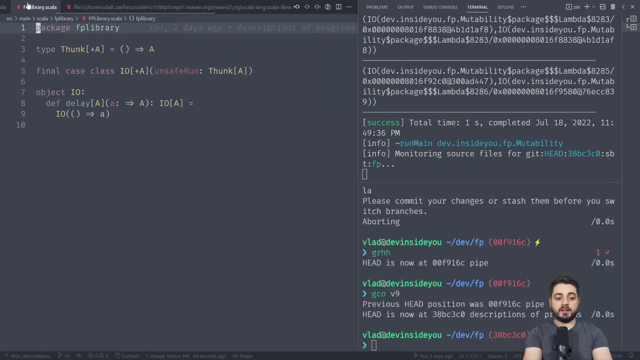 So it's like an in a package, uh functional programming library And then over here I just kept writing everything in this file, We're importing everything from this library and we're using, like uh, using it at the bottom. 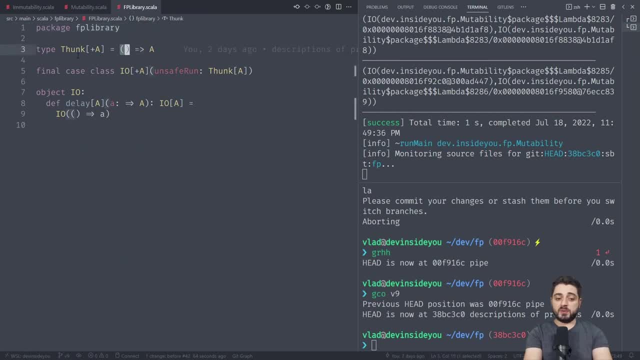 Okay, So, uh, a function that does not, uh, contain any arguments is called a thunk. Okay, So this is a thunk that will produce an eight. Ignore this Completely, ignore, Okay. So when I'm going to call this function, by giving it no arguments whatsoever, it is. finally. 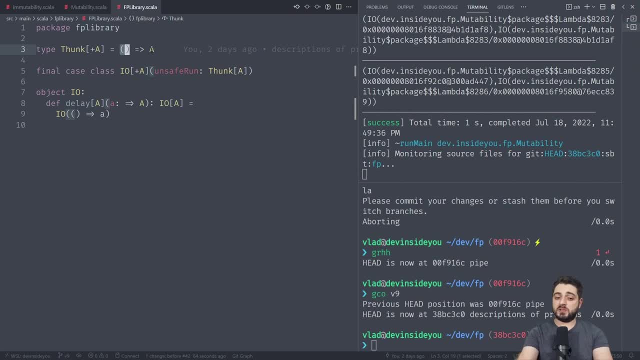 going to give me the eight, Like in our example, the eight is actually unit, because it's just going to be like some sort of print line. Now, for convenience, we're going to take this thunk and we're going to wrap it into a data. 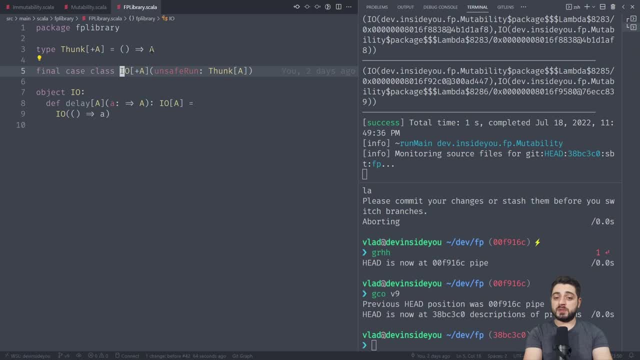 structure and it's going to be called IO, which stands for input, output, right? So it's for those things like okay, like how do we actually send an email, or how do we actually read something from the database, How do we print stuff out? 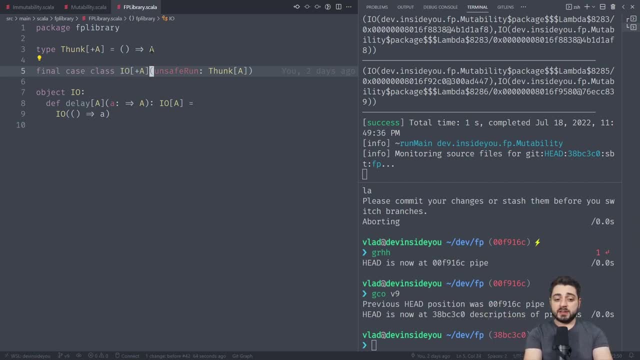 How do we, you know, read, you know, user input in there? It's just a data structure That contains one of those thunks right, And usually it's called unsafe run because, um, until you run it, your your entire application. 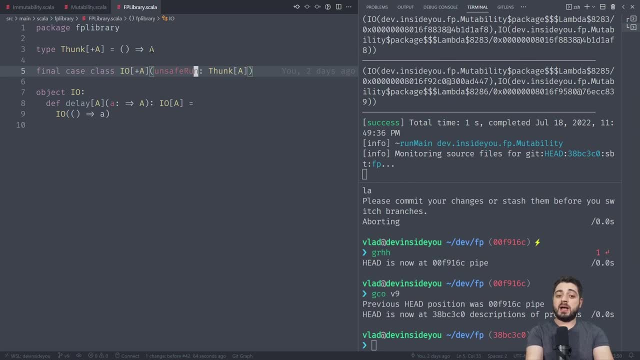 is safe right. It means that it's within the substitution model. However, as soon as you run it, all bets are off. but you're not going to run it And we're going to. we're going to get to that point. 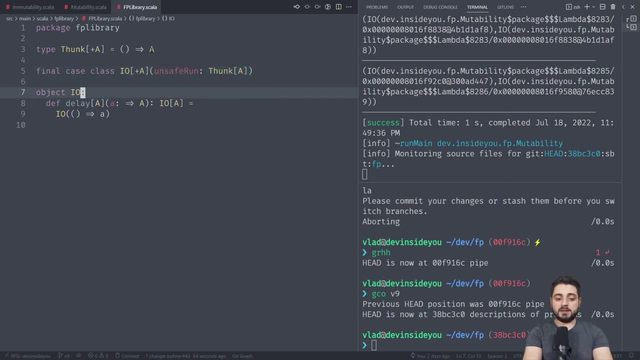 Now, this is a companion object, um, for, for this class, And if you're not familiar with Scala, companion object are: are ways to have sort of like static methods, right? So, uh, we can do IO dot delay without having an instance of IO. 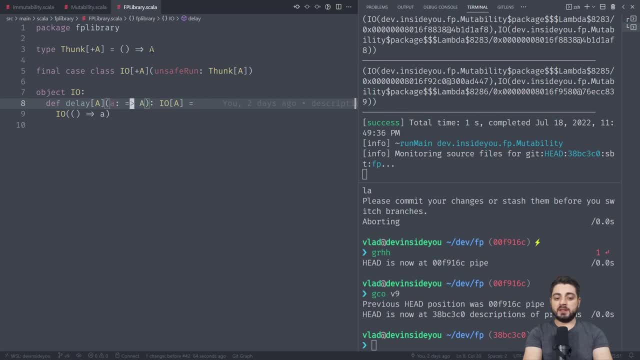 Okay, And there's just a helper function to uh, where we can give it an A, and it will wrap this A into a thunk and it will wrap this thunk into an IO. And there's a tiny trick over here. Uh, this is called a by name parameter in Scala, right? 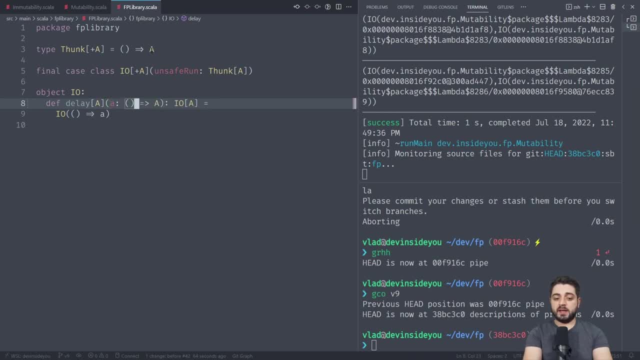 And you can think about it as if this was already a function right, And so over here we're just calling it like this right. So this means that, um, and then no circumstances. is this A evaluated right? It's, uh, you know, if you give it a five, this five only be evaluated. 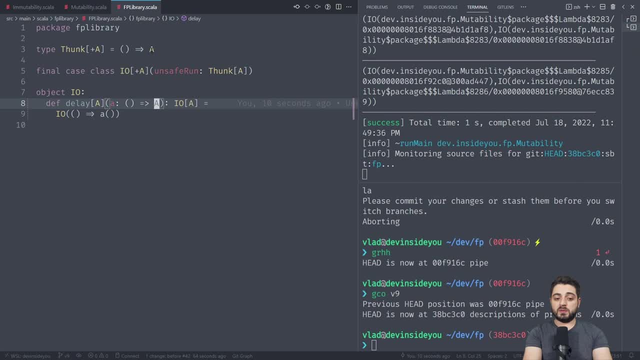 At the very end of the day, when somebody calls unsafe, run right. So over here. this is just like syntactic sugar for what I've just shown you. The value of A is not is unknown here, It's just being captured in the function. 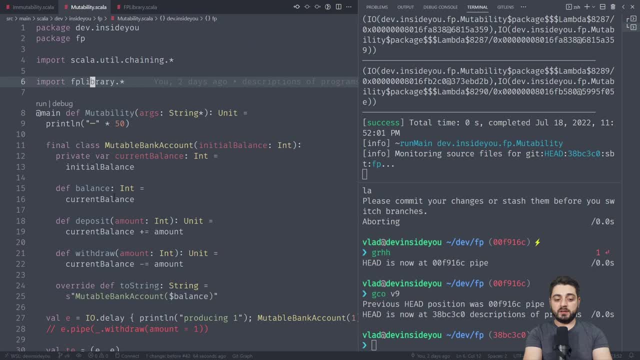 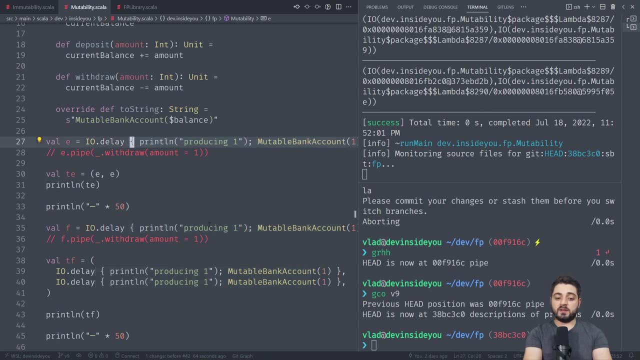 Okay, So this allows us to do like uh to to go over here, And whereas before we just had these curly braces, uh, now we can just say IO, dot, delay. and in Scala, whenever a function has only one uh argument, you can uh replace you. 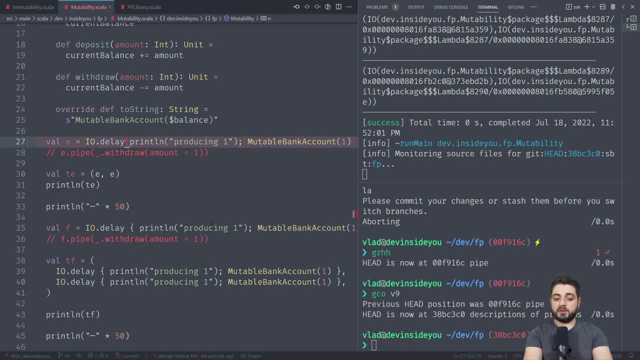 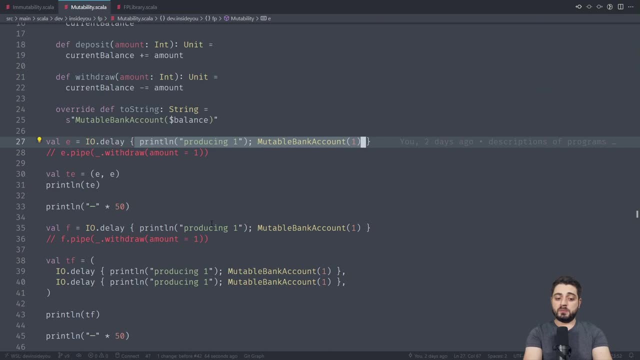 know the parent, which would be like in any other language, right? Okay, The curly braces: Okay, So this is a function, call Um, everything inside of these curlies is one thing, And therefore we're passing this one thing to this function. delay, remember, is being 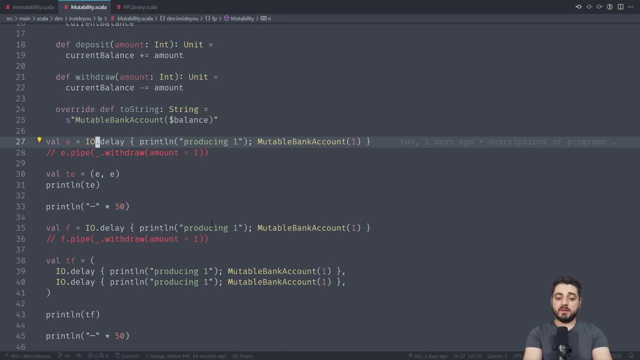 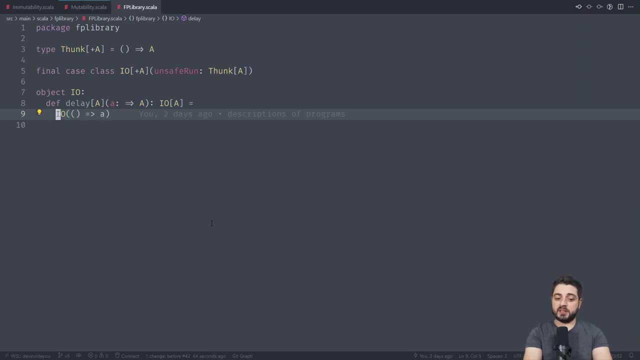 passed by name. So this print line did not happen yet. Okay, So it goes in over here. It is being stored in a Lambda. The Lambda is being wrapped around in a data structure. IO, just for um, just for uh. 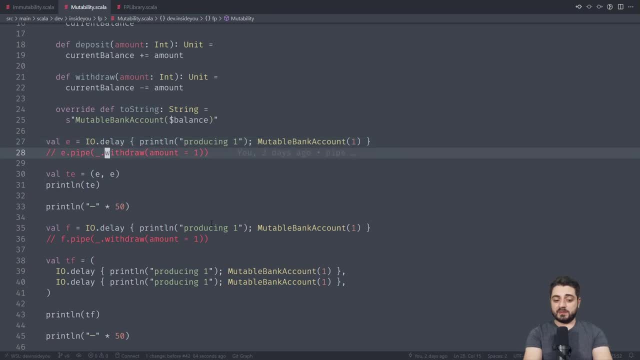 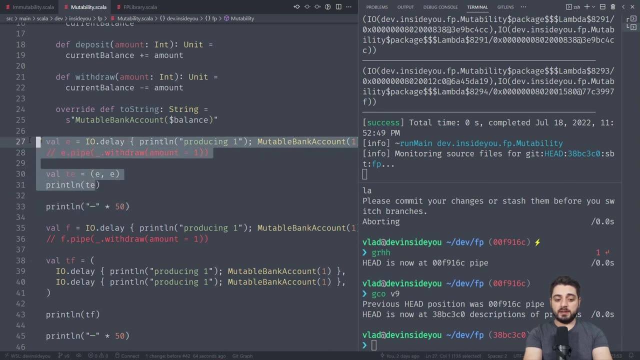 for convenience, Okay. So what happens now is that we don't have this withdrawal yet, Right, But like, what happens now is that already these two programs, like these two, well, technically like these two, right, Like print lines, like, like these print lines are just for you guys. 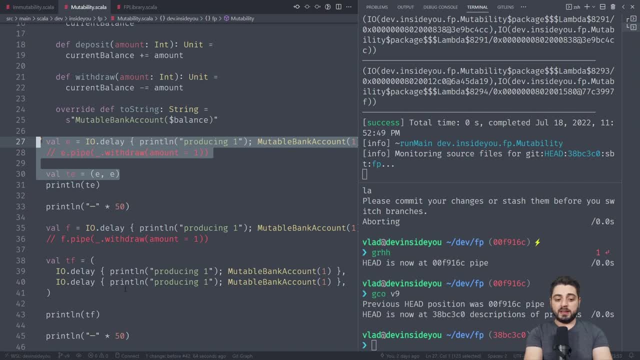 Okay, Just to see, Okay, But like, as you can see, like this program is now equivalent to this program, Right? Uh, you kind of see over here like the objects are different, but this is just a you know. 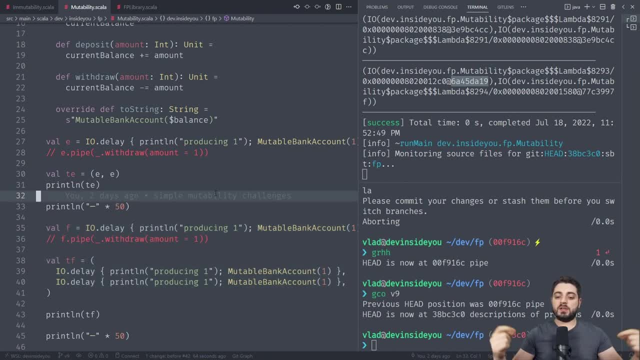 this is not. this is not what this is about. Right? Obviously, these are two different objects, Right, But the program behaves exactly the same. Right, Because what are those objects? Well, those objects are descriptions for for running computations. 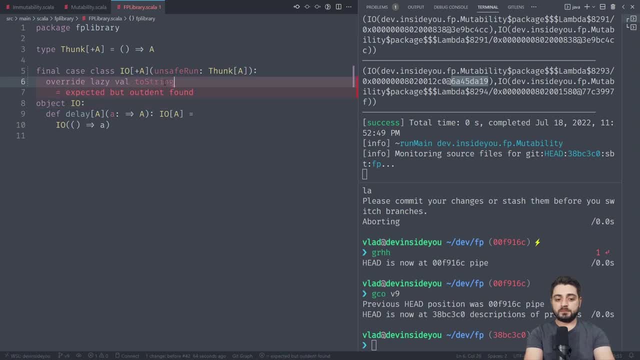 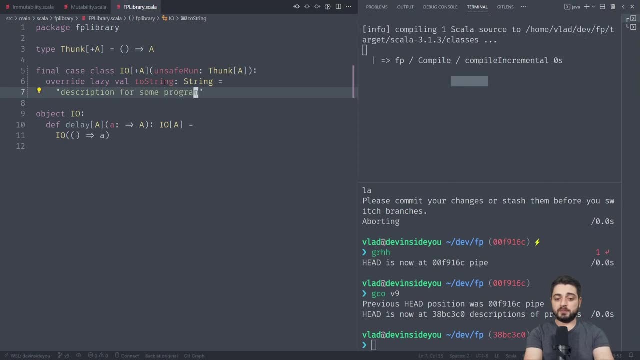 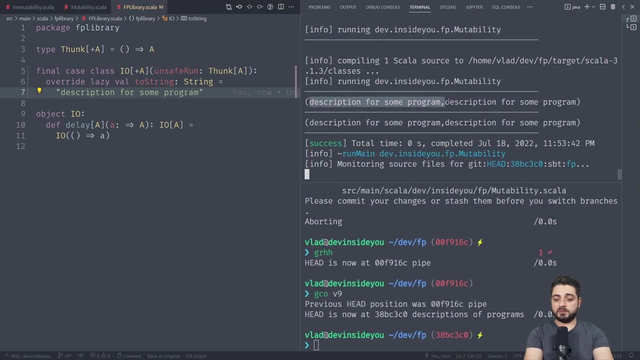 Okay So we can go over here Right And write a little bit of code and say, okay, well, I'm just a description for some for some program. Okay So, and as you can see, we just have two tuples each with with a description, description. 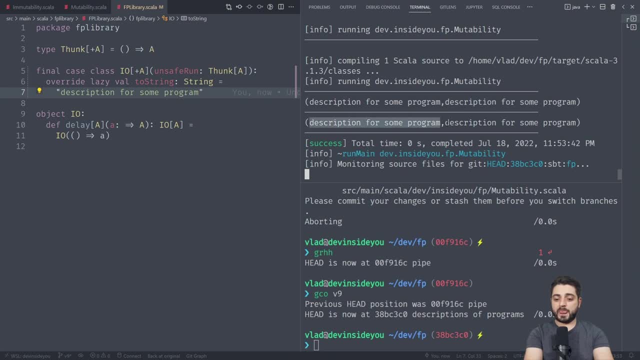 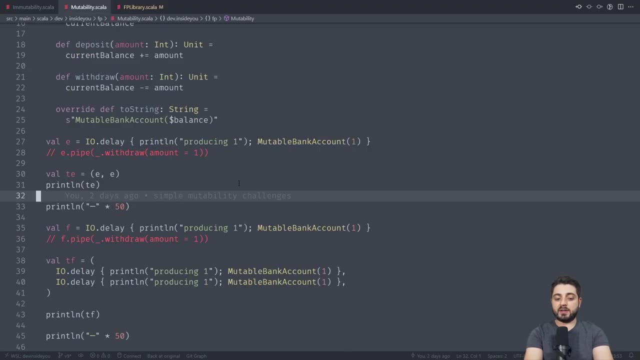 description, description, description, Okay, And there we go. This is it, Like, this is how this problem is solved. It just that now you kind of have like other problems. It's like: okay, how do you, how do you work with these things? 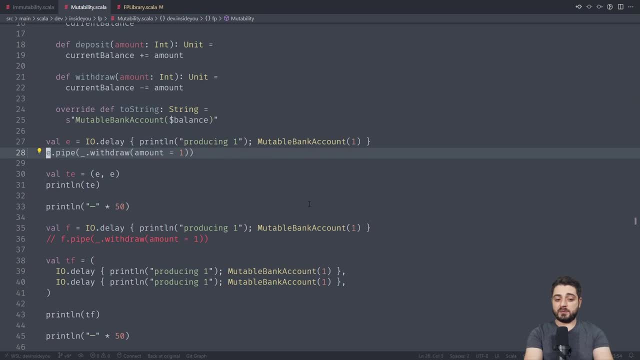 Okay, And this is how we're going to move on, because now we cannot do this pipe, Right? Because now it's going to say, well, withdraw is not a member of this IO thingy, Right? And this is how we're going to go to a function called map which is going to do what pipe. 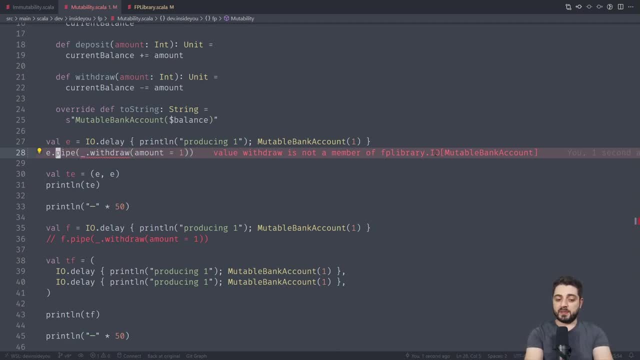 used to do, But for these, like nested things, these are at things, Right. So map will know how to go like inside of this IO and convert this value, sort of like, without running it. it will describe how to run it Right. 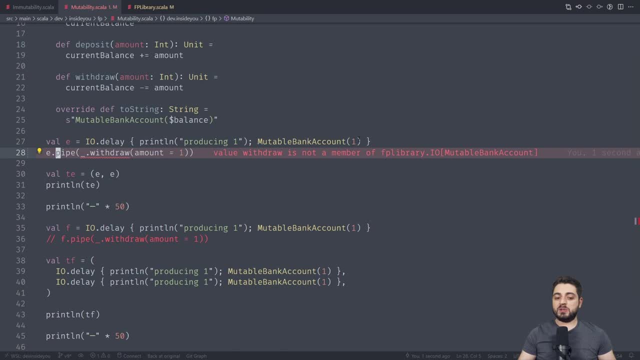 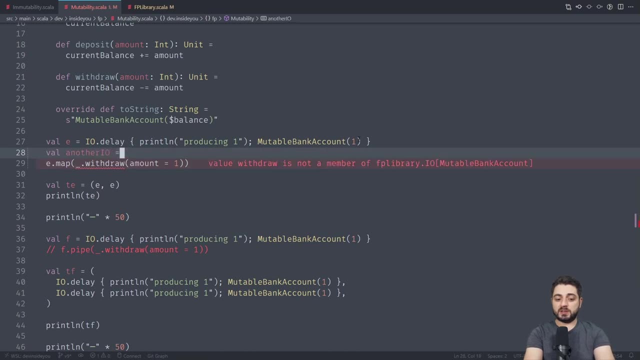 But, like none of this stuff is going to run just yet, Right. Which means when we're going to call map over here, it is going to produce just another IO, just another description And same as with the immutable bank account. we're not doing anything with it. 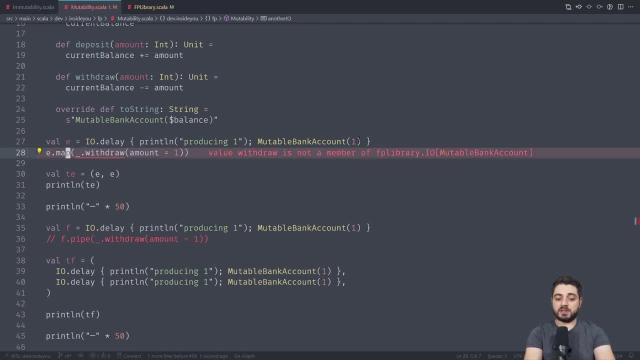 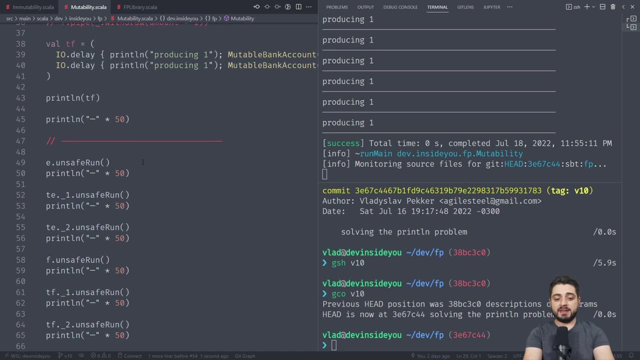 Right, And therefore it will. it will stay. uh, it will stay fine. Okay, Let's see. Let's see what is happening in the next commit. Let's check out V 10. V 10 now basically has this, this line, which is just a comment. 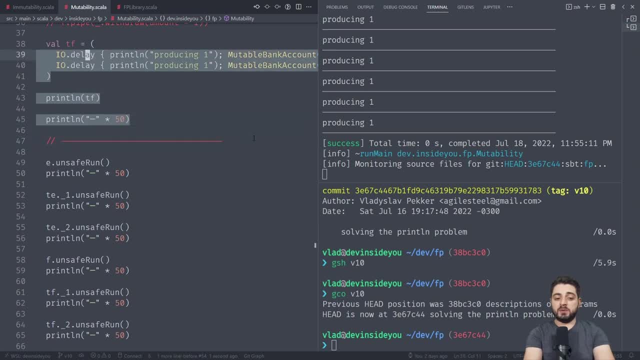 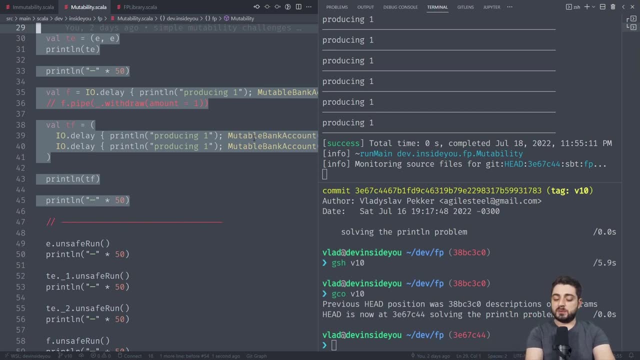 Right. But this is separation between between the immutable pro part of the of the uh, of the application Right, And I'm saying immutable I mean like between the part where the substitution model for procedure application is not broken and the other part. 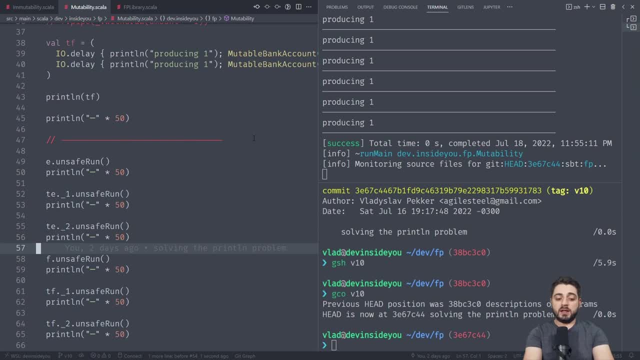 Okay, Okay. So if, if you're using uh in the programming languages, uh you, you will never even have this thing, For example, in Haskell, right, in Haskell, the main method does not return unit, It returns IO of unit. 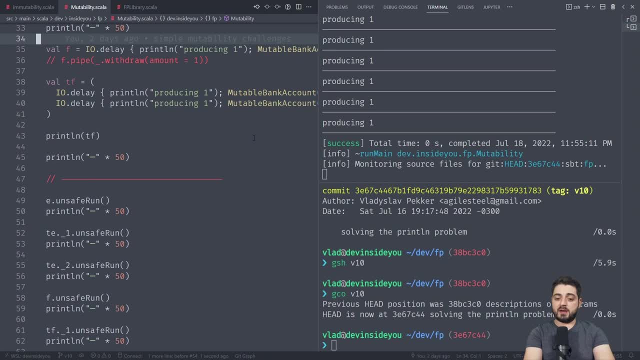 Okay, And so you will construct all of your descriptions somehow and you will just give it to the runtime and it will run it. So your program, like 100% of your program, is, uh, within the substitution model. Okay, get there, just yet. We're going to have conversations about this in just a bit. This is where we let 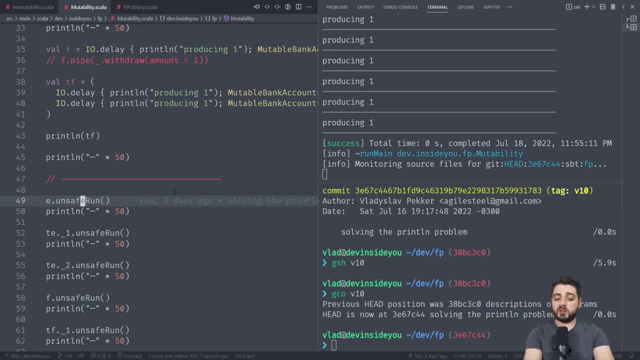 things blow up right. So this is where we break the substitution model by actually calling unsafe run. This is now unsafe right, And usually you would have like only one call to unsafe run. But over here we kind of like for now, at this stage we have like what like six programs, right? 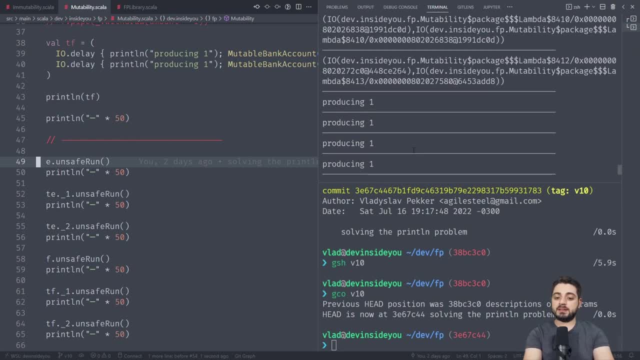 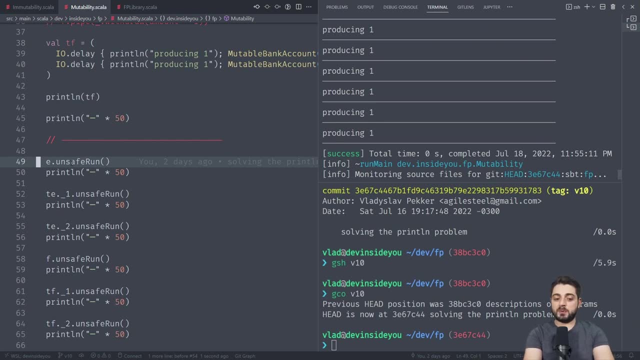 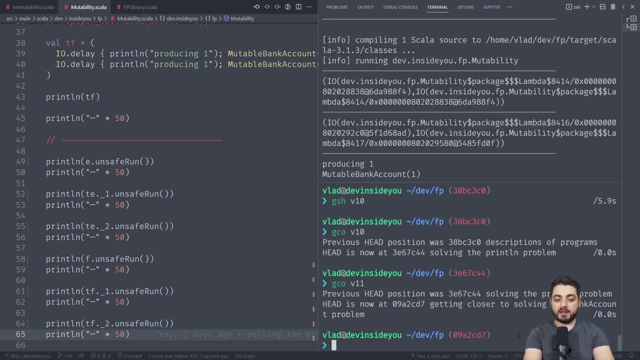 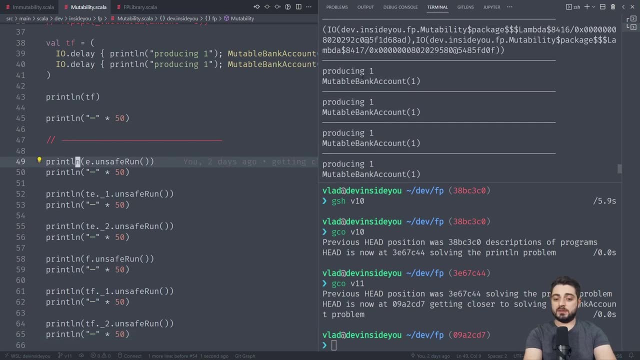 accounts. Okay, And I believe this happens in V11.. Okay, We're actually surrounding. this was a print line And now you see that all of these programs behave. you know, all of them are identical. Okay, They first do a print line or producing one, and then they're actually giving. 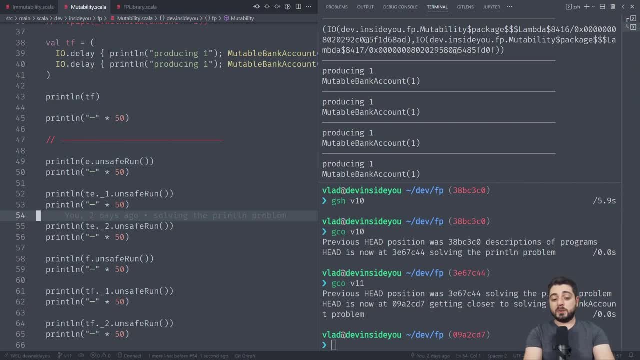 you the immutable bank account. So I want to reiterate a little bit. So what we did is we had side effects and we converted them into effects, pure effects, right? So what we did is we had side effects and we converted them into effects, pure effects. 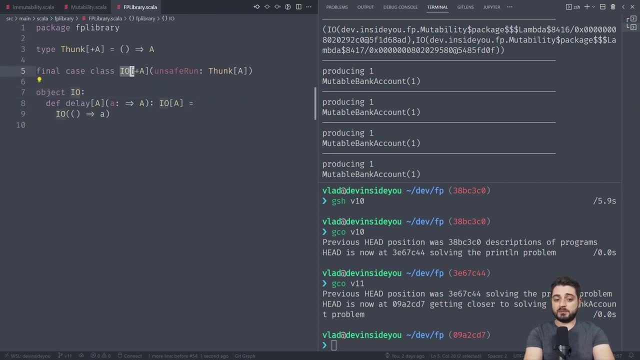 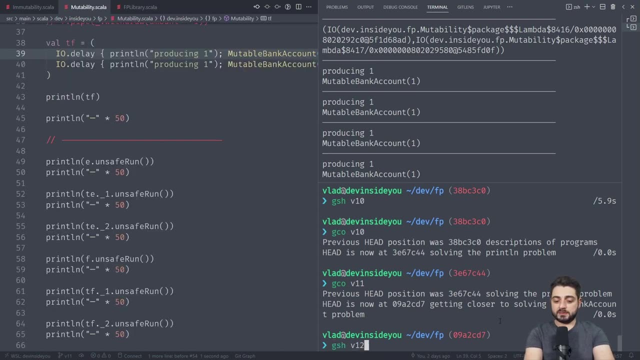 right. So this is also the reason why IO is sometimes called an effect type, right, But it's just a data structure, just to wrap around the thunk. Okay, Let's go back. Let's see what I did, what I did next, Okay, And by the way, we're going to. we're going to start. 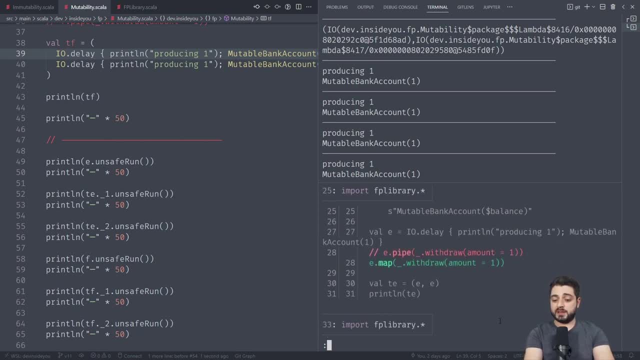 moving like faster, because you know we have 32 commits to go through, but we're already at 12.. Yeah, So the next one is the map, because we somehow need to withdraw right. Like how can we withdraw? Like the only the only way we can withdraw right now is by calling unsafe. 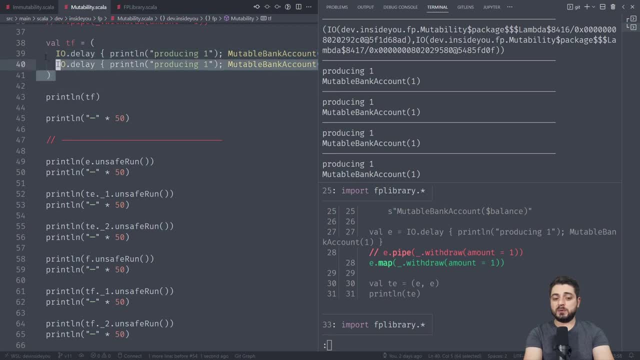 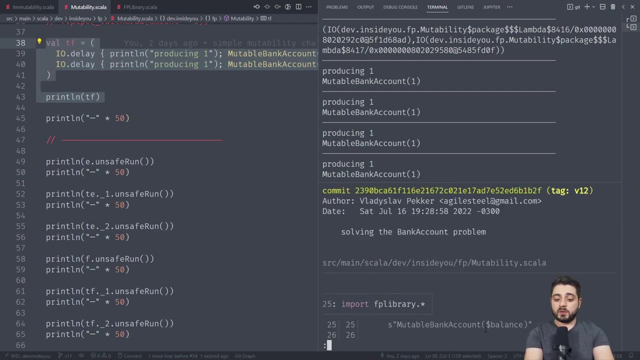 run, which we- which we don't want to do because, like we want, we want to do it here somehow And we cannot call unsafe run here, because we want to be in the safe world of the substitution model. Okay, So, uh, what we're going to do is we're going to: um, define a helper method. 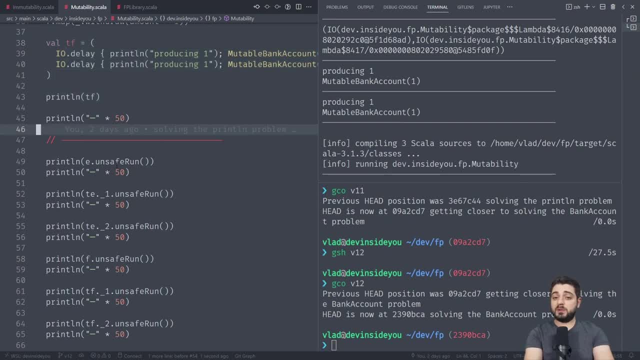 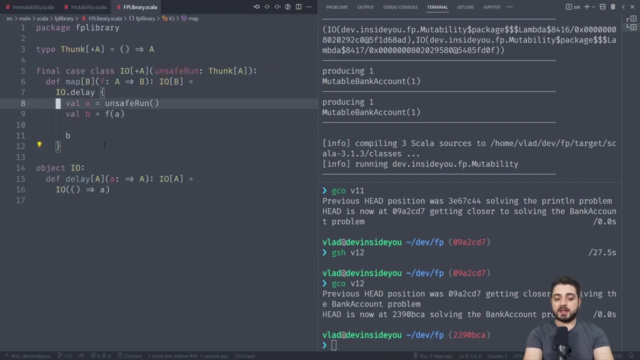 on IO, right? That will, in an immutable way, call unsafe, run for us, right? But it's not going to call it right. It's going to just create another IO that will call it once we run the entire application. Okay, So if we go over here, it's pretty much exactly what. 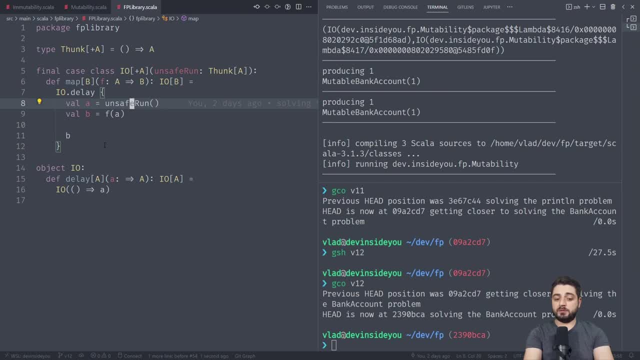 you know what we need to do. So unsafe run, for example, it would, you know, actually get the bank account right. So the A is the bank account right, Then we will apply the transform transformation which is going. 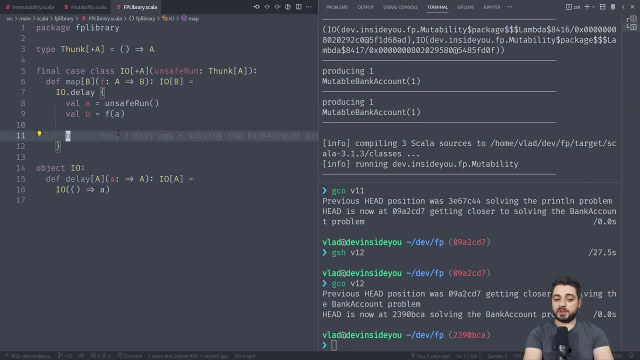 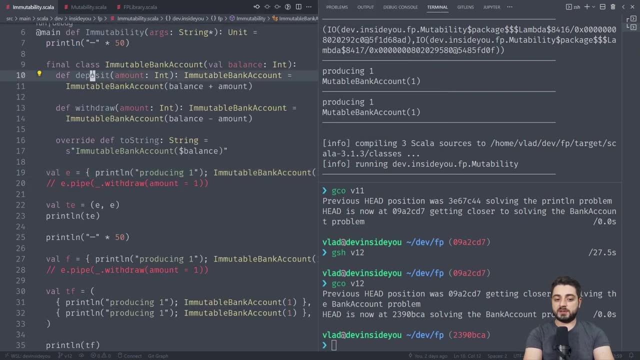 to be the withdraw something, right, And that's how we going to produce the result. Okay, So compare this with the immutable bank account, right? So if we go to the immutable bank account, okay, So something like a deposit, it's a very. it's the same pattern, right? There's. 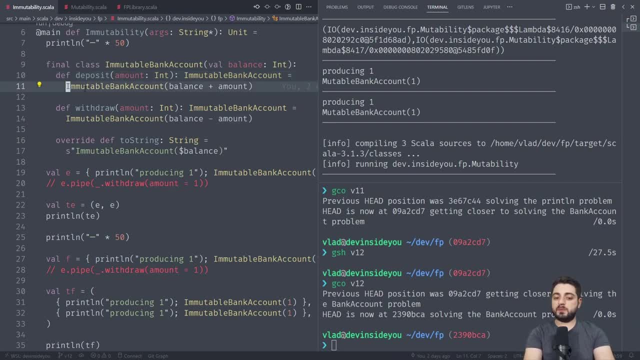 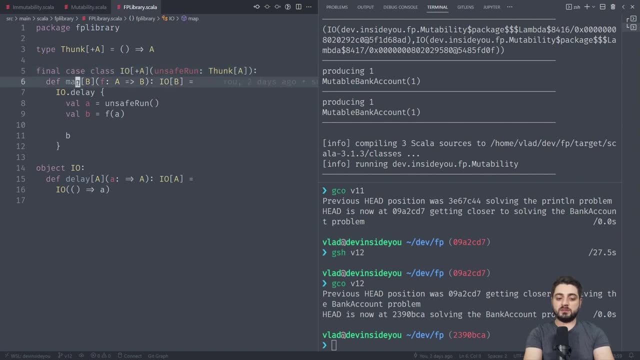 some parameter goes in, you know, and then the first thing that we do is we're creating another data structure right Another immutable bank account. Exactly Same thing is happening over here. We have IO, we have a function. It has some. 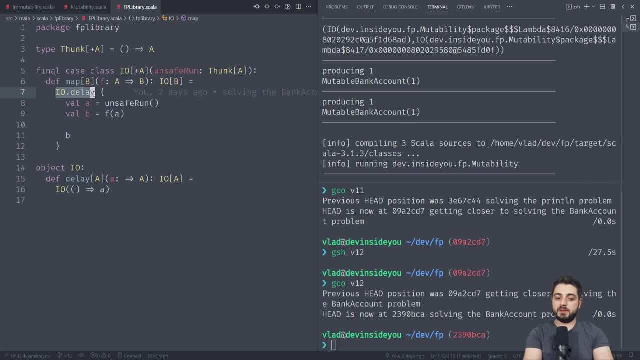 parameter. The first thing that we're doing is we're creating another IO, Okay, And does everything that is happening here is not happening yet. It's just a description, right? Because remember, like this is just syntactic sugar for creating IO and, you know, giving it a. 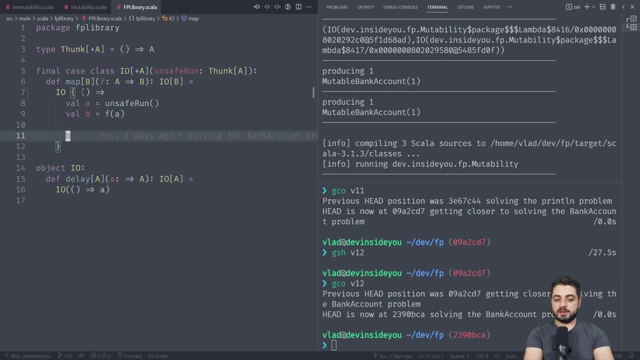 thunk. Okay, So all of this is inside of, inside of that, right. So th? this is just like a helper. this goal does not run yet, Okay, So we're just giving it a function. you know, we have an i o of a, we want an i o of b, so we give it a function: how to go from a to b. 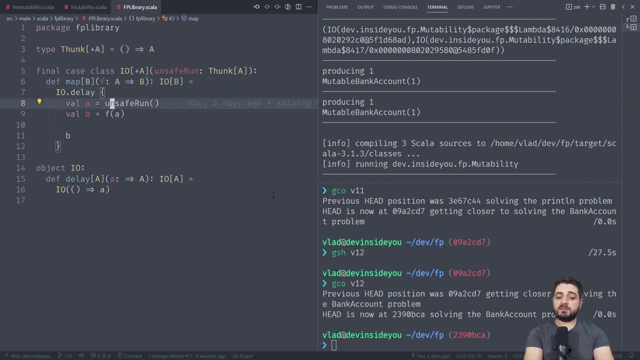 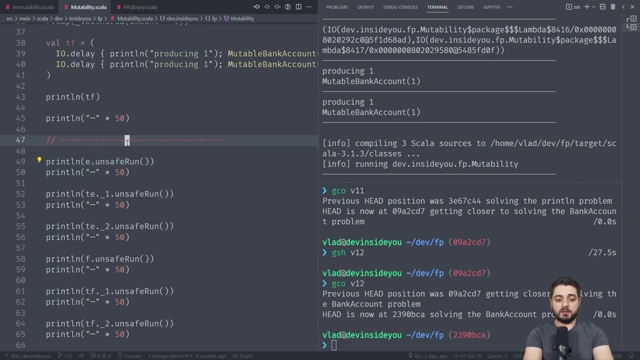 okay, it creates an i o. it calls on safe run to get you know. it describes how to call on safe run to get the a out. it sticks it into that. this function over here, right, this is how we get b out. and there we go. we have i o of b, okay, and so now, over here, what we can do is we can map right, but, as you can, 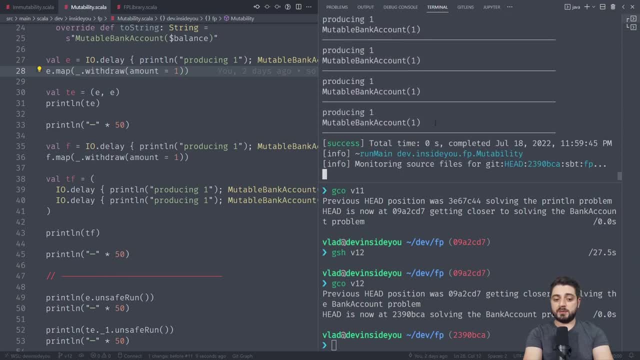 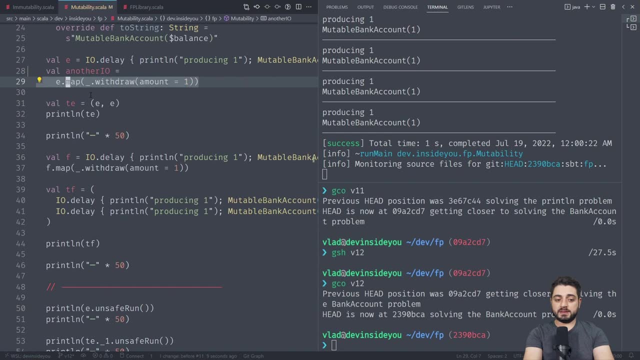 see, our programs are not affected. right, the programs are still the same. why? again? because this is just another i? o okay, and we're not touching this other i o right, this is an i? o of unit, but we're not doing anything with it, so it doesn't affect our program at all. it's exactly. 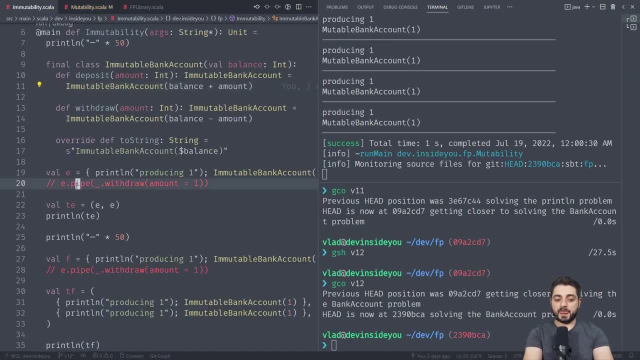 the same as what happened to our immutable bank account. right. so over here, you know, right, it just creates another immutable bank account, but we're not doing anything, we wouldn't care about it. it's a new bank account, like whatever. okay, so let's see what happens. 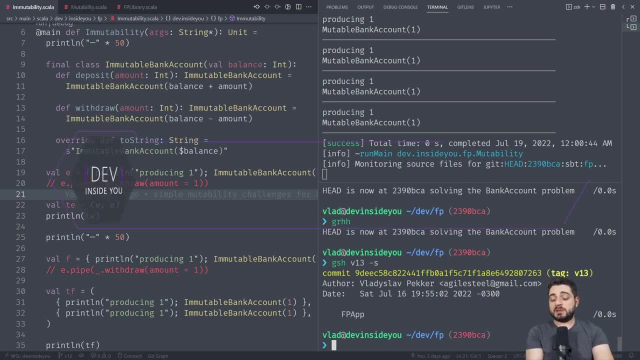 in in 13.. this is this is an important one. this is what i was saying before in a in a in a programming language like haskell, um, this runtime that knows how to run this description is built into the language in scholar. we don't have that and, in fact, this is one of the biggest reasons why i'm making 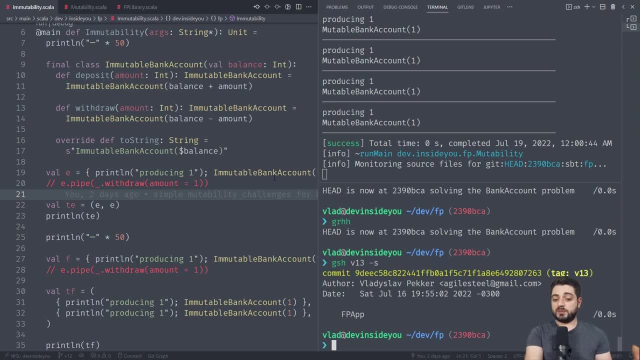 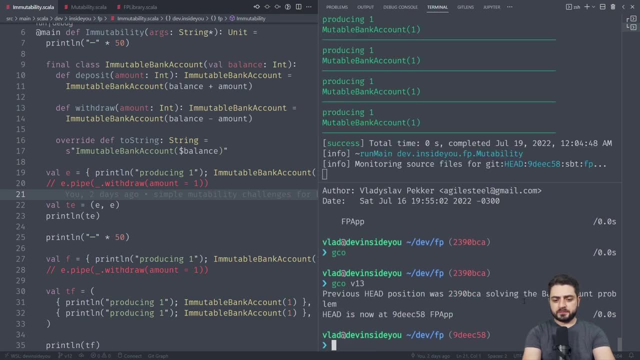 this video is because we have competing libraries that try to do that. what these libraries do is they um, create a um, they create a trait, usually called like fp app or something right. so i put it like in the fp library, and then i'm going to create a new one, and i'm going to create a new one and i'm going to 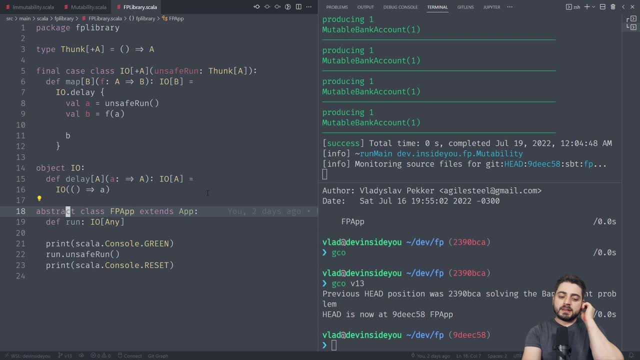 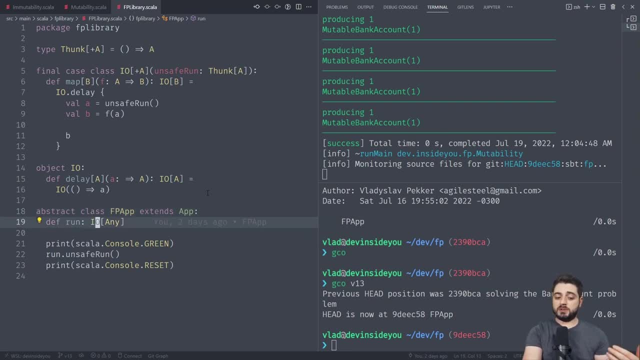 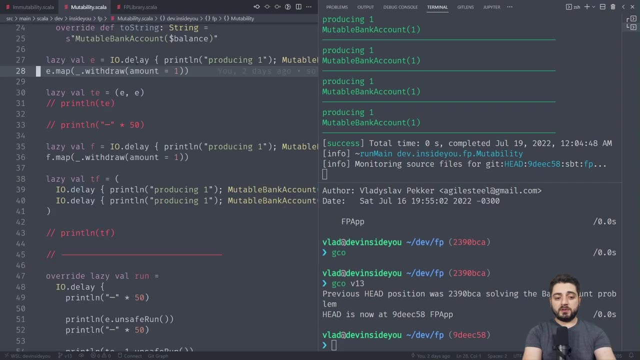 template class where you implement the run function, which you know. you give it an io, if any, and all it will do is it will call unsafe run for you. okay, so essentially what happened over here is that i removed this like dev. the whole thing now became an object, and i do like extends. 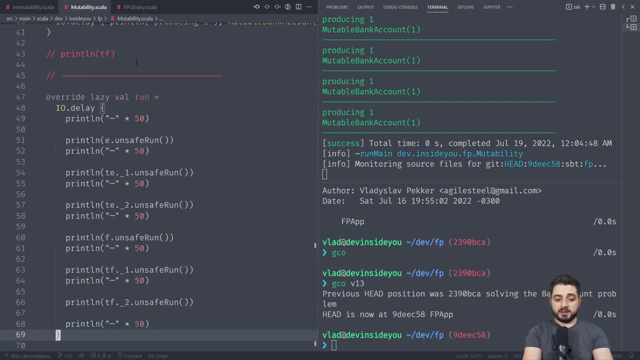 fp app: okay. and now somewhere at the bottom i'm going to say: well, run, run is going to be this one delay, right? so we're giving it like one, right? so, um, technically, like this line is not correct anymore because, uh, because this is still like one description, okay. 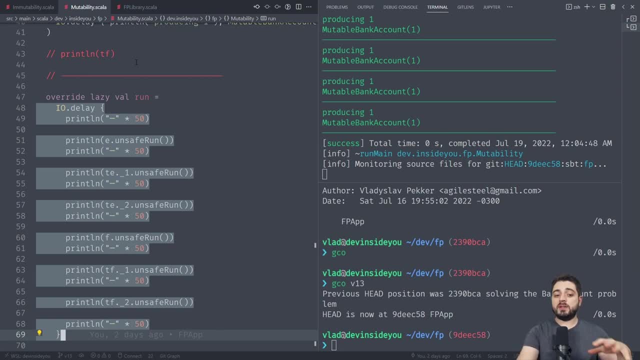 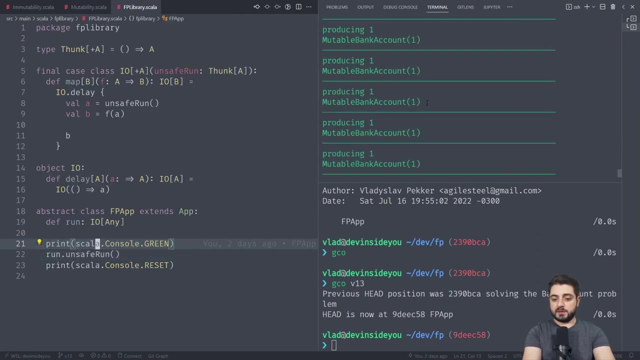 so we're giving this description to the runtime and it calls this one function. right, like our entire application became this one function right over here. this is our entire application and, uh, the runtime simply runs it. i also put uh, some green color around it, like this, okay, and uh, this is why the whole thing uh looks green. okay, but now, like, imagine that. 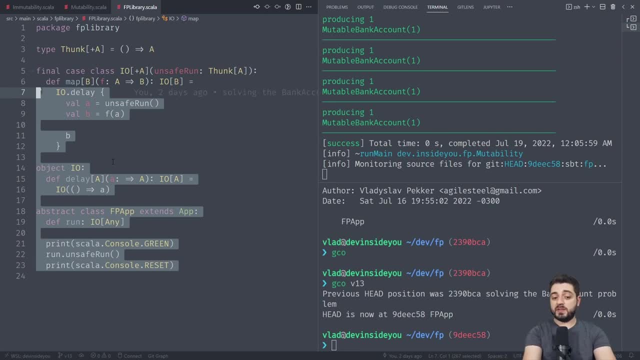 this library is not, you know, it's just another class path, right? we haven't written it okay and therefore our entire program is purely functional. this is what it means to purely function, right? uh, the substitution model is not broken anywhere. we can reason about it in a beautiful way. 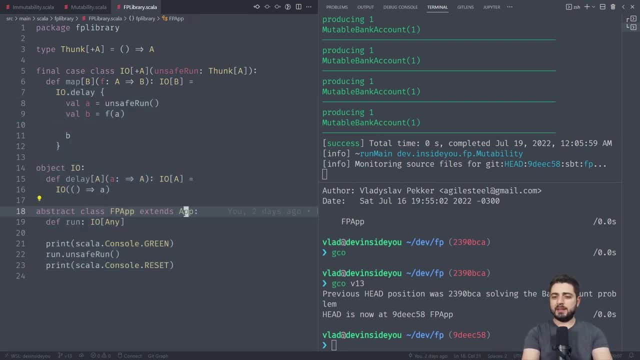 okay, so it doesn't really matter, uh, how exactly this stuff worked, because again there's some mechanical things like app is very useful, but but, as you can see, the etmeco logo is not working okay, so it doesn't really matter, uh, how exactly this stuff worked, because again there's some. mechanical things like app is a very useful thing to replace to run onrolled code. you, that's for sure. okay. so if we try to replace this and just say some scaled effects, if say connect, we can get to maybe cool things that don't work exactly what's all right. the application doesn't work because by definition puts into it. 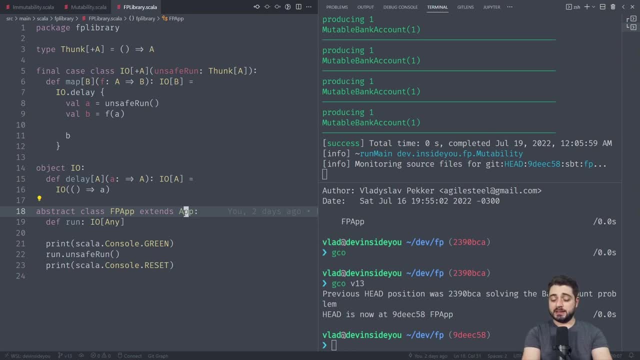 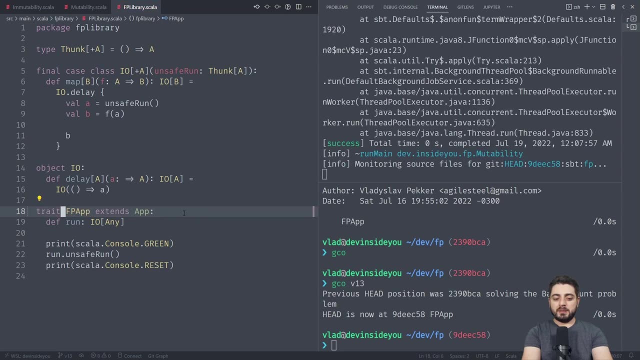 a very special trait, which uses some delayed initialization techniques. um, so it doesn't, it needs to be like an abstract class. if it's a trade, you know, then it's not going to work, you know. but but all of these things are like, just you know, some very specific scholar things. they, they have. 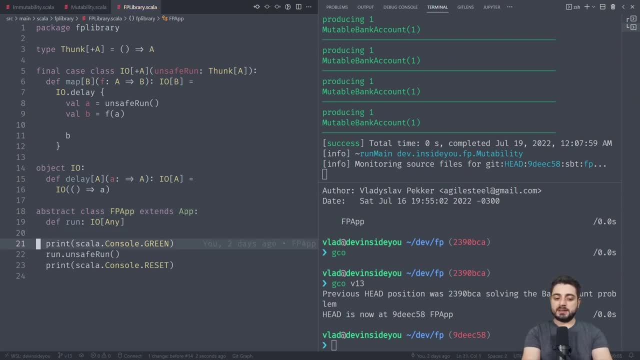 nothing to do with, uh, with what this is all about. right, so just a template. we implement run and it just calls unsafe run. right, so the unsafe code is not in your application, it's in that library, so you don't need to worry about your program. is 100 purely functional, which does not mean that you. 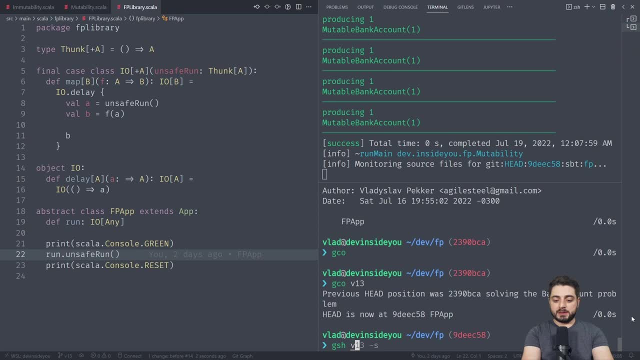 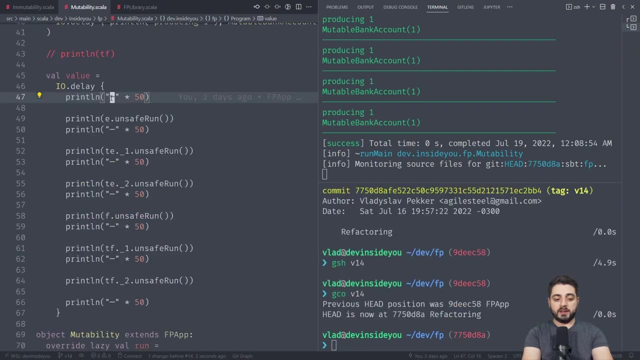 cannot have bugs, right? none of this stuff is bulletproof. let's see what i did next, because i believe, i believe, we're going to start talking about monads. uh, this one is just uh like. usually you would have like a distinction between like your program right and and like this part that. 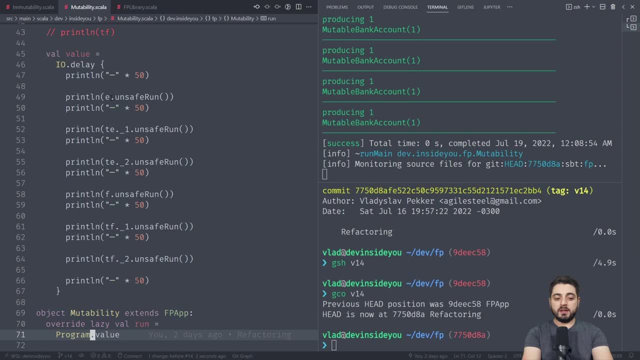 actually does. you know the extents app and you know on the run, okay, so, um, this whole thing now became an object, right, it kind of like ends over here. right, you can do like and program right and like. it has a value, which is our, you know, one single io delay. 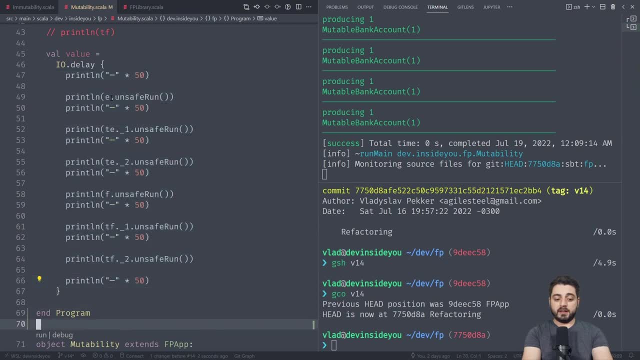 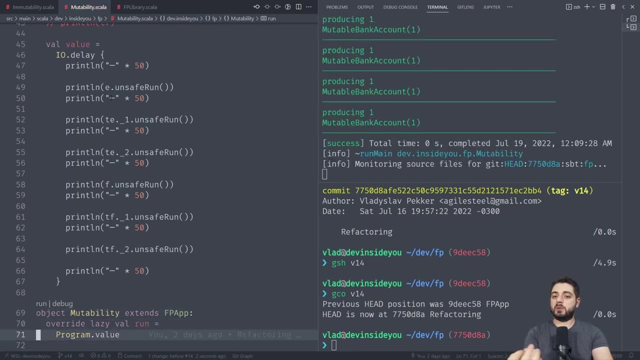 uh was like: this is like basically the our program and uh, you know, we're just doing like this one call over here, like we don't even have this one call what we call unsafe. run the library does it for us okay. but this is pretty much like the pattern, right, so you have like your main is that. 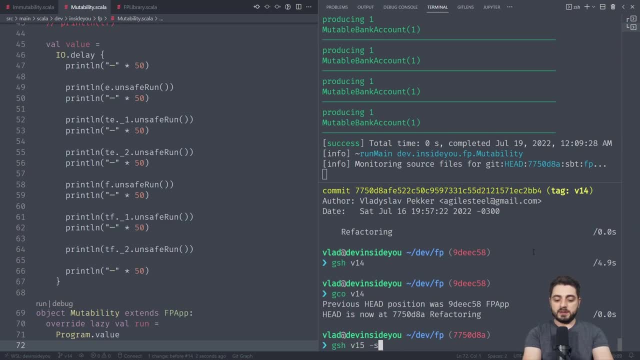 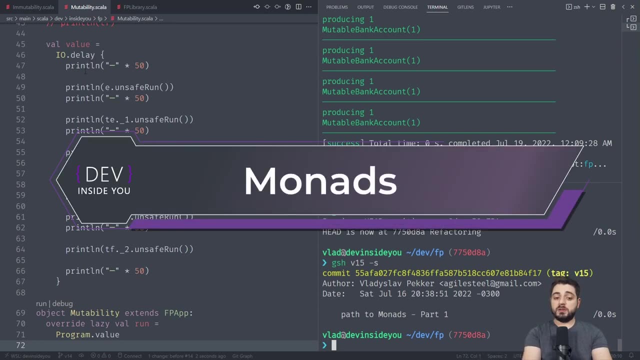 it's gonna look like this: okay, this is just a refactor. okay, so the next one is the path to monads. right, monad's really big word in functional programming. a monad is just a mechanism to chain these descriptions, right? so, the same as before: we couldn't call pipe, we needed map. 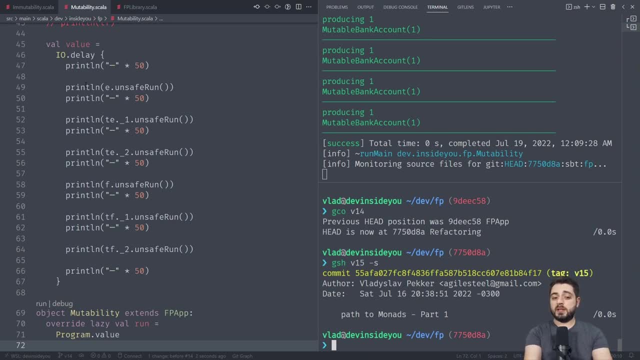 now we're going to realize that map is not enough. we need a slightly bigger boat to compose these. okay, so what? what we don't want is we don't want to have like one io, you know, one description, and then the description to be gigantic. and the second one? 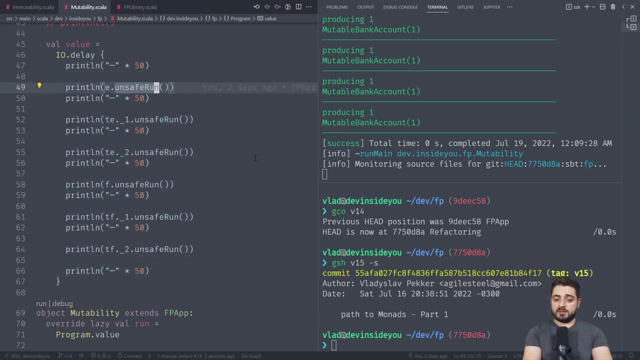 is that. what we don't want is we don't want to call unsafe front okay, even though it's within i, o and an, everything is kind of like fine. we really don't want to have that, because this means that inside, like everything that is marked currently marks, like everything inside of these curly braces. 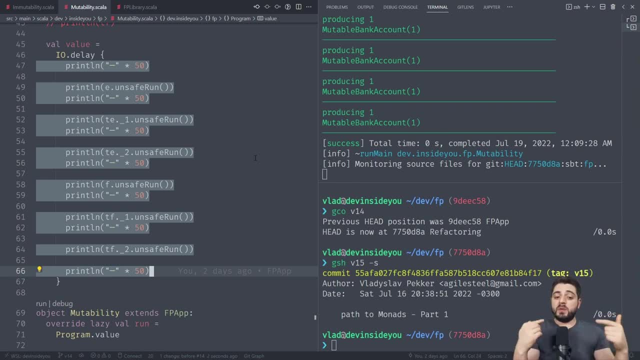 within this, even though tiny piece, we cannot apply the substitution model and we don't want that. in fact, some really advanced cases actually require you to do this. uh, but you know we're not going to do any, any of this stuff over here, okay, so, um, one thing that you always hear about functional. 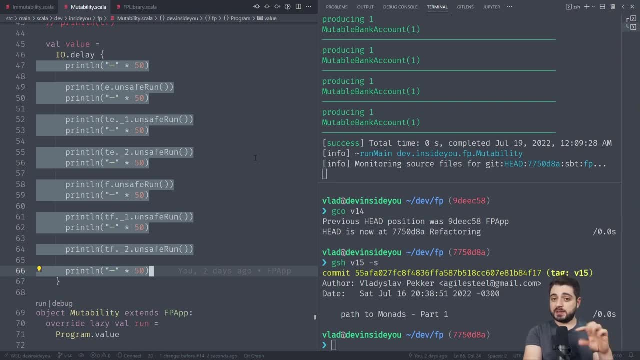 programming is that you can create like very, very small things and then combine them. this is the opposite, right? we have like one very, very big thing. so what we want to have is we want to split these things into many like small ios and find a way how to, um, how to combine them, right? 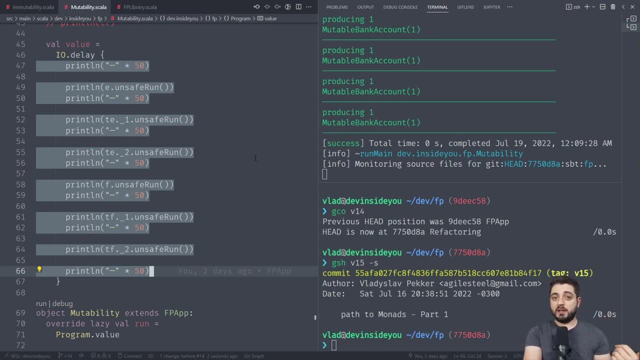 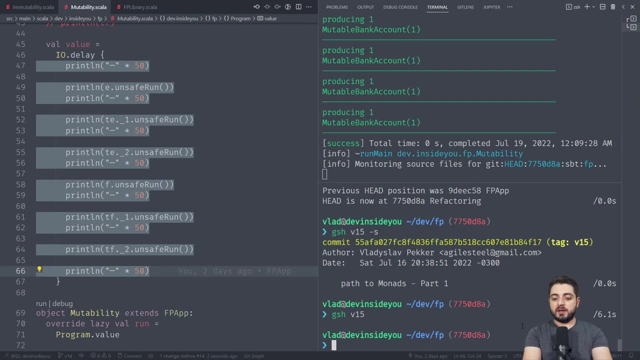 how to chain them, how to compose them. this is like the word that is, uh, you know, usually used. okay, we didn't check out 15, okay, so let me see what i did there. so the first one, like it's pretty much a refactoring right, it's a refactoring to um, to just explain. 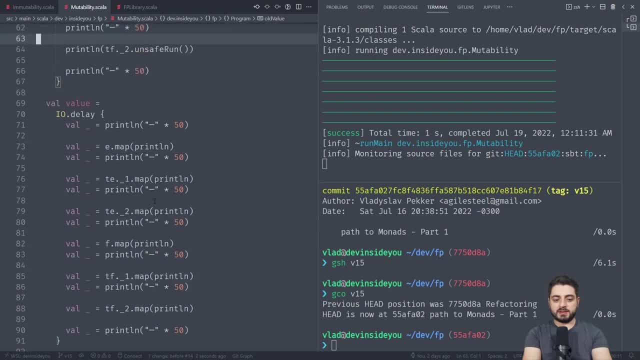 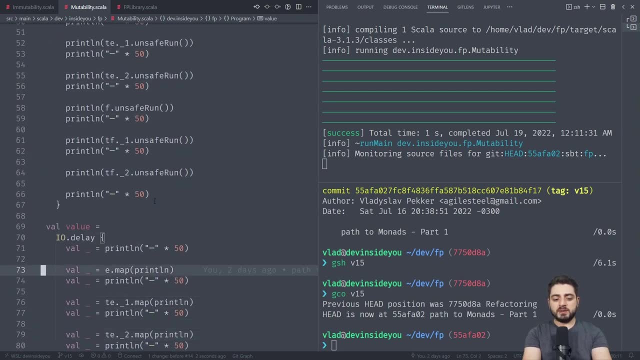 right. so, like, this is like the old value now and this is like the new value. okay, so it's still an io, still delay. it's exactly the same thing as before, right over here, right, um, but now we try to use first of all, we have, like these vowels right, just to remind you that everything has a. 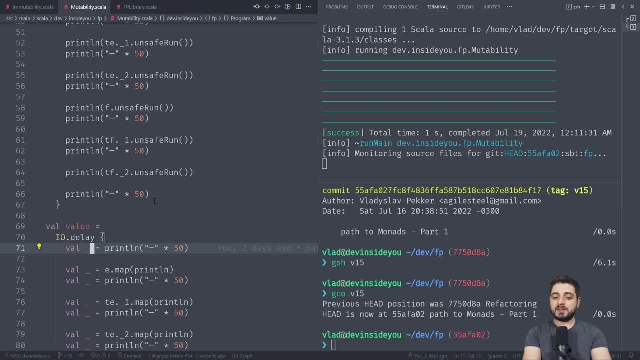 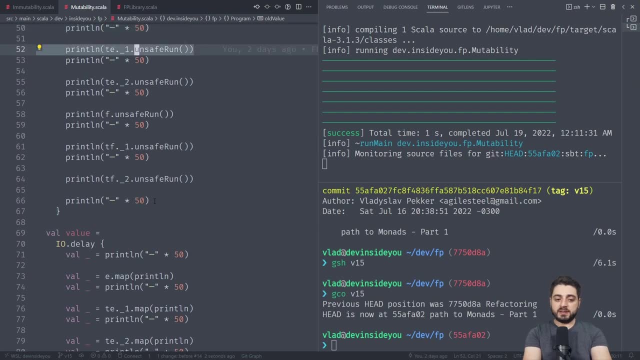 value. and then we try to remove unsafe run- right, and we successfully removed unsafe run. so instead of unsafe run, right. so instead of you know, for example, of this one right like uh print line, and we give it te, which is a tuple of ease, and we're getting the first value out. 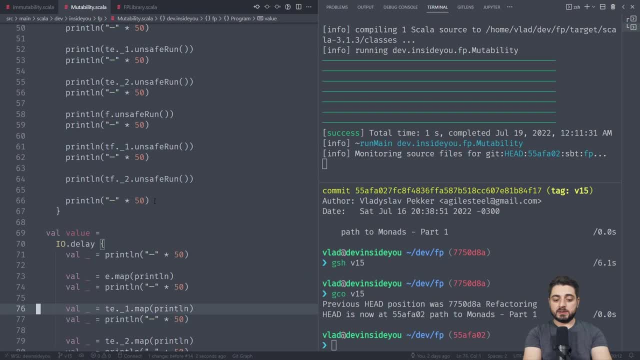 and we're calling unsafe run. instead, what we do is we're getting the first value sort of like pipe, remember, like pipe print line. we know that pipe doesn't work, but we know that we have maps. we try and with map and we successfully removed unsafe run. however, our program does not behave the same. 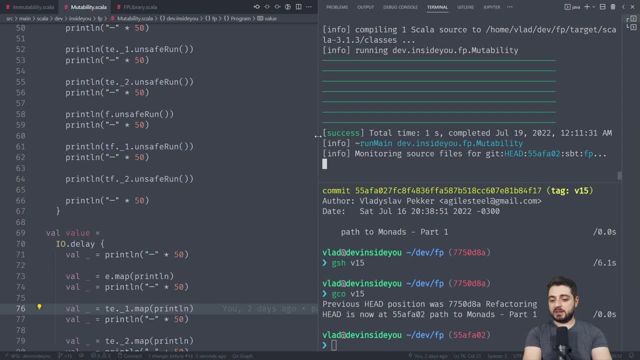 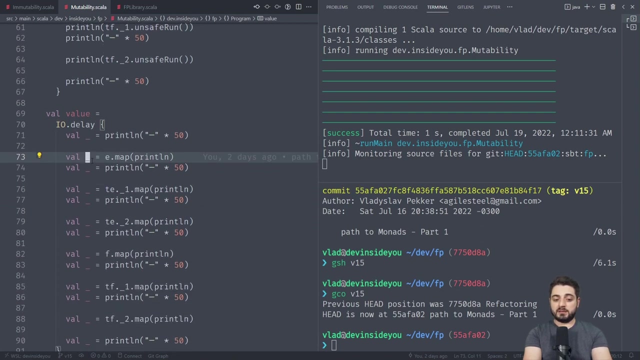 as it was before. so we see that map is somehow not enough. okay, because what is happening over here is that e is some sort of io. right, it's an io mutable account. okay, when you call map, well, you're converting this io into io unit. okay, well, great, now this underscore is io, but you're not doing anything with it, right? so map calls: 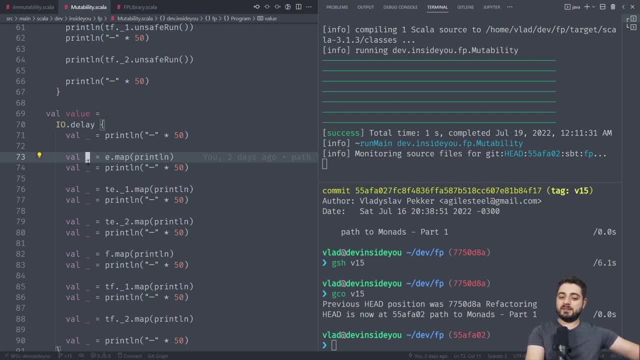 unsafe run, but we need to call unsafe run again, right to, to call this description right. we need to call unsafe run and we need to tell it that after it runs, it also needs to do the next thing, which is like this print line, and then do the same thing with the next one, and then do the same. 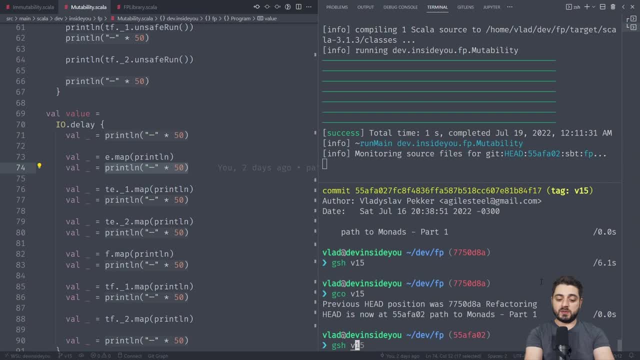 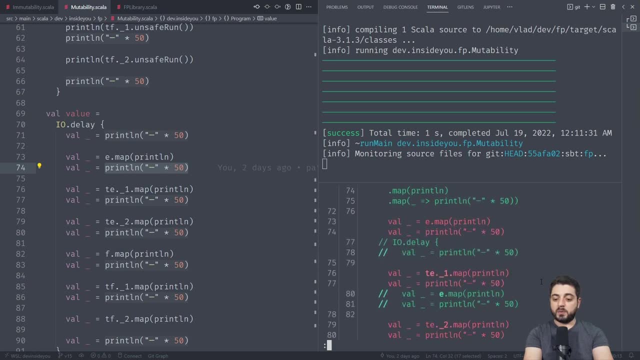 thing with the next one. okay, uh, let me see if we're doing this already in the next one. uh, well, not like this, right, like this. no, okay, we're not okay. so the first thing that we're that, um, that we're doing, is we're going to try to chain them right to, to connect them with map. so i believe. 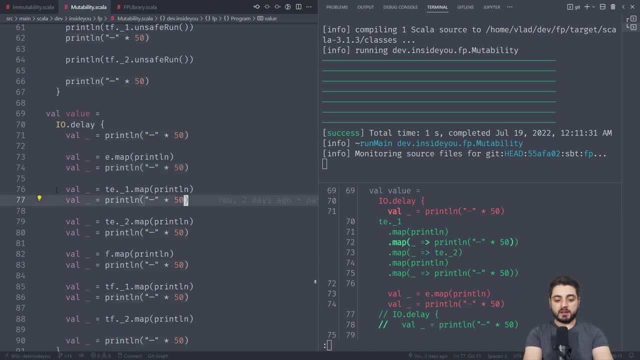 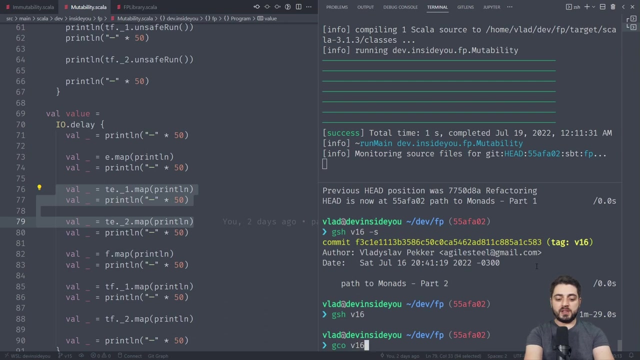 what i did was, um is i tried i took like uh, i believe these three, yeah, so as you can see t1 map print line right- and then i tried to like take these three out. i put them like before here: check it out, okay. so i commented it out and i said, okay, so let's try to use map, let's see if map. 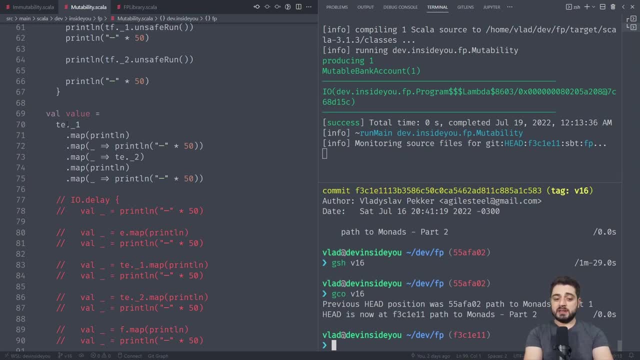 is enough and it looks like like it's: it's almost enough, right? so te1 says: okay, producing one and immutable bank account because of this map print line- great, okay. then we do map print line these underscores: great, this works. but then we do map te2 and here we're lost again, right, because look. 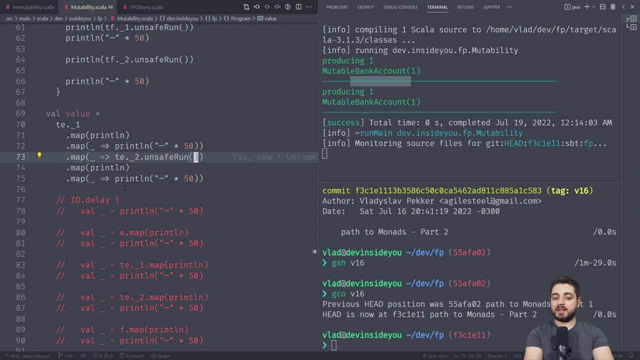 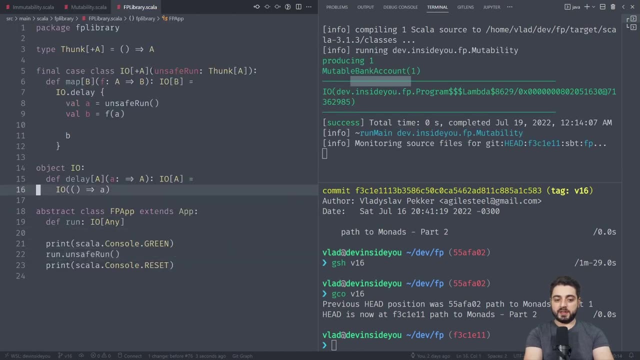 remember, we cannot do this right, like we cannot do this right, we're not allowed to call unsafe run, okay. so, and then we're kind of lost. we're, we're in this, we're in this description world again. right, so we're like over here again. override easy valve to string, which is a string equals. 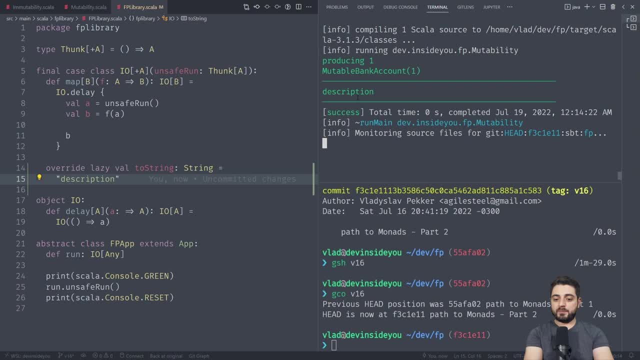 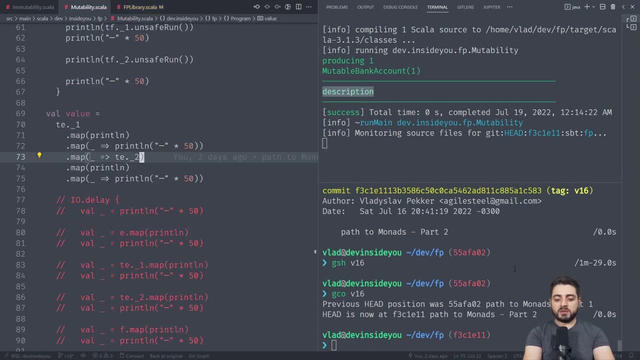 description right. so we need to call like unsafe run again. like this is a trick, we need to call unsafe run twice somehow. okay, i'm pretty sure that the the next one, you know. uh, the version 17 is just to explain the add expansion of here. so this print line is basically okay, the bank account comes in and we do a print line. 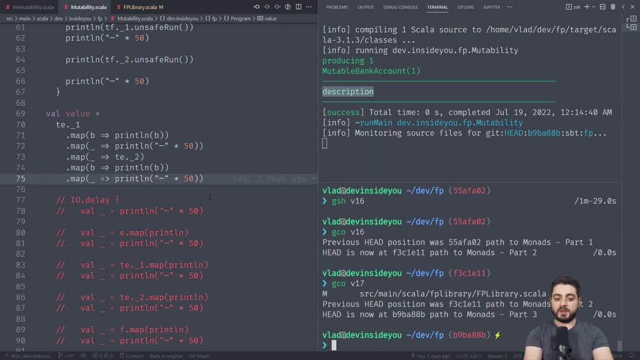 of the bank account, right. so, as you can see, they're all the same. okay now, but they're not all the same right because, like, print line is something that is already happening, right, it gives you like a unit, right, but over here, like this is an iof unit, right, and so we need to continue. 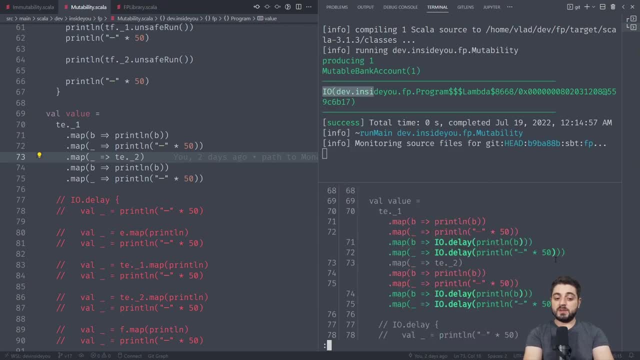 right, let's see the version 18. so the first one is: okay, let's, let's, let's level the plane field, let's make them all equal. okay, so we can't make them all like we can either go like down, right, so we can call like unsafe run, okay, now they're all like sort of like executed right. print lines is: 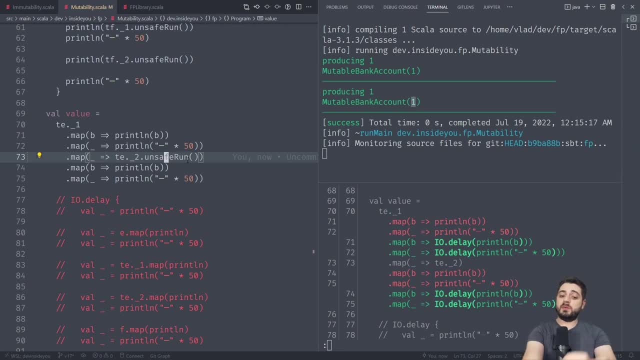 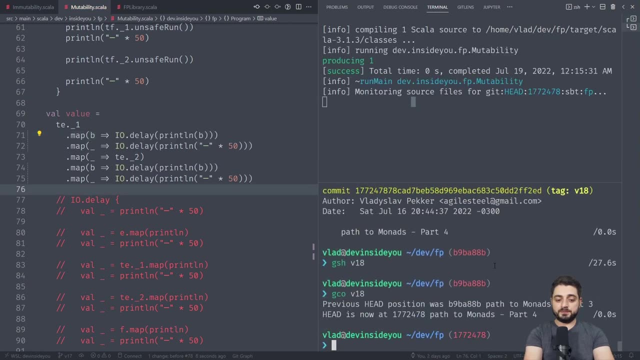 executed. unsafe run is executed. okay, but we actually want to go the other way around. okay, we actually want to want to delay the print lines. okay. so we check out 18, we're going to delay the print lines, okay, and now all we need to do is we need to create: 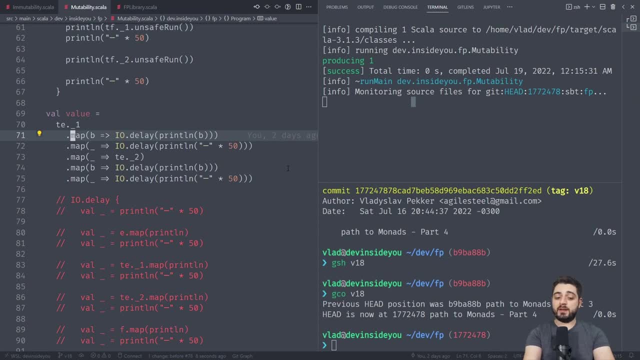 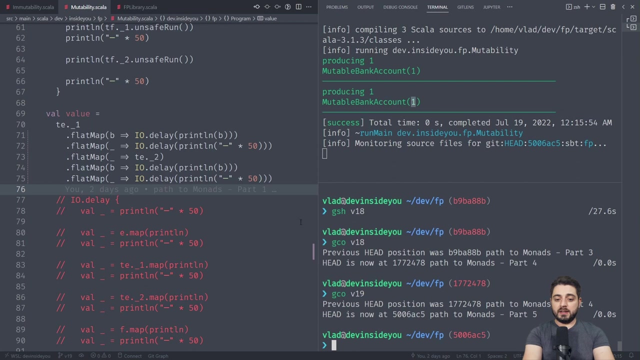 an iof, iof, so we need a map. but that will then flatten the ios, right? how will it do? well, it will call unsafe run again, right. so if we go to v19- right, you're going to see that we're calling flat map now, right. so everything is i o here, right, and flat map does exactly what we need. 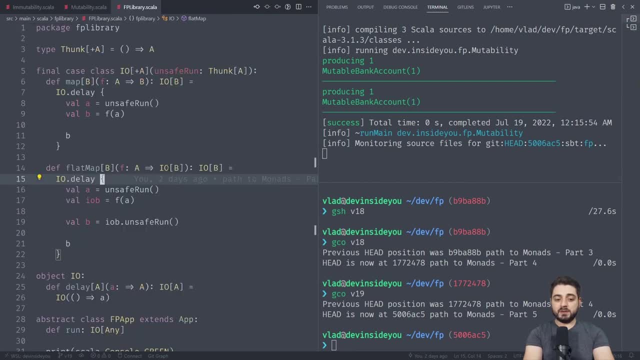 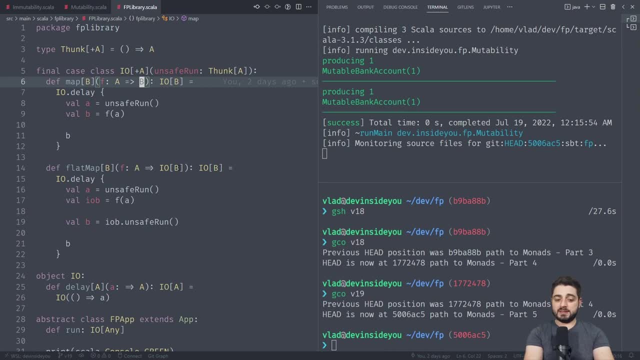 before it was a, b, which in our case was like unit most of the time, but now this is an io, and implementation is almost the same right. so first we're getting the a out, but then when we call the function, we don't get the b, we get the io of b, and so we call unsafe run again. and this is how. 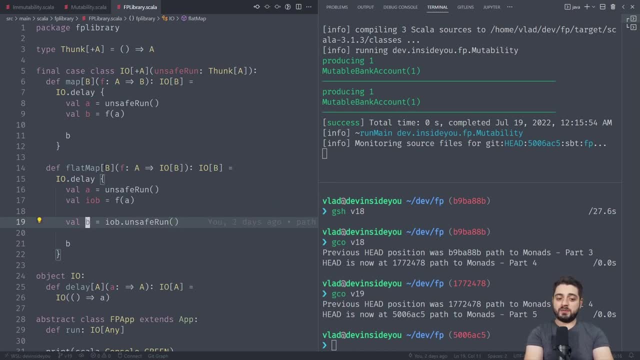 we get our b okay, and so again, we went from iof a to iof b, but this time was a different function and you know, a hand wavy way to explain monads is that monads is like that thing that has a flatten up pedantically. there are also laws that can be updated in the future, so we're going to 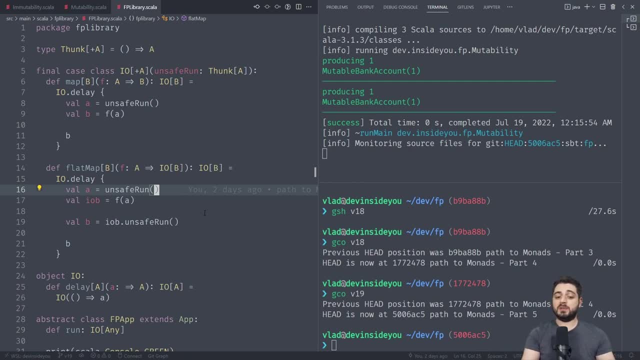 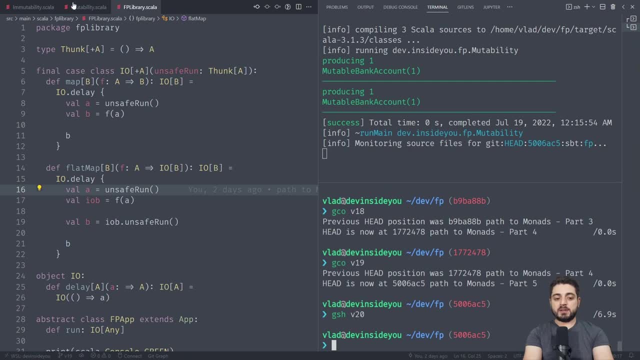 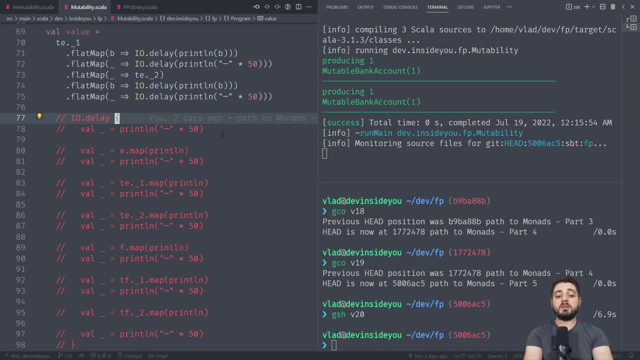 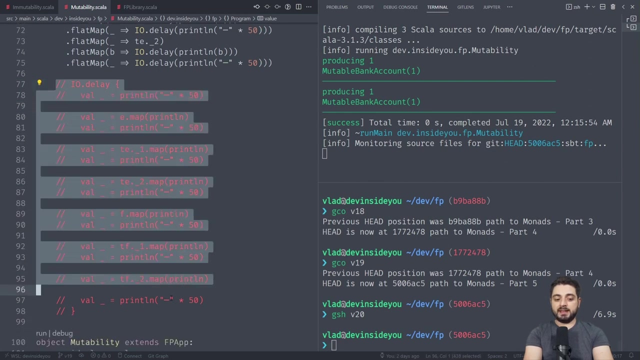 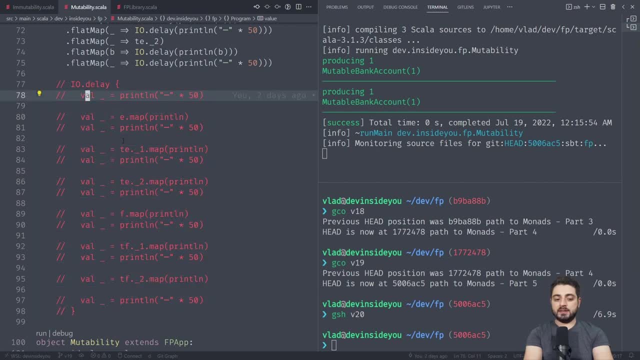 almost, as is okay, it's just that these valves will go away. these equal signs are going to look like this: okay, and over here, remember, this is going to be like delay print line, right, and this thing over here, right, it's going to have a four in scholar two that will be also in curly brace. 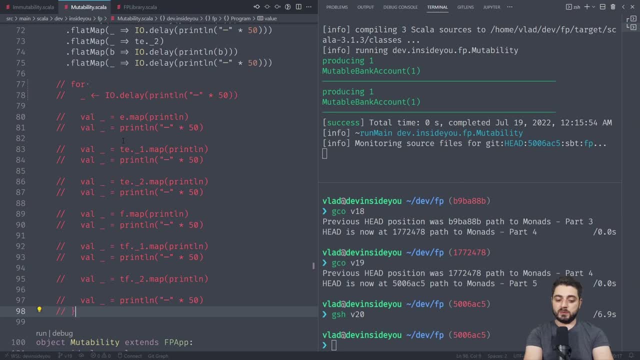 in scholar, in scholar three it's not required, and over here in scholar two, it will be closing curly brace and then yield. in our case, when we're yielding is a unit right, because this was an unit. okay, it's called three. we don't need this curly brace, okay? so i'm going to do throw, throw out what i. 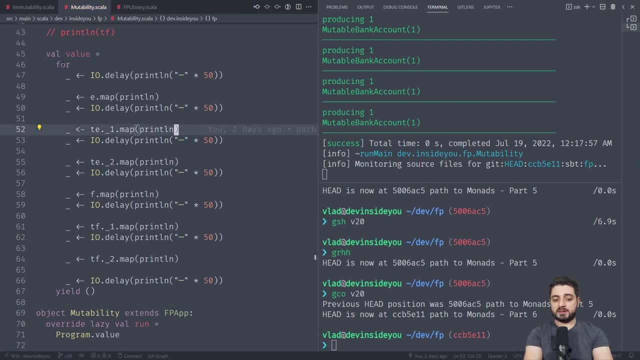 just did and check out v v20, and that's exactly what i just explained. okay, so instead of like doing it yourself- flat map, flat map, flat map- you have this four comprehension. technically it's not like precisely the same, because these are nested flat maps. what we had before was like chained flat. 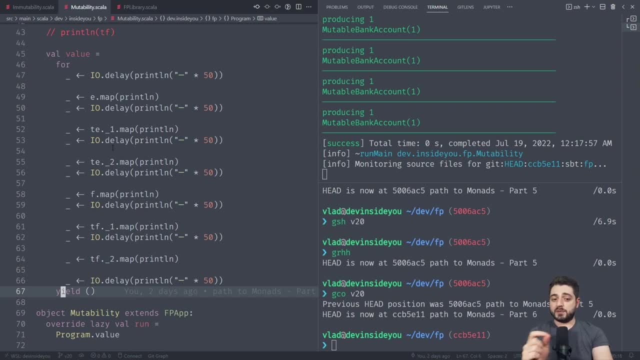 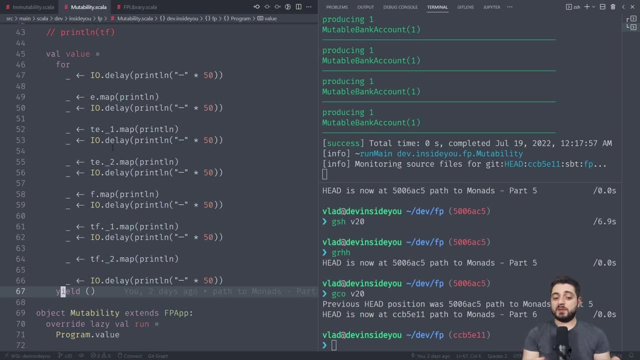 or you're not chained or you're not chained, or whether you test things or whether you chain things, it should behave exactly the same. that's also why it's very important to test laws when you create your own instances of monads, but usually you don't do this, because usually the 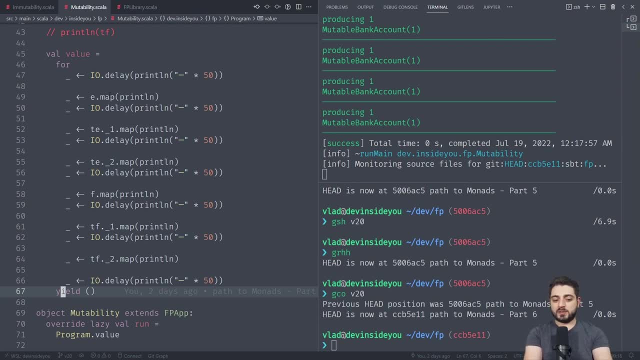 libraries do this for you. okay. now there's some, there's still some discrepancy right. we still have like a map over here. remember, we didn't, we didn't remove it, but as you can see, as you can see, it already works okay. so i believe the next steps are going to be to do, you know, flat map and then 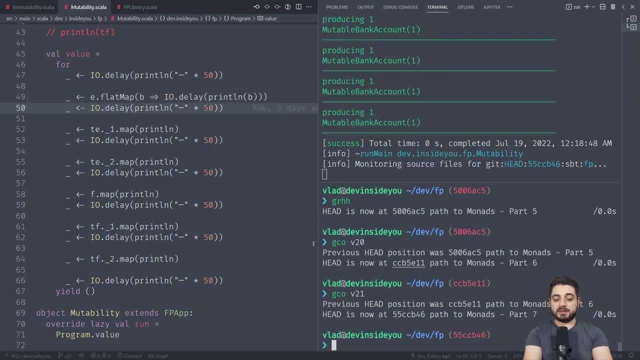 delay the print line, and so on. let me just check out v21. yeah, so this is like the next step right into flat map, and then we're going to have a b arrow to the right- io delay print line b, okay- and the next one is going to be: um, an introduction of our own console that is going to do this whole. 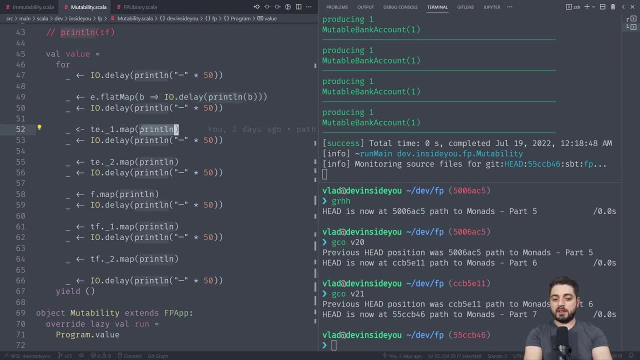 delaying for us because we want to, we want to do is we want to have at expansion. right, we want to. what we want to have is we want to have flat map and then our own. you know, i believe i call it fp console dot print line, because over here we cannot, we cannot use that expansion. the next one is going: 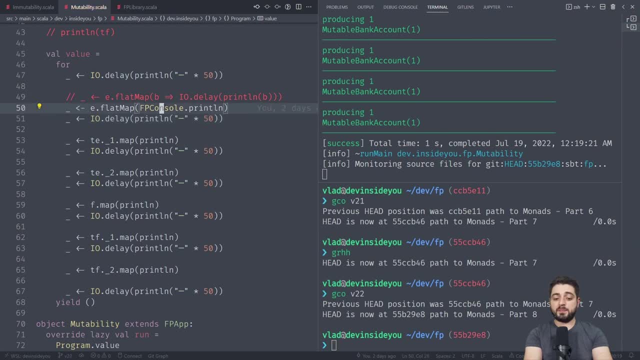 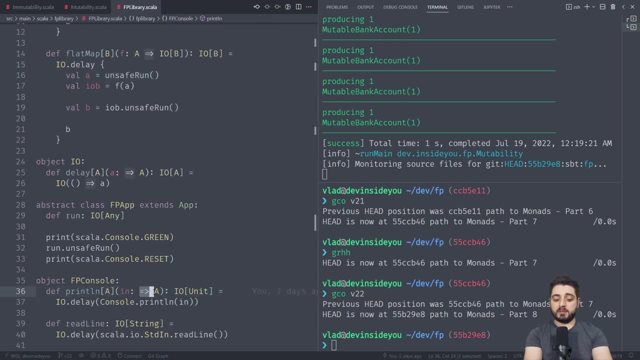 to be 22, right, which has this. yeah, it's pretty much exactly what i said. and fp console is just a teeny tiny object. it has print line and read line. okay, print line has a delayed- you know by name- parameter a, and all it does is io delay the regular print line. so this is. 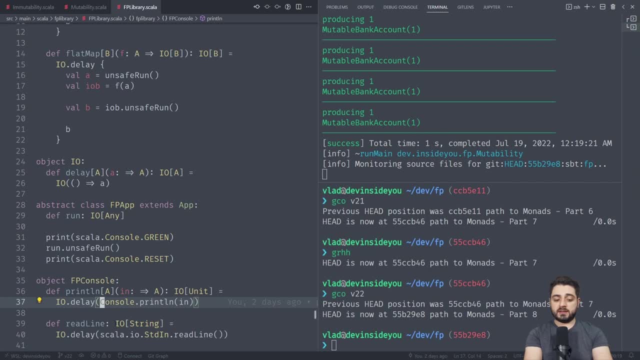 the regular scholar. this is the print line that we have been doing all along. it's just that, uh, i cannot do it like this because otherwise it would like to refer to itself, so i need to do a console dot print line, and the read line is pretty much exactly the same. it's like the opposite, it just 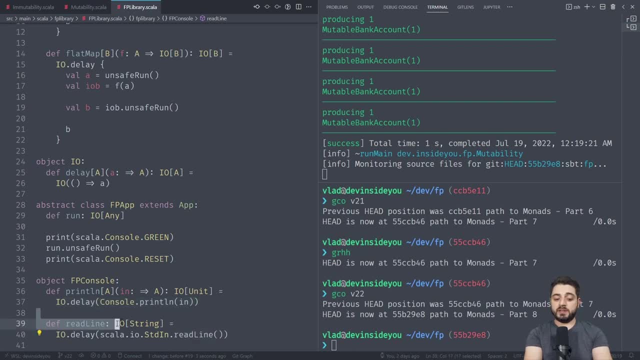 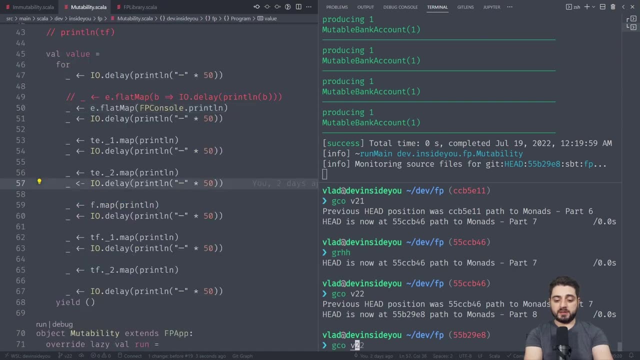 delays. you know the read line from the standard library. therefore, it gives you an io of string and there we go, okay, and the next one pretty much like rewrites. you know the rest and it also shows you that, because we're dealing with descriptions, we can store a description in a. 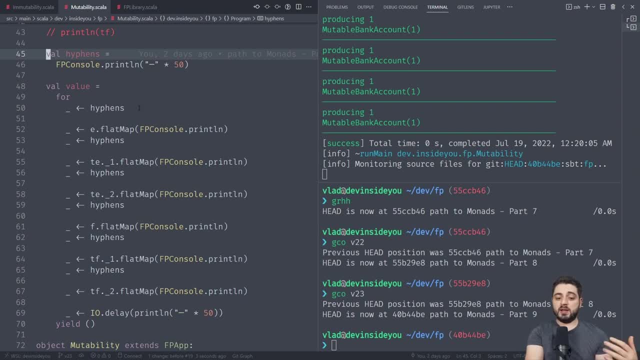 val. you know, with these hyphens and we have this full comprehension, which is okay, we'll do hyphens first, you know. then take a bank account flat map to print line and do the hyphens, now do the blah, blah, blah. but now we also have like flat map inside of a full comprehension, so we don't really 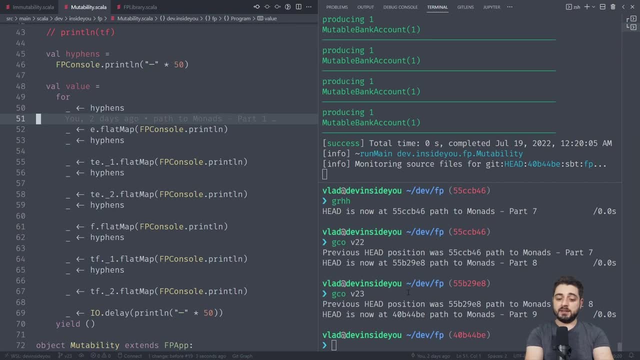 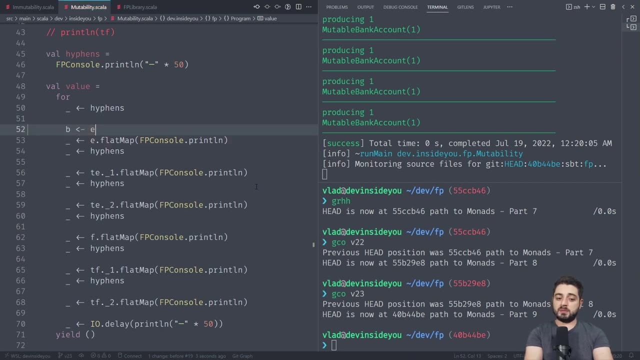 need this right. so i'm going to rewrite one of them, uh, by hand, and then i'm going to check out the next commit and it's going to do this. so basically we could say: okay, we'll get the bank account from the, from the e, which is a. 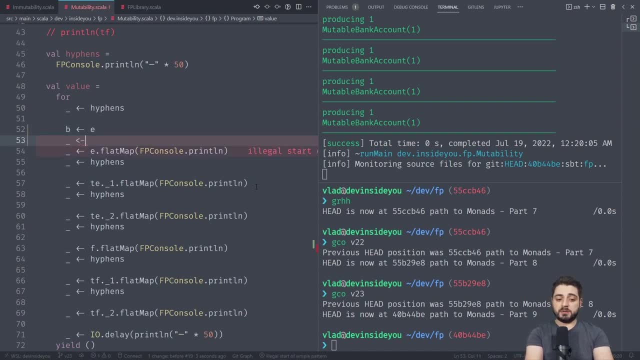 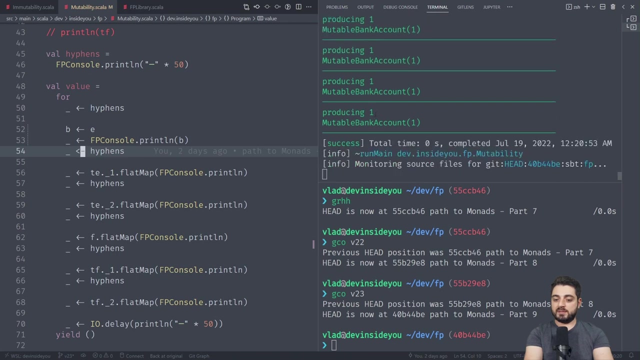 description of how to get a bank account, okay, and in the next step, just do fb console, print line b. okay, because like this thing essentially is a flat map, right? so it's going to look like this. it's literally the same code, as you can see. behaves exactly the same, okay. so let me do this. 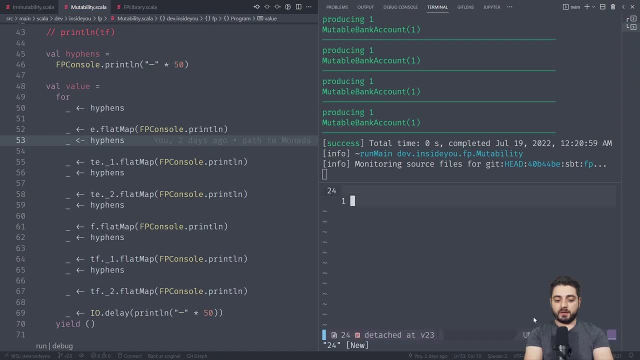 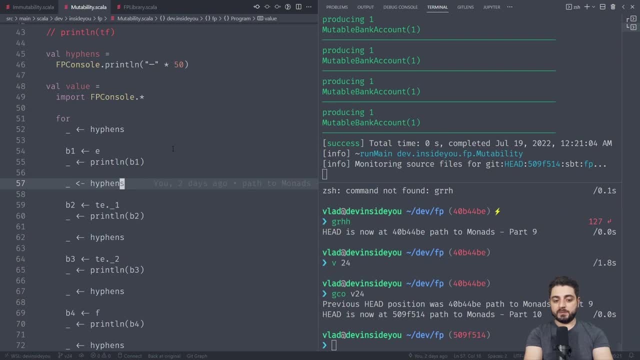 okay, so, let me do this. okay, so, let me do this. i'm in checkout v24. i'm in checkout v24. i'm in checkout v24. there you go. this is exactly what i just there you go. this is exactly what i. just there you go. this is exactly what i just said. okay, get the first bank account. 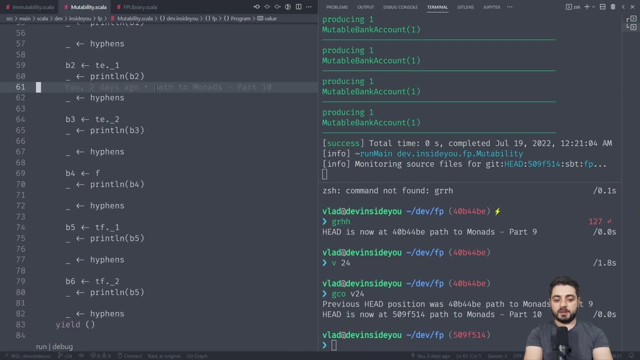 said: okay, get the first bank account. said: okay, get the first bank account printed out. get the second bank account printed out. get the second bank account printed out. get the second bank account printed out. okay, printed out, okay, printed out. okay. right, it's exactly the same program, right. 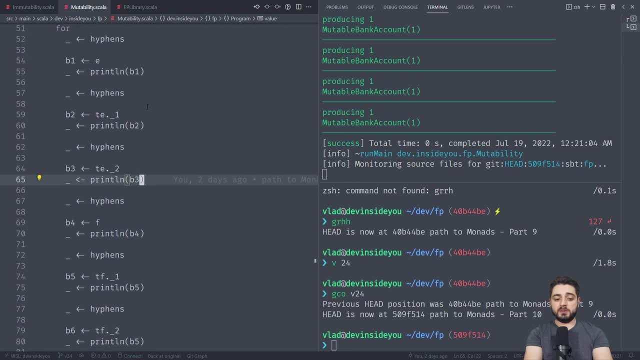 right, it's exactly the same program, right. right, it's exactly the same program, right. so this is like a huge full comprehension. so this is like a huge full comprehension. so this is like a huge full comprehension. and, by the way, when you're, when you're, please do this. okay, let me see the next one. so, basically, we're going to, instead of having this, 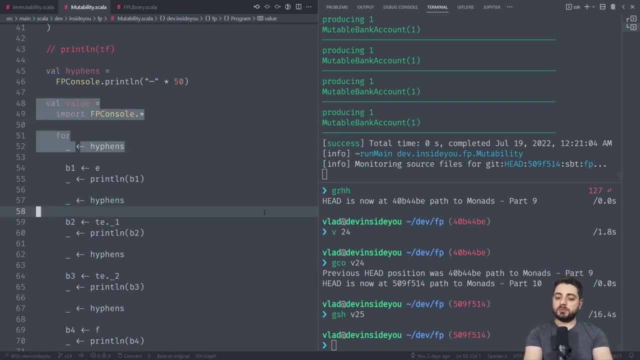 program that does like all of these things. we're going to go back to the original program that we have written. remember the one that starts with a bank account like adds 20, uh, uh, withdrawals like five, i believe. right, it just says written in this functional style: okay, and this is for. 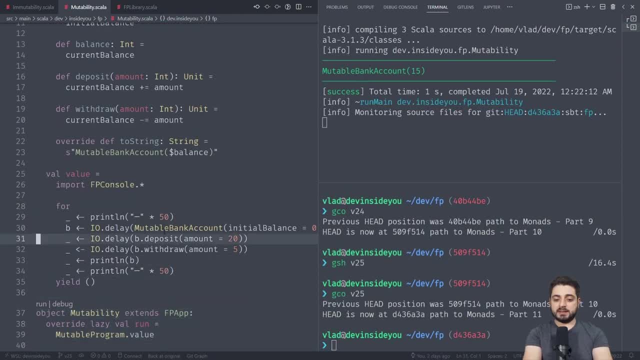 the immutable and for the immutable one. okay, so now, like now, like this is our program? okay and, as you can see, like at the end of the day, this program looks pretty much the same as it as it always looked, like it just said. now it's inside of the full comprehension, okay, so if we 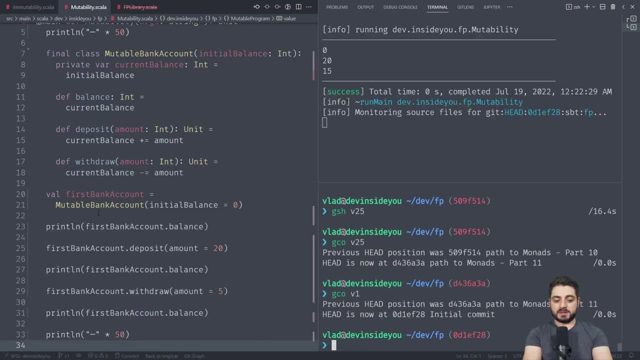 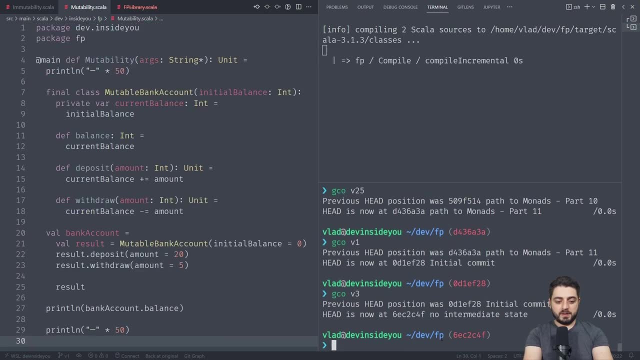 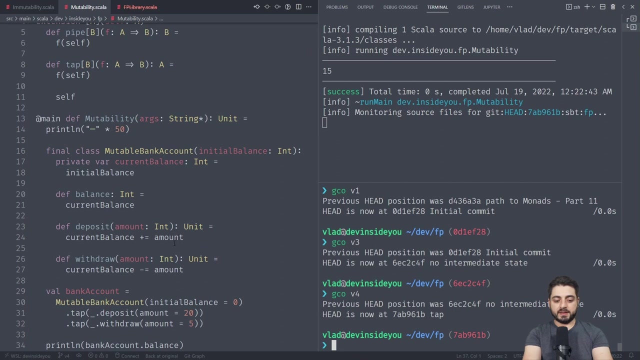 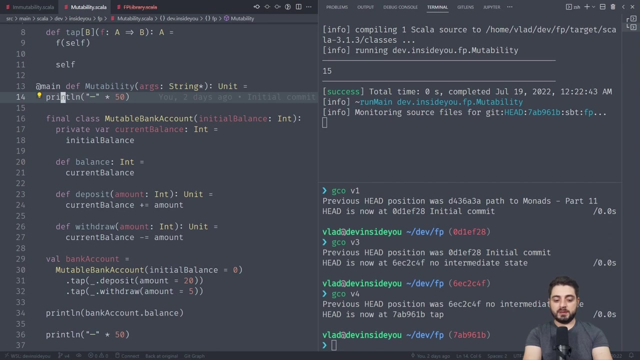 go to like check out v1 as you can see it was well, maybe not v1, hold on um, maybe like um, v3, maybe v4, yeah, like this one. see, it was like print stuff out, create this back out. you know bank account was like zero and then deposit 20, withdraw. withdraw. 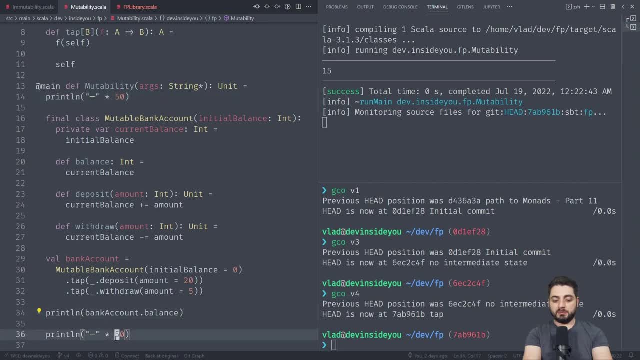 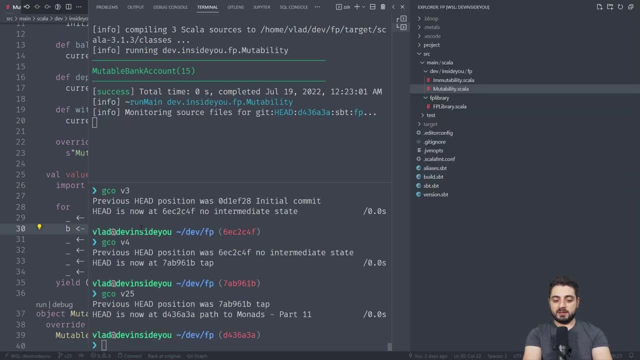 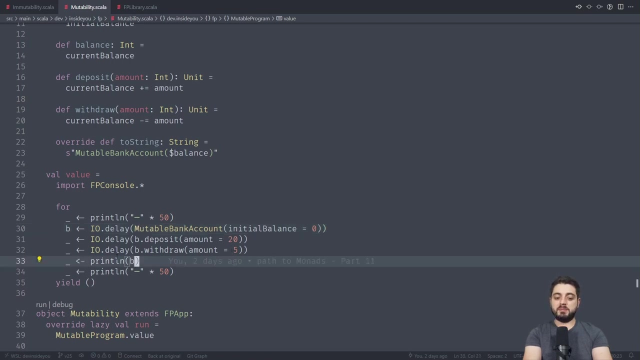 five and then another, another print, you know, print out the balance and print line 50.. okay, so this is. this is now how it looks like in a functional world. okay, print line 50: create the the um, uh, create the immutable account. it was, it was zero deposit. 20, withdraw five. print line the. 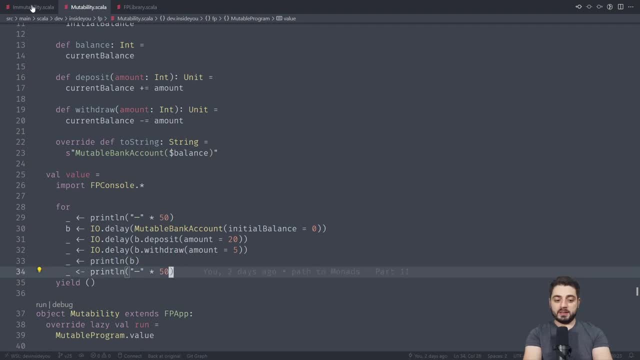 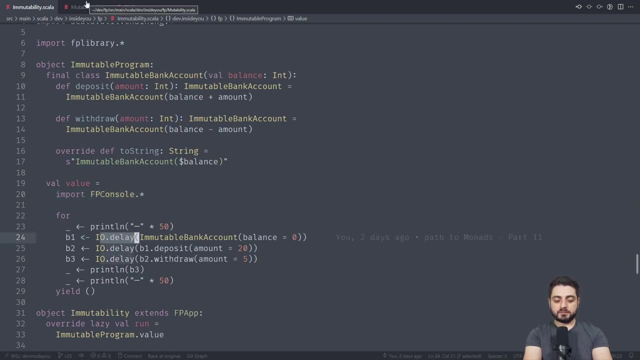 balance, you know. and then the print line: okay, and in an immutable world looks exactly the same. it just said over here: don't even need to do these delays because everything is immutable anyway. okay, so inside of the full comprehension, you can also do equal sign like this and go like, go like that, okay. 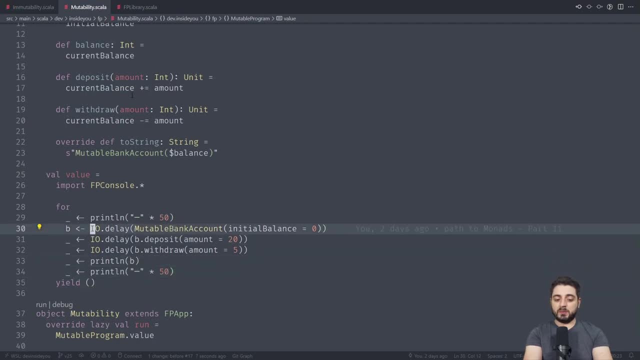 like this. now, in immutable world, you could do the same thing and you would actually not, not like most of the times you will not break anything. but there's a super subtle difference and for, like you know, 100 purity sake you should not do this, and i'm going to show you why. um, a couple of 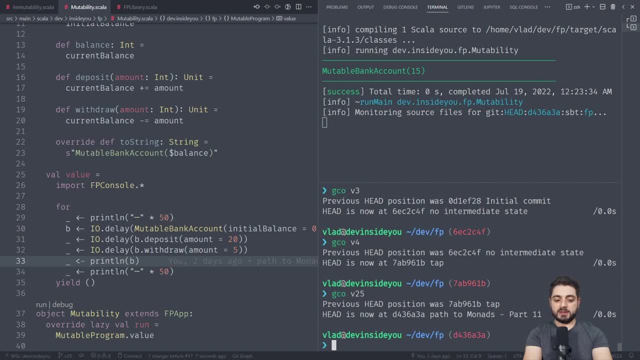 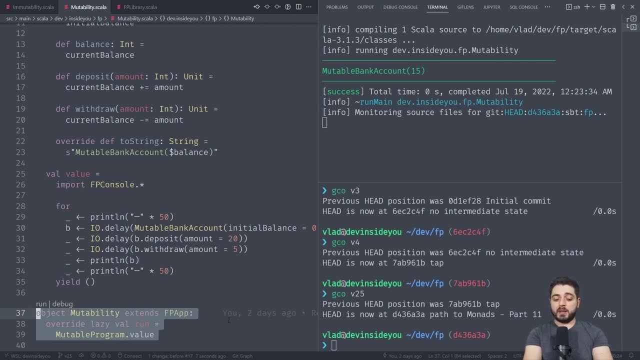 maybe even in the next one. so what the next one uh shows you is that, uh, we're going to remove this thing and we're going to run our program still ourselves, right by calling like unsafe run. and what we're going to do is we're going to show that over here we're calculating the description, right. 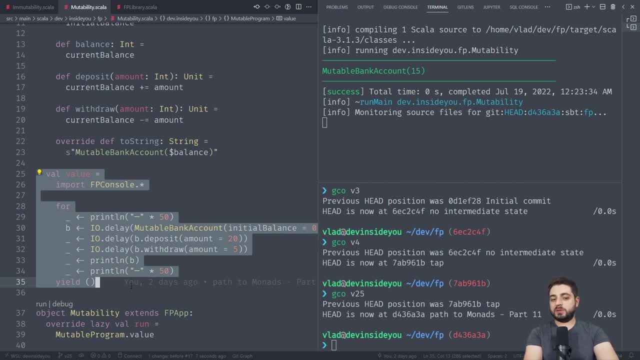 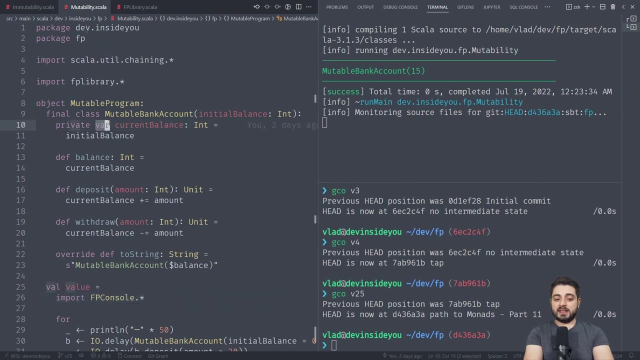 we're always calculating the description during the calculation. we should not initialize any mutable state. okay, we should also not mutate anything during the initialization. okay, so over here, when this class has been created, uh, there is some mutable state that has been created. this current balance is a bar, okay, so if you were to put a print line somewhere over here, 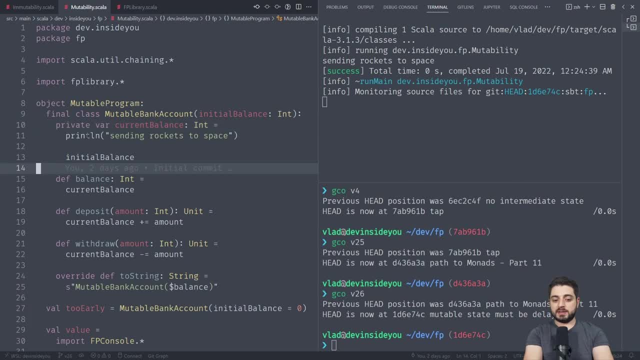 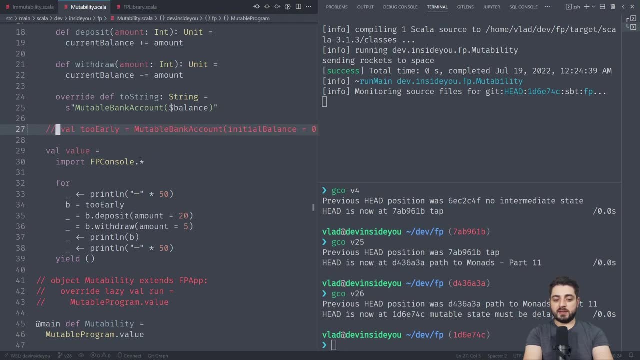 okay, let me check out v26. okay, so this: it puts a print line over there. okay, and now this demonstrates the substitution again. okay, so i'm going to comment this out, i'm going to uh ying until the end. okay, and i'm going to put it like: see, as you can see, like there's no delay here anymore, there's. 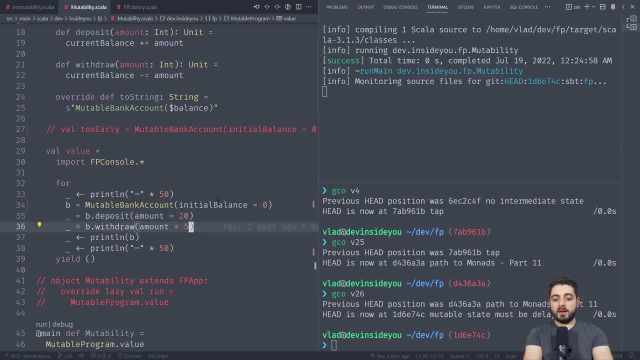 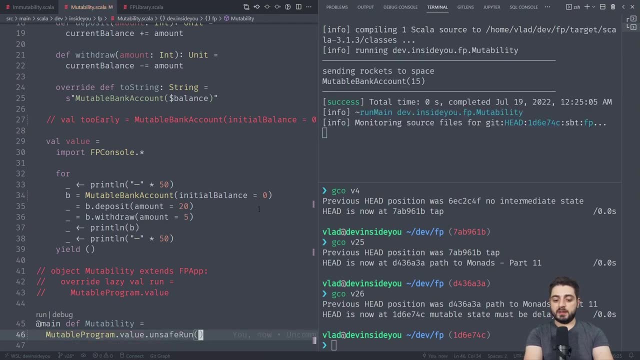 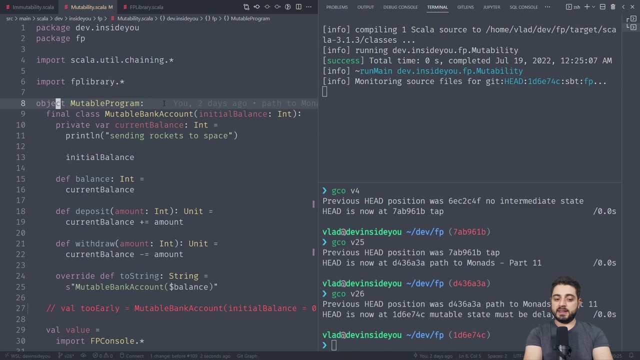 only like equal signs, okay. so if you have this program right, notice that over here we're not running it okay. so if we do like unsafe run now, we're running it okay, but we're not running it right. we're just saying okay, just like give me the description. the thing is that, like uh, objects in scholar are uh lazy. 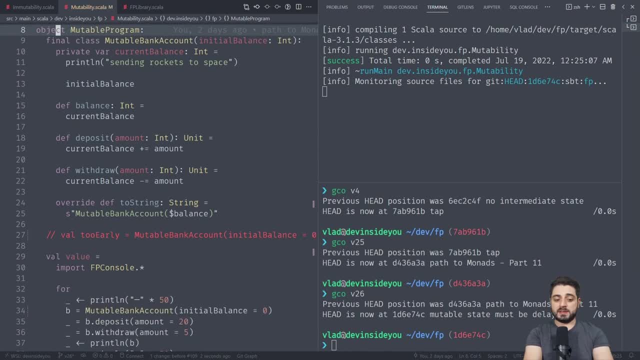 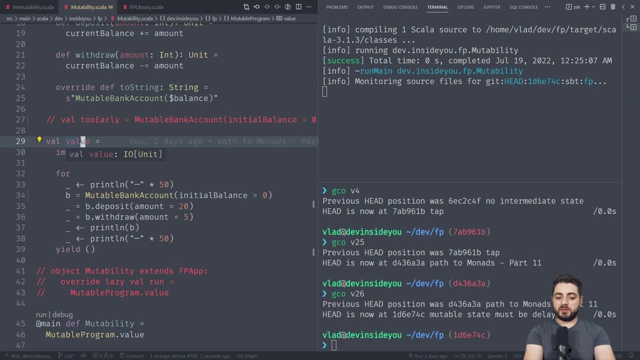 which means that as long as, like, you don't touch them, like, even though this is a val, it's not going to be evaluated. this is exactly why i'm accessing it. i'm forcing the evaluation, okay, but this is just the description, right, like this is just io- of units, so nothing should happen. 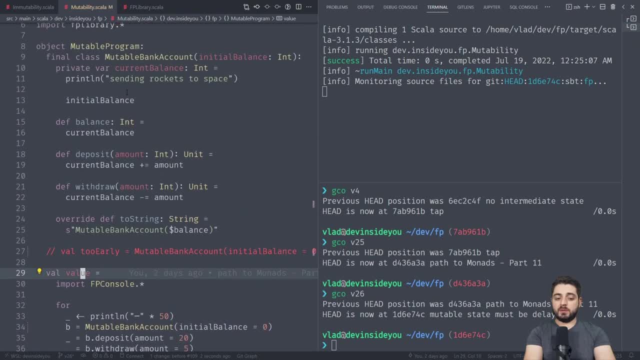 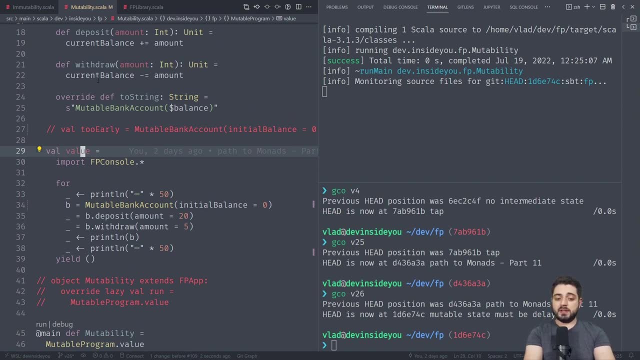 however, if you are not careful with the mutable state, even though you have io, you're going to run into issues, right? because, again, this is a substitution model, right? so imagine that there is this val and instead of using it over here, right, like this, right, if you do it like this, 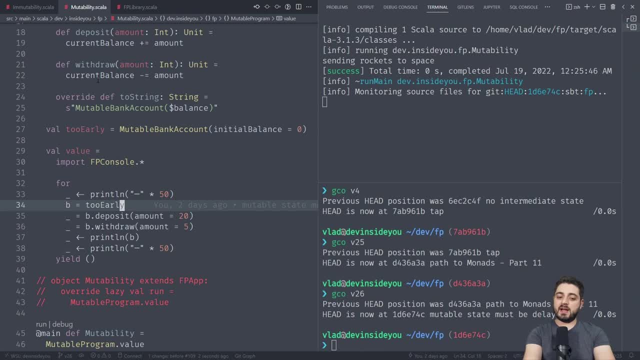 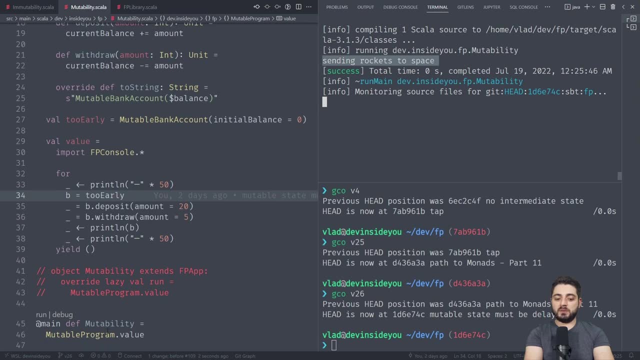 right? so sort of like the opposite of substitution, right? so instead of using the value, we're actually using the, the reference. right? so now, as you can see, we're sending rockets to space, even though when we haven't, we didn't even run the program yet. it just said during the 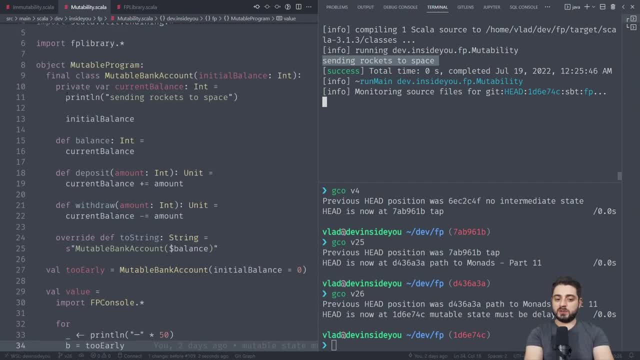 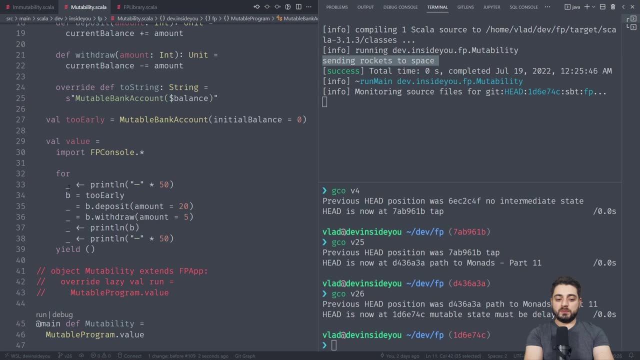 creation of the description. we accidentally send rockets to space. okay, like this. okay, so be careful. right, like avoid mutable state like a plague. so the next one is going to be: like let's forget about bank accounts, let's, let's do a functional programming hello world. okay, get checkout 27 and I believe it's. 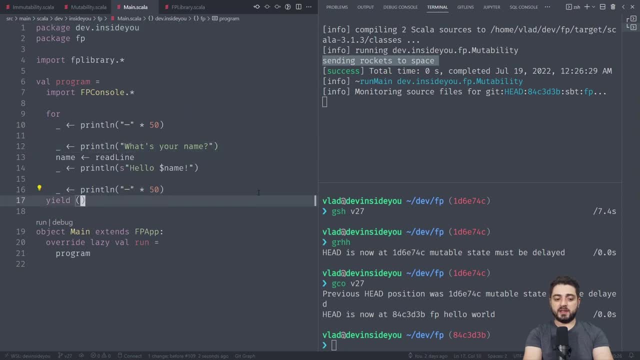 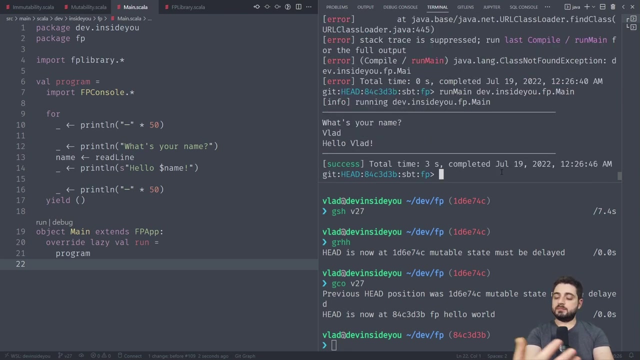 actually in a different file. so this is the functional programming hello world. okay, so it we need to switch to running it. we're going to run it only once, right, like, like this me, okay. so it just says: okay, what's your name? my name is Vlad hello black. okay, so this is the functional programming hello world. this. 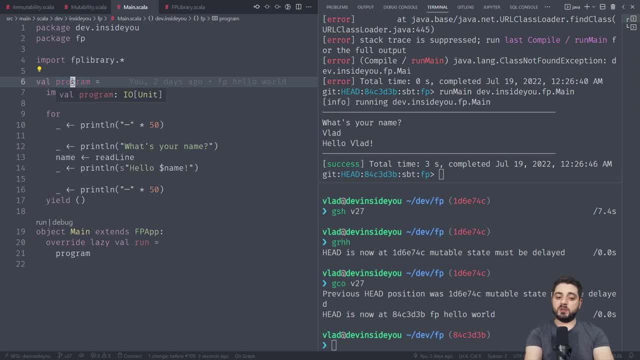 is how it looks like. first we're calculating the description right, so this is the IO of unit by using, for comprehension, print line, print line, read line, print line, and then we're giving this program to run. okay, this is a functional programming. hello world. now I believe the next one requires a lot of explanation. so this is: 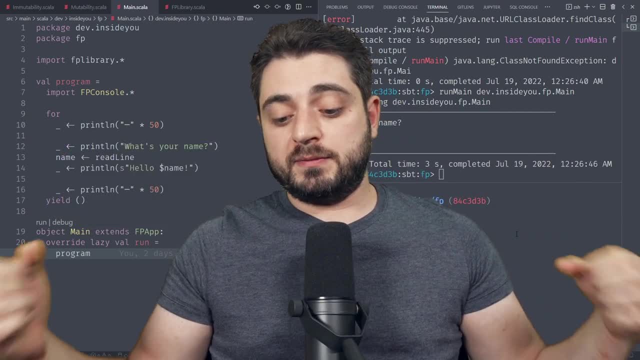 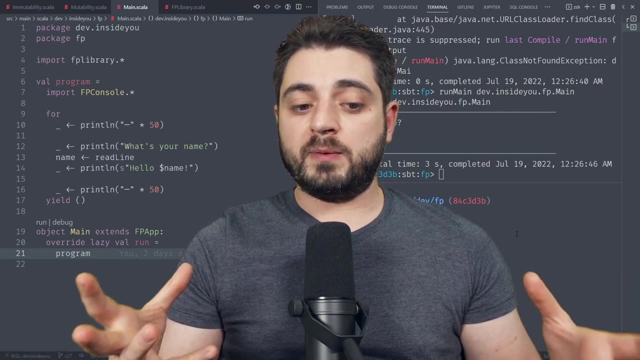 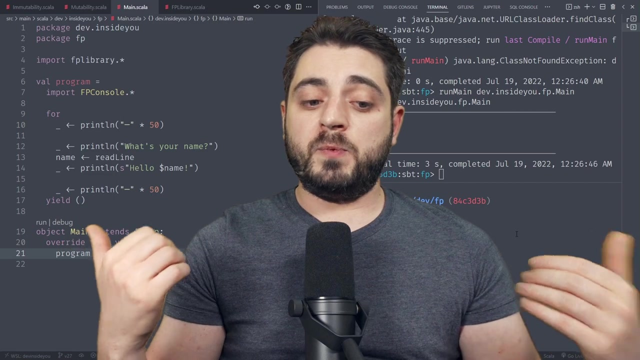 the path to tagless file. there's a technique called tagless final. originally, it was created to solve the so-called expression problem. right, it was basically: how can we add behavior or add new data types to our program without recompiling the existing ones? okay, this was the premise of the expression. 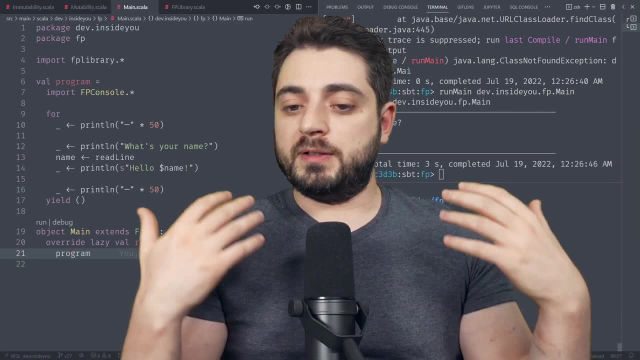 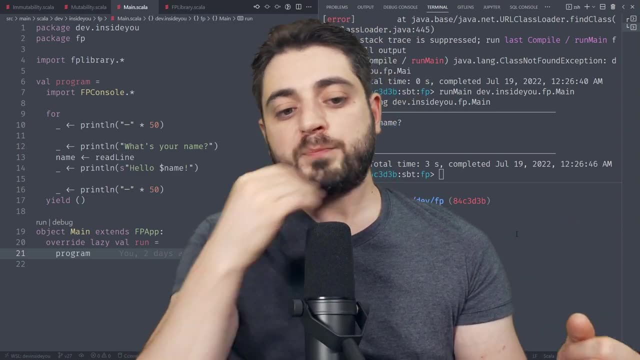 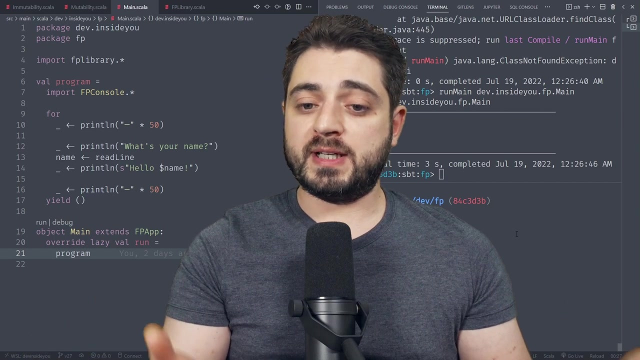 problem. it's called the expression problem, because the original example was um, a data structure which represented like mathematical expressions, you know, like adding two things together, subtracting things together. and so now in the scalar world, we, we, really we really adopted this um, uh, pattern, uh, it's called tagless. 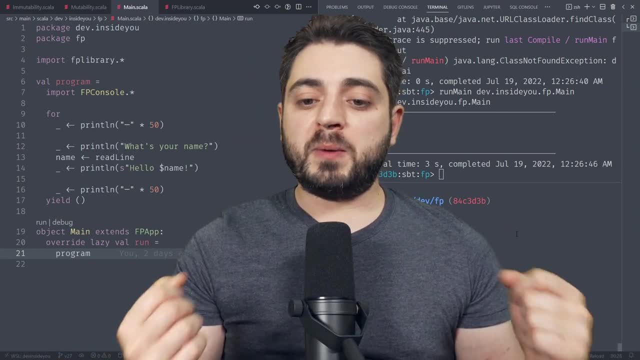 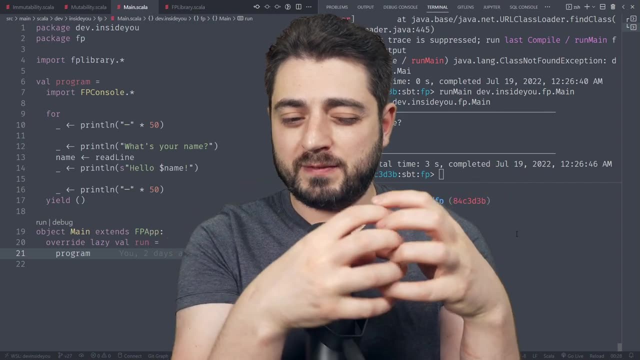 final. i have an entire playlist about it. you might want to check it out. however, we applied it to a very, very, very small problem. um, well it was, it was big for us, but we applied it to like a very, very narrow problem. okay, we did not care about the solution to the expression problem. 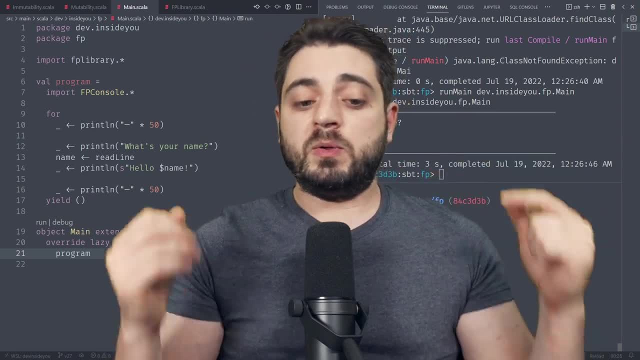 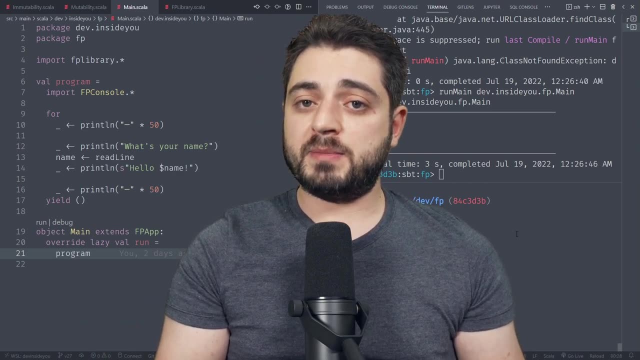 well, kind of did. right, it's all related, okay, so i already mentioned this, this, um, this problem, right, scala is not a purely functional programming language. therefore, uh, this effect, type io, is not built into the standard library. uh, as it, as it is in haskell, and so we. 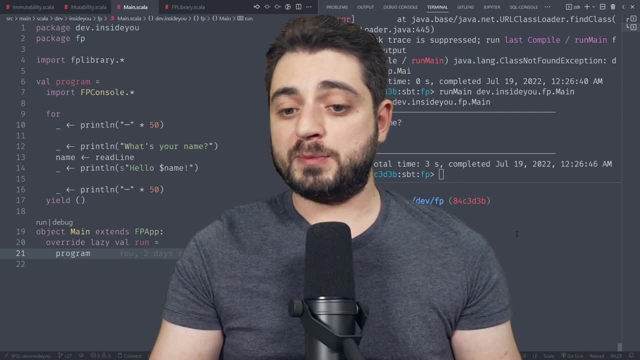 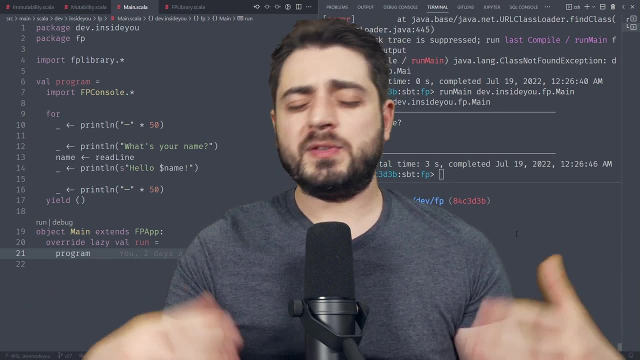 have competing libraries to uh to provide these effect types and the scale community is very small. a lot of projects have been maintained by like one guy or like a very small group of people. there is okay, there are always like occasional community contributions, but it's not something that you can, like you know, rely on as a company and so 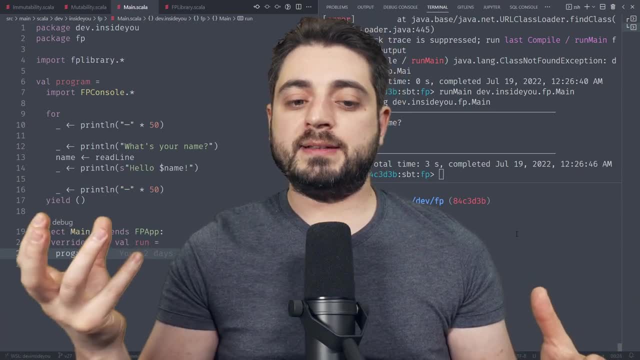 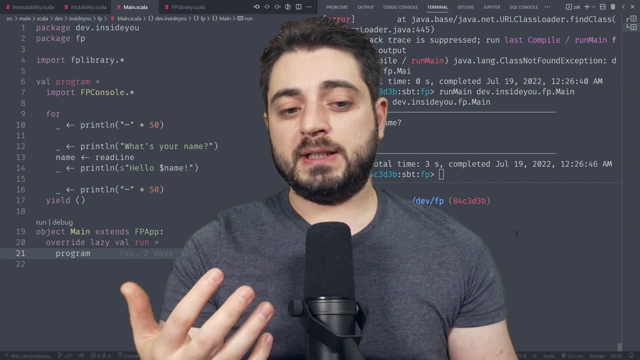 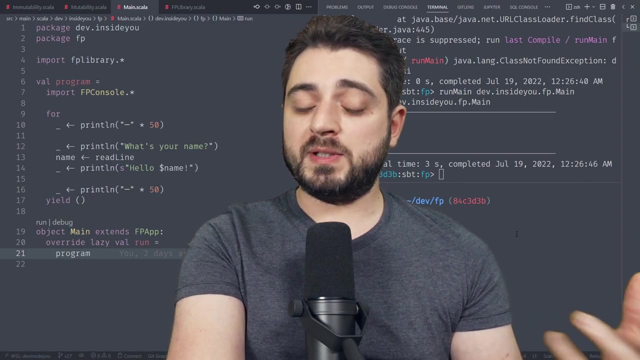 what happened over time is that we kind of took tagless final as a mechanism to abstract, a way which of these libraries we take and therefore, um, it's sort of like defensive programming: if one of the libraries stops being maintained, um, we can very easily switch to another one, because the way this works is that 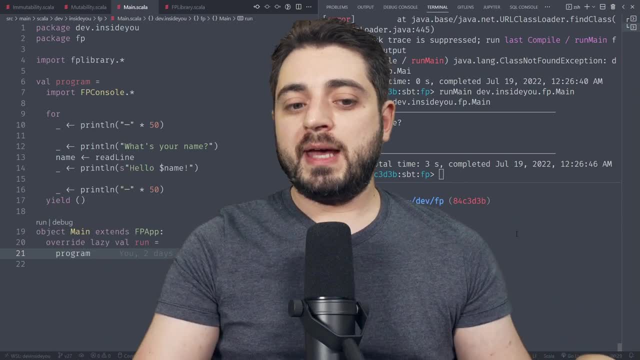 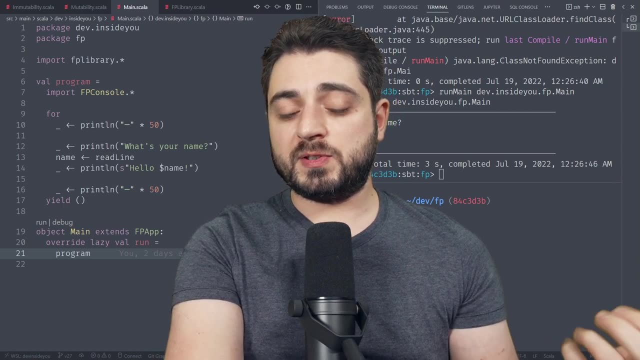 we abstract everything that we need from these effect types and only in the main method we say which which of these effect types we need. this pattern kind of dominated the functional programming ecosystem, uh within scala for the last couple of years and now it's slowly fading away. it's still debatable, it's 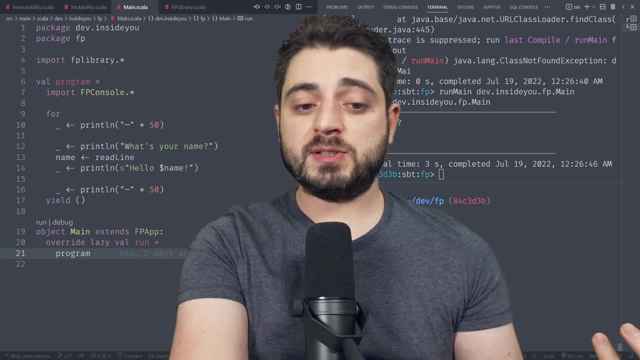 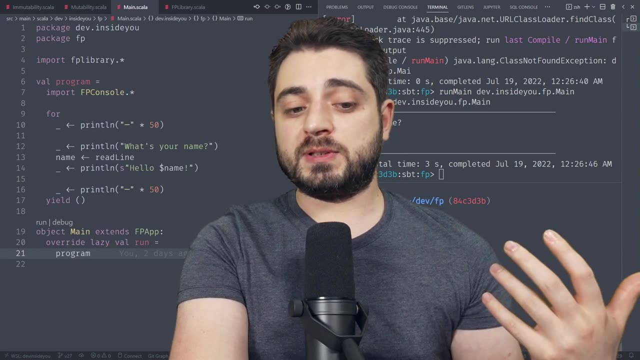 still very negotiable, like which way is better to develop applications. in my opinion, it's just not worth the trouble. um, i've been using it for a couple of years and i concluded that it's not worth the trouble. so it's uh much easier to use an io type uh directly. um, and we're gonna get to this okay. 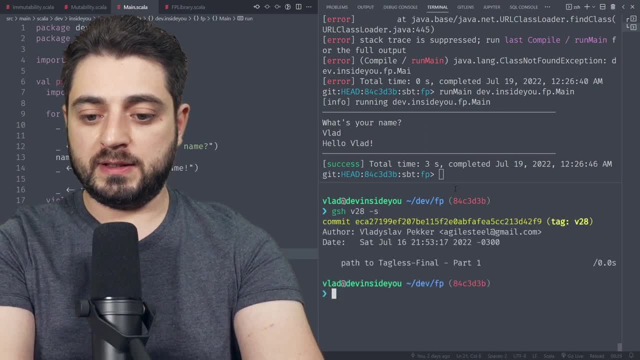 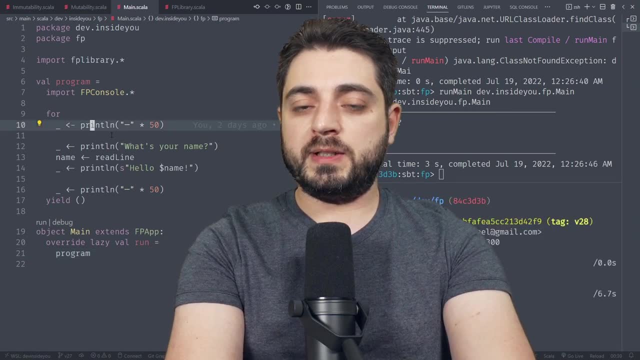 so let me see, uh, what i did. in the main method we say which of these effect in the. in the first one, right, so this one in 28.. if you look at this over here, like what are we doing? okay, so we are calculating the description of the pro of of a program, but specifically for 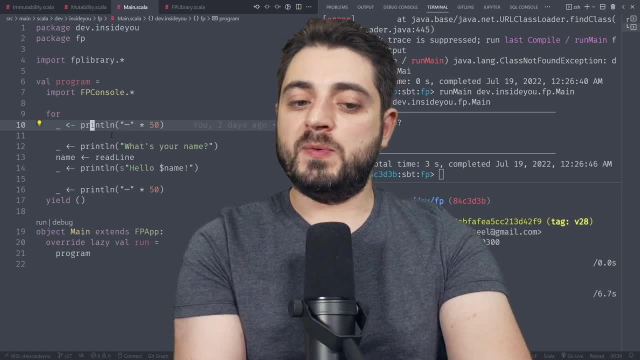 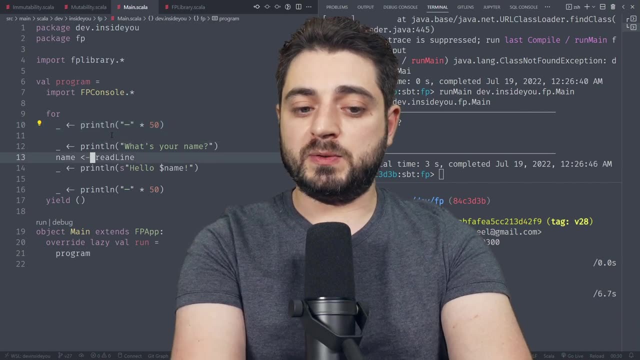 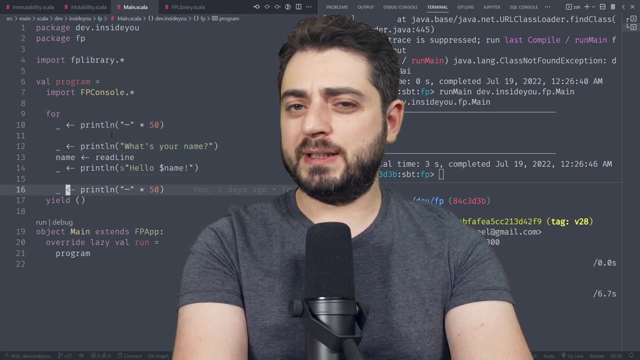 this program like: which parts of io do we need right and it turns out well, we need that part that knows how to print stuff. we need to know. we need to have that part that knows how to read stuff, and we also need that part that does the flat map right, which is like the monad part. what? 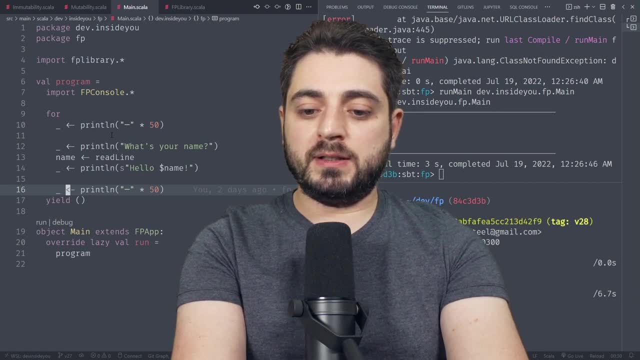 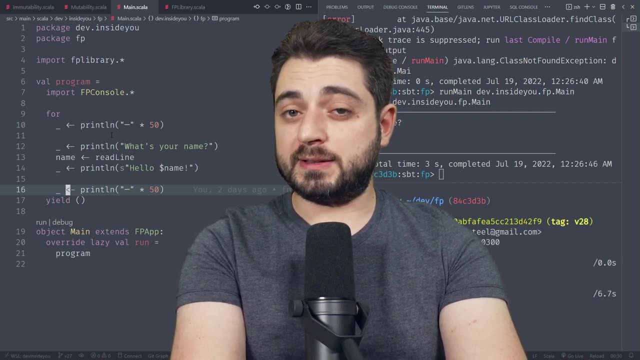 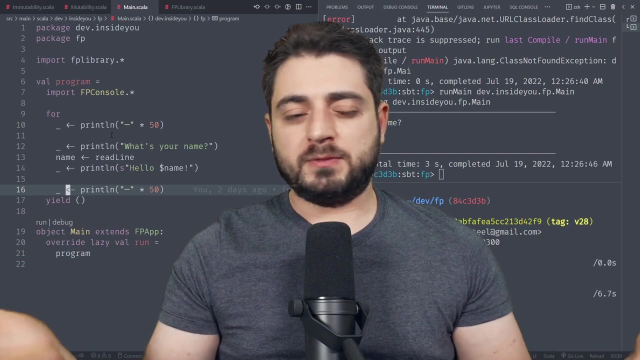 we did is we created type classes, which is a pattern that now i'm realizing, takes a little bit of time to explain. so let's run through the connection real quick. uh, every program- um, well, not every program, like every program of any like relatively decent size requires two kinds of 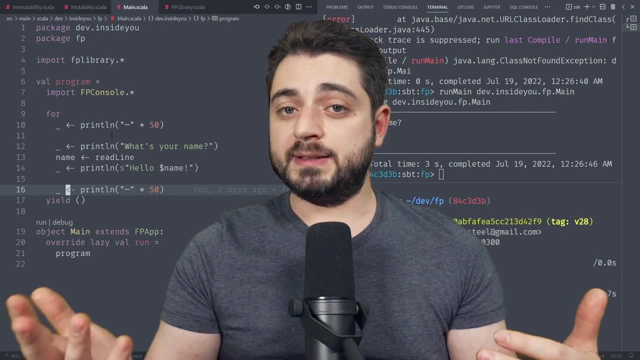 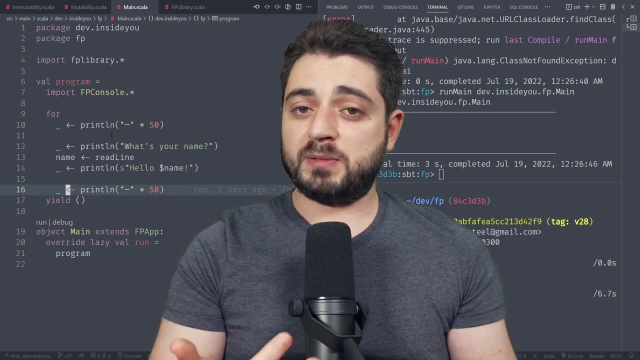 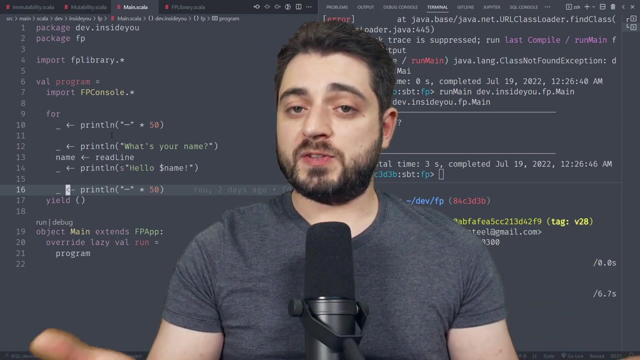 one is called parametric polymorphism. think of something like a list. parametric polymorphism means that your lists can have many shapes, but independently of which shape they will be in, they won't change their behavior, right? think about list of strengths, list of hints, list of dogs. no matter which of these lists, you have the method size on. 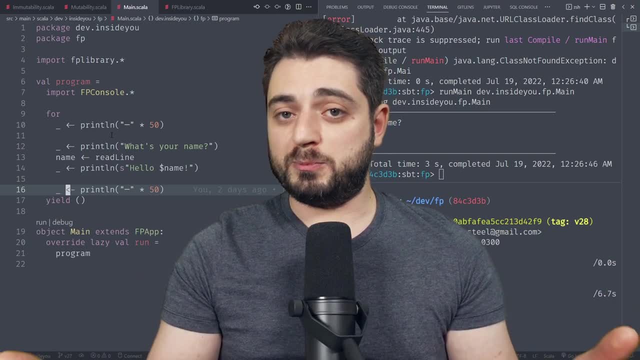 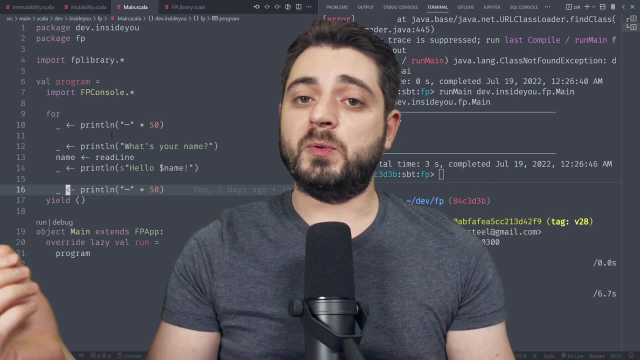 the list behaves exactly the same, right? this is called parametric polymorphism. independent of which which shape, the behavior is still the same. the other kind of polymorphism is called ad-hoc polymorphism, and it works the opposite way, right? if the shape is different, then the 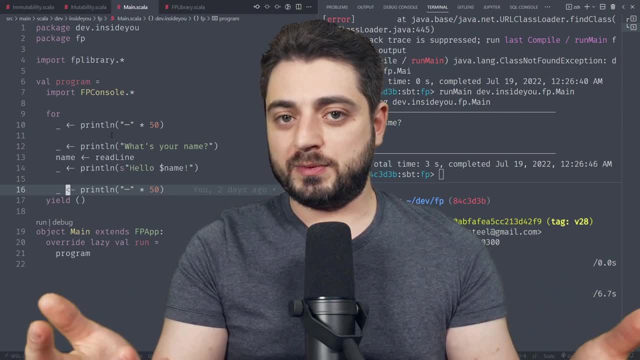 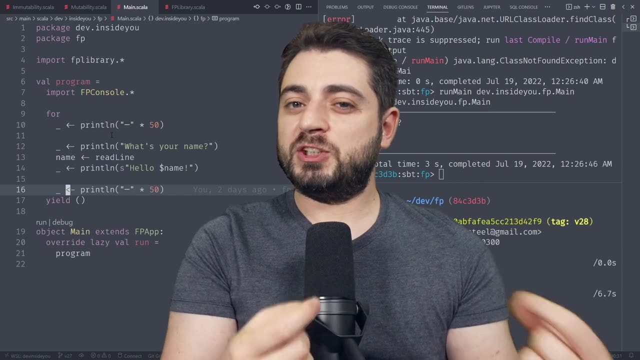 behavior is different. think of this typical, you know, animal dog example. right, so you have animal, the animal can eat or something. and now you have a dog which is a slightly different shape of of an animal. right, and it can eat in a different way. right, because the type is different, the shape. 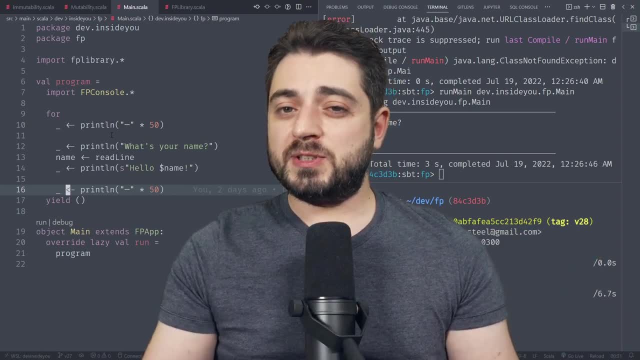 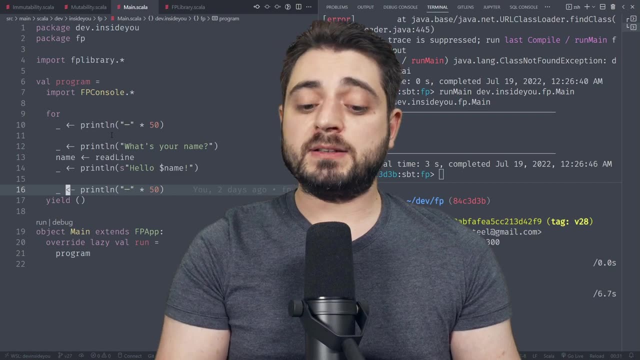 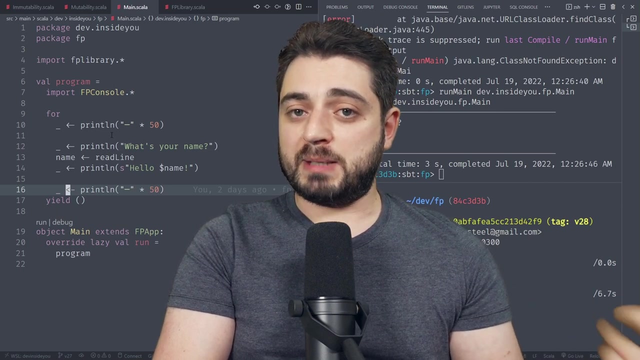 of the type is different. it behaves differently now functionali programming languages. they don't have subtypes and so the pattern that they use is called type classes in functional in. in functional programming languages like haskell: uh, this is built in into the language. there's like a keyword type class. uh, in scala, we mimic type classes. uh, we mimic them. 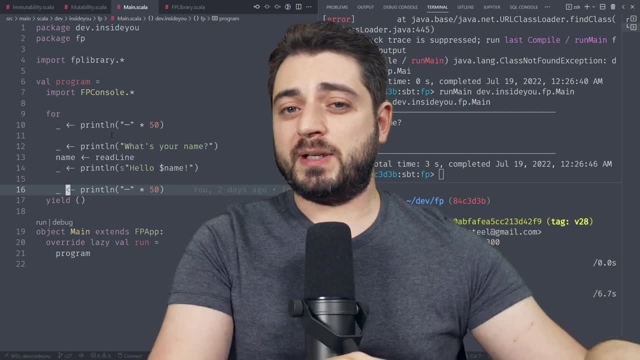 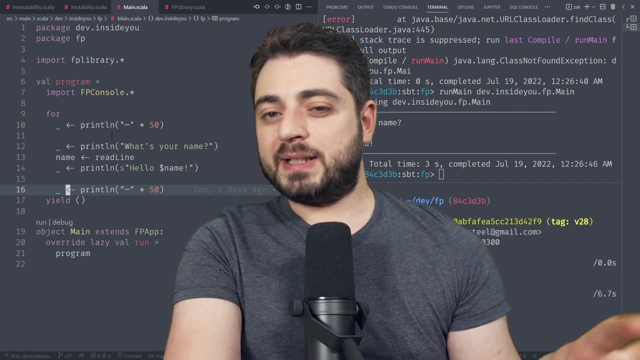 with implicits. in scala 3 it's not very visible because we kind of like moved away from implicits and we we also gave, like uh, specific keywords for uh, for something like type classes, but also not directly. we still don't have a, we still don't have a keyword for type class and in scala 3 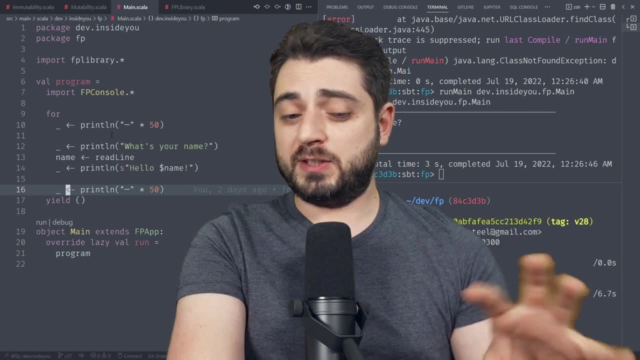 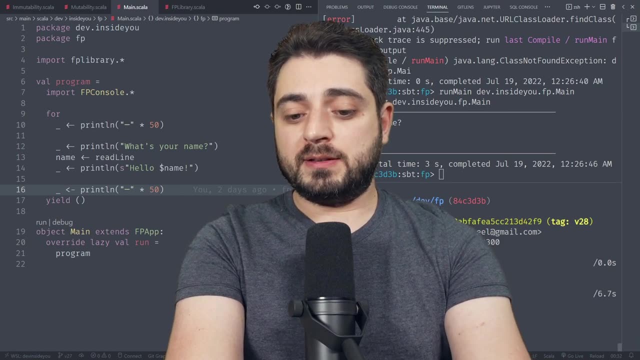 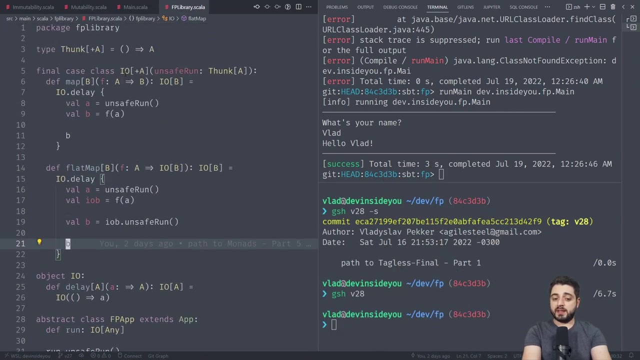 syntactically you won't even see the difference in usage. right in the declaration there will be, but in usage you won't see it. okay, so what the next thing uh is? uh, you know what the next uh is explaining is that, in an object-oriented way, uh, to look at things, io is a monad. 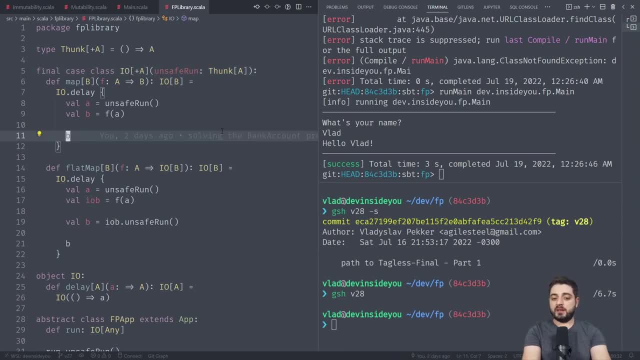 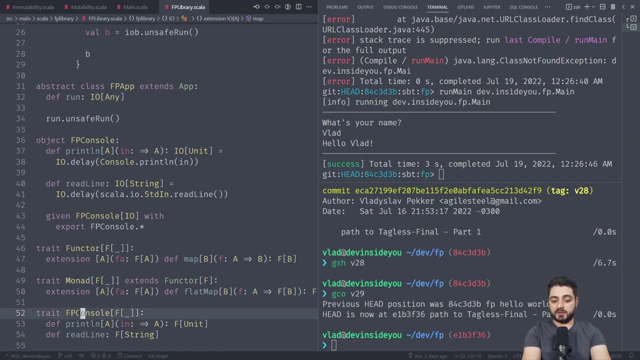 however, in a functional programming way, io has a monad, okay, so the next thing i'm going to show you requires a lot of like scala mechanics, okay, so at the bottom we have two traits- uh, actually three traits. right, there's also one for the console. actually, i jumped. i jumped like too far. i think i wanted to jump to 28 first. so we have. 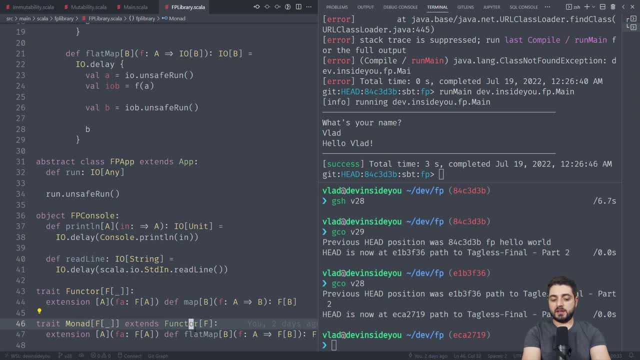 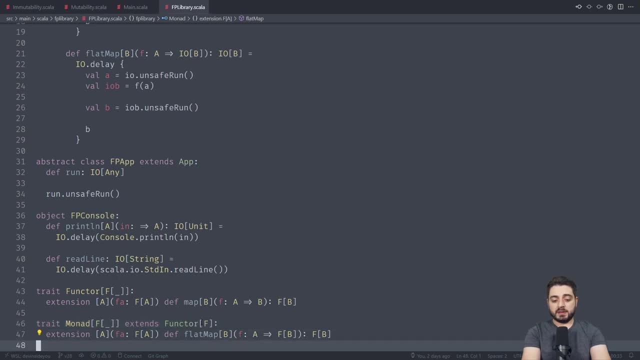 like the functor and we have the monad and monad extends the functor. okay, and basically, like we, in a hand wavy way, we said, okay, monads, everything, it has a flat map, okay. so this is how monad looks right, but there's no like io inside. also, there's like no thing inside that you're going to call. 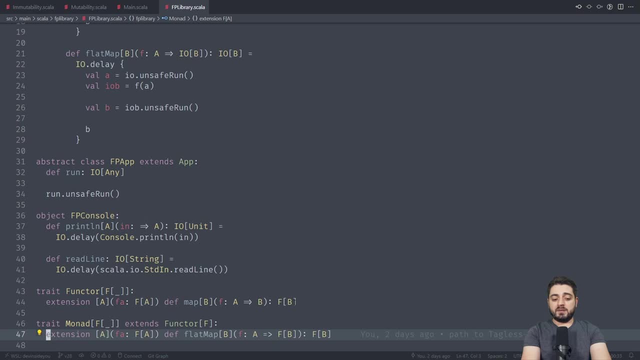 flat map on, and the way this works is that, like, whatever extends this trait is going to have flat map as an extension method. okay, so we're working with like parametric types over here. okay, so we're saying: okay, so there will be a monad for some type f which is of a higher client. 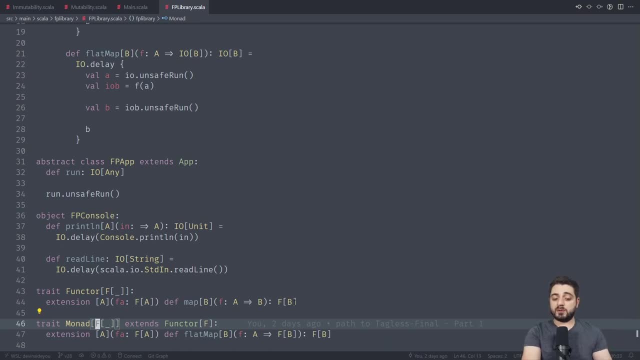 right. so there will be something inside of this app like f could be a list, could be an option, but in our case it's going to be io, okay, and because of this we're going to be able to call flat map, and so, like the definition of map and flat map, it stayed exactly the same. 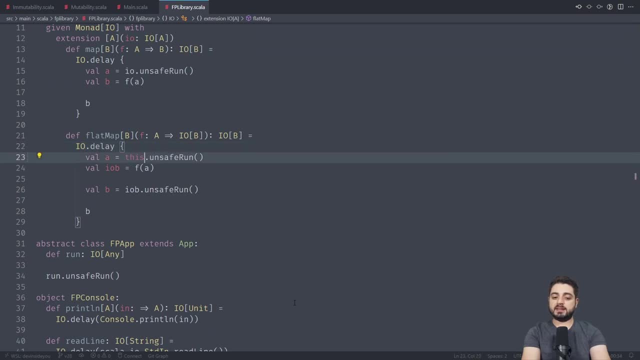 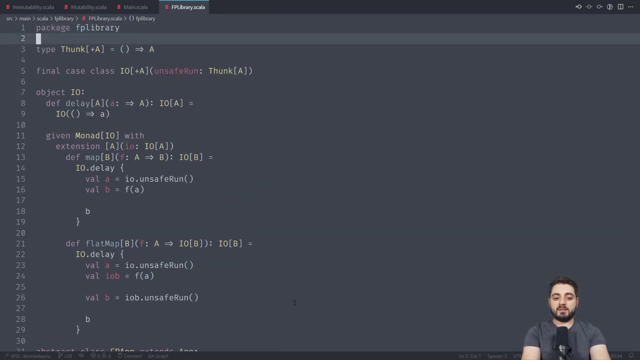 it's just that instead of calling unsafe run, so instead of calling like this, unsafe run, you know we're calling iota and safe run and io comes from this like extension thing, syntax okay, and so effectively io becomes a simple data structure. okay, but there's a type class called monad. 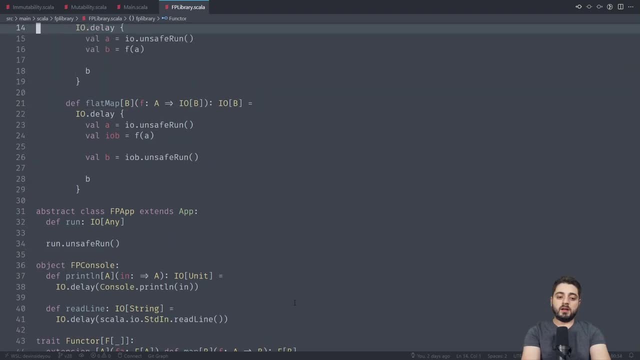 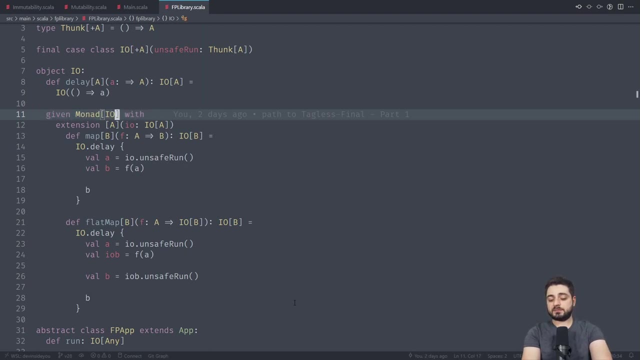 somewhere which extends the functor, which doesn't really matter, and over here there is an instance of this type class. so, given an instance of the type class, if it is in scope, this color compiler will actually inject it for us. there will be extensions, extension methods on io which are like map and flat map, right. so i'm actually going to show you. 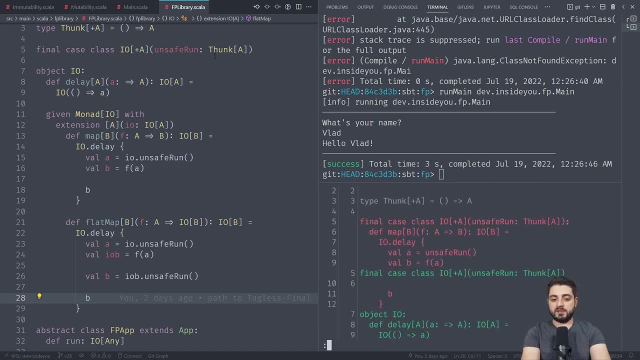 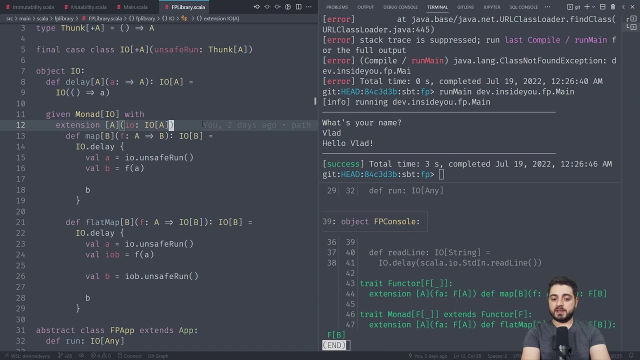 this. so if you look at v28, right, so the functional programming library class like file changed right was everything that i just explained, but nothing else changed right. so this is what i meant, like syntactically, like the on on the usage side, you wouldn't even 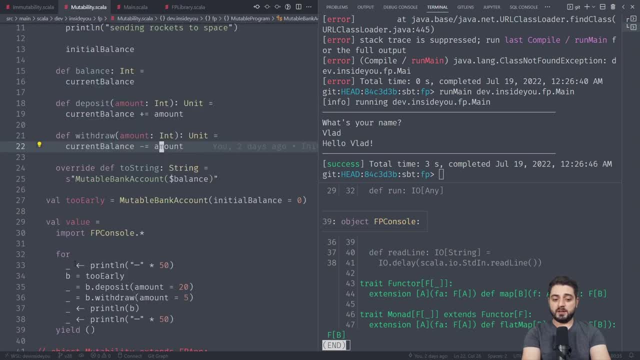 notice a difference, right? so, for example, here you know, the full comprehension still works because it still looks like as if io simply had a method called flat map. okay, so as a user, you don't even see, uh, whether type classes were used or whether subtype polymorphism was used, but on the 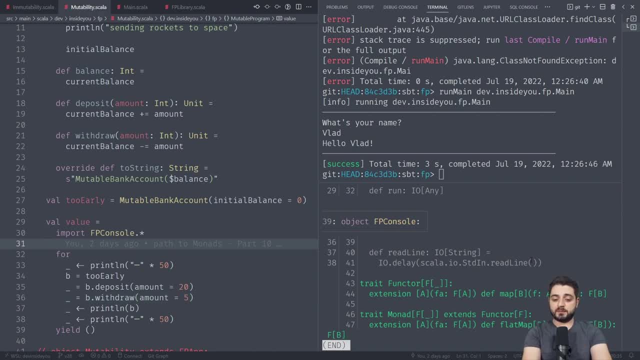 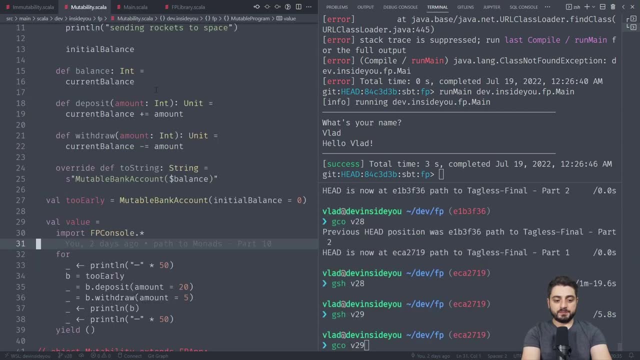 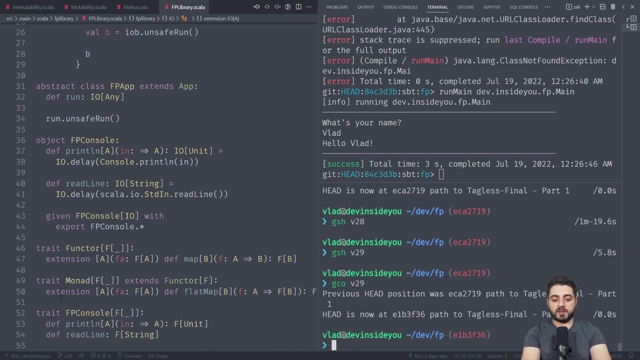 declaration side there is a little bit of like scholar mechanics. okay, so what this allows us to do, which i haven't done yet. let me check out v29, but i actually don't want you to see this file yet, okay. uh, a function program library. okay, so checking out 29, and in 29 we also have another tab class for console, right, so it pretty much. 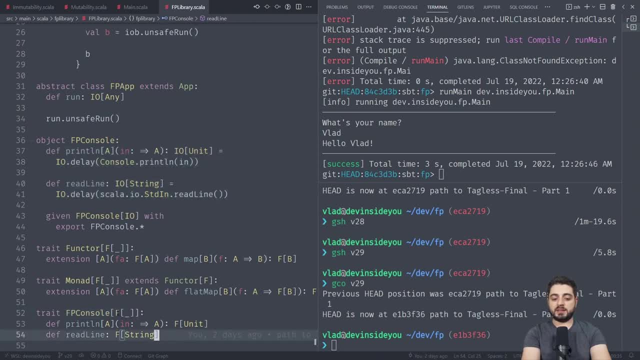 looks exactly like this object. it's just that the methods are abstract and it's not hard coded to io, it's hard coded to some f right, and so the result is like an f of unit instead of io of unit. here is f of b instead of io of b. this is kind of hard to explain like. this is another instance, right. 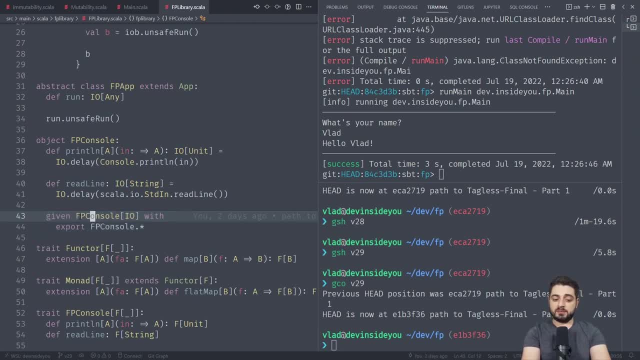 it's an instance of a different type, class, it's a. it's an instance of a p console of io. okay, this is, it's a very subtle thing. by the way, these instances, they need to hard code for which type. right, and this is how you can do uh, composition, how you can favor composition over inheritance. 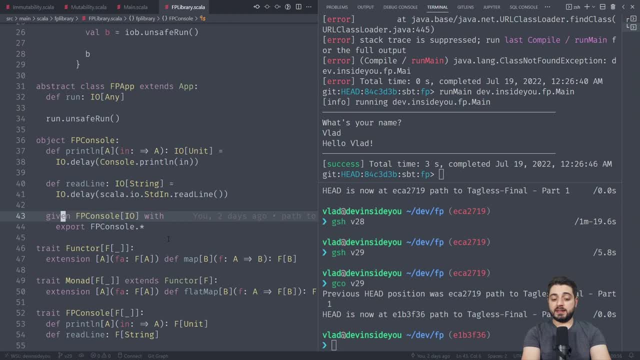 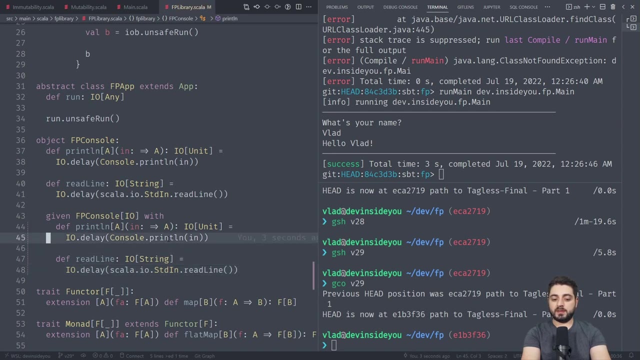 in scholar three, right? um, basically you're saying, okay, this instance is going to have like exactly these things. okay, so basically, like this export thing is doing exactly this, right, like what just happened is exactly the same code, right, it just said i didn't need to do that. 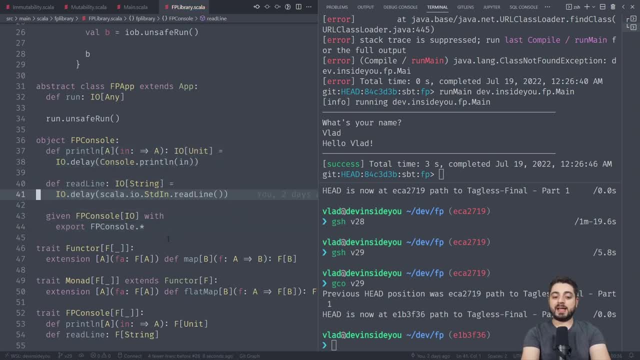 i could just say: import everything that is inside of this object. uh, export everything. okay, exactly the same code, okay. so now that we have these pieces in scope, we can say: we can write our program in such a way that it doesn't depend on io, but it depends only. 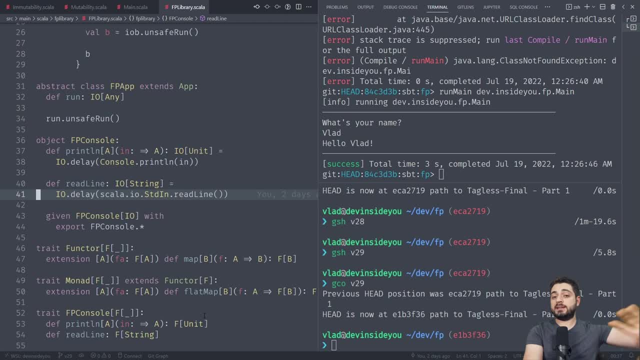 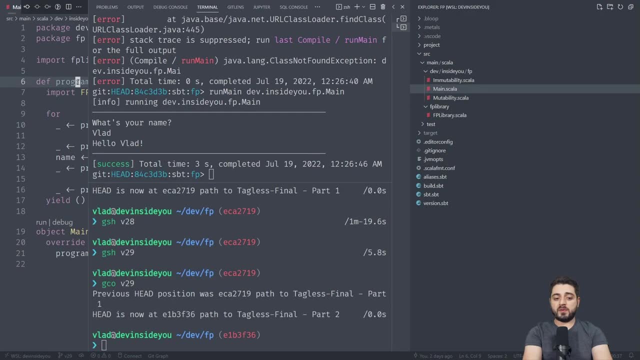 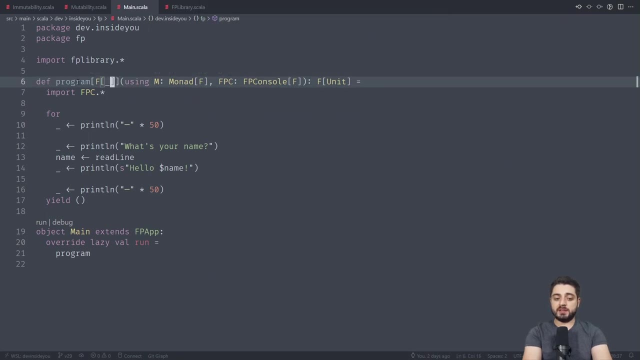 on these pieces, and the trick is that these pieces are in a separate library, right, it's going to be a free file and it provides these type classes, okay, so in our main method, the program is now like: there's no i o in sight. okay, if you look for io, there's. there's no io in this file, okay, so 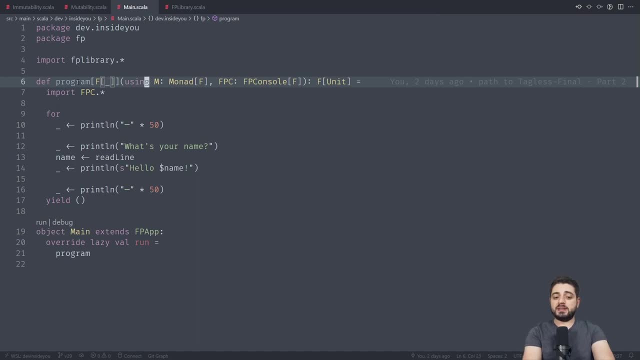 it's going to be a program for some very abstract f and assuming that there is an instance of the monet type guess for this app and there is an instance of the fp console type class for this app, which is going to be you, then somehow we're going to do something and we're going to produce. an alpha unit, right, and so the problem is, the reason why we're going to have a type class for this flat unit is because this type class is called a nice class, right. because the anime type class is a防 пор mission, right, and so the problem is the program. we need to have this type class to be in use in. 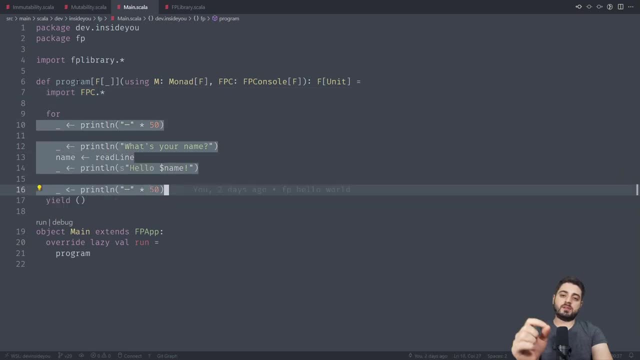 the project. so if you have a type class, this will give us this type class. this type class, that is fishing method, And so the program stays exactly the same. well, because the methods in those type classes are called exactly the same. okay, But now there is no IO inside. 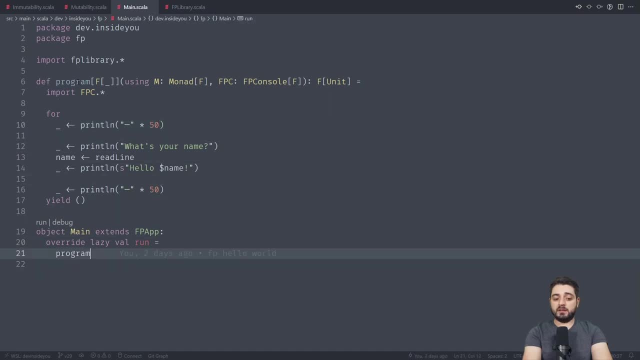 And therefore at the very end over here, type inference help us out, but essentially the compiler inserts IO over here. This is the only place where we mention IO and therefore we can switch between those libraries, assuming that we have some other libraries. 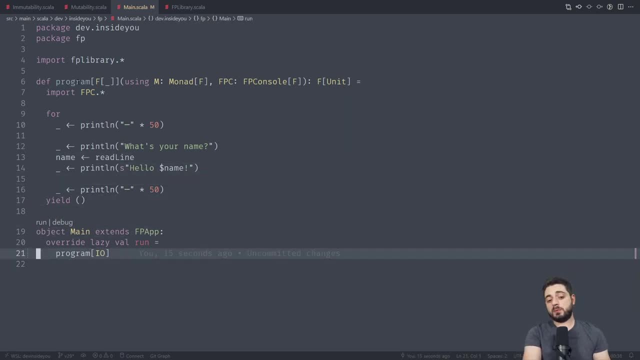 that bring in the instances of those type classes. okay, And so what happened in Scala is that we had a library called monics, which had a first mover advantage. It came in with. I believe it's like iomonics, I believe it's iomonics eval task. 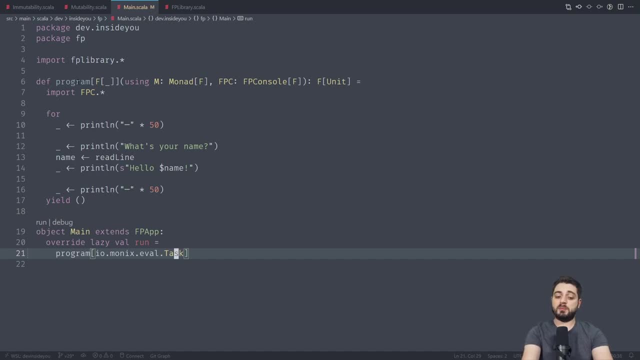 I don't have it in the class pass, but it would compile with, like certain things, It would compile, okay. Then after this, we had a library called cat's effect. right would work exactly the same way, right. And all of these libraries. 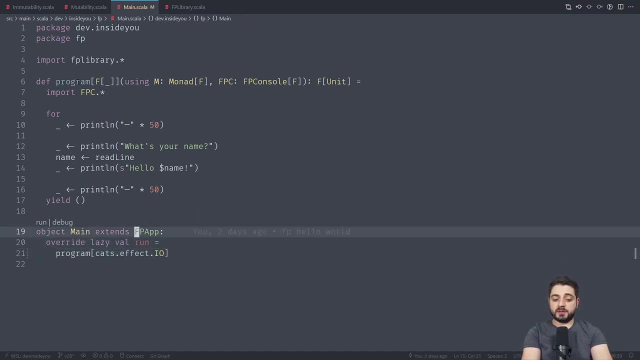 they come with like a similar looking trade thingy here And cat's effect is a little bit confusing because cat's effect has IO, It has instances for the type classes for IO, but cat's effect is also that library that defines those type classes right. 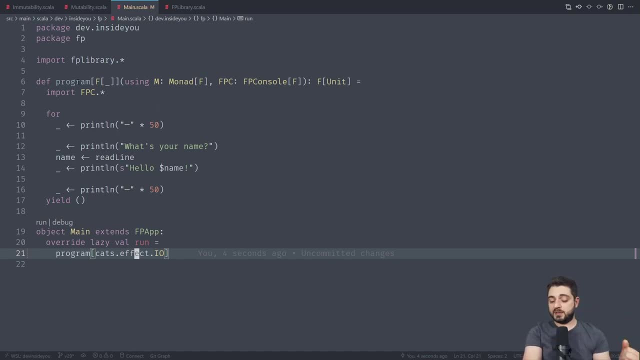 that monics implements and that the next library that I'm going to introduce to you is also going to implement. okay, And the last one is called. oh, good question is called uh, zio, right, so this would be like zio dot. uh, i believe it's called io, or maybe it's. 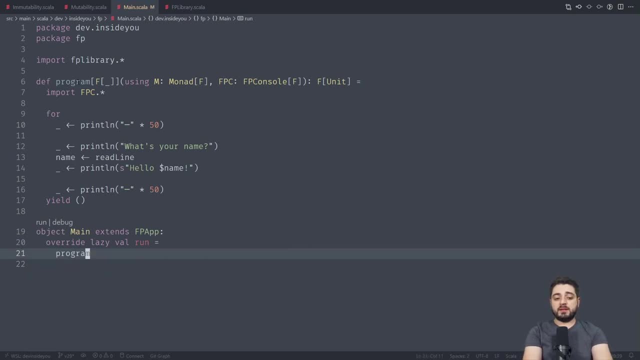 called task? i don't remember. that's not the point. one other thing that this tecla spinal technique provides is what is called tracking. in particular, in this case we're tracking the effect type, so it's called effect tracking. okay, so before, when this was io, you couldn't, kind of like know what. 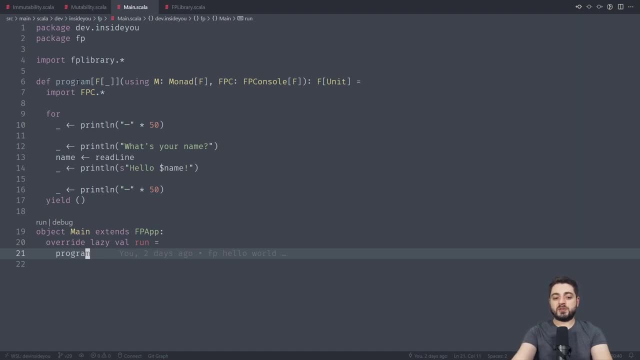 the program is doing? what is it? what is it describing? it could be a description of sending rockets to space, or it could be a description of simply printing uh stuff out. you would only know this once you know uh, after you looked at the implementation. on this case, the implementation is: 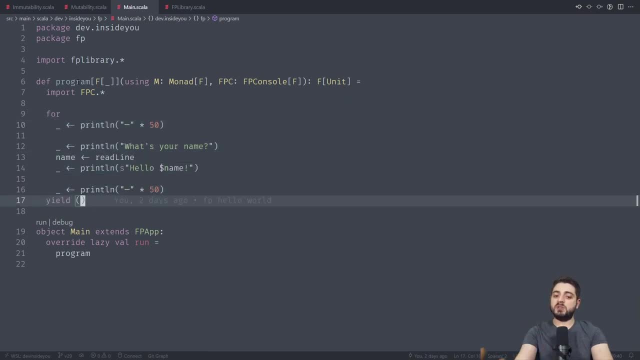 just a couple of lines, so it's not a big deal. but imagine if this was like a huge method. okay, with this, you kind of see what it has access to. you see, okay, like it's going to be some abstract app, but all it will be able to do is whatever limona you know allows it to do. and 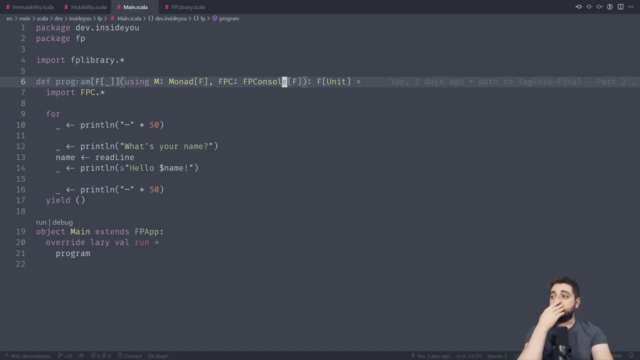 whatever the console allows it to do, so it kind of gives you, like this, um, a little bit of a false uh confidence uh about, about your code. in practice, it turned out, uh, not to be uh that valuable though, and, by the way, this is just my opinion, right, because what happened in 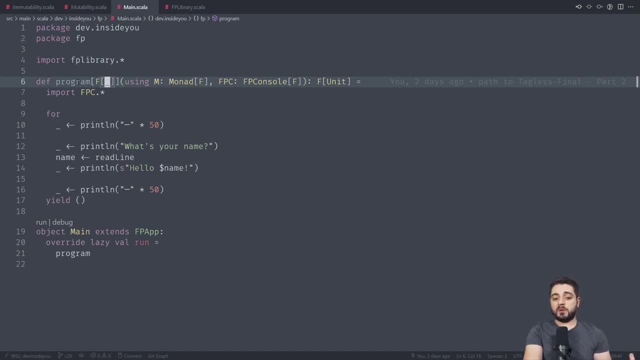 practice is that most of the time, uh, like all of your ass, will require a monad uh and also a capability to uh throw or handle errors right in cat's effect. it's called monad throw, okay, and so most of the times like at least this effect tracking portion was not. 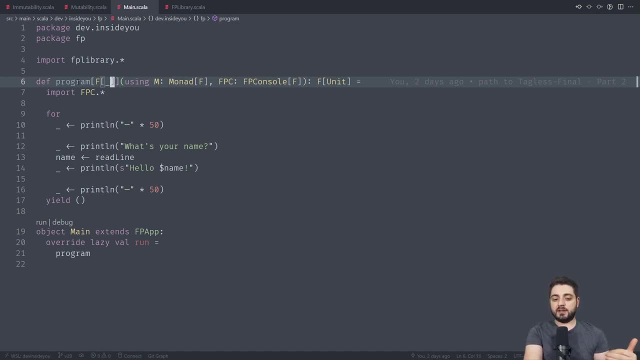 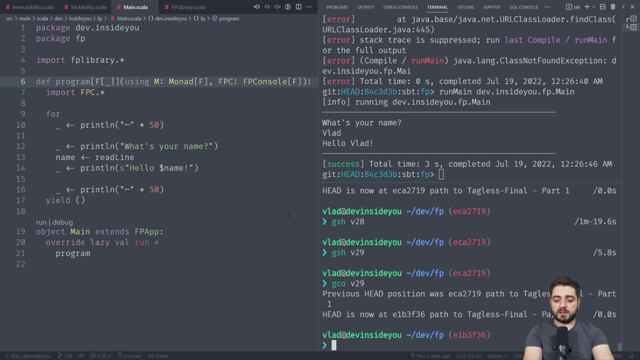 was not valuable enough to justify, uh, rewriting the code like this, um, and i should. i should show you a couple of examples of it later. okay, so let's actually move on. we're almost done right. we're 20, 29 and there are only 32. okay, so i believe the next one shows just a couple of syntactic. 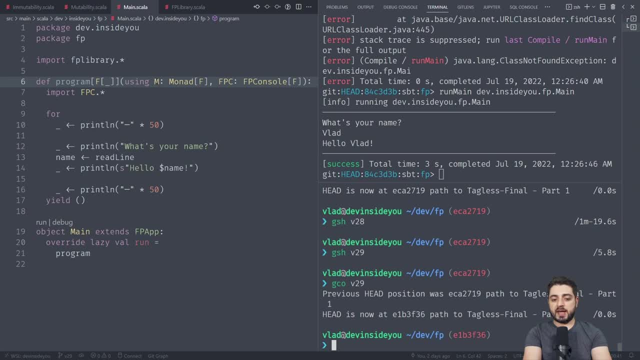 things over here. so, if you notice, we're not actually using the m anywhere, right, but the compiler knows that it's there because of this using thing. okay, and so, uh, this one we do use, um, save a couple of keystrokes, right, and the way this works is that by, uh, by splitting these. 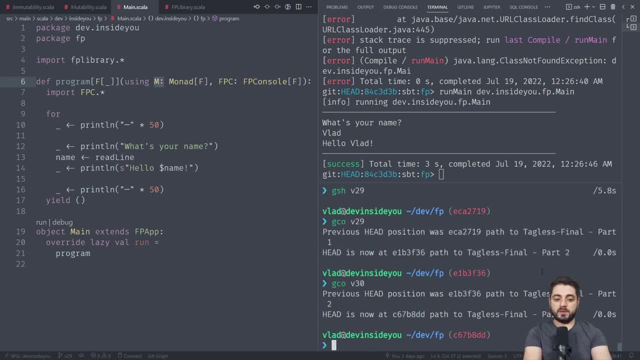 parameter lists. okay, so if we check out v30, you're going to see that now that these parameter lists are split, in this one you can have, you can mention the type classes that you're not going to need to reference by name, uh, but in this one you're actually going to require the names, okay. 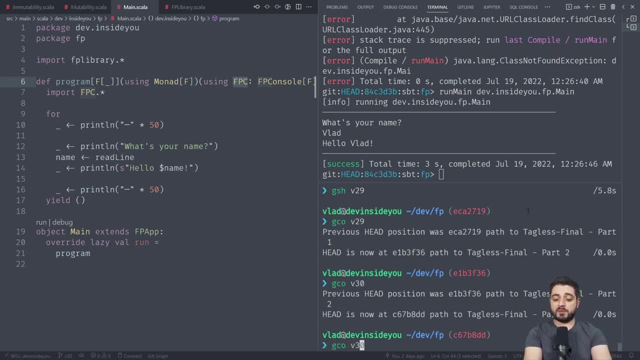 and we also have another syntax called uh- context bounds, where we basically can say, okay, well, f is not a monad, but f has a monad. so we're going to say, okay, well, f is not a monad, but f has a monad, right, and the way it works is that we have like a colon over here and we do like monad over here. 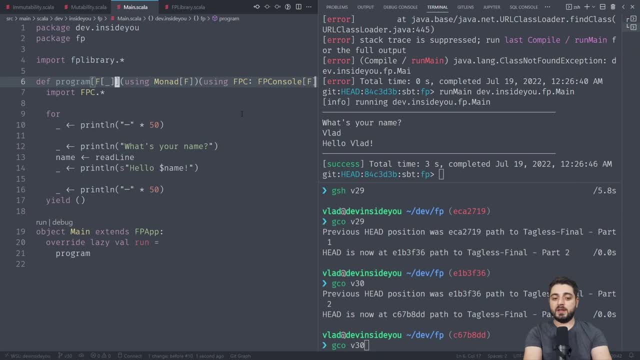 it's a little bit shorter because we don't need to mention this f. okay, so i remove this and then check out um 31 and this is exactly how it looks like okay, so usually, like in most cases, you would see like it needs a monad and you know it needs an fb console and so on and so on. uh, however, like. 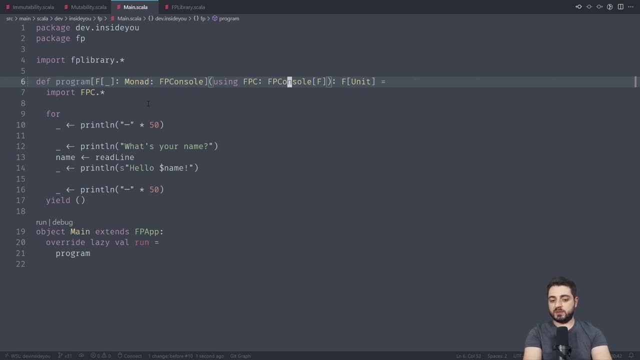 in this particular case, because we actually need the name, it's more convenient to do it like this: okay, another way to do this would be, um, to like remove this and to have like a val over here, fbc, and you would say, well, uh, could you please? 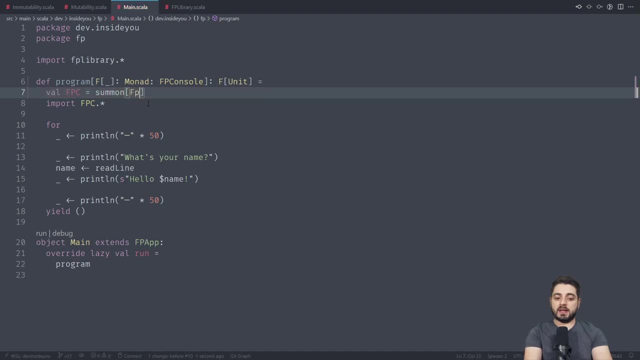 summon uh in the instance of the fp console. fp console for f. can you please summon this? and summon is just a uh function in this color standard library and it looks like this. i'm gonna call it find or something like this: right. so find some a right, and it's going to be like a. 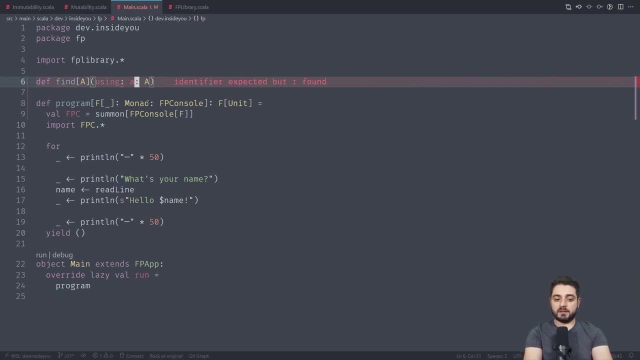 using of this a um. like this, right, and it will return this a right. how's it going to do this? well, like this, okay, so this thing works exactly the same way, right, so i can put find over here. right, and it's going to work exactly the same thing, right? fbc is like fb: console of f, right? so basically the 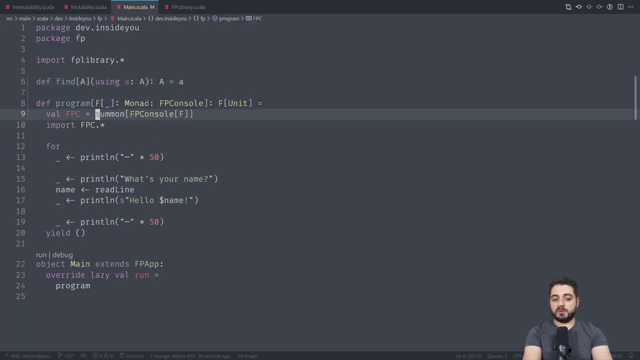 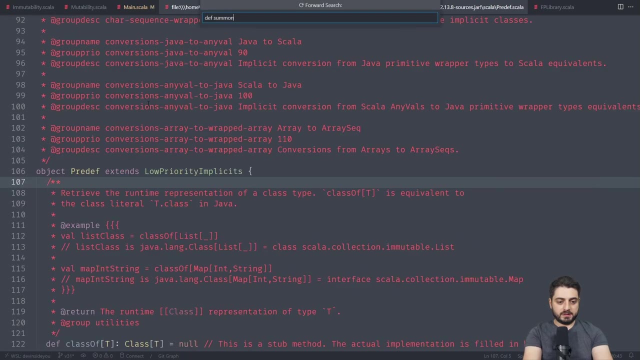 compiler will inject this a and we'll just give it back. so if we go back to summon, i would jump in there. you're going to see that. uh, let's see, i can't find it, but this is how it looks like. okay, go back to my code. we're pretty. 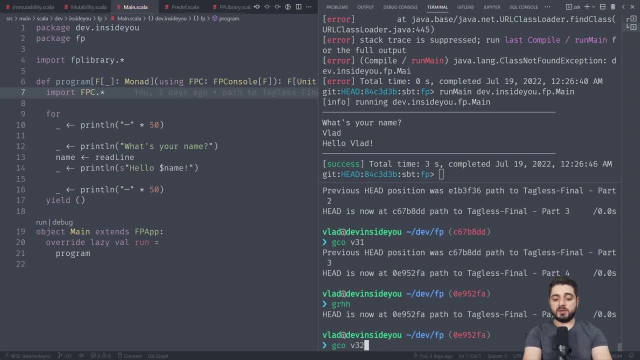 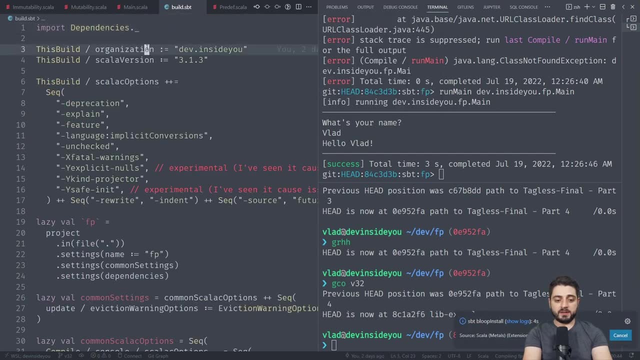 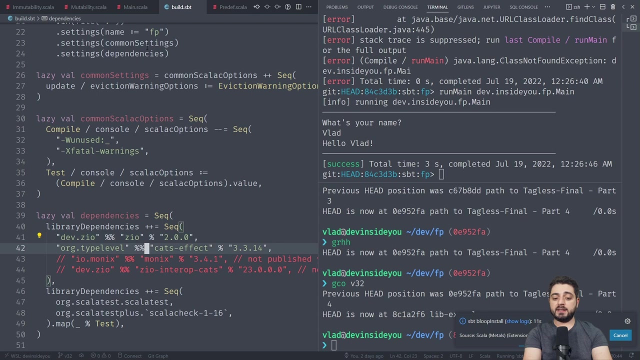 much at the end. the very last uh commit is going to show, um, how these libraries are actually used. okay, so in in the build file, um i went and um i went over here and i added zio and i added cats effect. monix is not published yet. zio interrupt. 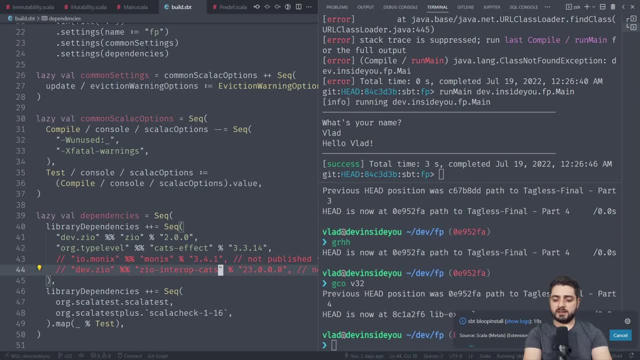 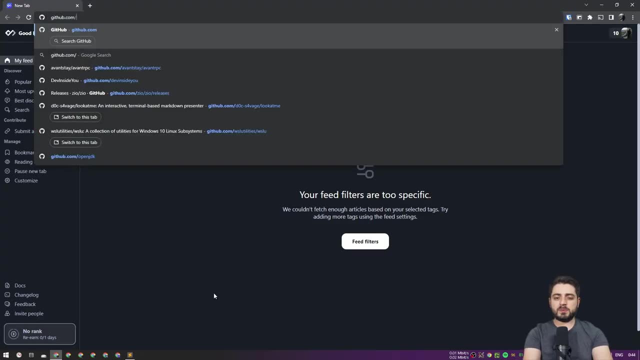 for cats is not published yet. in fact, maybe it actually is published, uh, already. uh, let's actually check this right now because, like some of this stuff is very new, because we're i'm using like a cutting edge version of scala right, so it's like the latest scala 3 version. zio 2 just came out and, um, let's see. 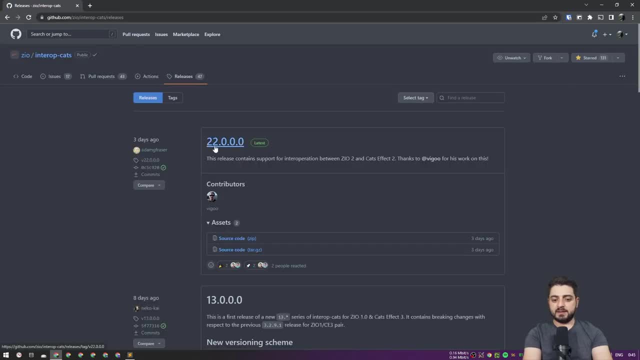 so zio, interrupt cats like. as you can see, this one just came out three days ago and they recently switched to an epoch kind of like release. so you have like major minor patch over here, but over here you have like the first two, and then you have like the first two, and then you have like the. 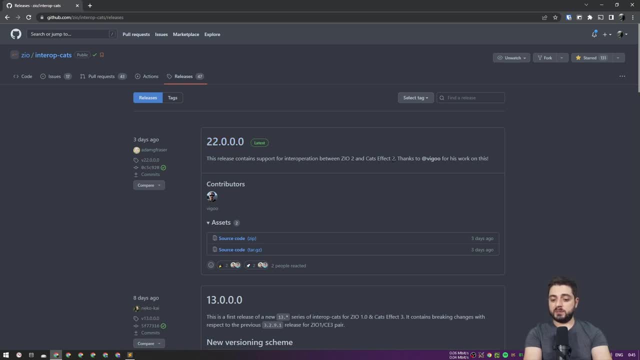 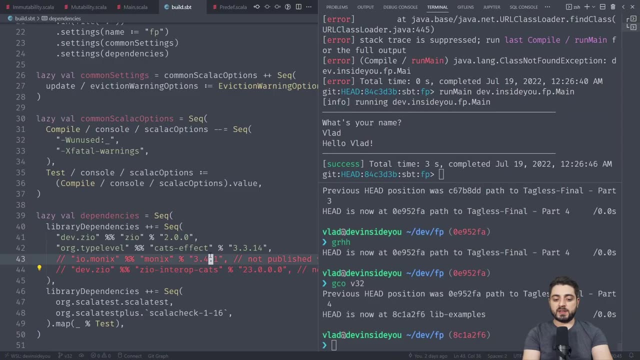 second two stands for zero two and the second two stands for cats effect two, and we need two three for zero two and cats effect three, which is not published yet but i'm sure it will be in just a couple of days. this is also like one of those things that like uh, techless final technically. 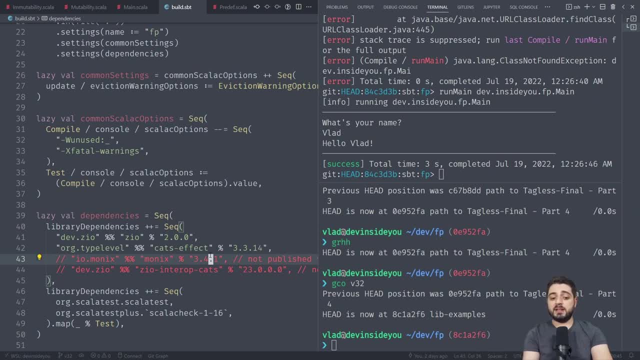 protects you from your um effect library not being maintained anymore. however, you might also run into the situation where you know the interrupt library is not maintained like as fast at least. okay, it's not exactly the same thing, but you know it's getting there now like in the main method um i 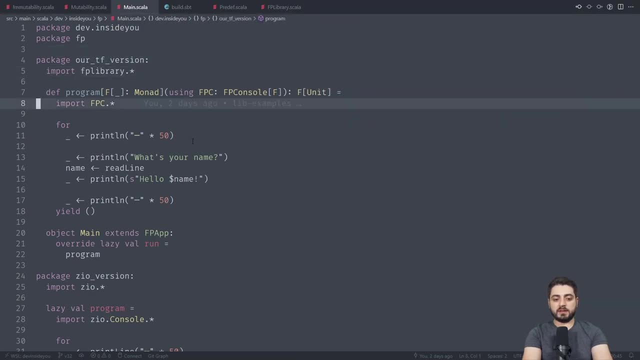 have like a couple of versions, uh, over here. right, so this is like our version it's called. you can define packages inside of other packages, okay, so this is still our version. still looks exactly the same, okay, and this is our main. you know, and stuff. this is the zio version. you're going to see that it looks pretty much the. 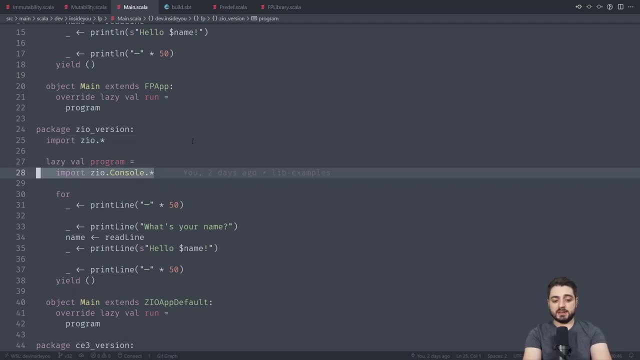 same same way, just the import is different. uh, the console is like somewhere else. the method is called slightly differently. you know, print line, print line, read line, blah, blah, blah. the main looks pretty much the same, it's just that we're extending that thing from the library instead of 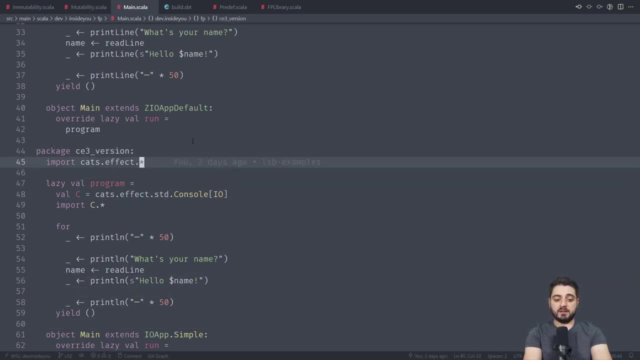 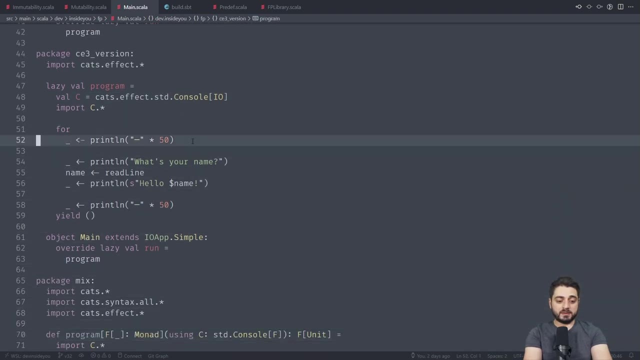 this is the cat's effect 3 version. you know, you import cat's effect star. uh, there's a slightly different way to obtain the console, but but however, the you know same goes. you know, printer line, printer line, read line: blah, blah, blah. right, so this is now. it's kind of hard to read, but 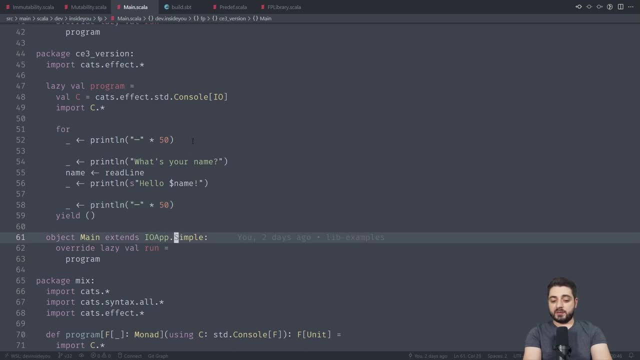 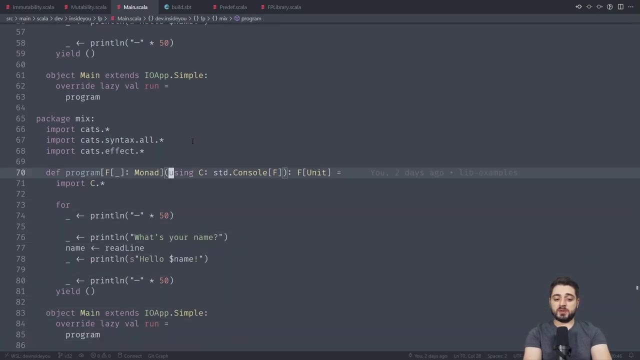 essentially it's i o unit, slightly different trait, you know, named slightly differently but behaves exactly the same. you know i o app simple and this is a mix like this is a techless final. we had the message but we cannot inject like any other effect type because the libraries are not. 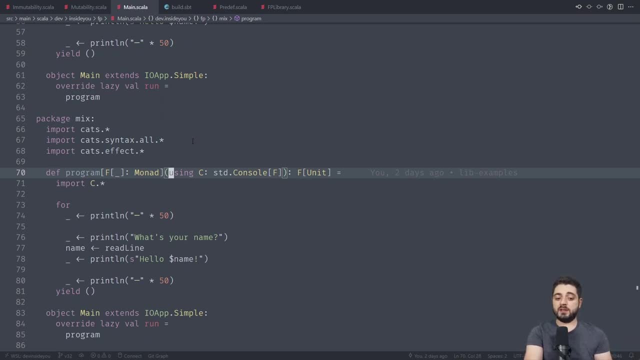 published yet. so the only effect type that we're going to inject is going to be still cat's effect. okay, so, as you can see, we need, like, more imports. we need cats because it brings the mono type class. we need cat's effect, which brings the console type class. we need the syntax so that we 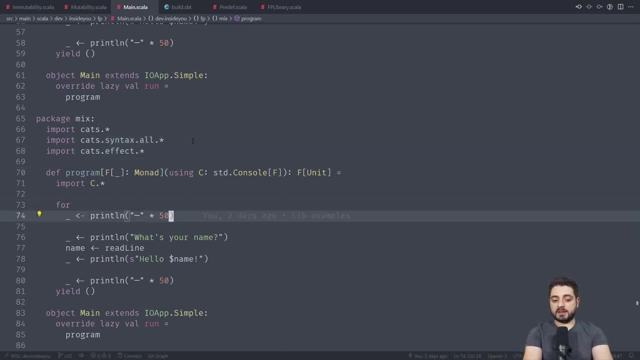 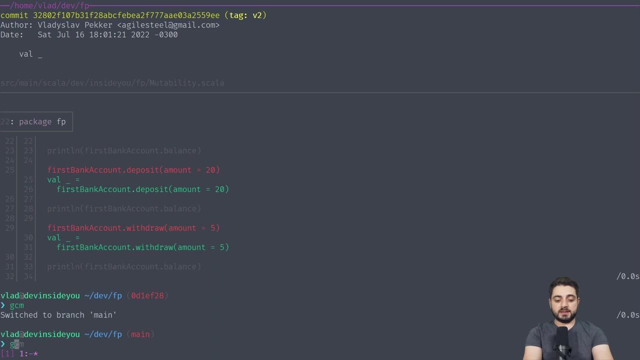 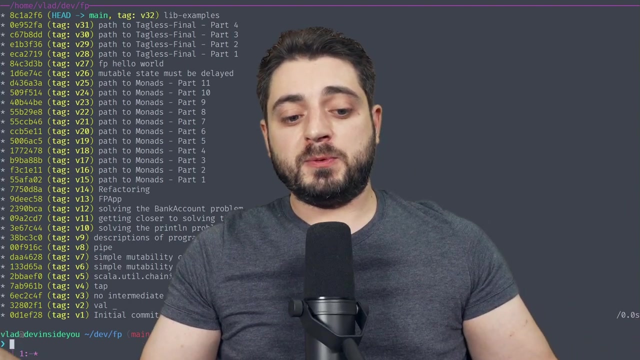 can do the dot flat map and, in the end of the day, the program looks pretty much the same, right? so, yeah, these are all the versions. repository is going to be available on github and you can check it out, um, at your own pace. let me finish this video by saying a couple of words. now. which one should you choose? uh, when it's called. 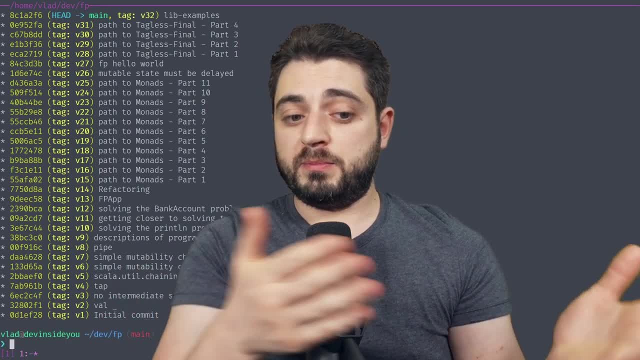 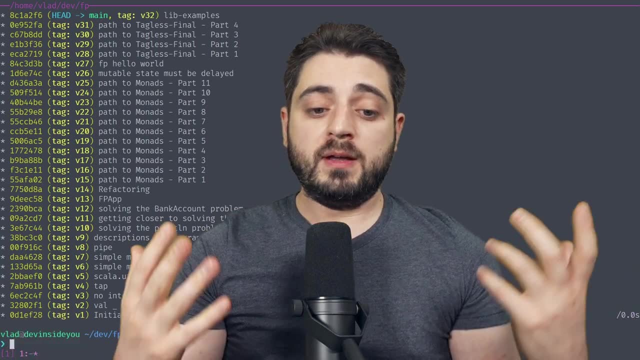 it's called. we have, uh, basically either three options, right, either monix gets effect or xeo, or you can go with tagless final, and then, at the end of the world, you can decide which of the effect types you're going to choose. okay, now, uh, monix has the first mover advantage. it's been around since. 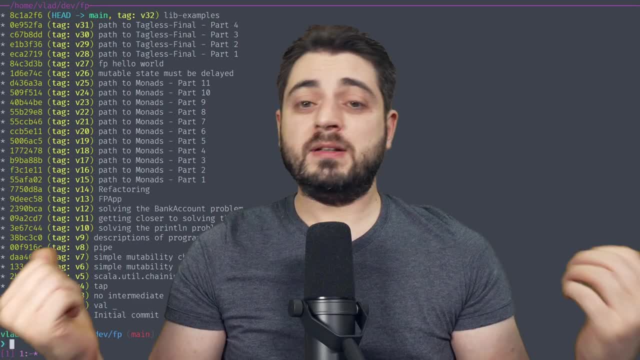 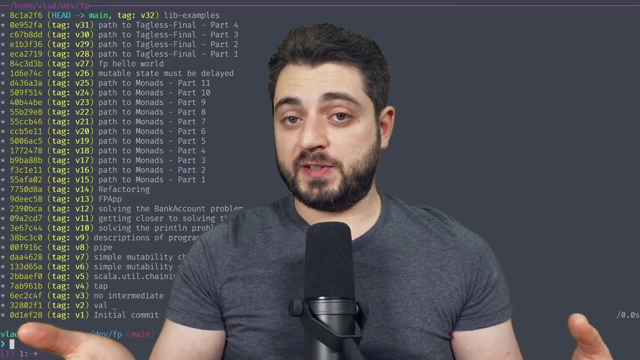 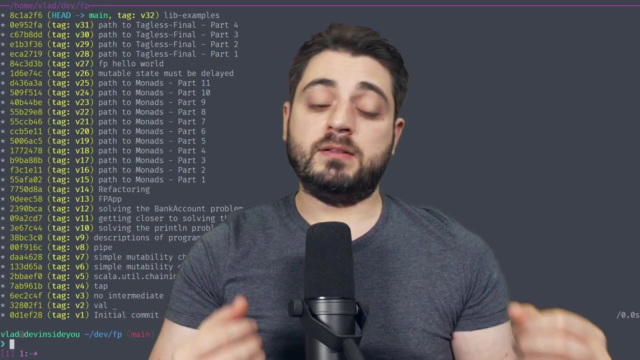 2014, 15, maybe even 13, um. um, it's a very good library. in fact, we still use it at work. uh, the issue with it is that the bus factor is very scary. okay, it's, but it's maintained by a very small, uh, part of the scholar community. uh, in fact, recently, the main maintainer had some personal issues in. 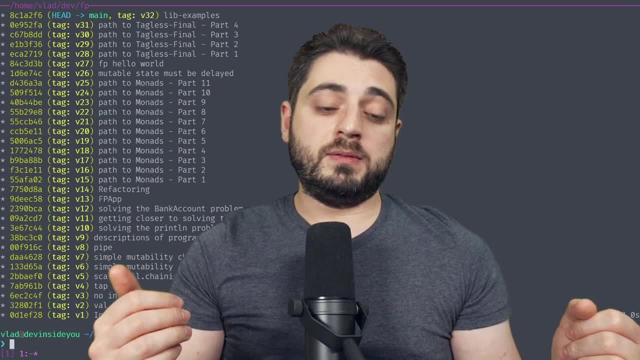 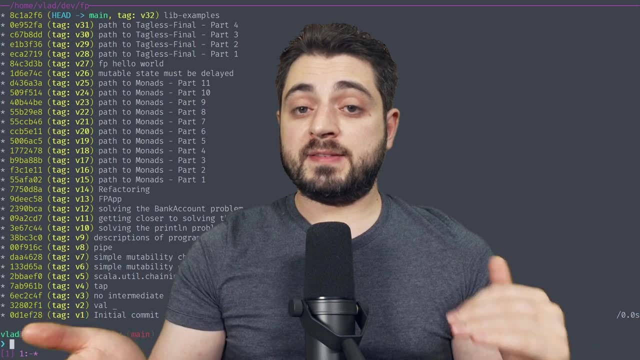 his life, uh, so it wasn't maintained for a couple of months, um, or maybe like even half a year. luckily he came back, so it's still still alive, it's not dead or anything like this. um cats effect, um is the uh battle tested library, uh, especially cats effect 2, because very recently cats effect 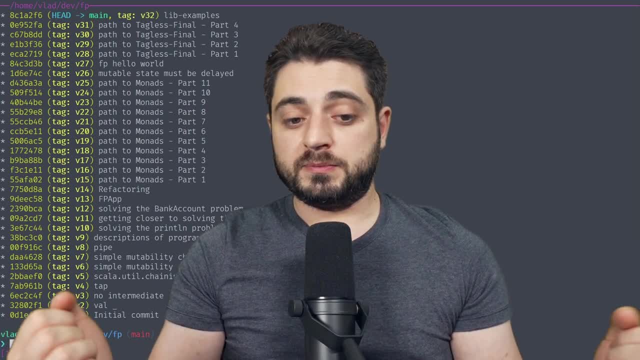 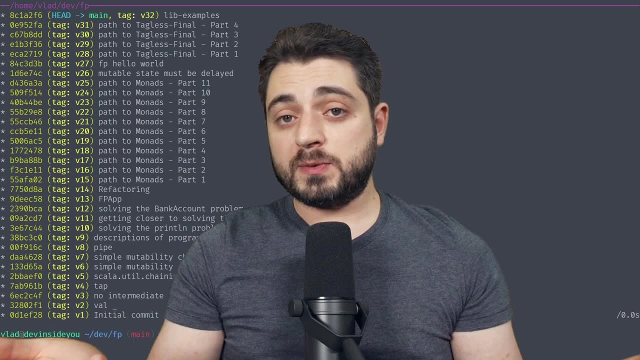 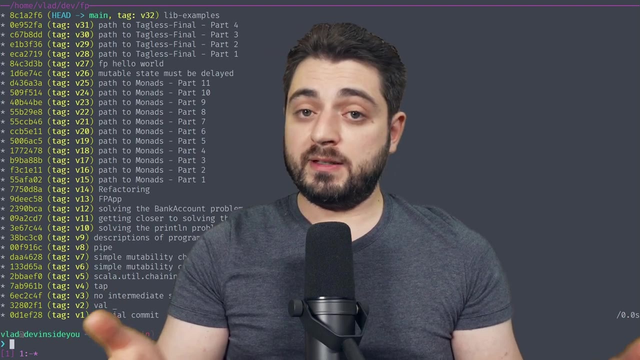 3 came out. uh, and you know, only the time will tell um how it behaves. you cannot go wrong with cats effect 3 um xeo is probably, like the, the youngest one of them. however, the youngest also means a couple of years. um, just a couple of weeks ago, xeo 2 came out. and again, only the time will. 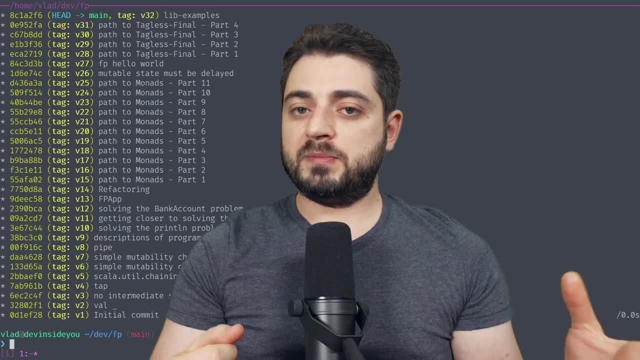 tell how good it is. uh, xeo is slightly different from the other two in how it handles errors, and it's a little bit different from the other two in how it handles errors, and it's a little. and also, uh, it has an optional way to do dependency injection differently, but you don't. 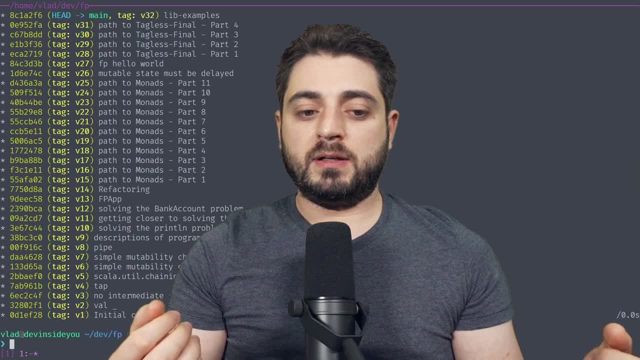 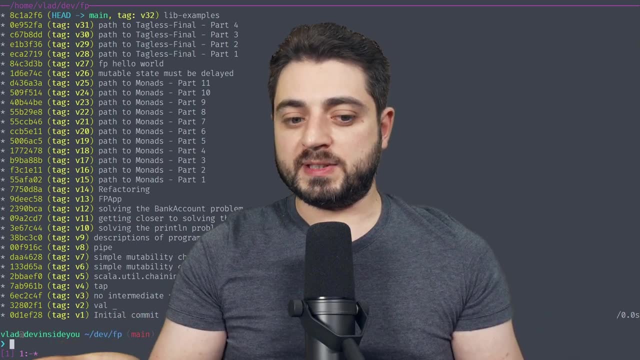 you don't need to use it. tagless final, it's kind of fading away, um, at least in my opinion, uh, because in my opinion, uh, it's not really, it's not really worth it. because, like the big, the really big fear was that, you know, some of these libraries are going to die, not going to be maintained anymore. 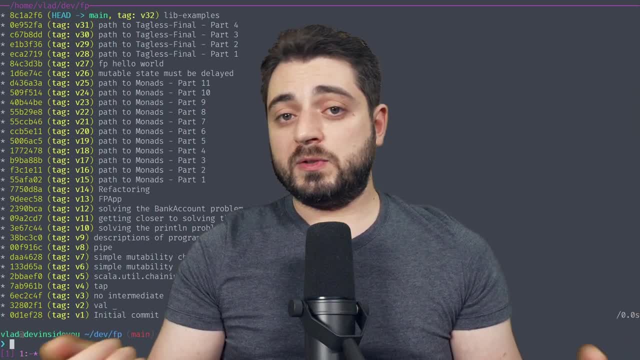 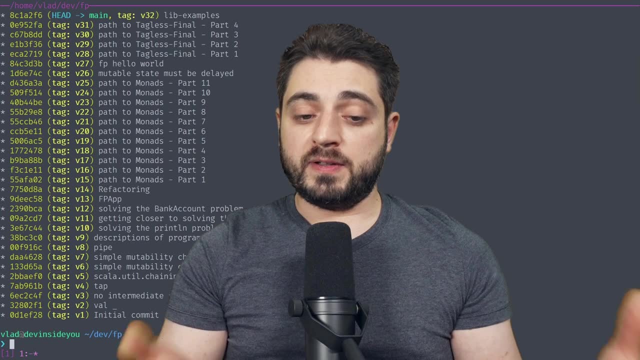 i'm betting on xeo. it doesn't look like it's going to disappear anytime soon. uh, you know, in the previous video that i made was for season scholar developers and over there pretty much said that you know Zio is winning, but it's not. like you know, it was not an easy fight and it's. 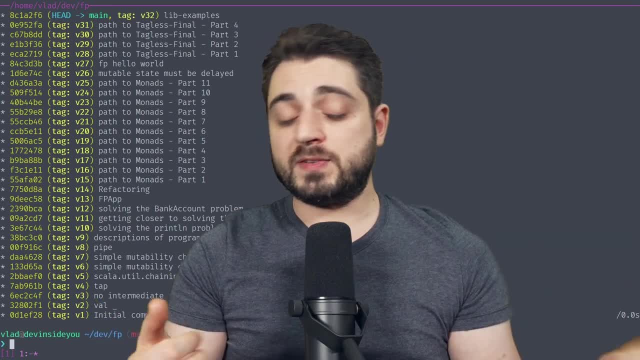 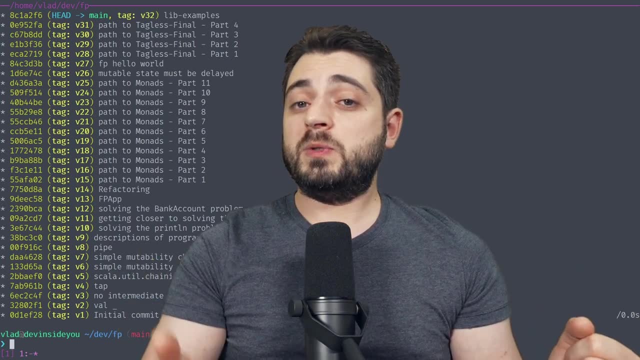 not an easy decision to make, whether to use Zio or Cat's Effect or Teclis Final. However, I would still choose Zio, because Teclis Final, to me personally, is just not worth it. However, you are a beginner and as a beginner this decision is much easier. Zio is much easier to learn, It's 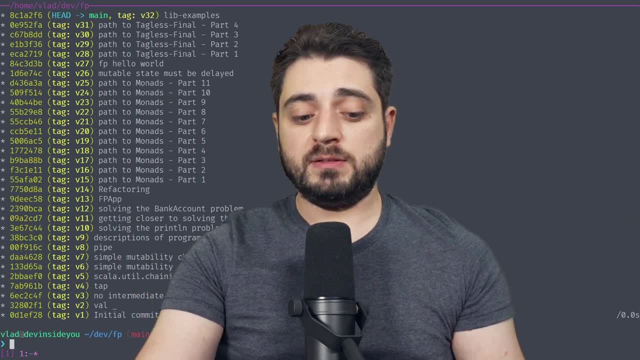 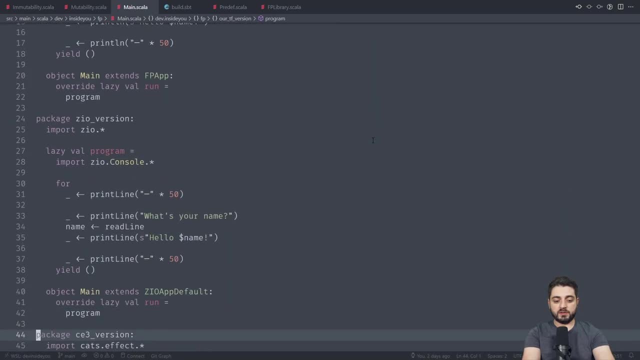 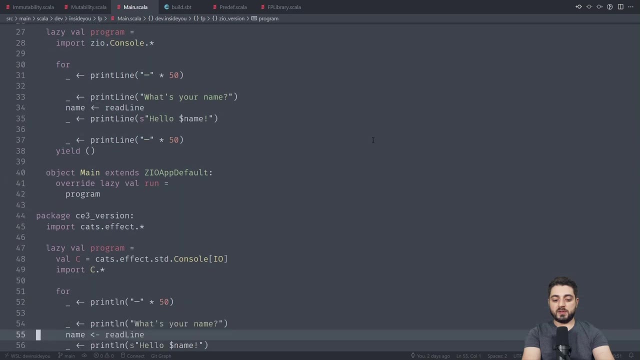 more beginner friendly. Even if you just look at what we just did, you know the Hello World, even just the Hello World in Zio, which is over here, is the most pleasant one out of the three. Okay, So it's more pleasant than the Cat's Effect, because you have to obtain the console in some 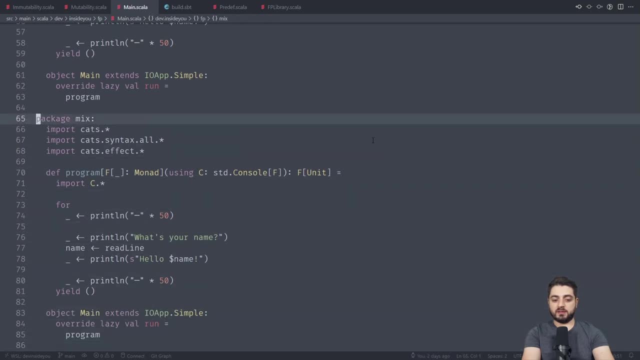 weird way And it's more pleasant than Teclis Final because you need like extra imports, You need to understand like type classes and all this relatively heavy Scala syntax and intrinsic details. But yeah, but this is mostly just a personal preference. Like in the previous video, for example, I said that 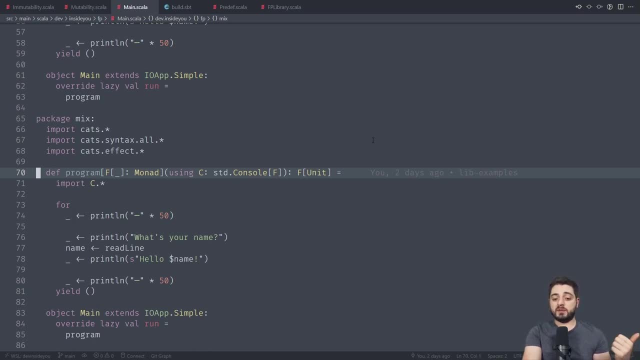 you know, if you already have a big code base in Teclis Final, you're not going to gain too much, you know, from rewriting it to a concrete effect type like Zio, for example. But if you're starting fresh, I would start with Zio. All right, Now, as I already mentioned, this repo is going. 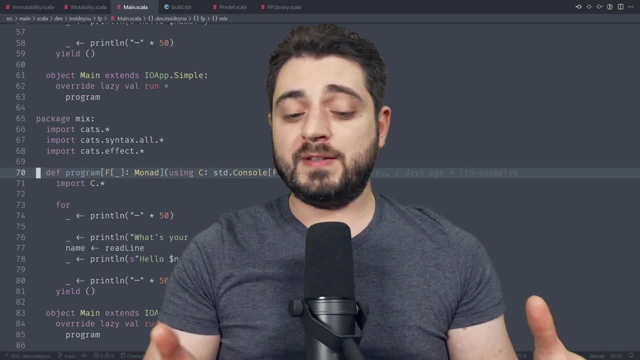 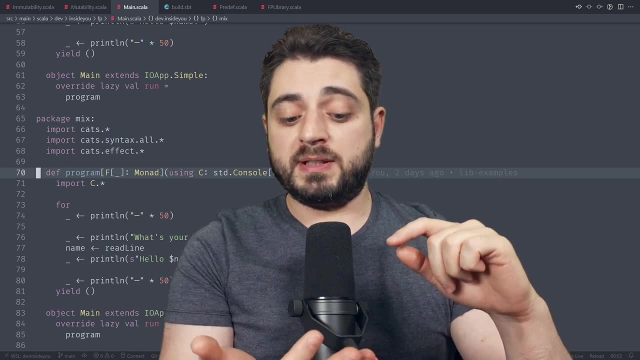 to be on GitHub. And also, if this was too fast for you, I have videos about all of these things. I have a playlist about Teclis Final. All of them are here on YouTube free playlist. So I have a playlist about Teclis Final. I have a playlist about Zio. I even have a 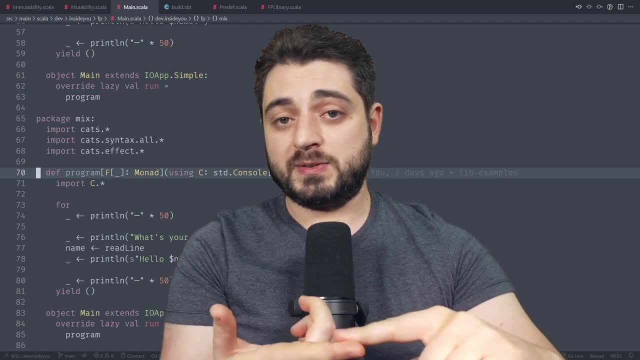 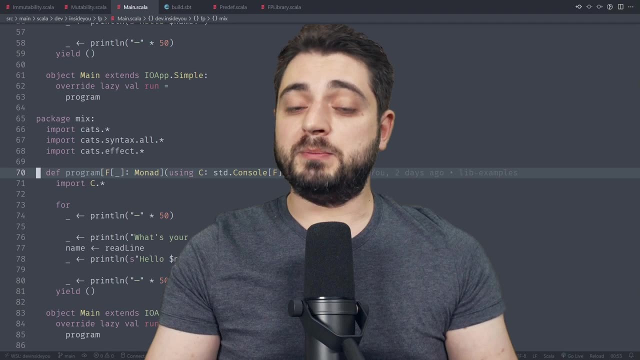 series about Git. I have videos about, you know, ZSH, where I use, like all of these alias. I have videos about all of these kinds of things, right? So don't forget to subscribe. even. you know, hit the bell if you want to be annoyed by the notifications. And, you know, if you stuck around, 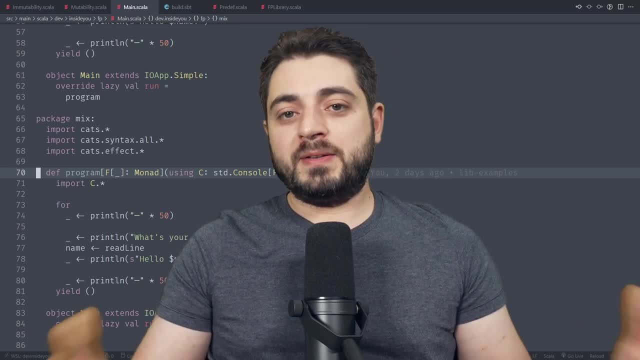 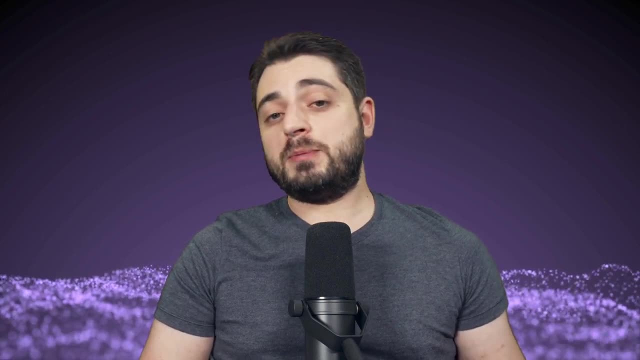 for so long. you obviously liked the video, So please hit the like button. All right, I hope you enjoyed this video. I'll see you in the next one And for now, as always, it's been Vlad from devinsideucom. Don't forget to like this video if you did Subscribe, if you're serious about